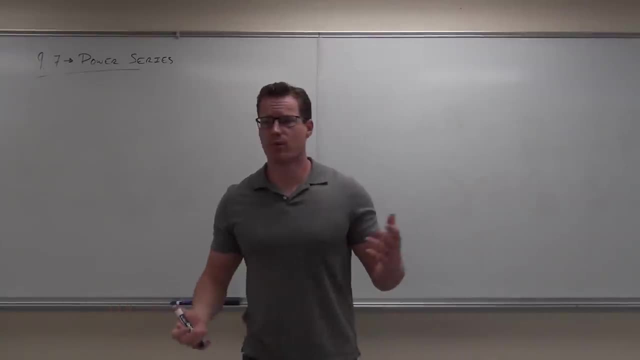 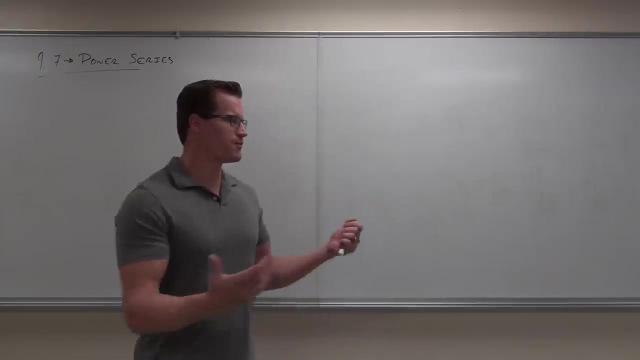 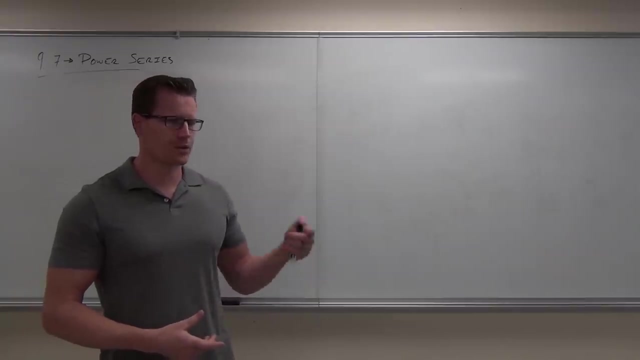 Okay, so moving on to where the rubber hits the road, Why we dealt with the series in the past few sections is because we want to talk about power series and what these things are. So real quick, brief explanation of what a power series is. What a power series is is a series with some variable in it, Not like n, but like x, Like our typical variables- that's being raised to some power. That's why we call it a power series, because we have a variable raised to some power. Let me write that down for you. 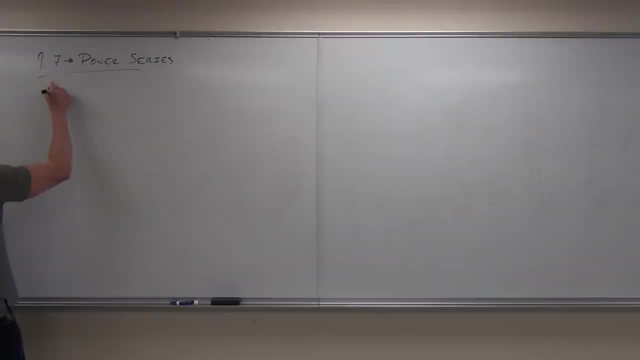 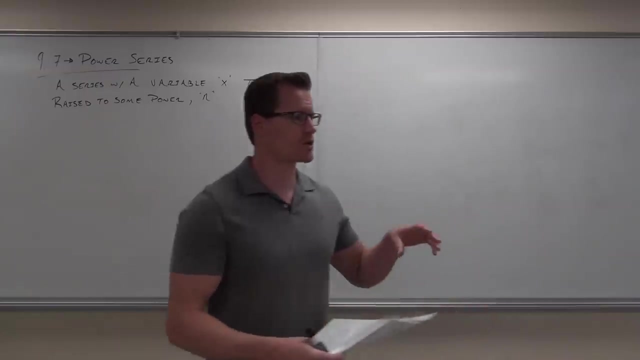 Let me write that down and explain what they would look like. So a power series: it's simply a series with a variable x that is being raised to some power, And that power is based on n. Now what we're going to talk about in this class are two types of power series. We're going to talk about power series centered at zero and we're going to talk about power series centered at some constant c. 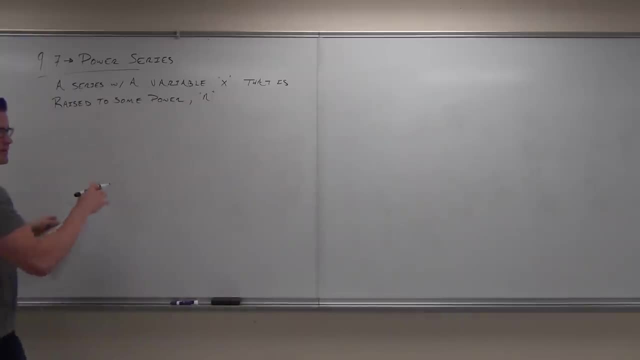 So there's two types we talked about. Other than the fact that they're centered in different places, there's really not any difference between them. So there's two types of power series. Power series is a series with a variable in it. 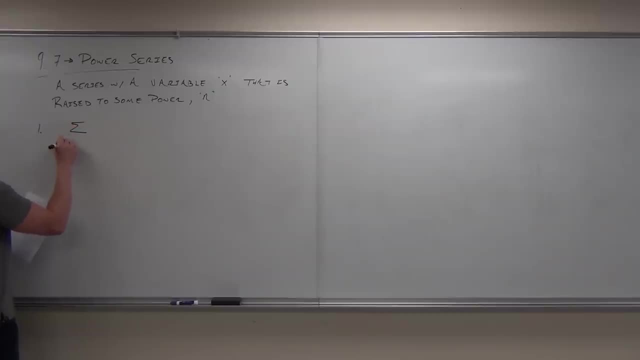 Power series number one. Power series number one looks like this: It's a, and this is going to look very interesting to you because you've never seen it before. It's a series. We start them at zero, So the first term starts at. n equals zero, typically. 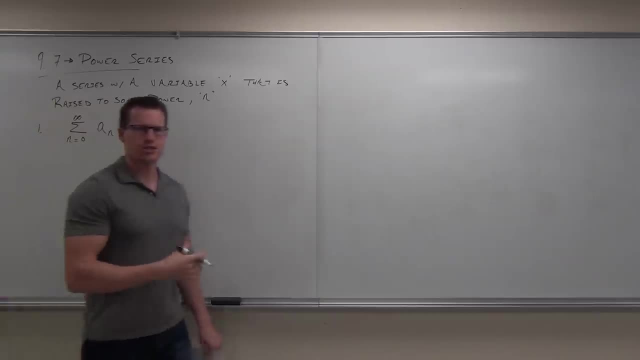 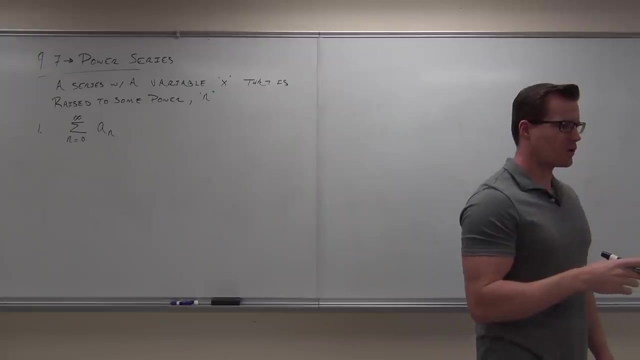 And what it's going to look like is: well, that would be just a normal series, wouldn't it? Just a sub n, Something like I don't know, n squared over, n cubed plus one. That's a type of a sub n or whatever we have. 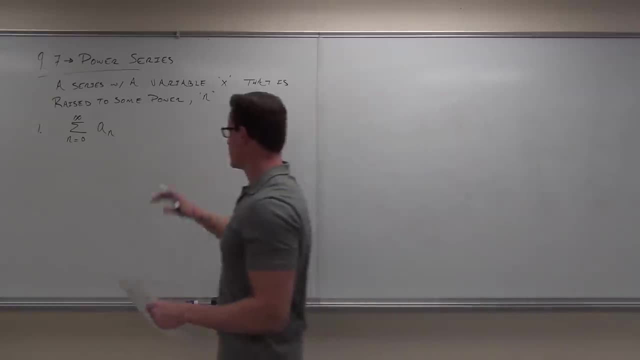 We've had many of them, Ln over square root of n, whatever. We've had a lot of different types of sequences from where we get our series Now for a power series. the difference between what we've done before and what we're doing now is, instead of just having this, we also have a variable raised to some power. 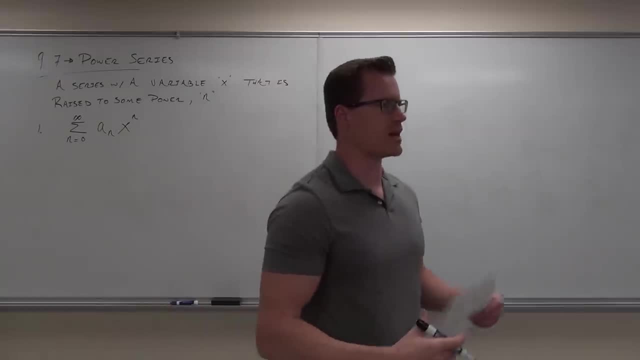 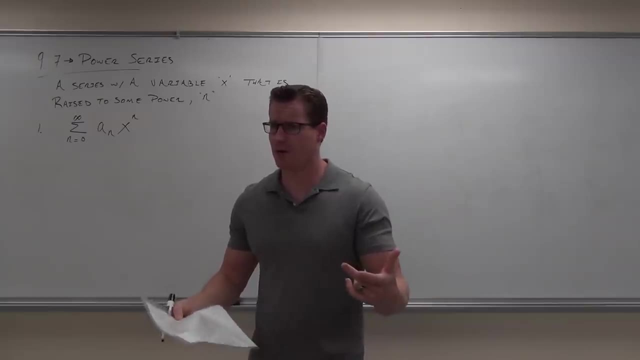 That's what's giving this idea of a power series. It now has a variable in it. Does it make it harder or easier? It's just different. It's going to use a lot of the same concepts that you already know. We're still going to be doing things like 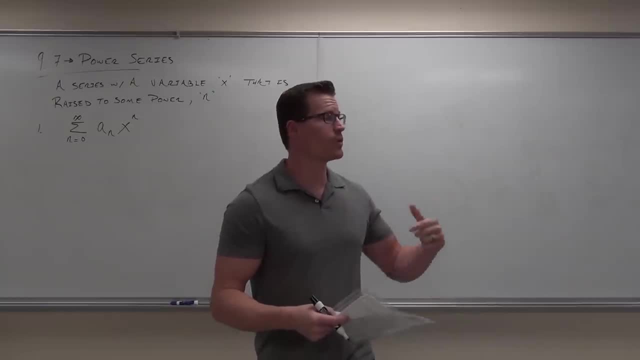 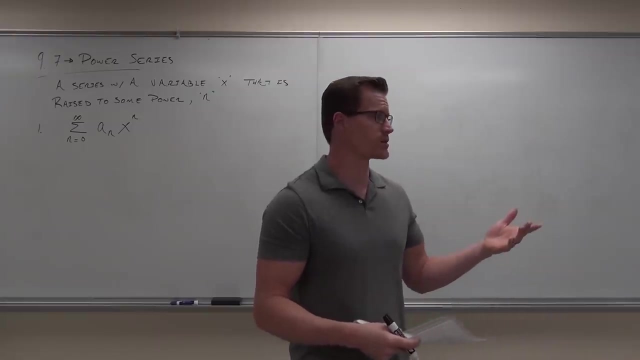 the ratio test and absolute convergence and all sorts of that stuff. We had to have that, and you're going to see why as we go through this section. okay, So when we get down to checking for endpoints, when we get down to radius of convergence, when we get down to finding out whether these are convergent or not, we're using the same tests. okay, 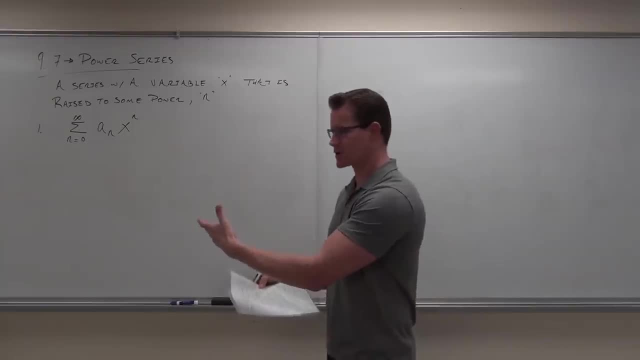 It's all the same stuff, So we had to have all that so that we could accomplish this section. So let's talk about what this would look like, Just the first couple terms, how it's going to look, Where do we start these power series? 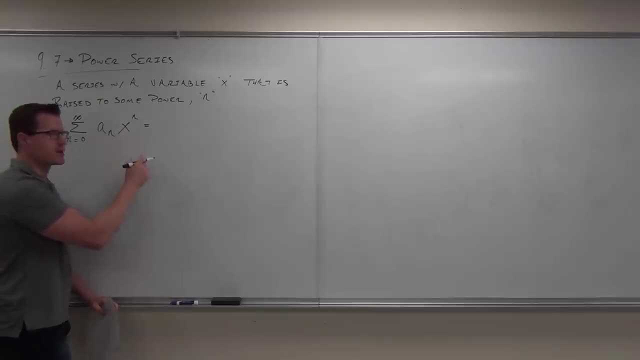 So if I plug in zero- well, I don't know what this is explicitly, but I know it's going to be a sub zero, True, Yeah, And it'll be x to the zero. What's x to the zero? 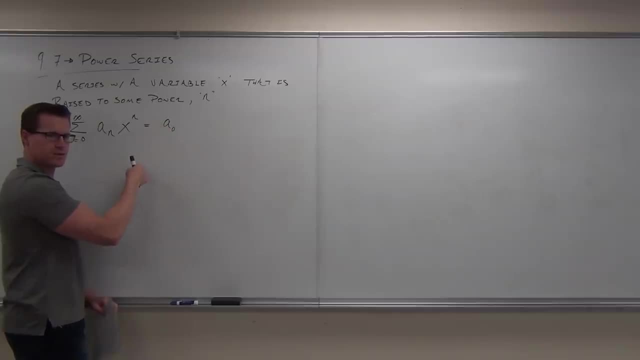 So our first term is simply going to be a sub zero. Are you with me on that one? Yeah, And we're going to okay. plus, it's not alternating typically, unless we have something in our a sub n that makes it alternate. 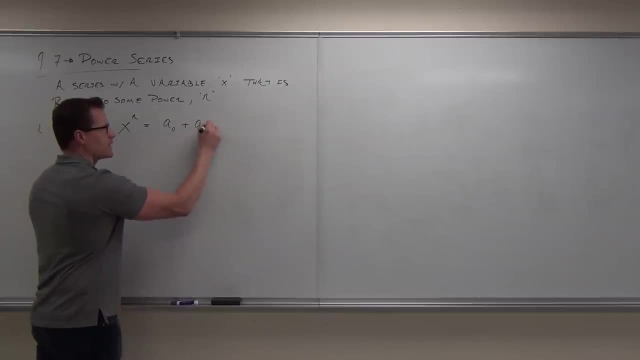 Plus, I would plug in one and I would get x to the h first. Good. And then I would plug in two and I would get x to the second. I'd plug in three and I'd get x to the third, and so on and so forth. forever and ever, and ever and ever. 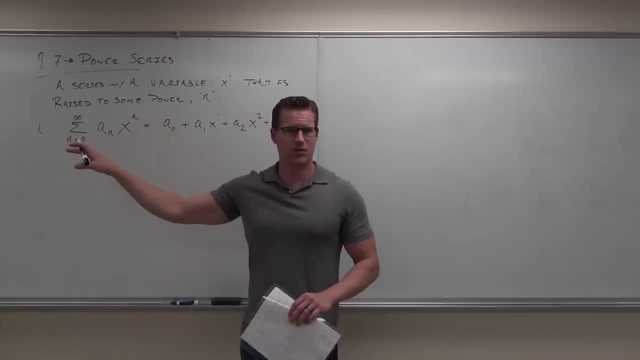 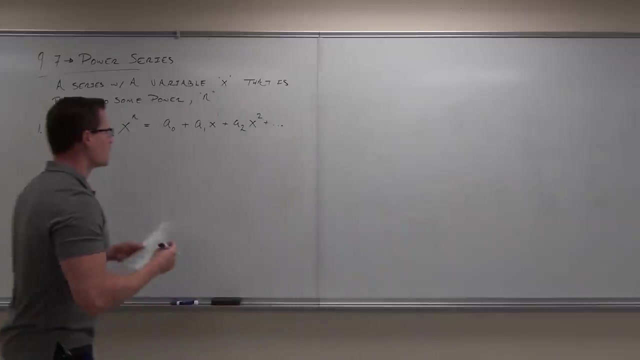 because this thing stops at infinity. You guys okay with that so far? Yeah. Now just a little heads up. I want you to think about functions. Do functions ever stop? No, No functions go into it. So right now, what we're doing here is we're actually defining a function which is interesting, and we'll talk about that in a minute. 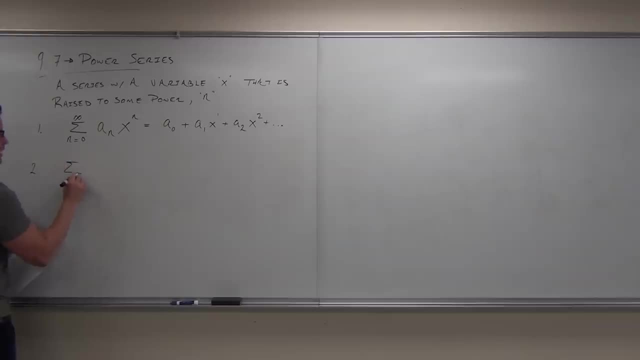 So number two, The other type of power series you can have, is one that's centered. Oh, you know what? I forgot to tell you a little something. I mentioned it, but I want to write it down for you, to make sure you have it. 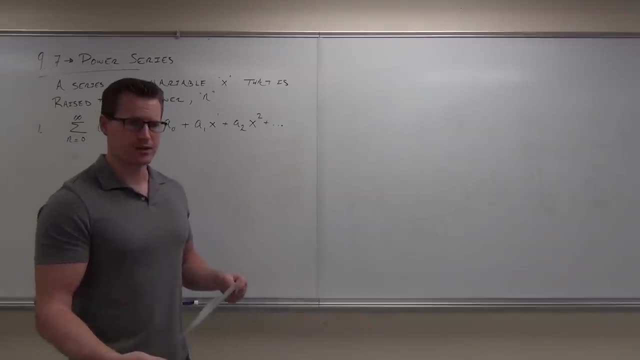 What this is. this is a power series in the variable x which is centered at the origin. The origin would be our zero. I said centered at zero, centered at the origin. You can use it interchangeably: This is centered at zero or centered at the origin. 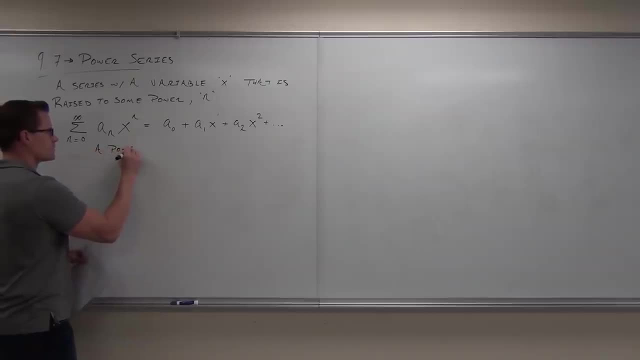 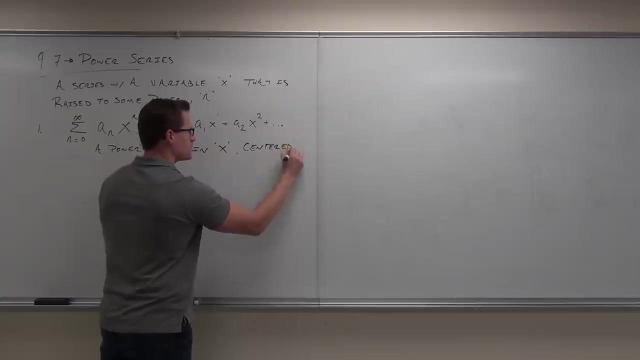 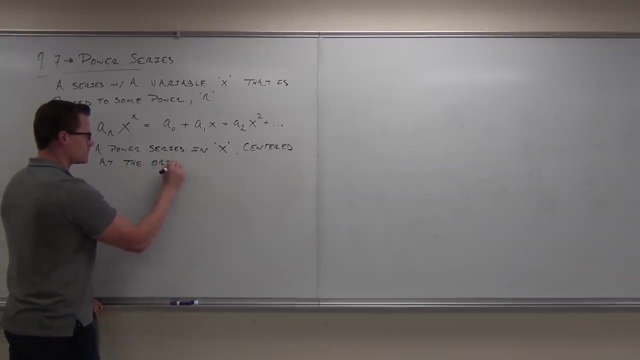 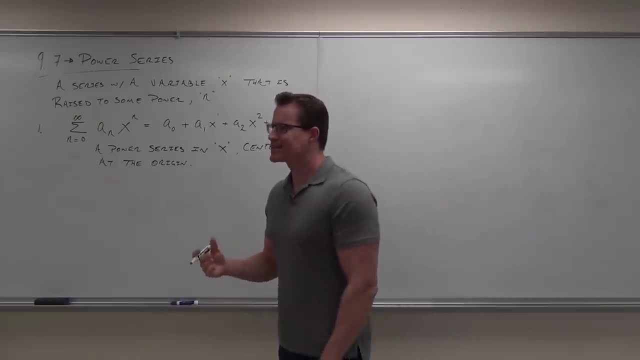 So this is a power series In x, which is our variable. this means it's a power series based on the variable x, which is centered at the origin or zero. Why is it centered at zero or centered at the origin? Why is it centered there? 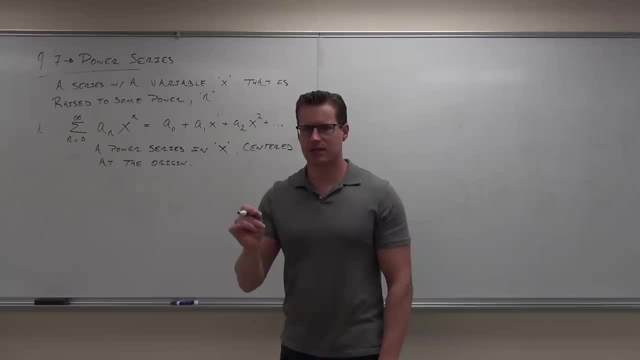 I want you to look at the x. Is anything being added or subtracted from the x? So zero is being added or subtracted from the x. Nothing is being added or subtracted. Therefore it's centered at the origin or centered at zero. 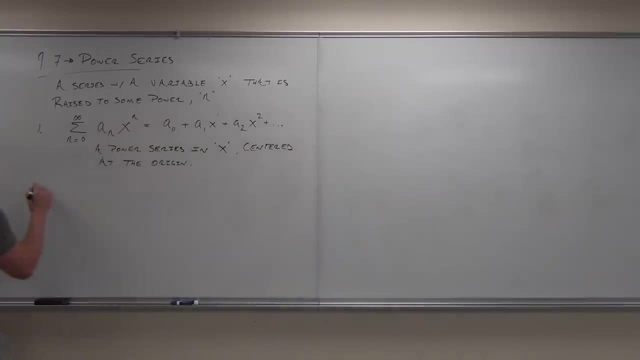 Quick head note, if you're okay with that one, Compare it to this. Suppose I had a series started at zero, never ending a sub n, x minus c to the n. Of course the first few terms are going to look really similar to this. 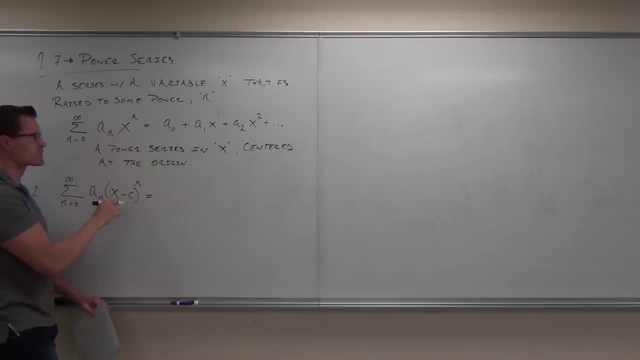 Let's check that out and then we'll consider the differences between our series themselves. If I plugged in zero, I'd still get a sub zero, I'd still get x minus c, but this is going to be raised to the zero power. 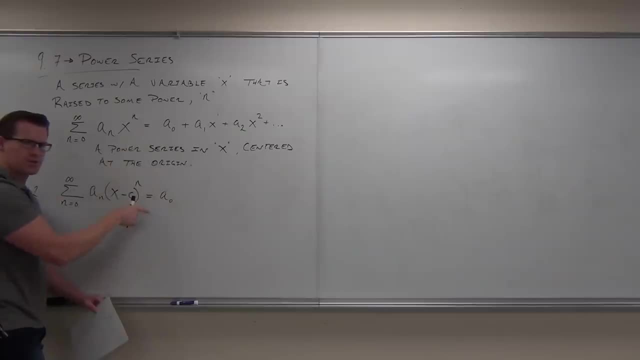 What's anything raised to the zero power One? So it starts out exactly the same. Do you see why? Mm-hmm Plus, I'd still have a sub one, but this time, instead of having x to the first, I'm going to have x minus c to the first. 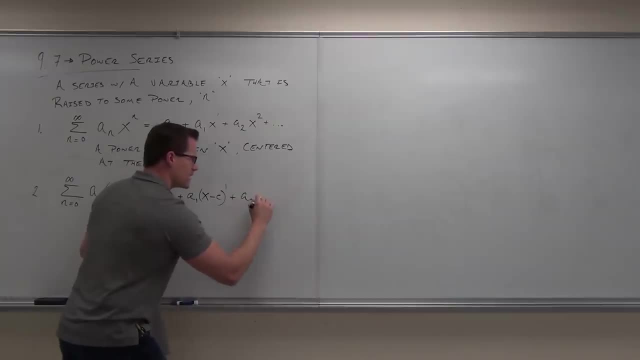 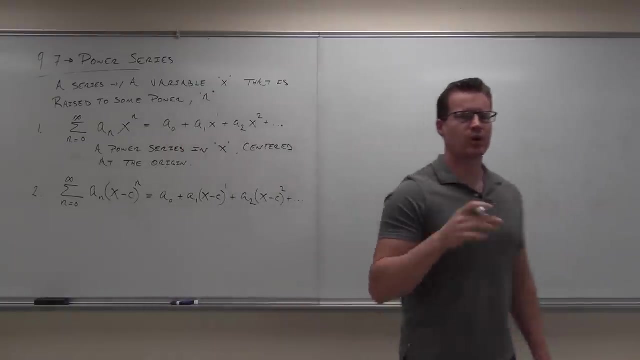 Instead of having a sub two times x to the second, I'm going to have x minus c to the second. Other than that, there's not any change. Okay, There's no change to it, It's just where this thing is centered. 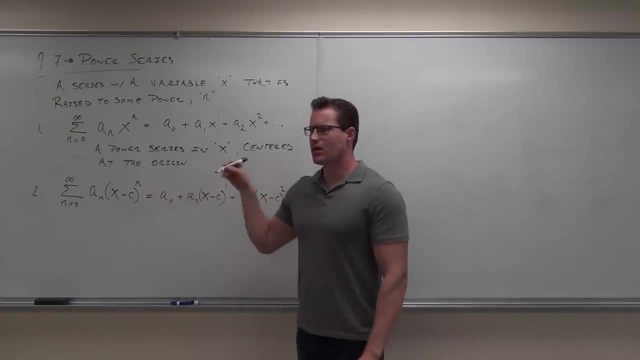 So that little c that says x minus c. that c is what your center is. So if I have minus three, we're centered at three, If I have plus two, we're centered at negative two. Did you catch that? 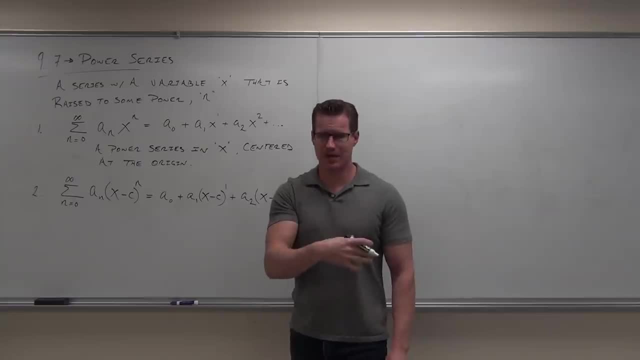 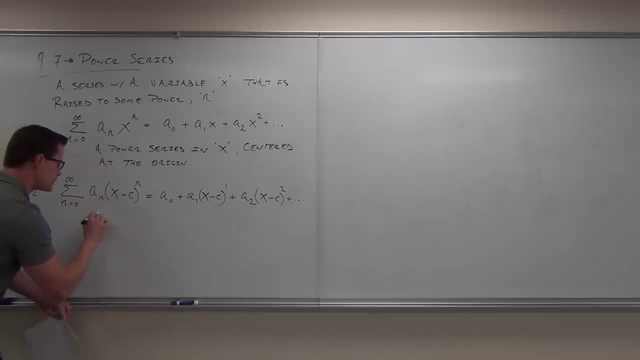 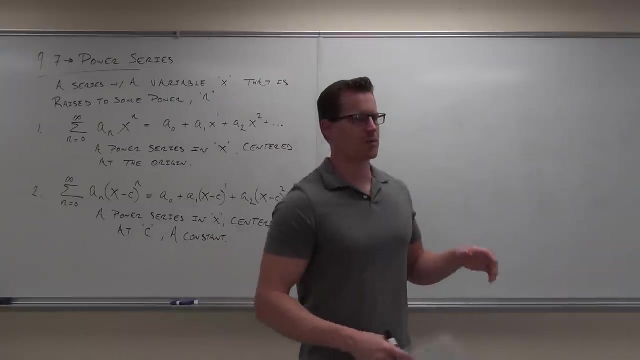 Are you sure? Because it's minus c, so minus negative would make that plus for us. So, anyway, we have a power series in x still, but this is centered at c. Where c is, it's a constant. Now, of course, I'm going to give you some examples in a little while, and we'll talk much more about this as we go through. 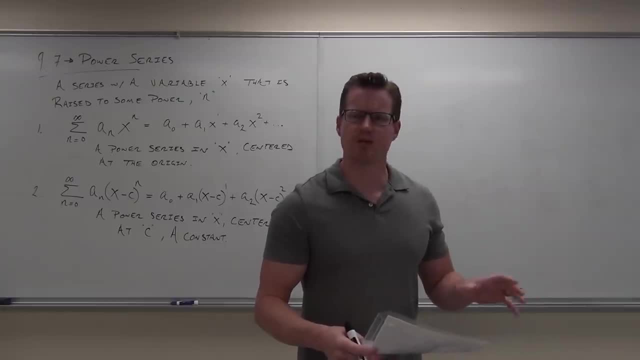 But for right now, we're not going to work with these things. I just want to give you examples of how they look. Would you guys like a couple of examples of how these things look real quick? Okay, So here's an example. 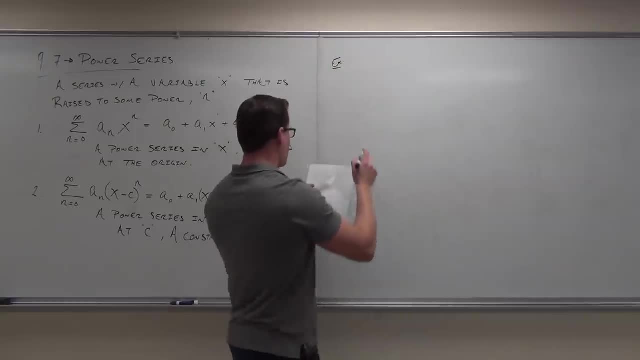 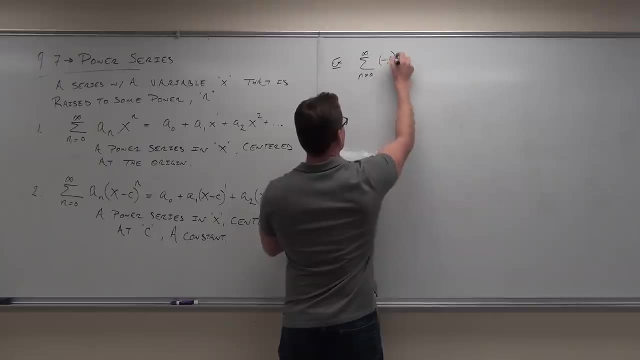 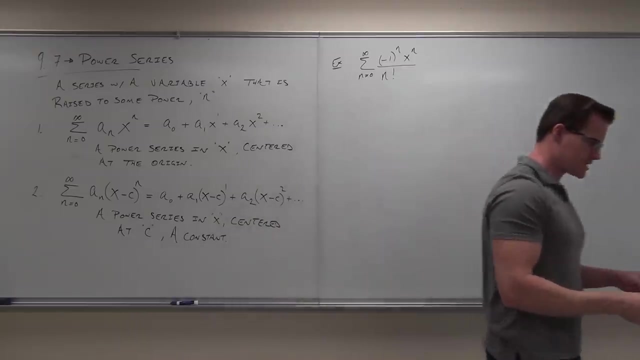 Just for a few terms. we'll see what these things are doing And, of course, we'll talk a lot about them as we move forward. You know, the first thing I want to know, I want to know if you can tell that this is going to be a power series just by looking at it. 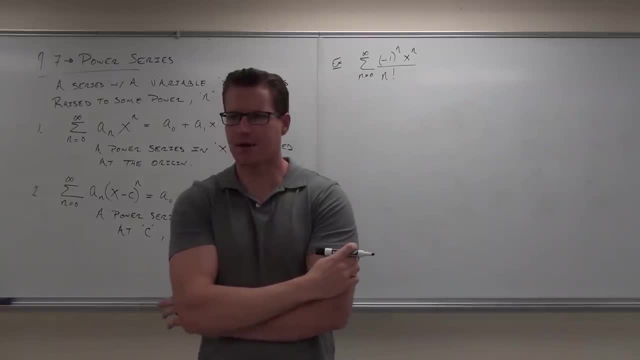 Can you tell it's going to be a power series just by looking at it? Yes, What's it got there that none of our series before has had? I mean, it's a variable being raised to a power. That's a power series. 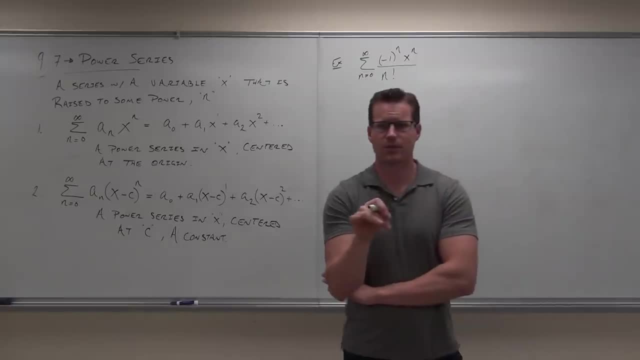 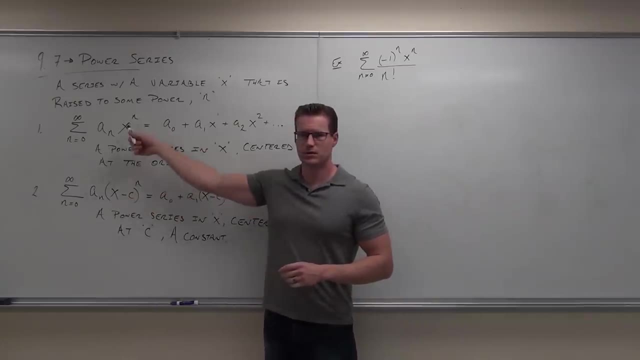 Now quick question: Do you think this is going to be centered at 0 or centered at some other number, centered at the origin or not? What do you think? Does it look like number 1 or number 2?? It looks definitely like number 1, because we have nothing being added or subtracted to our x itself. 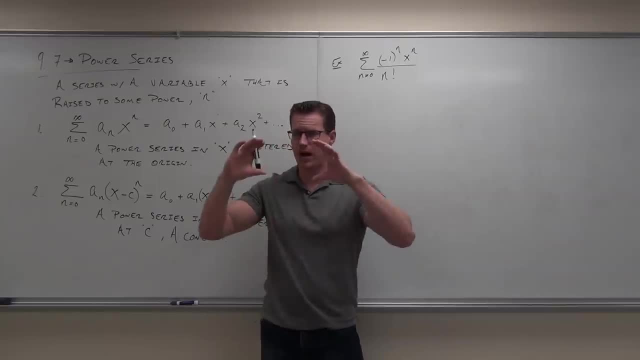 If it's not centered at the origin, it's going to be x minus or x plus something, Not sure if you understand that, Okay, Also, can you pick out my a sub n from here? Can you pick out my a sub n? 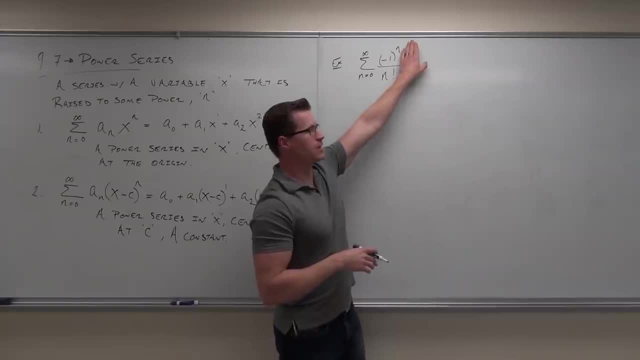 What is it? Just cover that up, And that's a sub n. That's it. So this is the sequence, right, that we're getting our series from, And then, after every term, we're just tacking on an x. 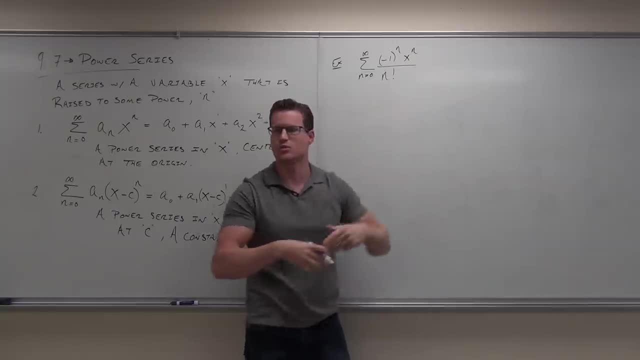 x to the 0,, x to the first, x to the second, And that's what's given us our power series. So really, if we wanted to do this, we could write out just the sequence here and put x to the 0.. 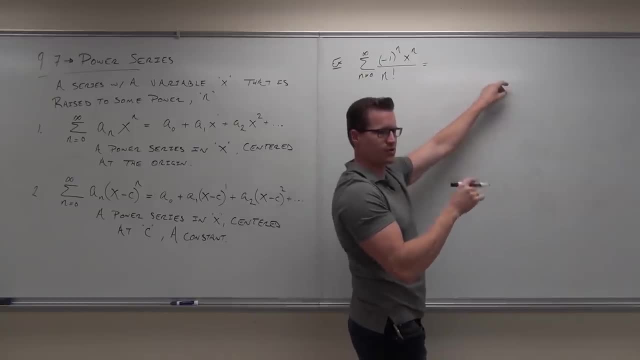 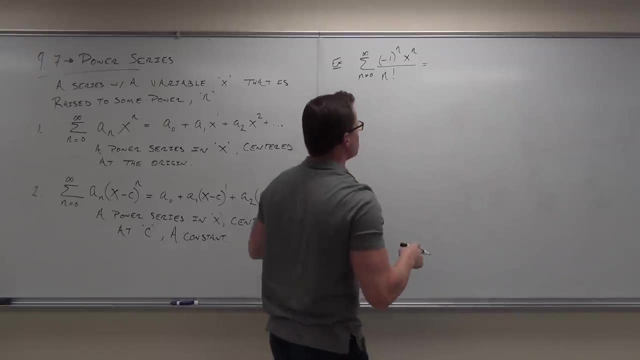 x to the first, x to the second, x to the third, after every single one of those terms And we'd have the appropriate series. Now, of course, we're going to do this all at one time, But let's try it just for the first few terms. 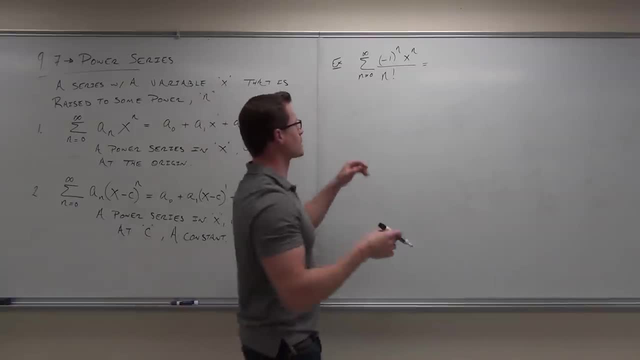 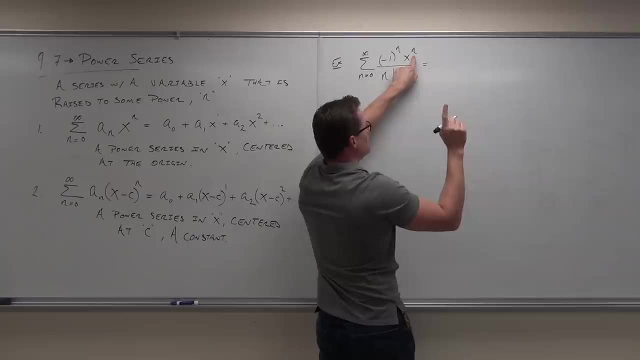 Where do I start again? 0. Let's plug in 0.. What's negative? 1 to the 0? 1. 1. So we're going to have 1.. What's x to the 0? 1.. 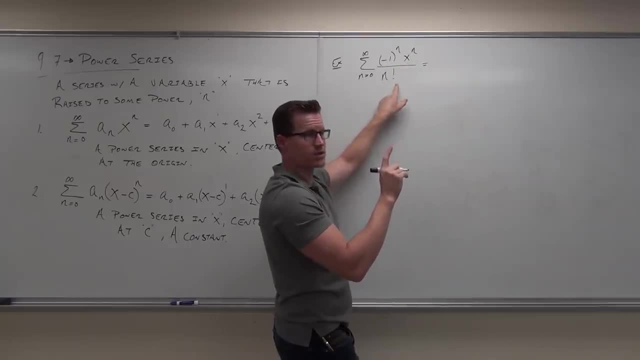 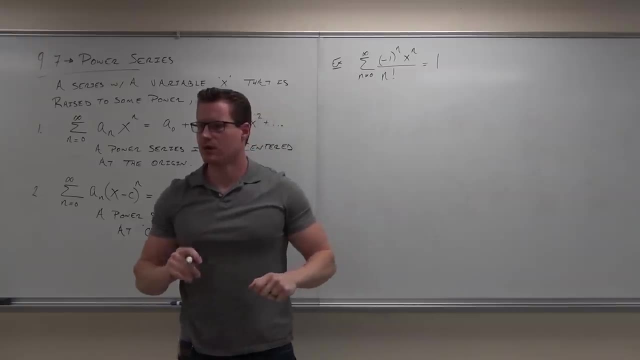 And what's 0 factorial? 1. 0 factorial is defined to be 1. if you didn't know, that is 1.. So our first term here is 1. 1. 1. You OK with that so far? 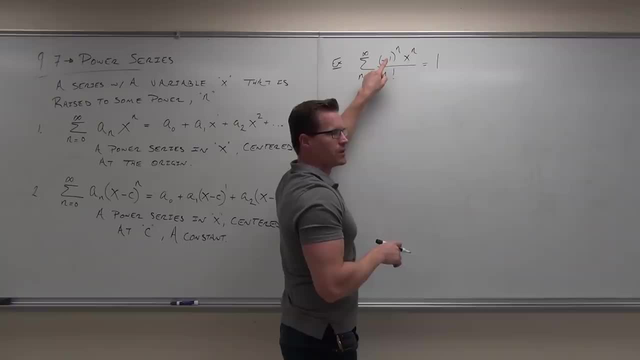 Next term, Let's plug in 1.. And if you plug in 1, what's negative? 1 to the 1? Negative 1.. So I know I'm going to be subtracting. Hey, what type of a power series is this? 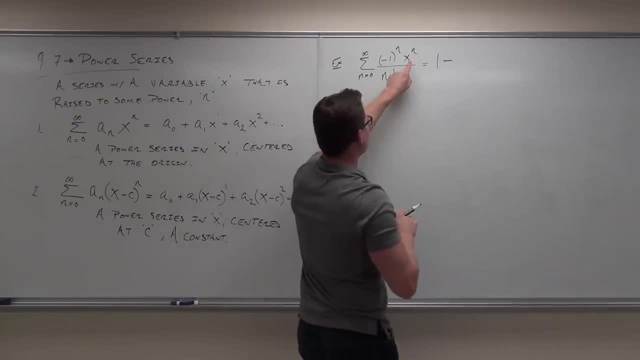 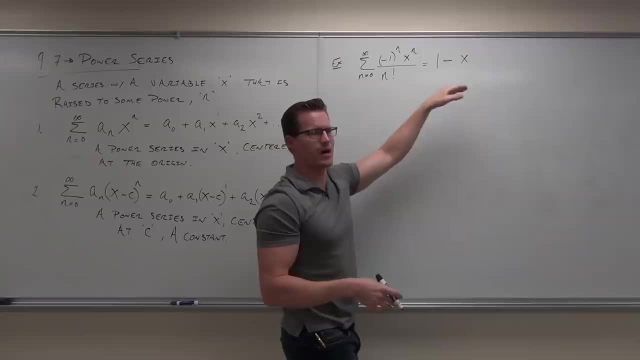 Over 1 factorial. You could put the 1 factorial here if you just want to see the pattern. OK, So right now we just have x, But if you put 1 factorial, you're going to see the pattern in just a minute. 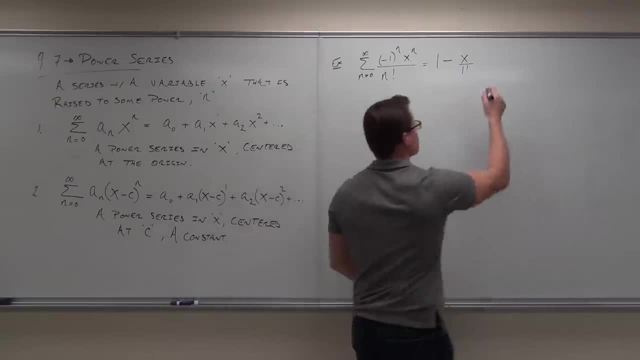 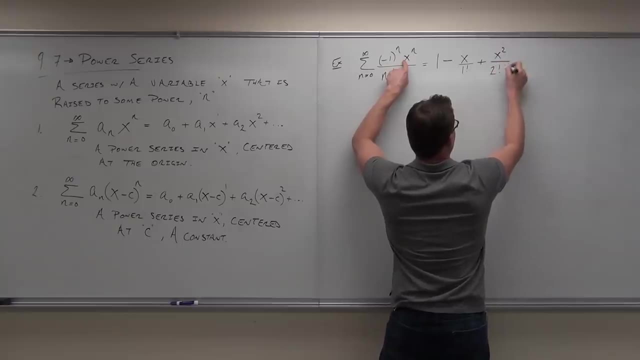 Next one: Is it going to be plus or minus? everybody Plus Sure, And what we'll get is 1. 1. x to the second over 2 factorial Good Minus. x to the third over 3 factorial plus. 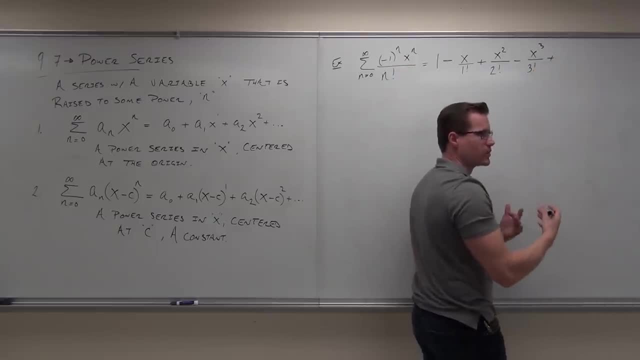 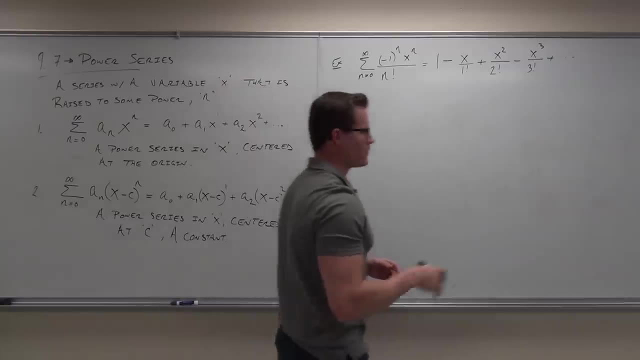 And do you see the pattern? It's easy to see the pattern once you get the first few terms. That right, there is the first few terms of our power series. Let me give you the next one. I'll make a couple statements about this. 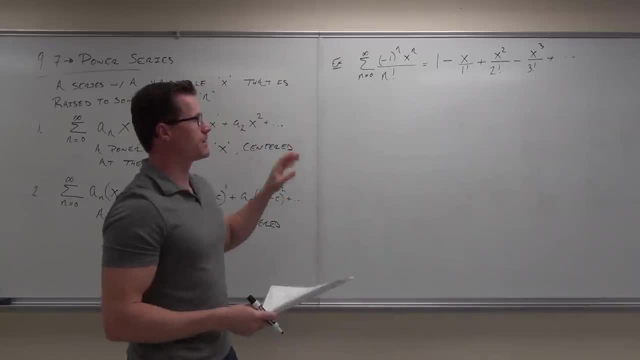 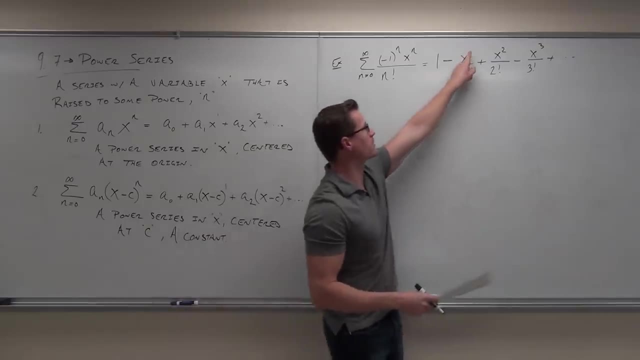 I do want you to understand that this thing is centered at the origin there. Have I made that very clear for you? Yes, So it's a power series. no problem, because it's got x to a variable. You notice how the variable here is 1,, 2,, 3, blah, blah, blah, blah, blah. 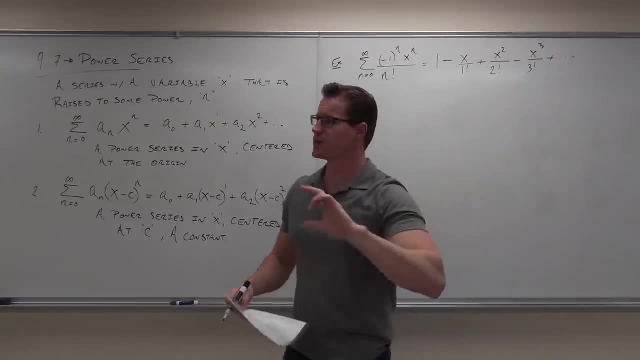 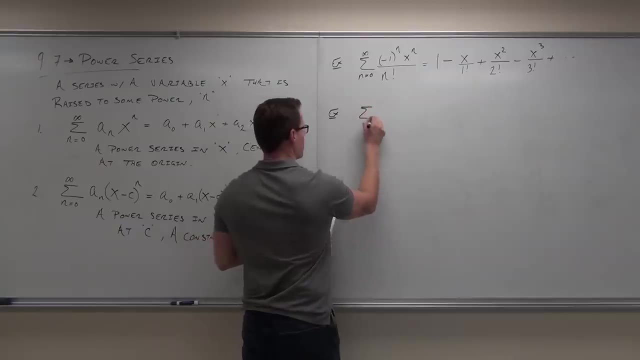 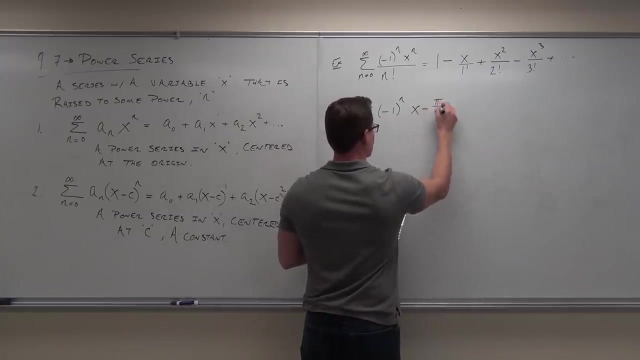 It's going to continue and continue. We have it centered at 0 because nothing is being added or subtracted from our x. Now compare it to this next one. What's that going to do for us? Okay, It might look a little nasty, but don't worry about that right now. 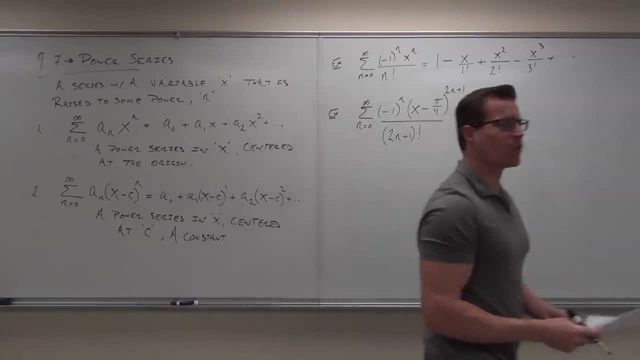 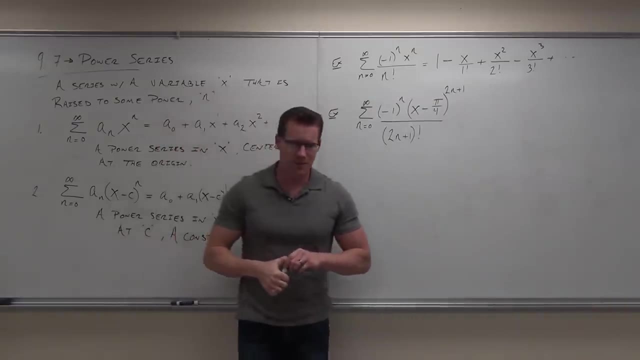 We're just going to kind of talk about this one for a second. First thing, you notice, what type of a series is this? Is this a power series? Yes, What tells you it's a power series? A variable, It's a variable. 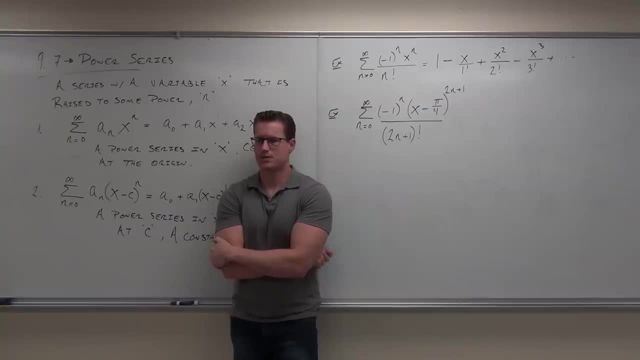 It's being raised to a power. Now let's see. Is this more like the number 1 or more like the number 2? Number 2.. So is this centered at the origin? No, Where is it centered? Pi over 4.. 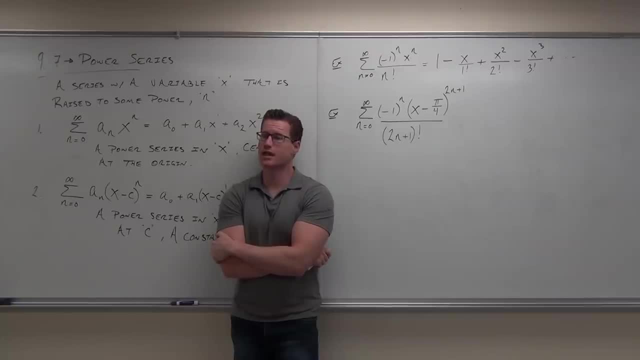 Very good. Do you understand why it's not centered at negative pi over 4?? It's x minus Right, It's x minus the center. Just like finding a root, Like if you did x minus 2, the root of a polynomial, x minus 2, means your x intercept is at 2.. 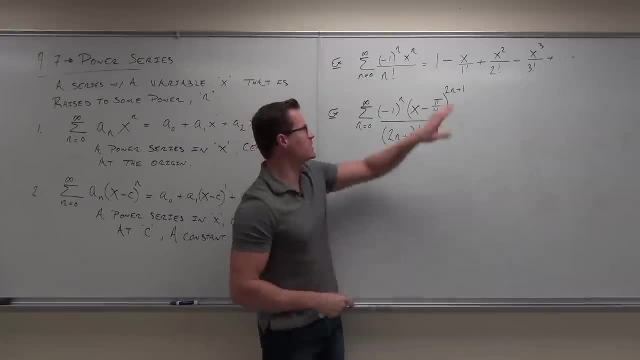 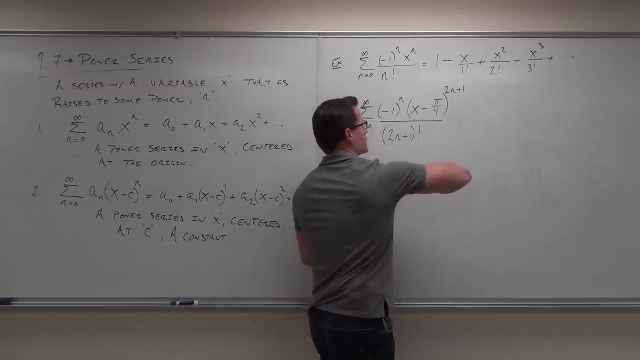 So that positive 2.. You can think about it like always a changing sign. Well, it's not really. It's defined to be x minus your center, so the center is pi over 2.. If I had had x, oh my god. sorry, I said pi over 2,, I meant pi over 4.. 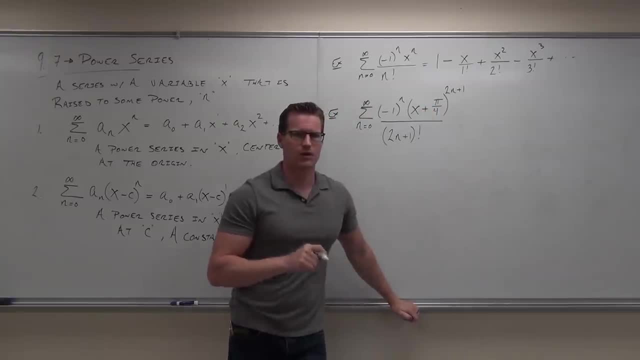 If I had x plus pi over 4, the center would be at negative pi over 4.. Very good, That's exactly right. So let's figure out a few terms here. What's the first thing we plug in? everybody? 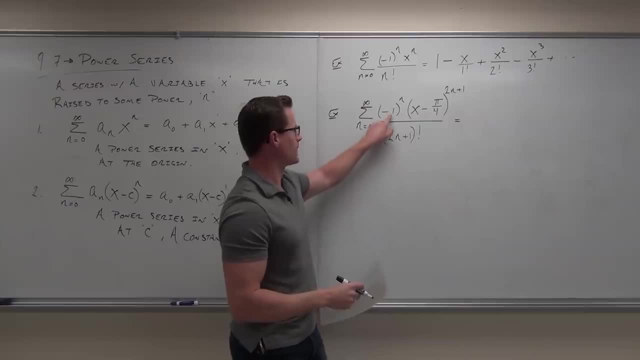 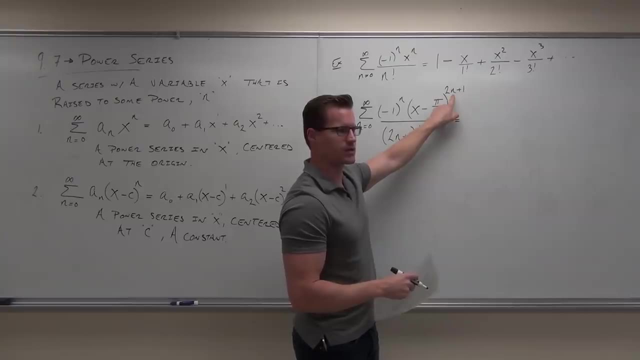 Zero. So if we plug in zero, we're going to get- let's see here One. There's one. Plug in zero, Oh wait, So am I going to start with? oh, that's going to be different than we had before. 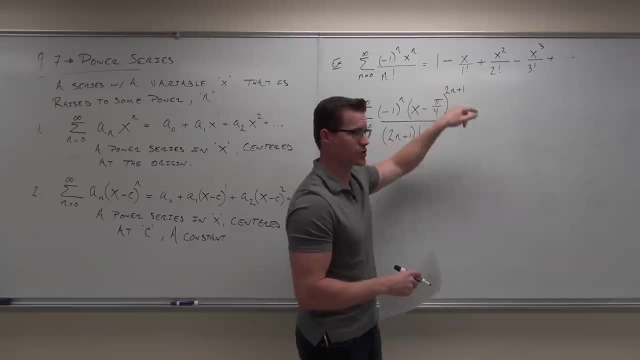 So this actually does something here. So don't just automatically assume we start at one all the time. That doesn't work. So this does give us one. This gives us well, two times: zero is zero plus one is one. 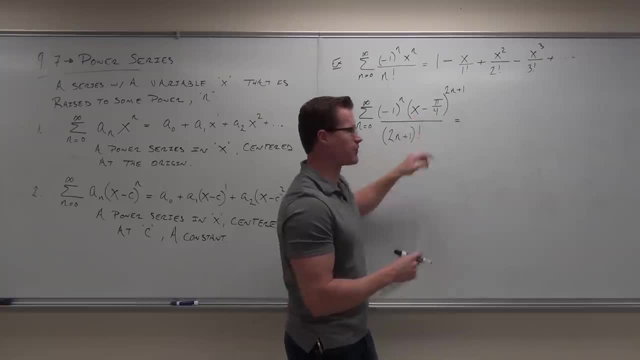 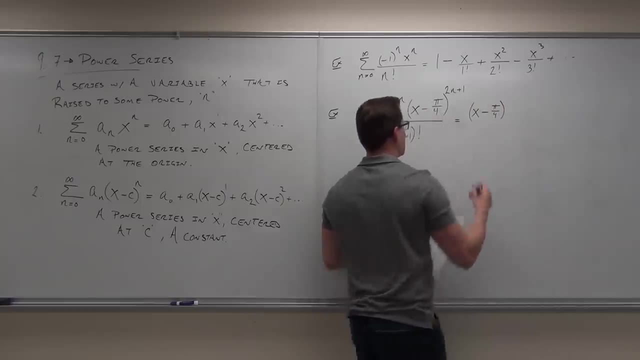 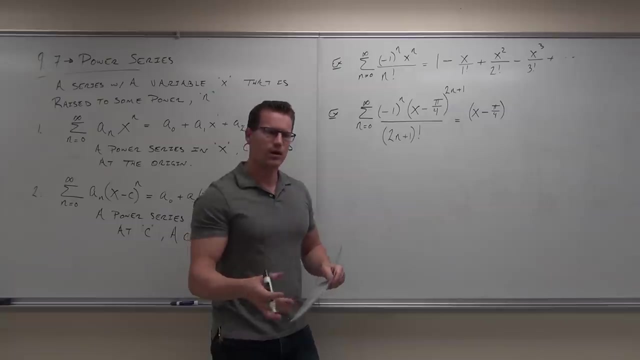 So we're going to start with x minus pi over 4.. If I plug in zero here, I get one factorial, which is just one. You guys okay with that so far, Yep, Next term, is it going to be positive or negative? plus or minus? 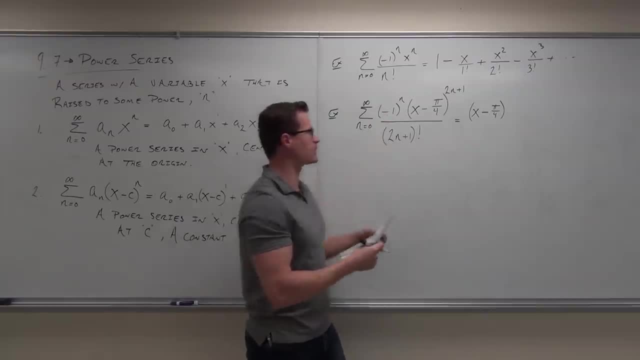 Negative And this is an alternating series because that thing is alternating, So we're going to get minus. I'm still going to get notice what happens here And what doesn't happen here. actually, are there any n's in here at all? 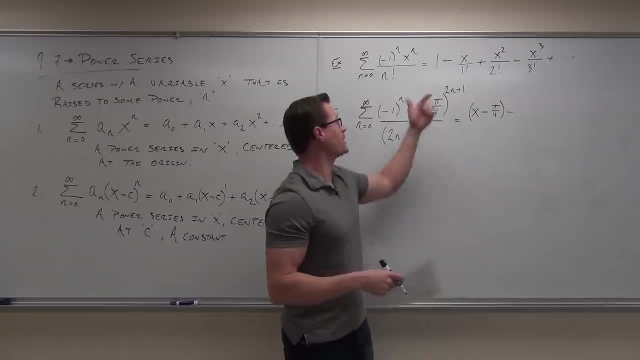 So is this thing ever going to change? No, No, it's not changing. So you're going to be writing things like x or x minus pi over 4, over and over and over again. The thing that changes is the power. 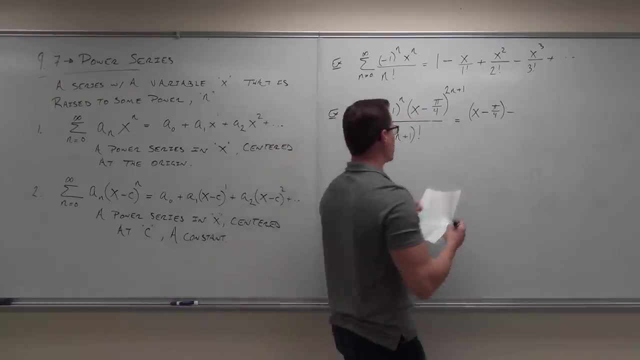 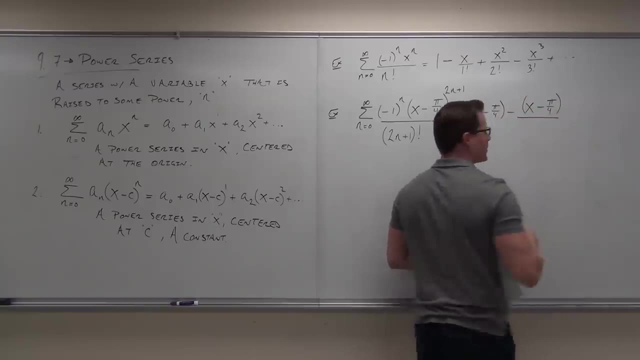 It's a power series. The power is changing of our variable and this denominator. So I still have x minus pi over 4, but my power is going to change and my denominator is going to change. What's my power going to be? 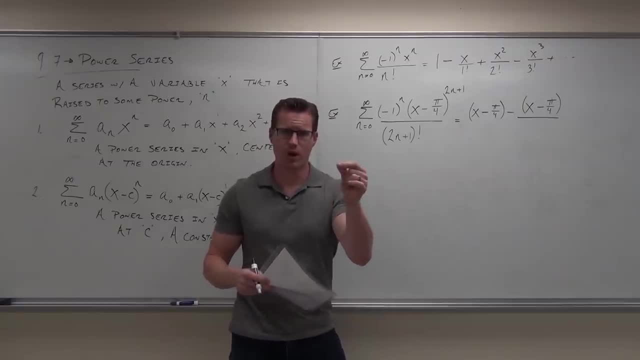 Remember that I plugged in zero first. I'm going to plug in Zero first. I'm going to plug in 1 now What is it? Zero first. So this is to the third over and notice how this is the same as this. 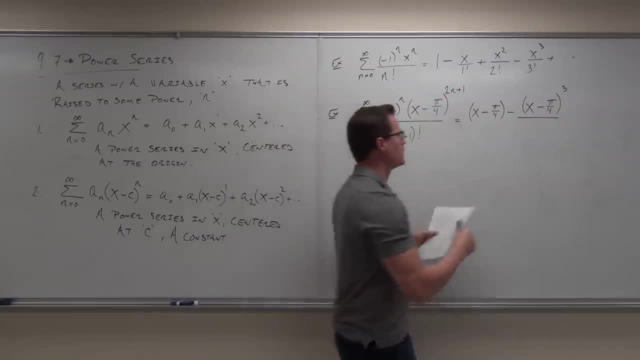 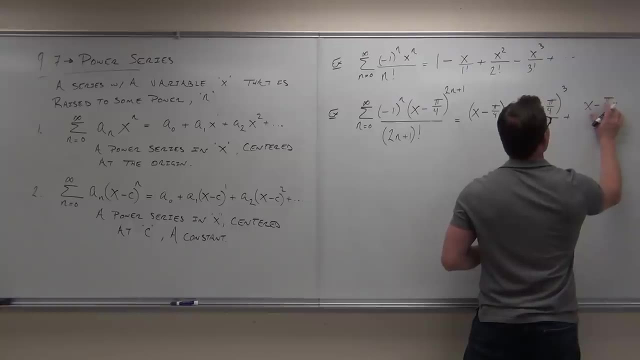 So if this is 3, this is 3 factorial. If this is 5, this is 5 factorial. Plus, we have x minus pi over 4 to the fifth over 5 factorial. What it's giving us is odd numbers. 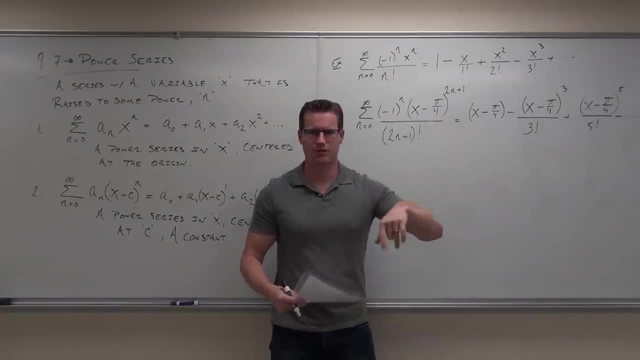 The next one would be: 7 over 7 factorial, 9 over 9 factorial. Does that make sense to you? That's our power series, centered at pi over 4.. Now we're going to talk about the theory kind of some notes behind this. 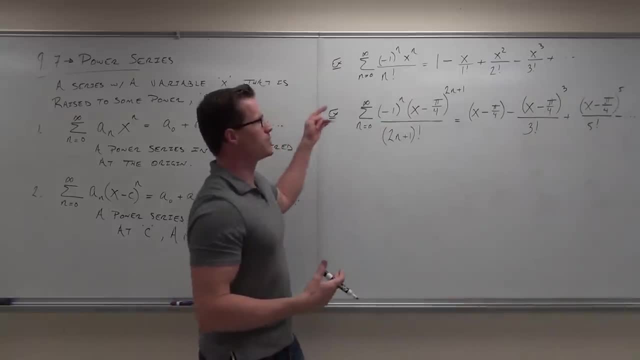 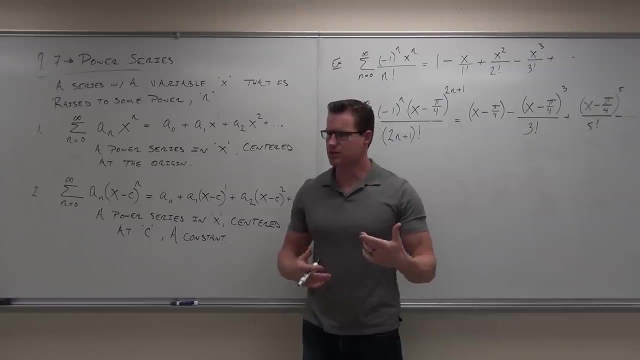 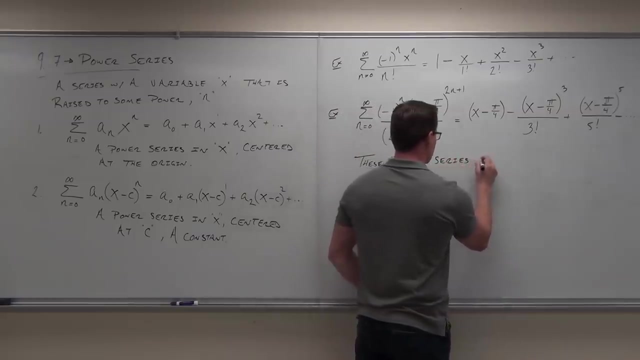 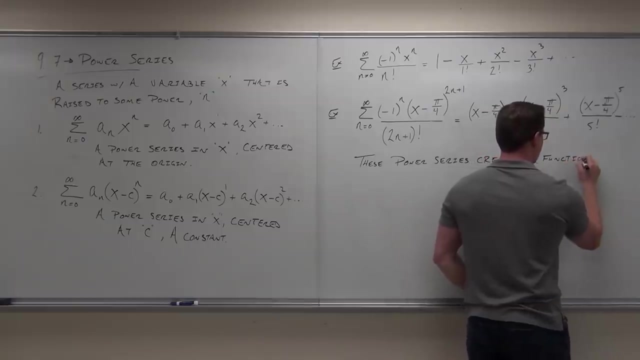 First thing: do you notice that when I'm doing this, when we're doing this, we're actually getting a function out of it? Do you see that We get a function based on x, so a function of x? These power series are all going to create functions of x. 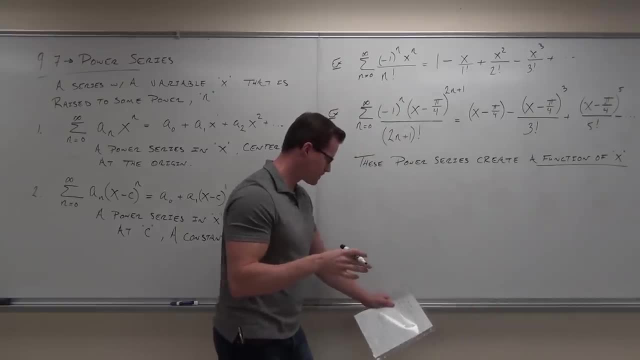 So if these things create a function of x, then what we can do all the time with our power series. do you understand that? what I'm talking about? a function of x, Yes or no? If I actually do the series, there's no more n's. 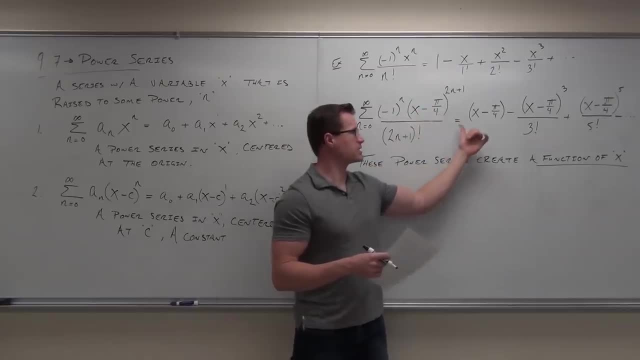 The n does 0,, 1,, 2,, 3,, 4,, 5, 2, infinity. What I get is a series of terms, all of which have variables in them, and that variable is always x. Does that make sense? 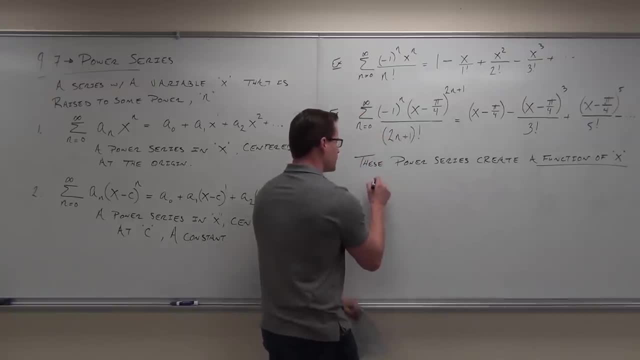 It's a function of x. So what that means is that I can define a function of x to be equal to a function of x. I can define a function of x to be equal to my power series. By the way, I'm wondering if you understand why I'm using this form of our power series. 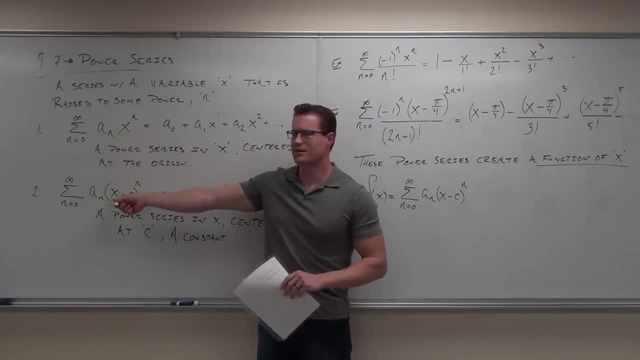 rather than this one. Do you understand that this form is like the general form of this? If I have c equals 0, then it gives me this one. So therefore I can always use this and be correct as far as my general power series. 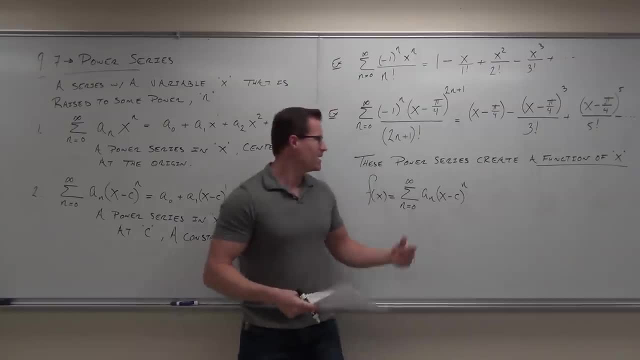 Quick head nod if you're okay with that one. Okay, So Does that make sense to you? If this thing is a function of x, we already said it was- because what happens is I'm going to get a sub. n is going to be a number, a constant number for every individual term. 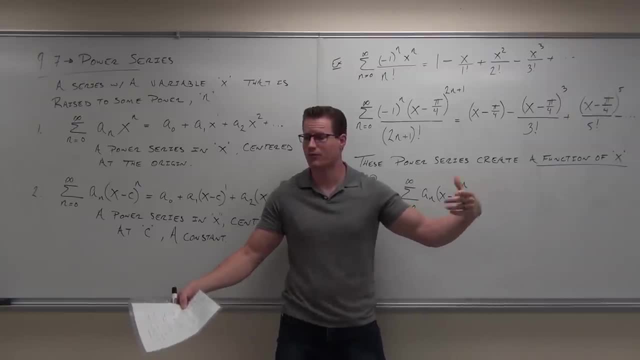 when I put 0 or 1 or 2 or 3 or 4 or 5 or whatever, into my n, That's going to be a constant. This, of course, is going to be a variable. That's going to be a constant. 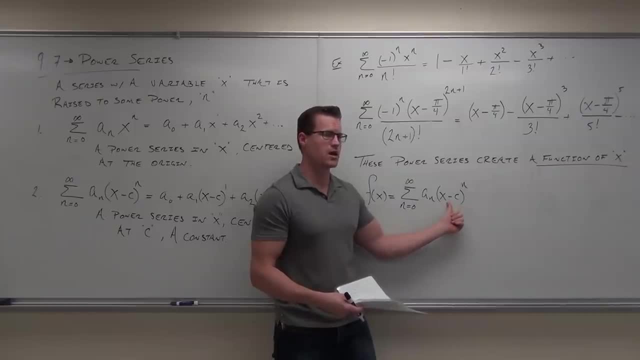 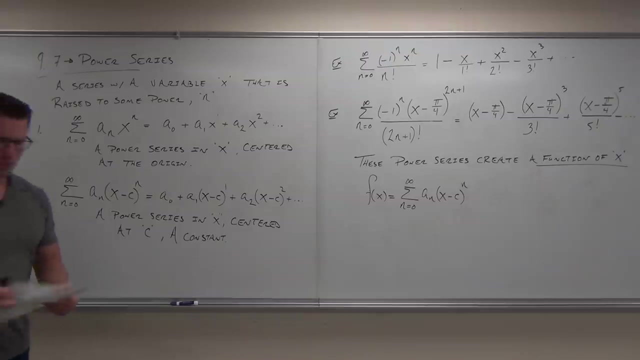 So I'm going to get a function in terms of whatever my variable here is. It's going to be a function in terms of x. Now this is what's going to be interesting. Please listen carefully. If I have a function equal to my series, when I plug in some x, when I plug in some. 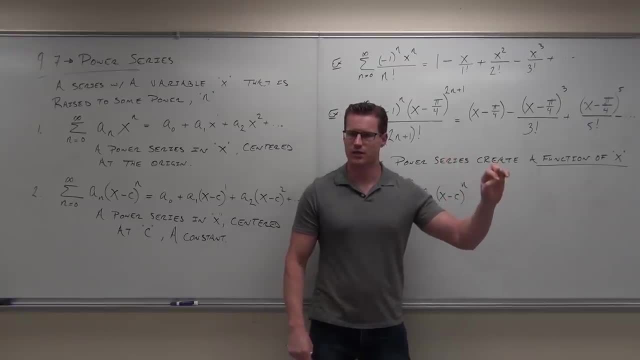 x. I'm going to get a series of terms correct. That series is either going to converge or it's not going to converge. Does that make sense to you? So I'm going to have this series. I'll have x's in it. 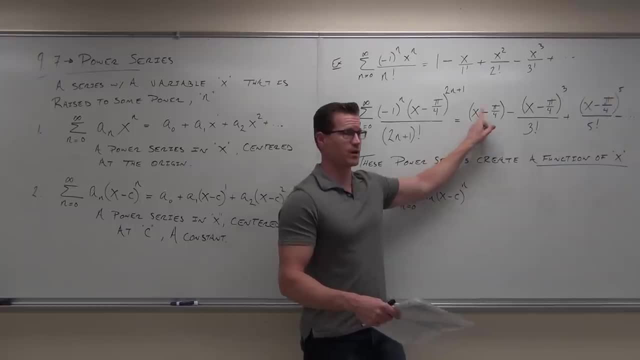 You say, hey, give me an x. Whatever you give me, I'm going to plug in my x. Either this series will converge or this series will not converge. Does that make sense? If the series converges, we would get a sum out of it. 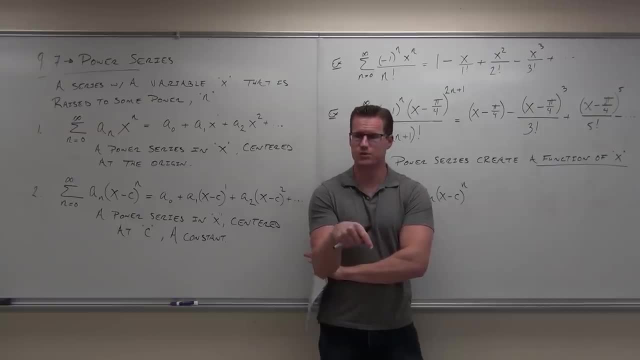 Does that make sense? If the series does not converge, of course, we wouldn't be able to find the sum. So if the series converges, we get a sum. That sum is the output of my function. The input of my function is, of course, my x. 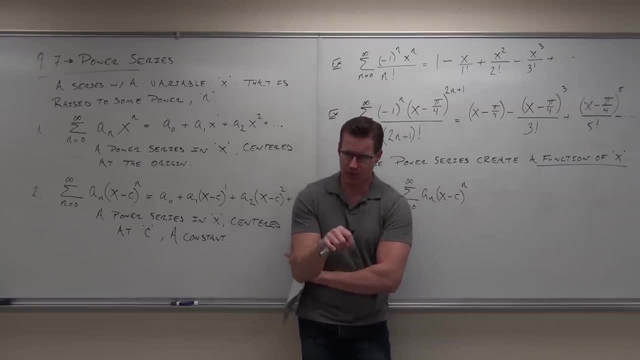 But I only will get a valid output if my input makes sense. The output makes my series convergent. Let me go through that one more time, because this is kind of a theoretical. Wait a minute. Does that make sense to me? Let me say it again. 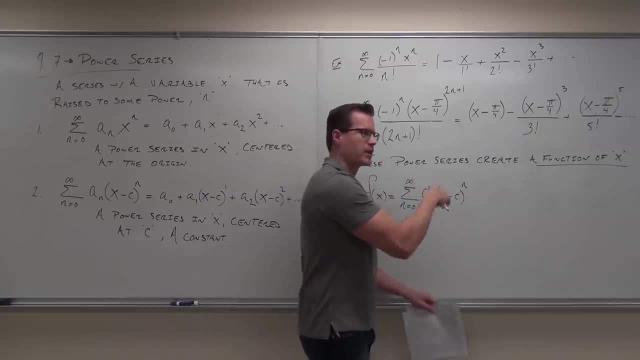 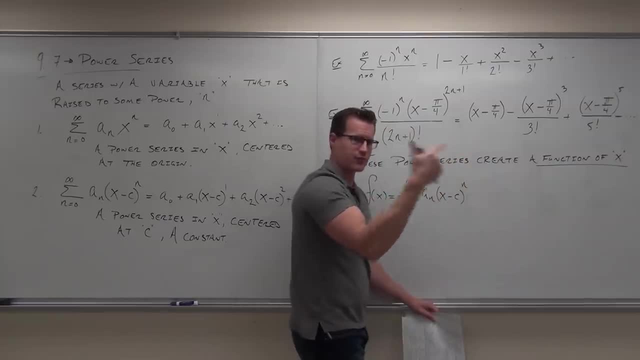 I'm going to get a series that either converges or diverges. Does that make sense to you? If it converges, I get a sum. That sum is the output of my function. If it does not- converge, diverges, then I don't have a valid sum. 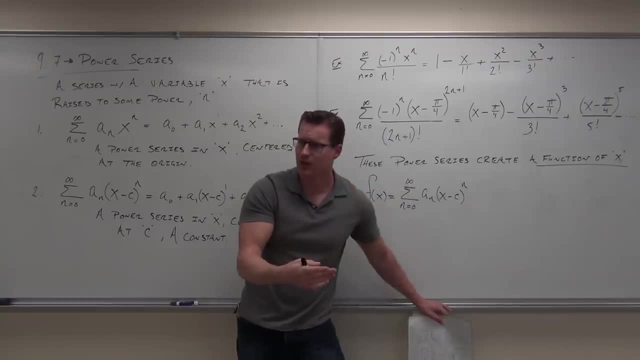 It would be like infinity or it would be undefined. We can't do that. So what we're saying here is: this function is defined with a domain- Remember that domain is all the things we plug in- With a domain of all x's, such that the series converges. 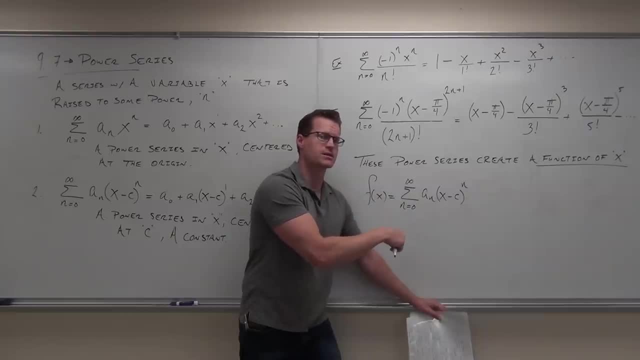 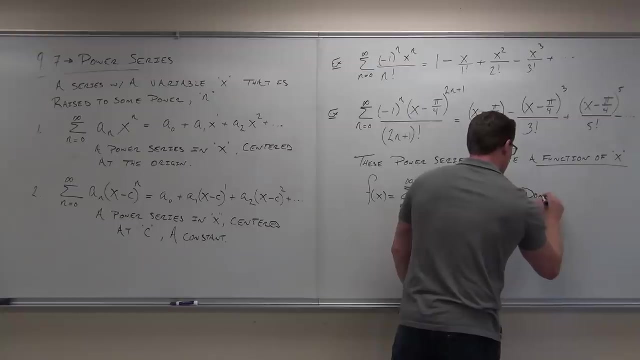 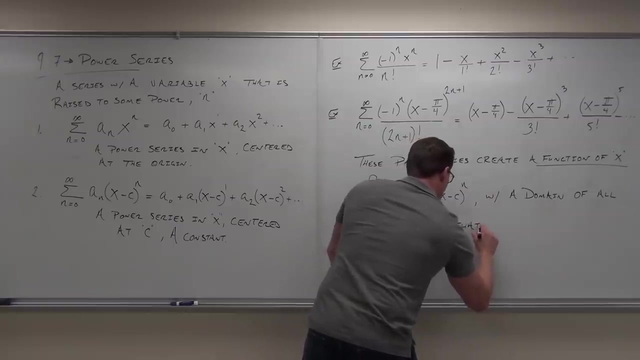 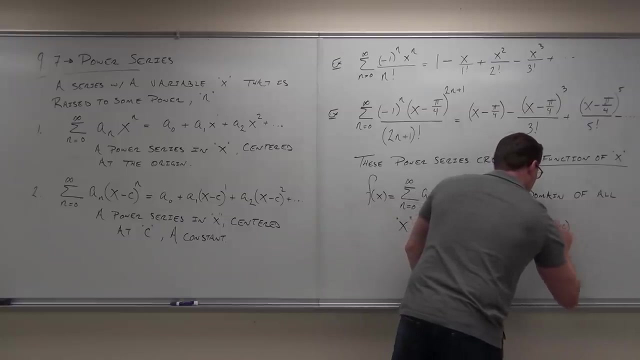 This is a function with a domain of all x's such that the series converges. If the series does not converge, then I don't have an output for my function. Does that make sense? Yes, Do you need me to explain that? 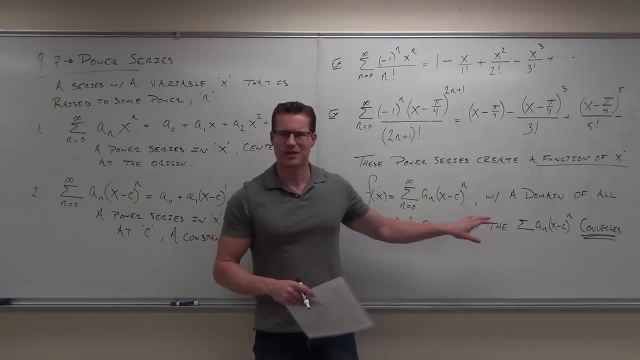 I tried to explain it three different ways, but they all ended up sounding kind of the same because it's the same idea. all three different ways, It's the same thing. Are there any questions on this idea? I know we haven't done any examples. 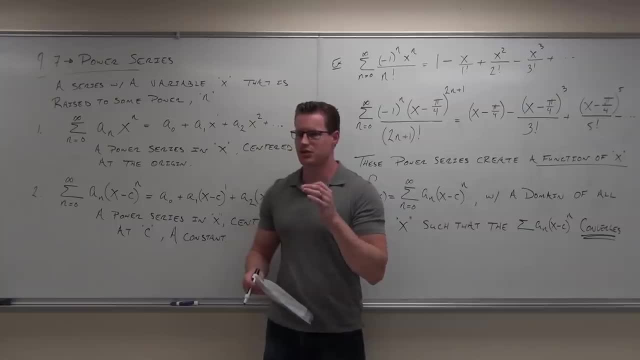 but I want to make sure this is clear before we go absolutely any further, to make sure that you get it. Do you get it that this thing can be defined as a function of x, because x is a variable? Do you understand that series either converge or diverge? 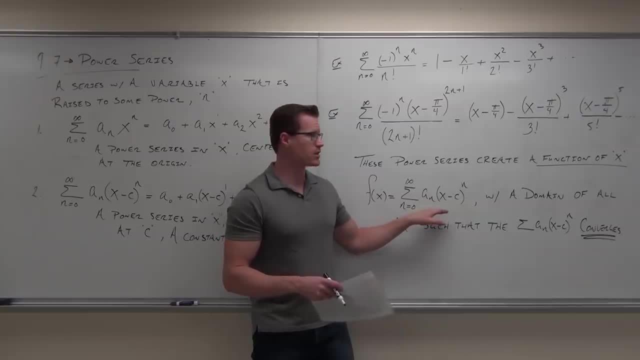 Okay, Do you understand that for certain values of x, this series will converge and for certain values of x, this series will diverge some of the times? So sometimes when plugging anything, it's going to converge. Sometimes when you plug anything, 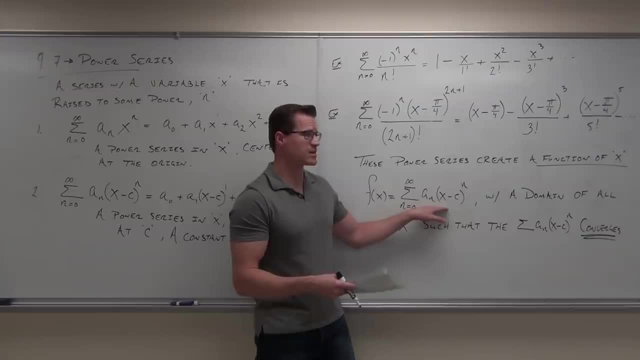 it's going to diverge, But a lot of the times we have some x's that's going to make the series converge and some x's that's going to make the series diverge. Do you get that? Do you understand that if the series diverges, 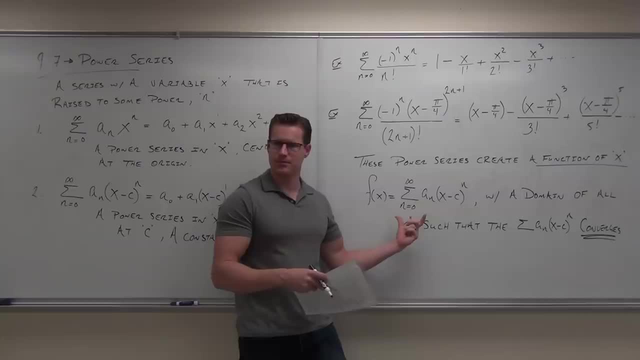 I can't really represent this very well with the function because I'm not going to have a sum. The sum is my output. I sound very sudden: My output, The sum is my output. Therefore, when you put in an x, it gives me a sum. 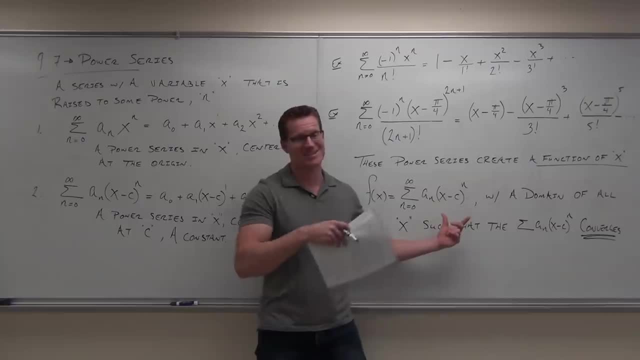 Not when y'all put in an x. When y'all put in an x, it gives me a sum, Not when y'all put in an x. I should say y'all put in an x. When I was 13,, my parents took me on a trip around the United States. and we spent a long time in the South and so I actually did pick up an accent from down there in Louisiana and Texas and all those places. So by the time I got to Boston I sounded all messed up, You know, at that age. 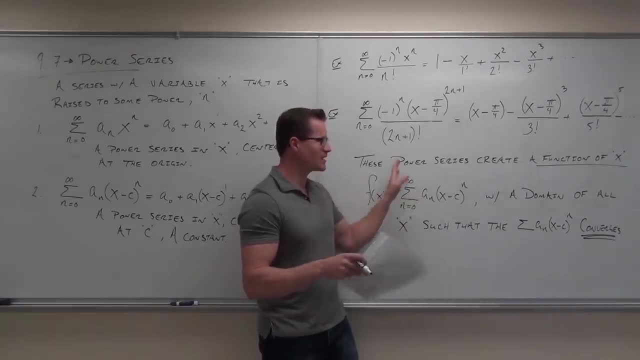 you're picking up a lot of language, So anyway, Anyhow. so if this thing is a function of x and I plug in certain numbers of x, some will make it convergent, some will make the series divergent, Those values of x. 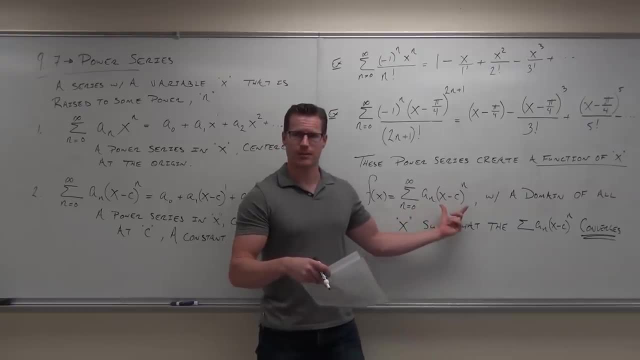 which make this series convergent mean that I get a sum for those values of x. If a series is convergent, I get a sum. So for the values of x which make this thing convergent, I get an output of my function. 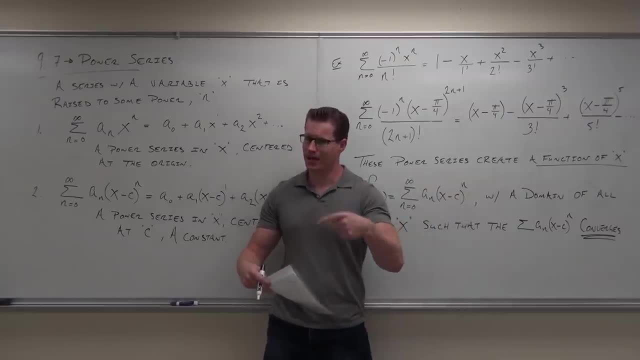 Therefore we have a function with a domain of all x's that make my series convergent. The x's that make the series divergent we don't care about because we can't define the function there. Show of hands, if that made sense. 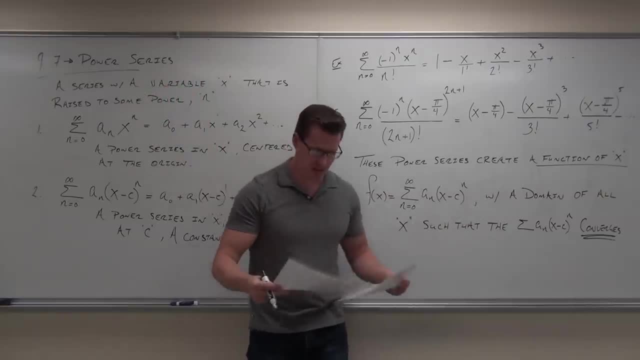 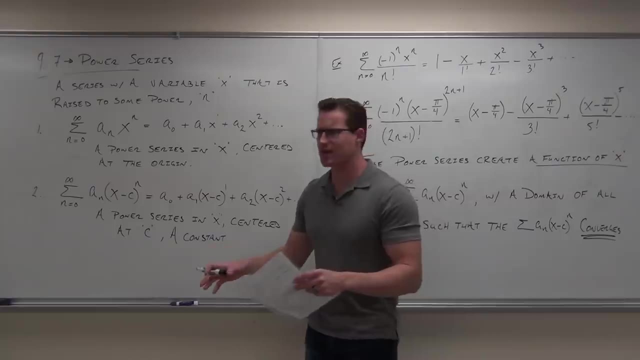 Okay, you understand a power series, then That is what a power series is. Now let me give you a couple examples on how we actually do this and what we can do with it- Not any hardcore examples, yet. We're still kind of on the note-taking part of this. 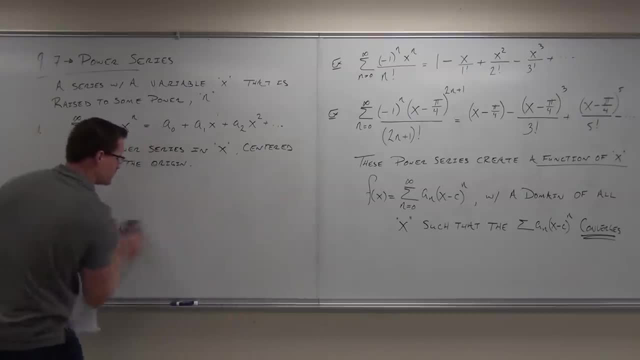 So we got the power series idea. The power series idea does make a function, so that our domain is all the x's that make the series converge. That's it. Now let's look at what we can do with it. Let's start with the most basic power series. 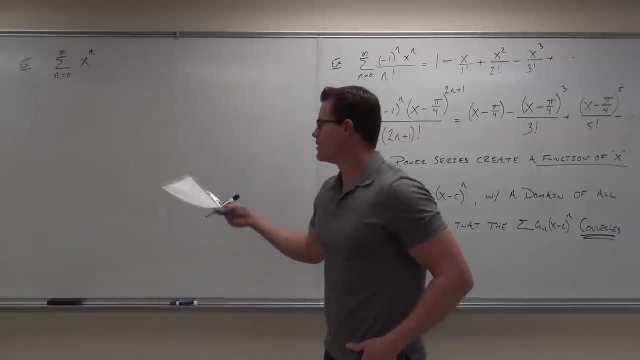 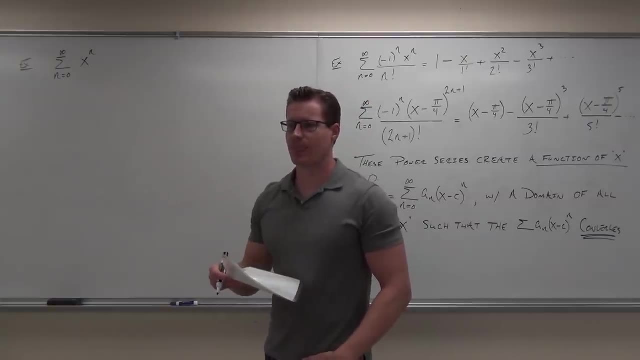 I can think of. It's just this: The series of n equals one to infinity. sorry, from zero to infinity, of x to the n. Firstly, is it a power series? Yes, Okay, what's my? a sub n One? 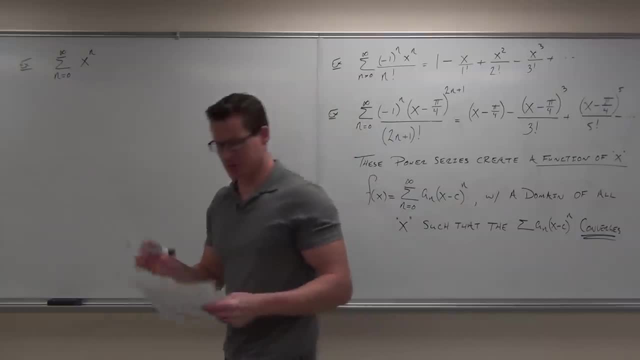 Yeah, that's a very simple power series, but it's still a power series. Let's look at some of you guys are zoning out. Don't zone out on me here. Let's look at the first few terms just to get an idea about what this is. 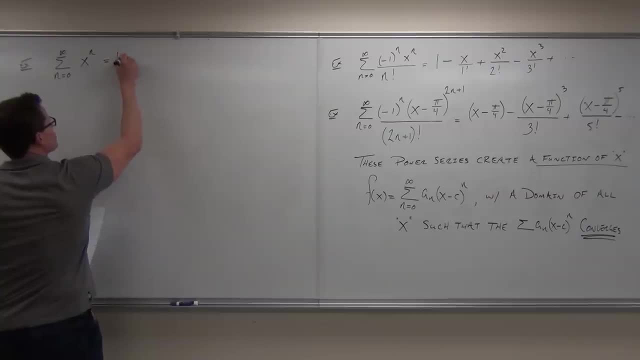 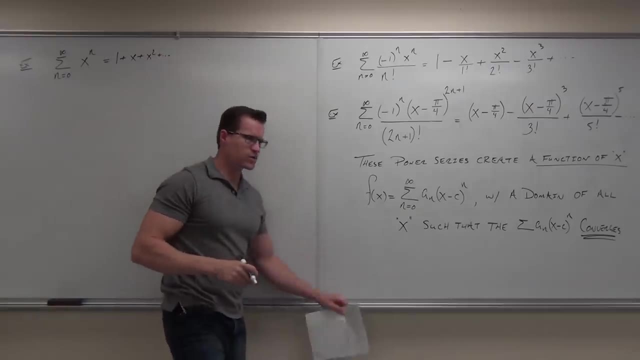 What's the first term here? One Next term, Next, Next term, Next term- Good, And then it continues, continues, continues. forever and ever and ever. Here's what's kind of interesting: These power series are going to represent series. 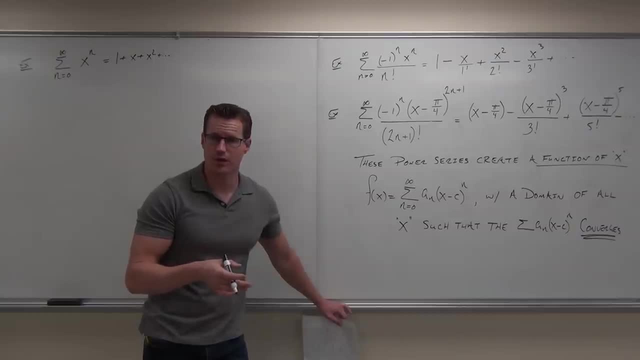 a lot of the times that you've seen before or that you can work with in the same manner you work with the other series. For instance, this right here might look weird to you. This is a geometric series. That's all it is. 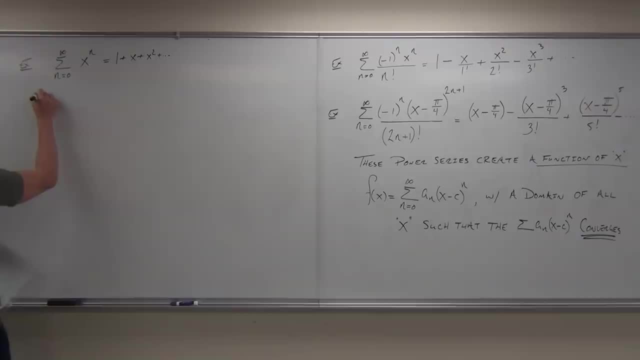 It's just a geometric series, and I'll show you why. This is simply a geometric series. Do you see it yet? No, No, Let me put this on the board. Do you understand that a geometric series is a times r to the n? 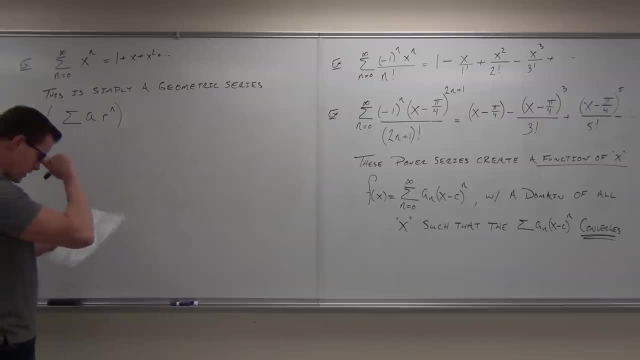 Yes, That's a geometric series. Yes, Well, if that's a geometric series, by the way, sorry, when does this thing? do you remember when it converges? It's all based on the r When r is less than 1.. 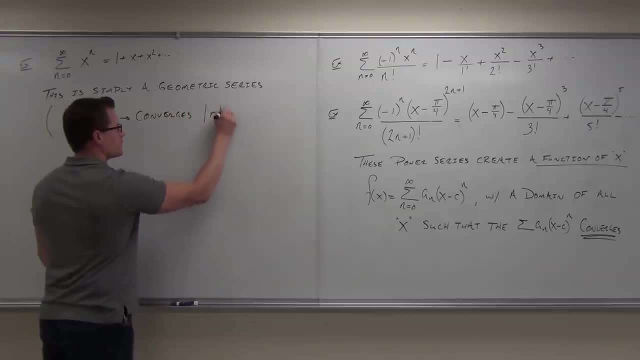 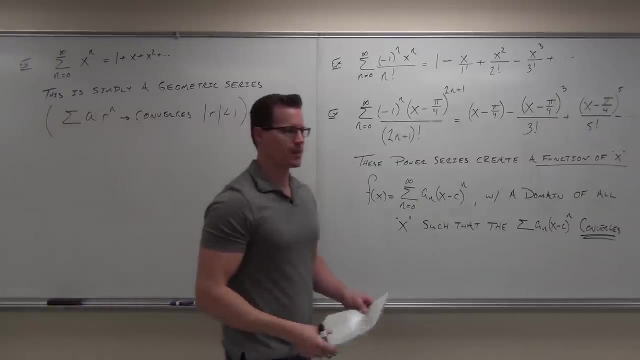 Absolute power. I see the value of r. Do you know what it's created? No, Yes, Plus or minus 1.. Plus or minus 1? Greater or equal to P series. greater than 1.. Make sure that's on your note card. 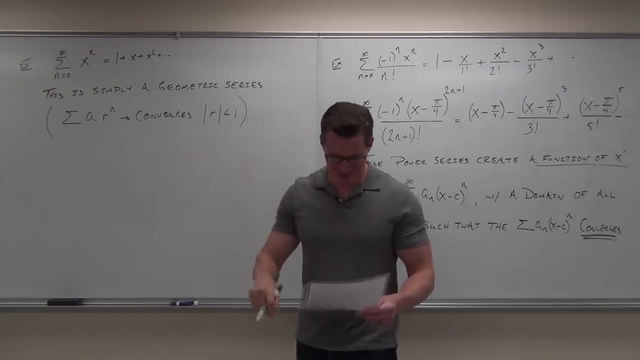 Note card. Note card. it right now, By the way, that r- I don't know if I ever told you this- that r is called the common ratio. Did I ever tell you that? No, It's called the common ratio. 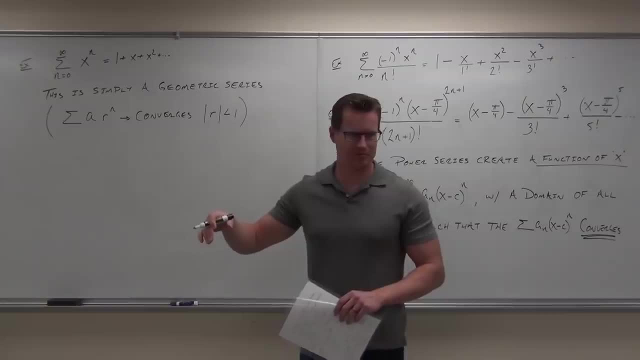 Like 20 sections later. Whatever, A geometric series converges when the common ratio r is an absolute number. Now I'd like to make this clear: The geometric series converges when the common ratio r is an absolute number. So in the geometric series, 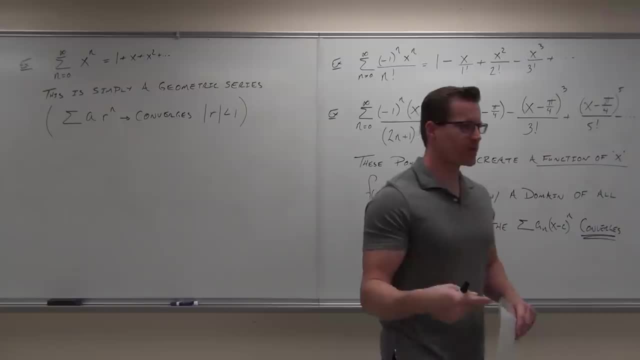 I don't know if I ever told you this, but a geometric series converges when the common ratio r is an absolute number in terms of absolute value, is less than 1.. That's what this thing is. Now I want you to consider this for a second. 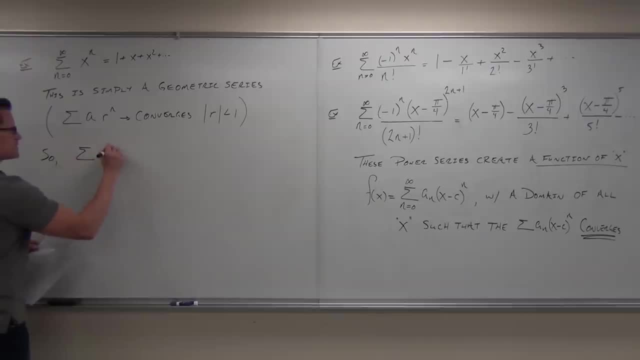 So the series x to the n has a common ratio of x. Look up here. Does this fit this format? What's our a? No, the a is 1.. a would equal 1.. What's taking the place of our r? 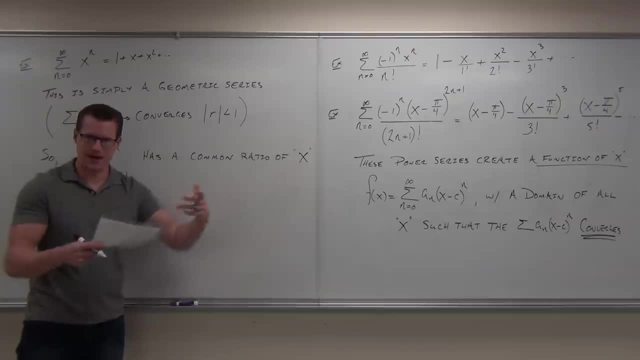 The x. That's what's set as a common ratio of x. That is the r in this case. So what's really interesting is that this thing is really a geometric series. Now the question is: when do geometric series converge? 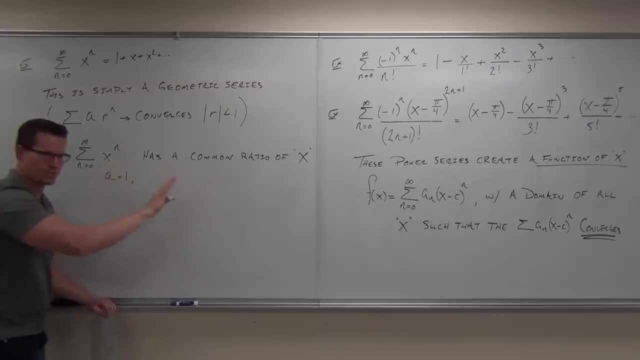 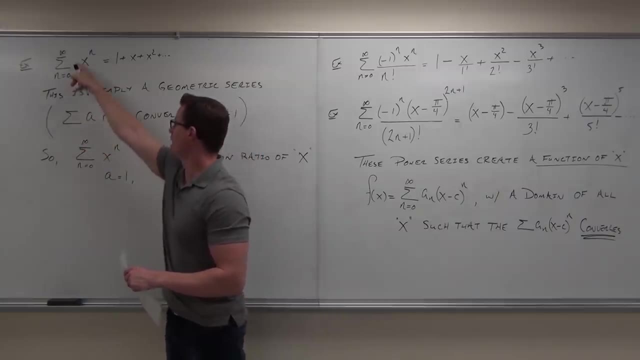 When the r is less than 1.. Okay, so I don't want to lose you here. Do you understand the idea that I'm trying to make this look like a geometric series? It is a geometric series, It's just that a is 1,. 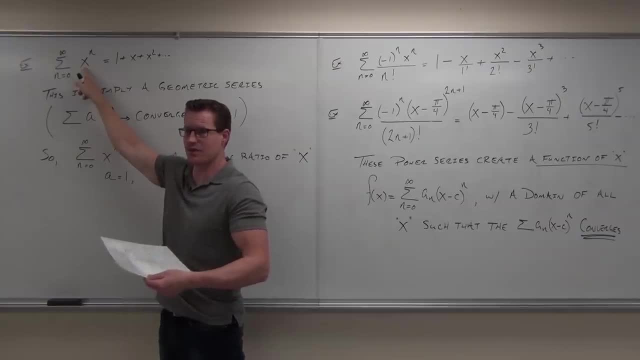 the r is x in this case. That's geometric. Now, if geometric series converge when the absolute value of r is less than 1, then this series which converges when the absolute value of x is 0. Less than 1.. 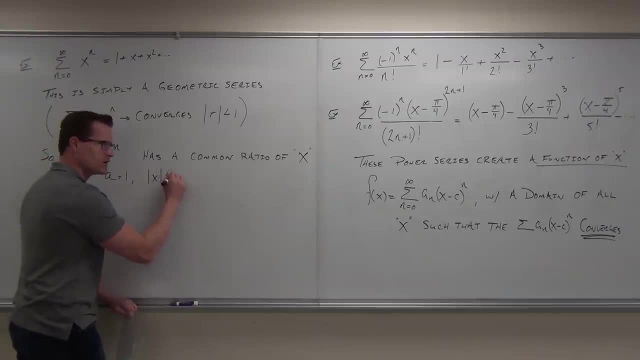 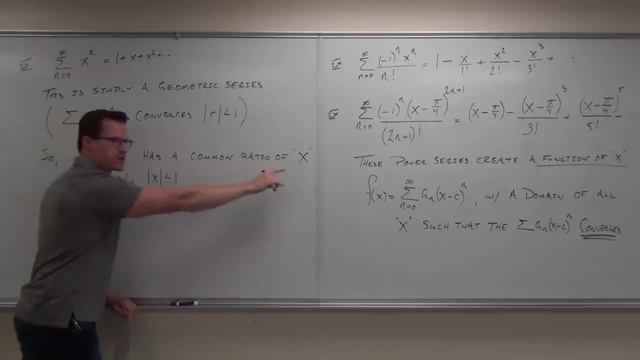 it says it converges if the common ratio is less than 1.. This has a common ratio of x. It will converge if x is less than 1 in terms of absolute value, Or if you want to think about it this way. 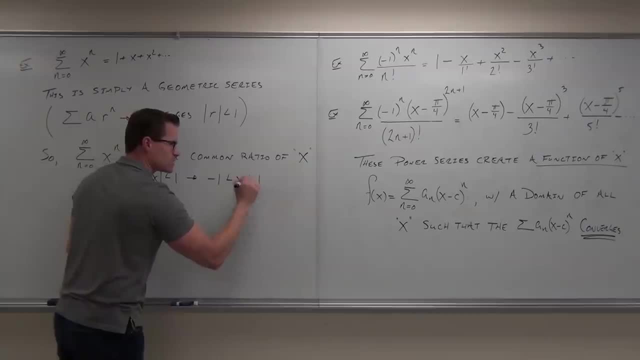 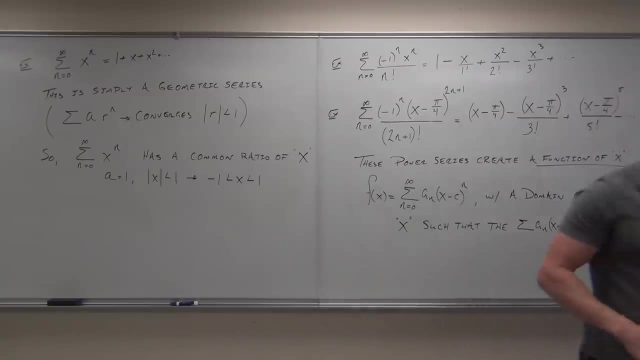 when negative 1 is less than x, which is less than 1.. So what's this diversion? It's convergent. Let's talk about it one more time, just to make sure that you are with me on this thing. First things first. 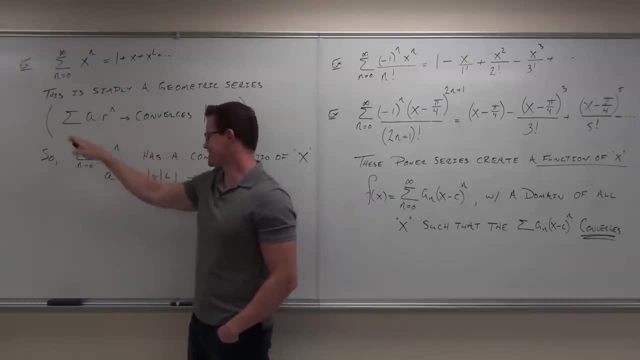 are you starting to see that this is geometric? It is. It is this: It just happens that r is no longer a constant. It happens to be a variable. Now, what we know about geometric series is that geometric series converge every time this number is between negative 1 and 1.. 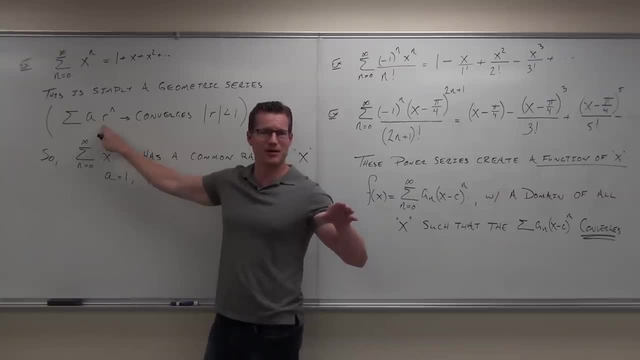 Therefore, I don't give a heck what It's a thing now. I don't give a crap what this is, as long as this number is between negative 1 and 1 non-inclusive. Does that make sense to you? That's what this says. 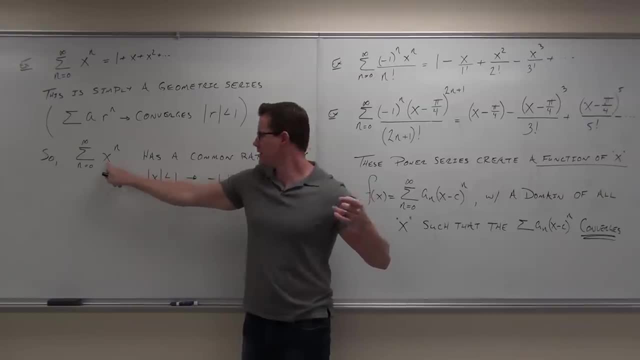 I don't care what this number is. as long as it's between negative 1 and 1 non-inclusive, This will converge. If I give you negative 1 half, is that going to converge? How about negative 1 third? Negative 1 fourth. 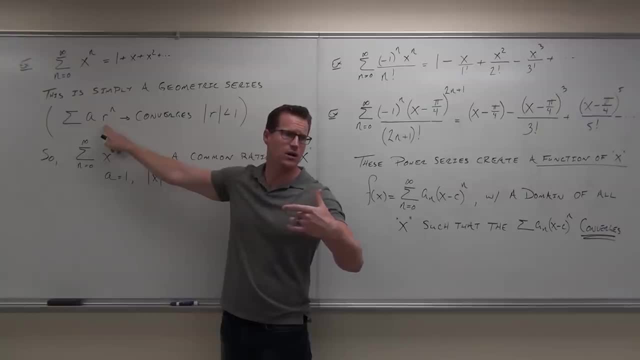 Negative 1 fifth. Negative 1 sixth. How about we get to 0?? How about 0?? How about 1 half? How about 1 third? How about 1 fourth? Yeah, it's going to converge for everything, as long as this is between: 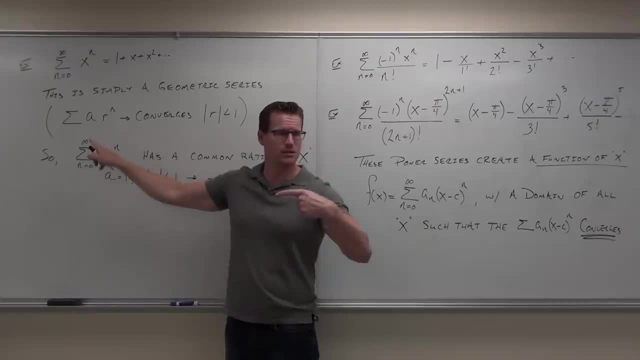 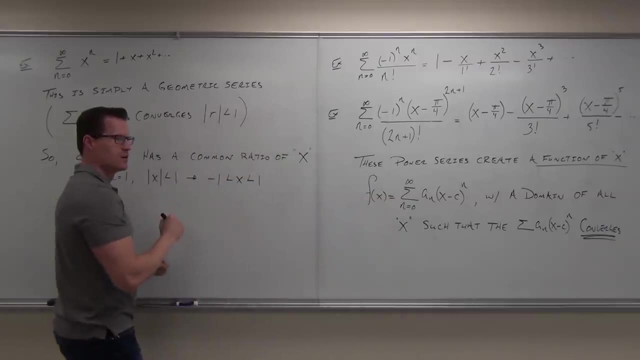 as long as this is between, because this is that It is a geometric series. Does that make sense to you? Yes, Are you sure? So our domain is right here. Remember that. the whole thing, Hey, this thing that defines. 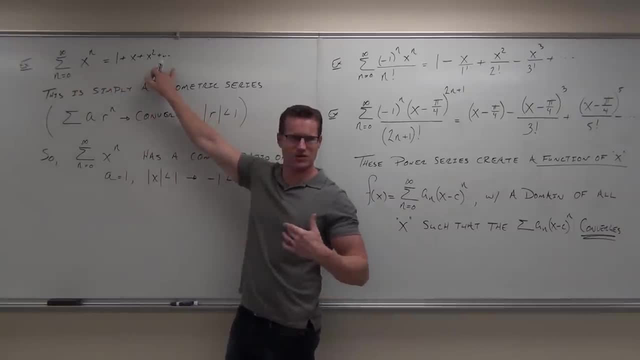 a function of x, doesn't it? Are you catching this? Are you catching this picture? This defines a function of x. When will this function of x converge? It will converge when x is between negative 1 and 1.. That's what we're saying here. 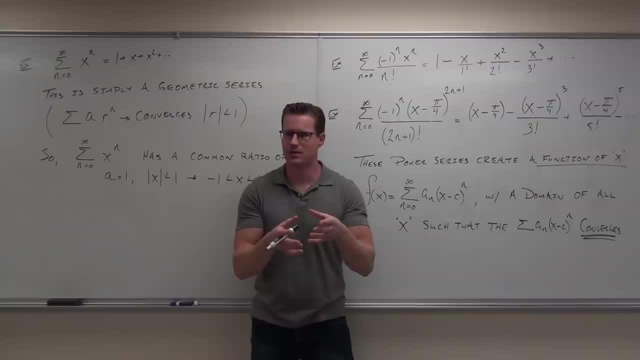 This is a function on a very specific domain. Is it a function defined everywhere, folks, Everywhere? No, It's defined for a very specific set of x's. What's the set of x's that this is defined to be Negative 1 and 1.. 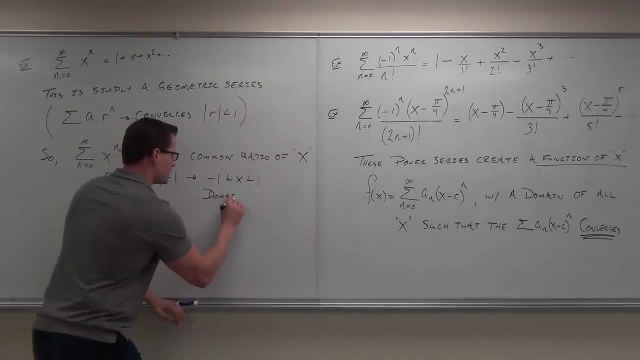 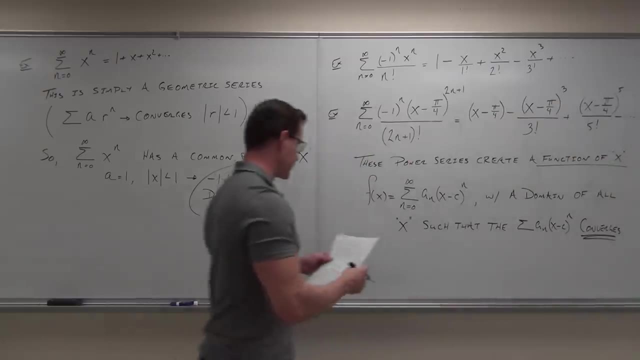 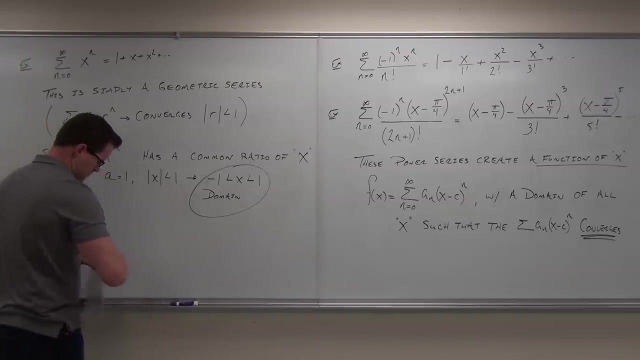 That's our domain. That's it. Now. here's what's also very cool. Do you know how to find the sum, Yes, Of geometric series a over 1 minus r? So in our case here, the sum is a over 1 minus r. 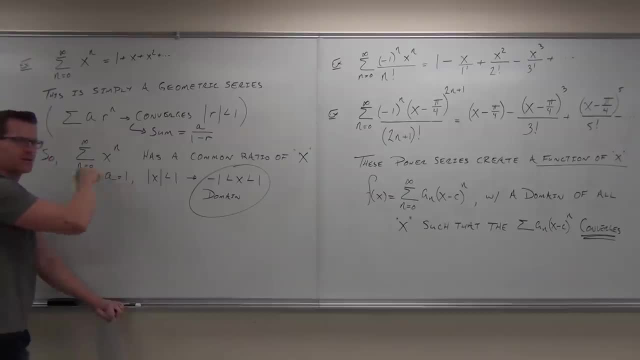 a over 1 minus r. Check this out. So if f of x, This is kind of how we'd write it mathematically. I said a lot of words here. You didn't say very much, Forget you guys, But I said a lot of words, all right. 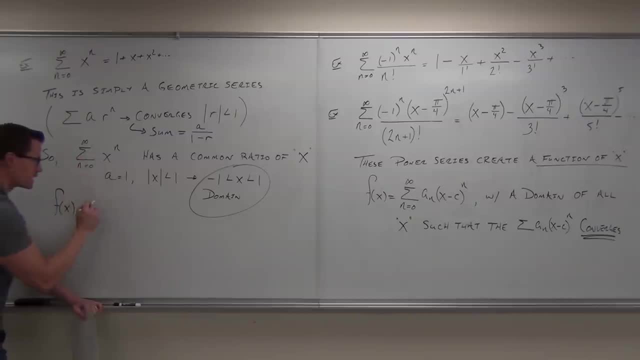 Here's what this says. This says: I have a function. This is a function of x. This function of x is geometric. If it's geometric, it will have a sum. The sum is defined to be a. How much is our a? 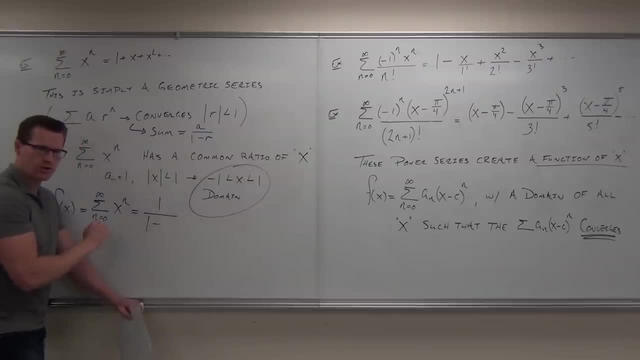 1. Over 1 minus r. What is our r, x? Aha, The common ratio is r or, in this case, x. Put it all together, folks. Do you understand that's a function of x? Do you understand that's geometric. 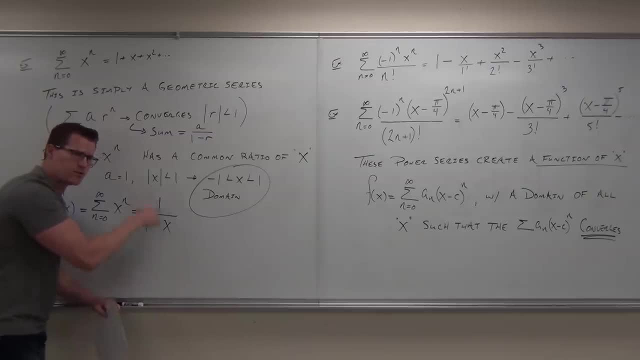 It will have a sum. Do you understand that the sum is only valid when this thing converges? Do you get that? Yes, When does this thing converge Between negative 1 and 1.. Yeah, This is awesome. This is really cool. 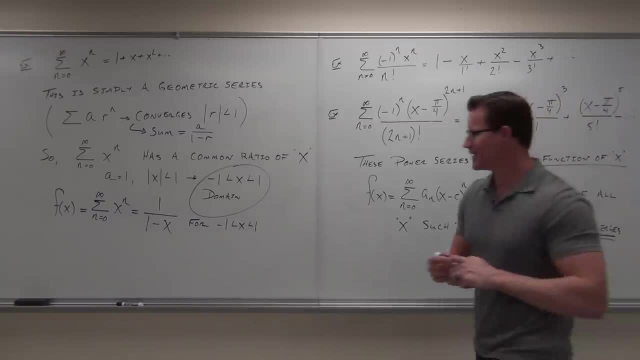 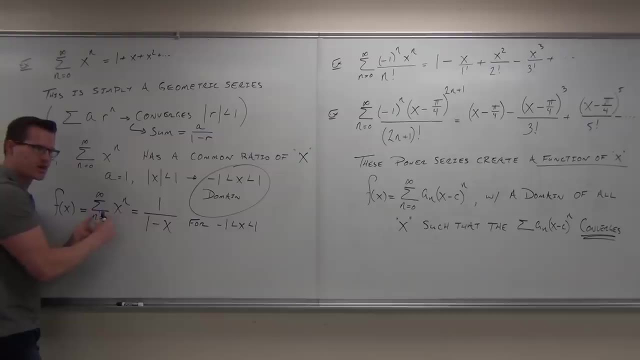 Because here's what this says: This is equal right. And this is equal right Because a series is a sum, and this is the sum of any geometric series when x is between negative 1 and 1, because that's when this series converges. 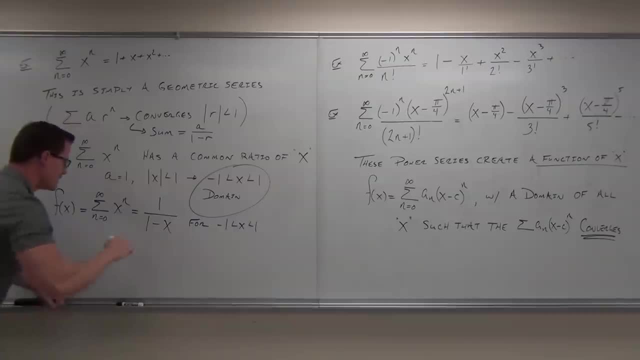 Therefore, when we can find the sum. What that means is that this series actually represents the function f of x equals 1 over 1 minus x. That's what it represents. So you can talk about the 1 over 1, but only on a certain interval. 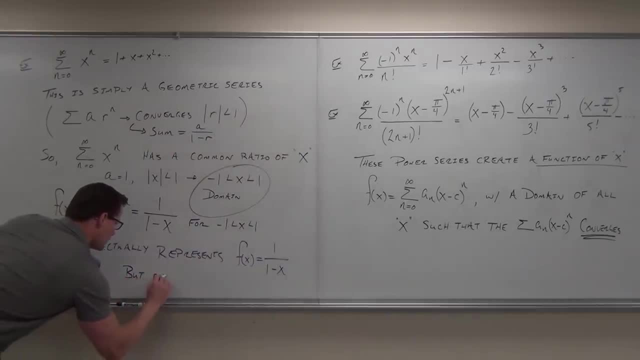 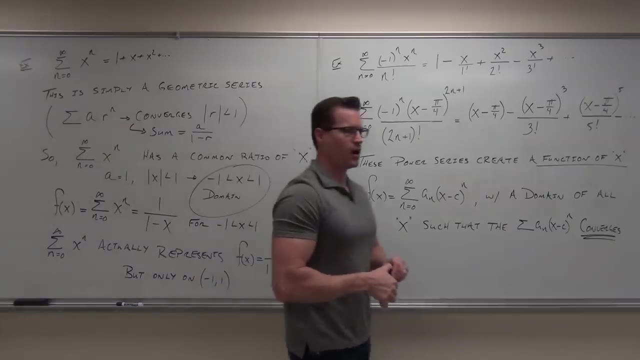 Only between what two numbers? Negative 1 and 1.. You got it. I'm using interval notation here: Negative 1 to 1. The interval is negative 1 to 1.. So, if you want to, What in the world are you freaking? 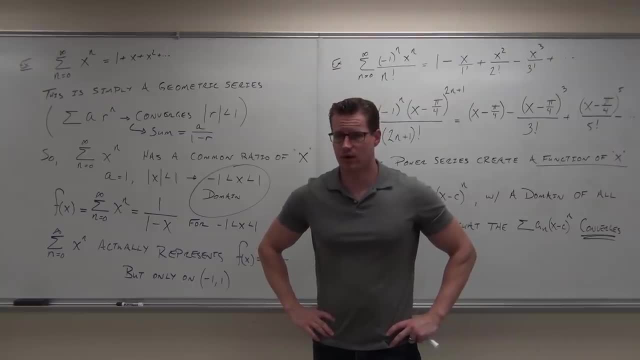 talking about Leonard. Here's the deal. Give me a number between negative 1 and 1.. 1 and 1 and 1 or half 1 and 1 and 1 and half 1 and 1 and 1.. 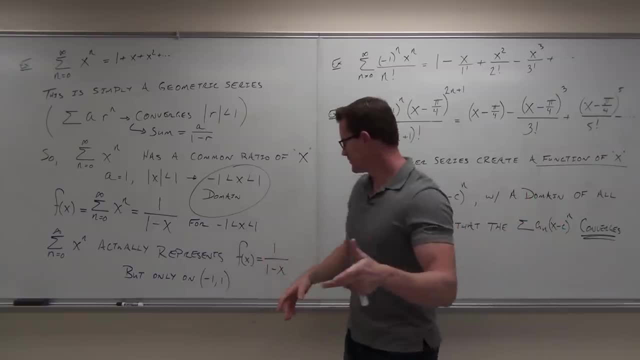 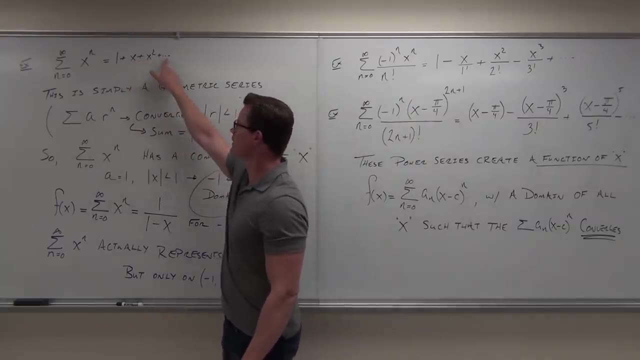 1 and 1 and half. 1 and 1 and half. You can plug a half in here, right, and find out what it is. If you wanted to, you could plug one half in here and here, and here and here, forever. 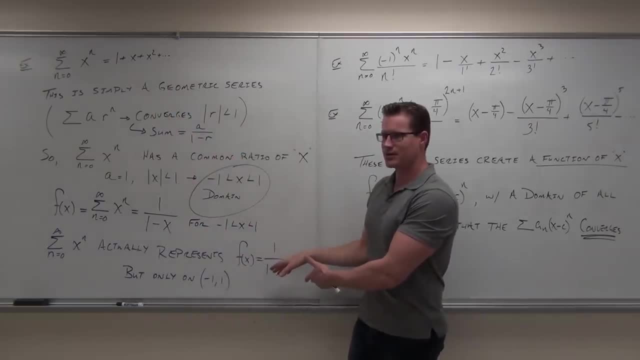 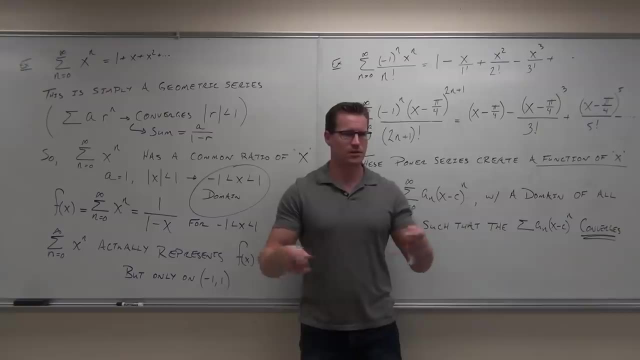 and add it all up, it's gonna equal exactly what you can get out right here. It's kinda weird, right? So we're using these series to represent functions, or rather, we're using functions to represent series. Same idea, Show of hands, if you understand the idea. 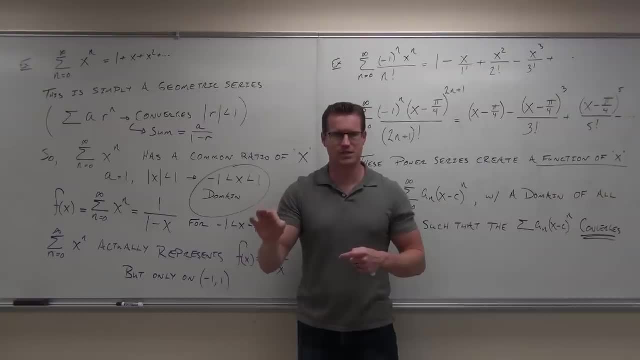 Power series represent functions. That's what they do because they have x's in them, functions of x. They represent these functions only on certain intervals, for which the series converge. If you get that idea, you do understand power series. Do you understand power series? 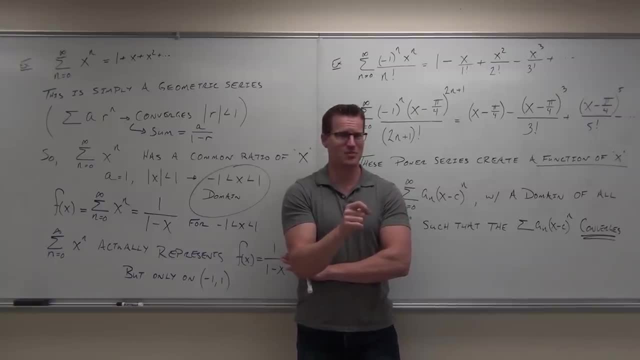 No, my speech is all off Power series. I thought you said parachute, Parachute. Do you understand? parachutes Jump out of planes. if they open, you live. It's not worse. Usually Okay show of hands if you honestly do feel okay. 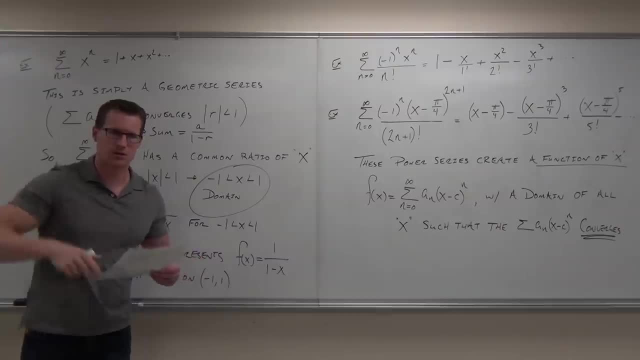 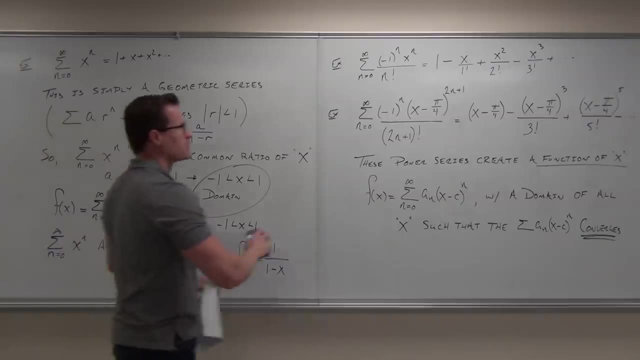 with that. Are there any other questions whatsoever on that? So our x is our input, our sum is our output. That's how it works. Couple other little notes for you before we get on to it. I do wanna kinda go quickly through this. 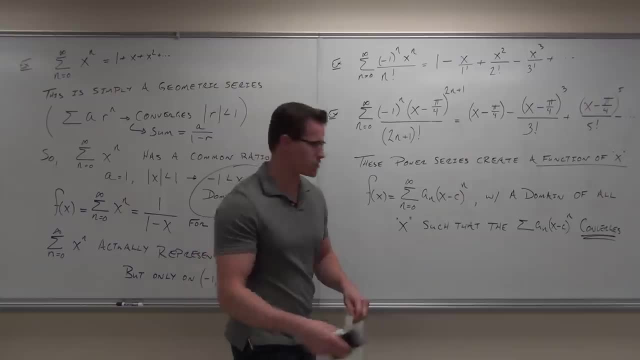 because I wanna do an example to give you the idea of what you're gonna be doing here. Question: That's just a proof, right? I want you to show this. My or I was thinking: did we find out if that thing? 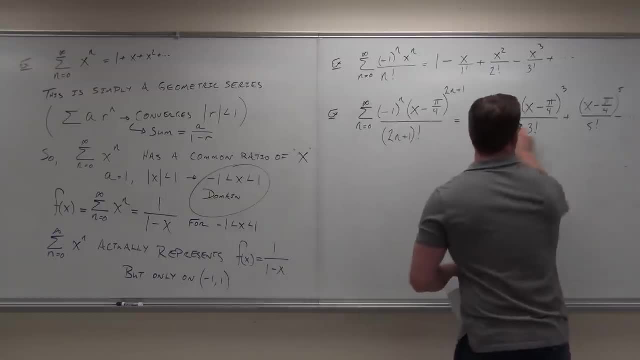 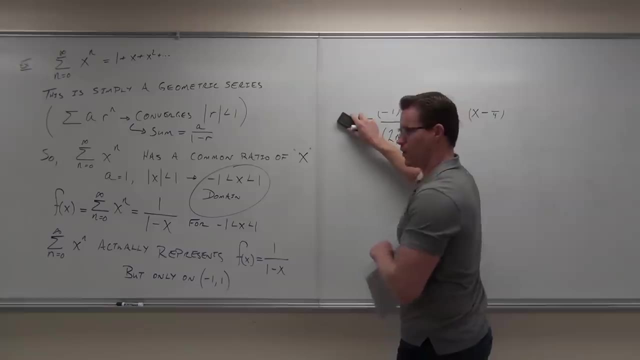 actually converges or diverges or not. Well, that's the whole point. is that your x is a variable, correct? Yeah, So I can't tell you, this converges all the time, Unless it converges for all x's. 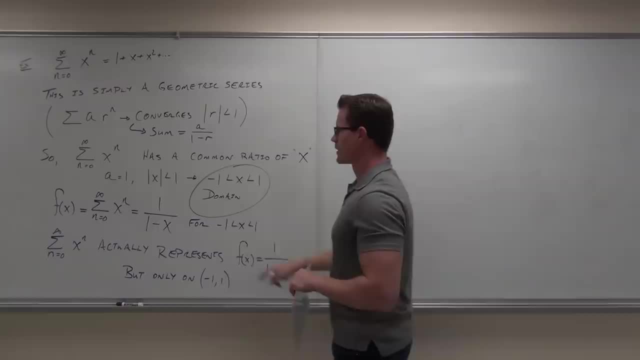 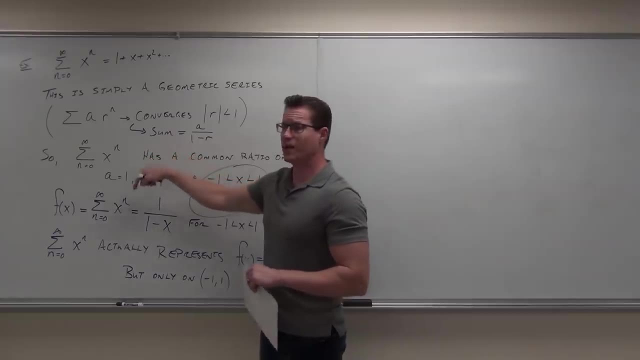 What you're doing is you're saying: okay, if this is this and this is a geometric series, then I know when it will converge. What you're basically doing is giving me the interval for which this will converge. That's what you're doing. 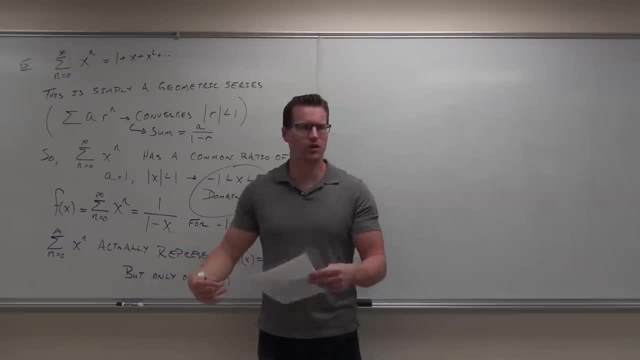 Not the other way around. You're telling me that it will converge or won't converge. It will at some point Give me the interval that it does converge at. Does that make sense? Then, the interval that it does converge at is the domain of your function. 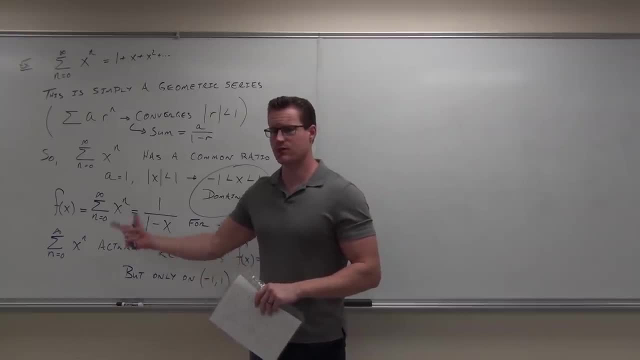 Otherwise there would be no sum. You could not define your function that way. So you guys get the idea. You're saying: will this converge? Let's find out, If it does, what's the interval that it will converge at? 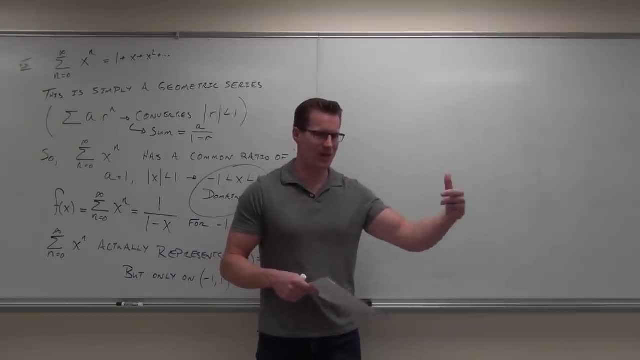 What x's can I plug in? That's my domain, Because you're defining your domain to be the values where your series converges. Therefore, you get an output for your function. If you don't get an output for your function, how do you do it? 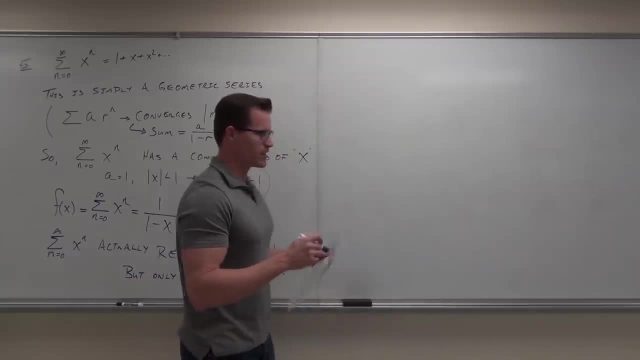 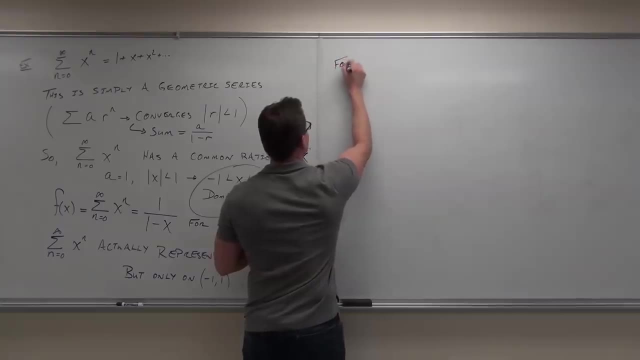 How do you define a function? Well, I talked a lot. Did that make sense to you? Yes, I think I said the same thing earlier, But I want to make sure you really got it. Now let's talk about for general power series. 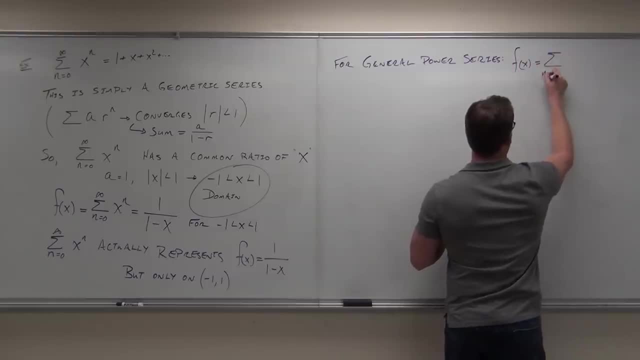 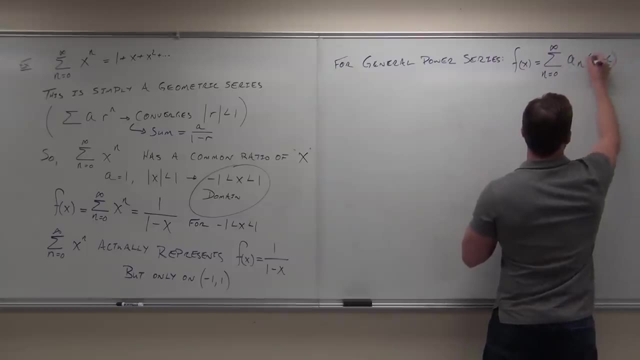 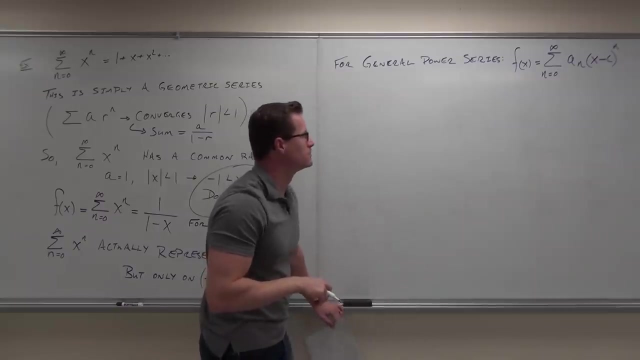 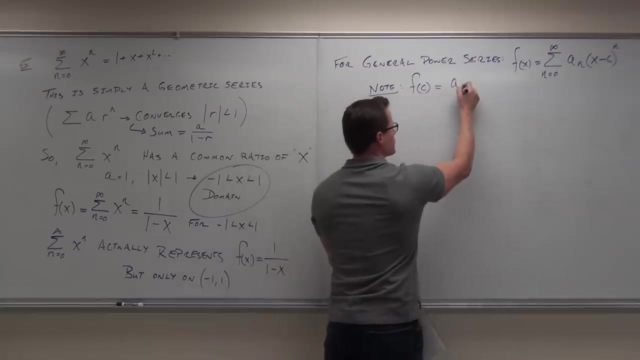 So when we have a function equal to a general power series, where it doesn't necessarily center at zero, By the way, if you, Where is this thing centered, C? Do you understand that if I plug in C, All I get is A sub zero? 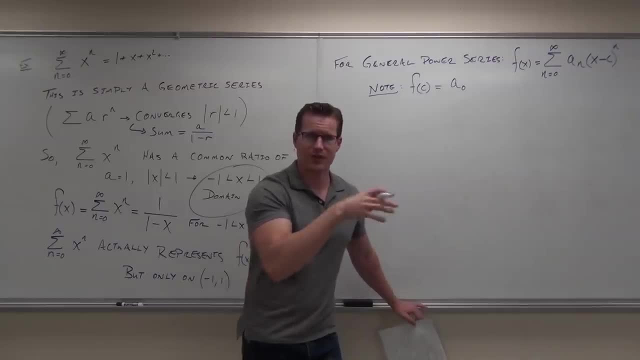 Does that make sense to you? If I plug in C, everything else besides the first term is gone, Because you have X minus C. If X is C, then X minus C would be zero, zero, zero, zero, zero, zero zero. 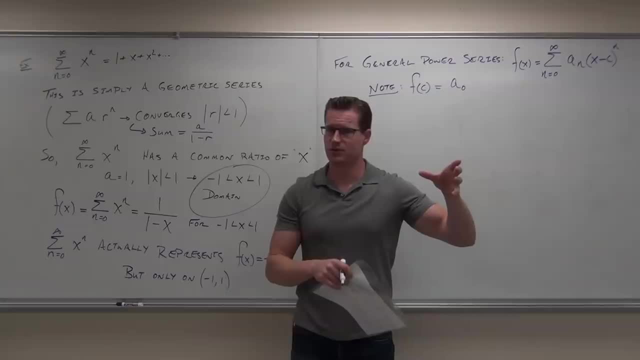 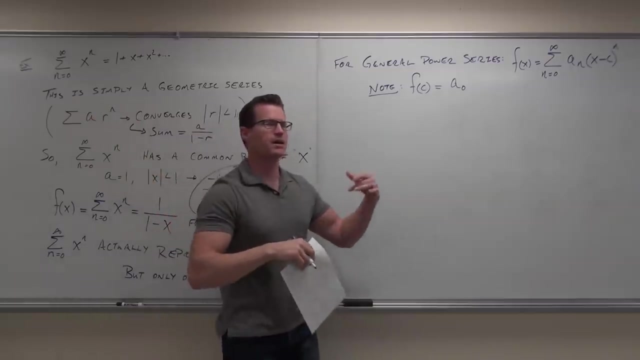 All I'd have is A sub zero. first, That's defined as your center. So the reason why we say it's centered at the origin- Please listen carefully- Is, if I plug in Like to, Let's see. Well, if I plug in my center itself, what I end up getting is something right around the origin. 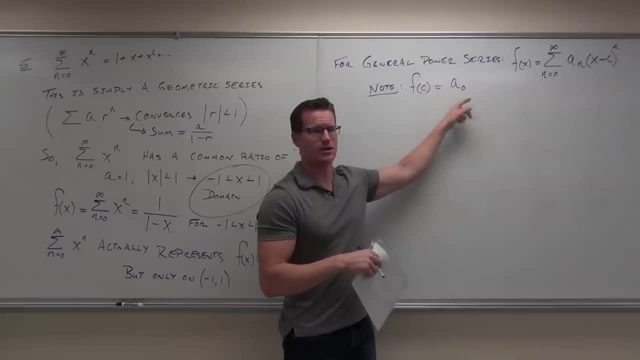 All right, If I plug in the center here, I'm going to get A sub zero. It's going to be centered at C comma A sub zero. That's going to be the first point of my function. Now, what else do I want to say? 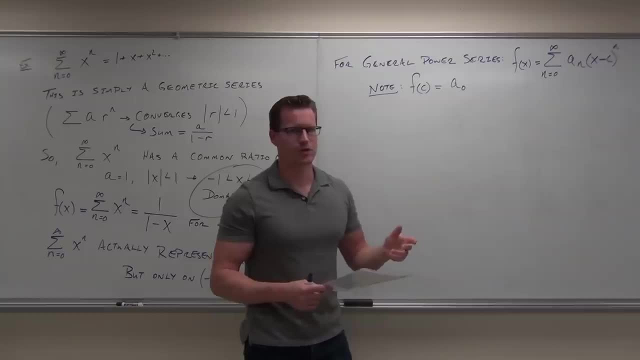 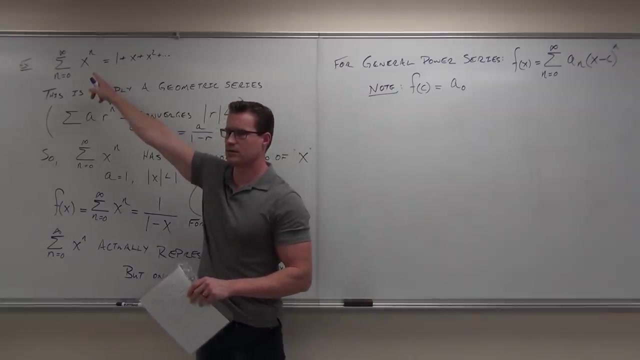 Oh yeah, The domain. This is kind of important for you too. The domain of your power series is always going to be some interval that is centered around C. Notice something? What's the center here? Zero, The center. It's got to be a constant. 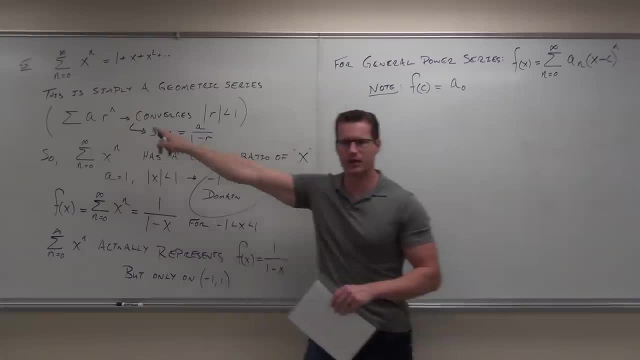 The origin, The center is zero. The origin is zero. Look at your domain. What's right in the middle of your domain? Zero, It's centered at zero. That's where we get the word center from. That's what center means, okay. 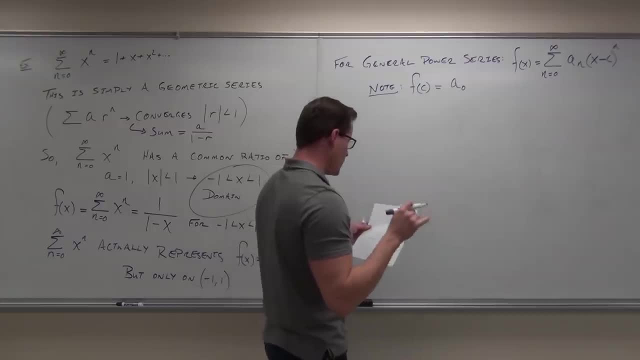 It's right at the center of your interval. So note for you the domain of f, of X, the domain of your function. your power series will always be an interval with X equals C at the center of it. All right, All right. 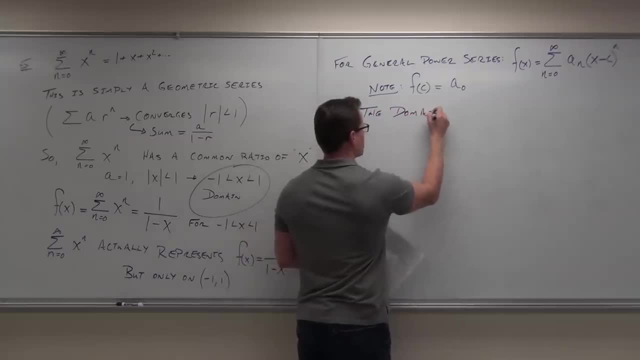 Let's go again. Just a moment, Let's look at that. Just a moment, Let's look at that. Okay, So what's the function of the domain of f of X? Zero, Zero. The domain of f of X is always going to be a constant. 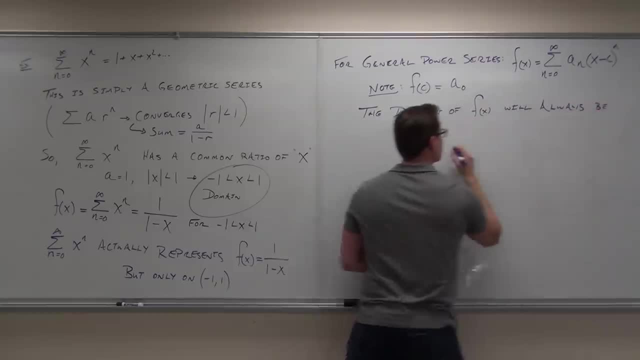 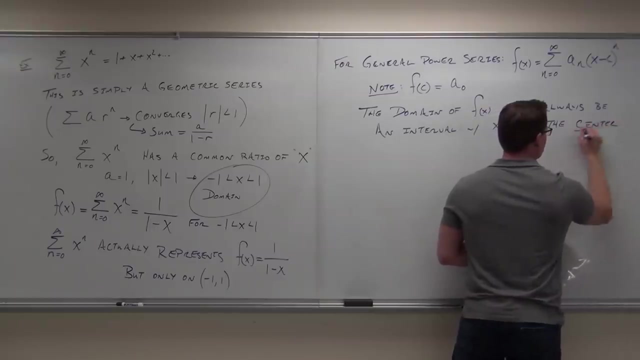 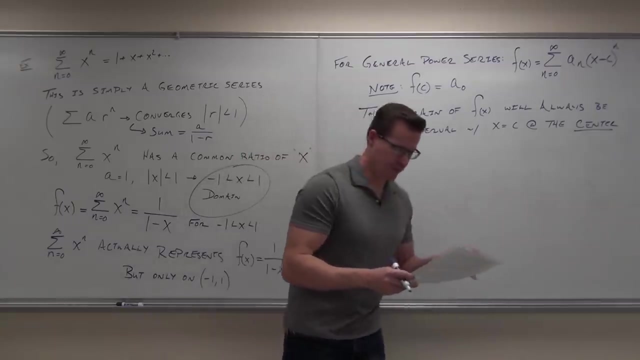 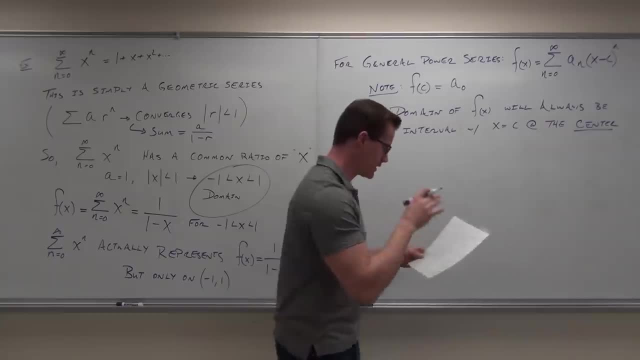 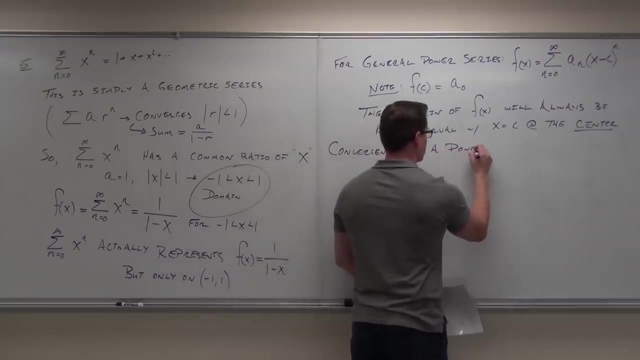 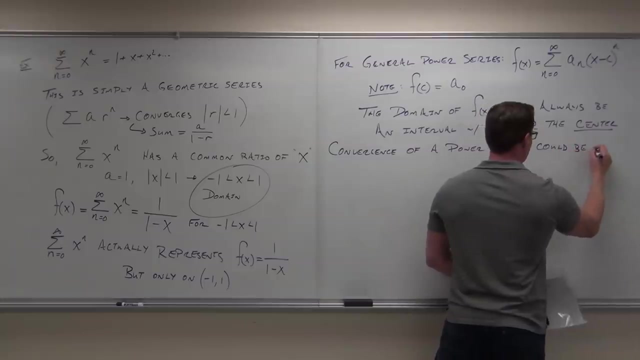 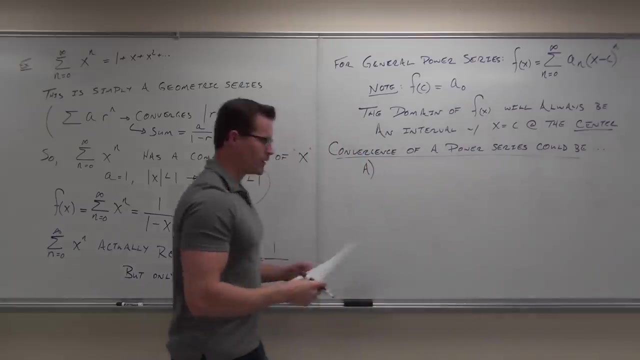 I really hope we get to our example today. I'm not sure if we will, but at least we'll get through this. So convergence of a power series could be one of three things. First thing: you might have a power series where the function is only defined at the center. 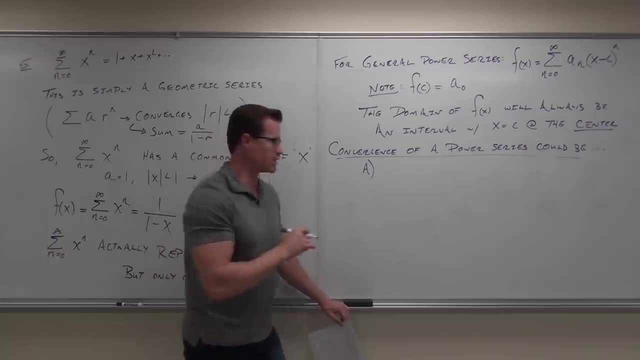 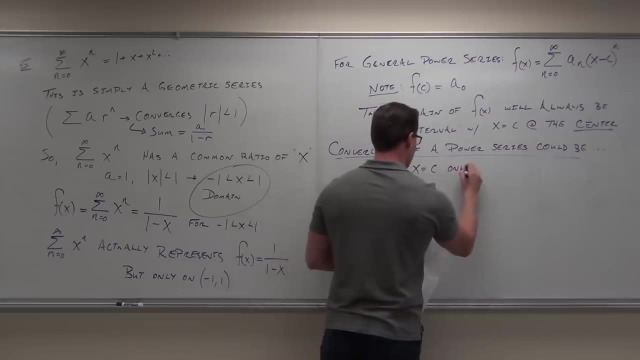 It could be defined just at x equals c. If it's defined at x equals c, only we would say that the radius of convergence is zero. A radius has this idea of you going around something, doesn't it? The radius of convergence is zero. 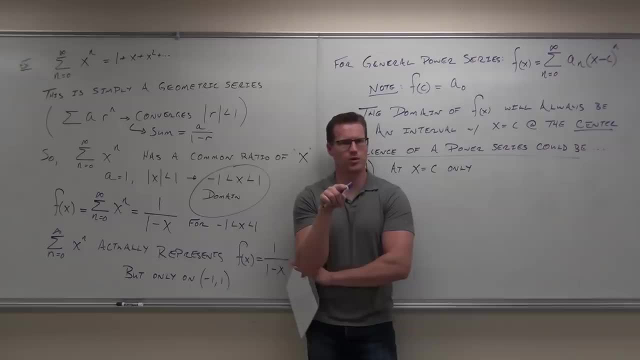 It's only at one point. Let me make sure you understand this here real quick. Look at the board. This has a center of zero. It converges at zero. It has a radius of convergence of One because it goes to negative one and one. 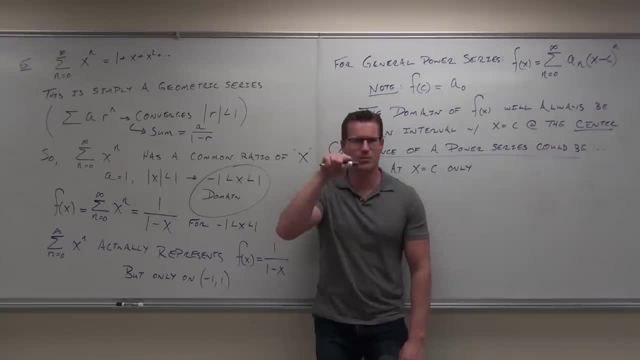 That's where it's centered. It has a circle. It kind of- yeah, sort of It's not going really up or down, but it's centered at zero. It has a radius of one. So we go negative one and one. 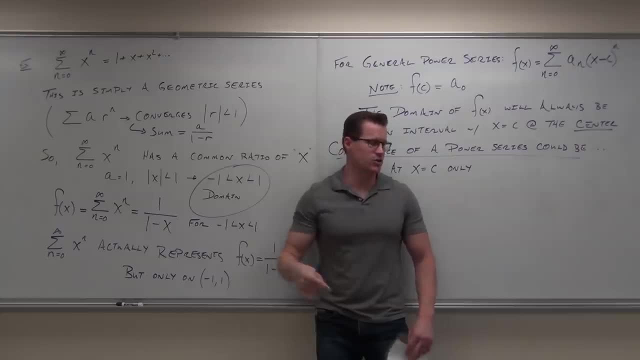 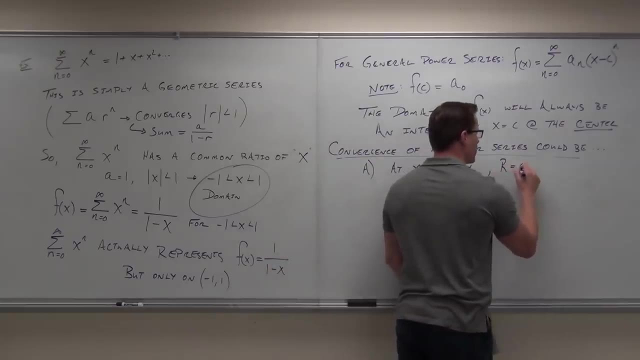 Does that make sense to you? So we can have power series functions which are defined just at the center and you have no radius of convergence. Therefore your r- I'm going to define r in just a bit- r would be zero and the interval would be this: 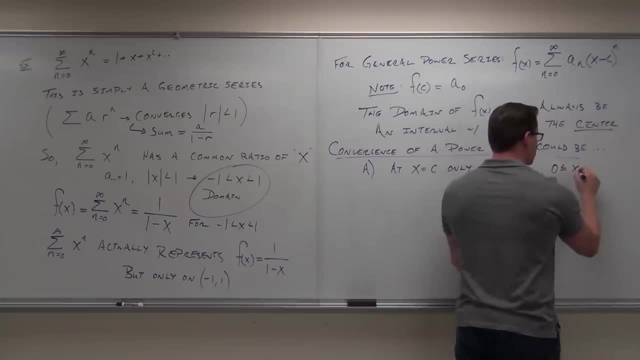 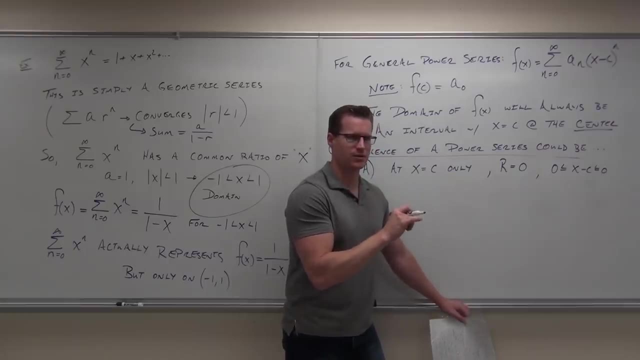 It's a silly interval, but it would be. zero is less than or equal to x minus c, which is less than or equal to zero. It would be the interval of convergence would just be right at the center. Does that make sense, Are you sure? 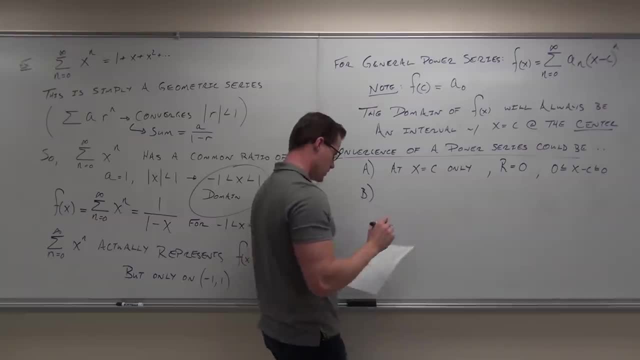 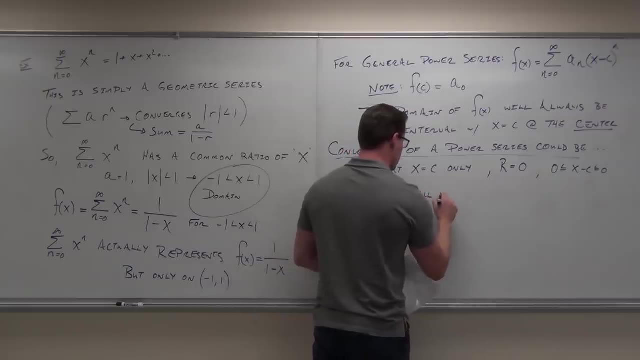 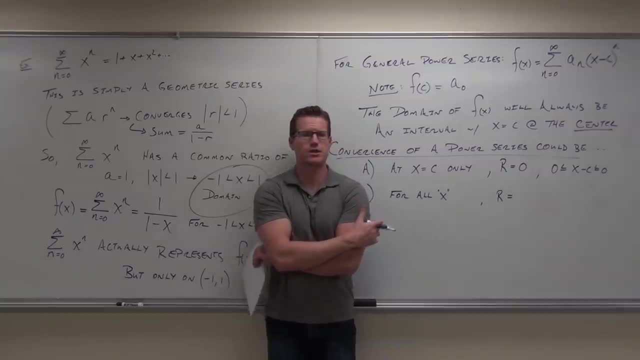 I don't want to say x. I don't want to say x. So are there times when a power series is always convergent? Yes, For any x. Yes, If I had a power series which converges for any x for anything. what's the interval of? 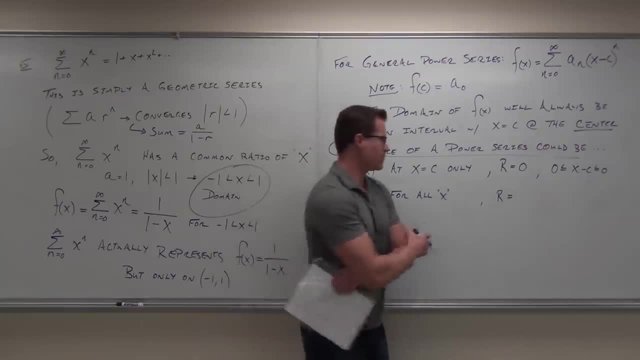 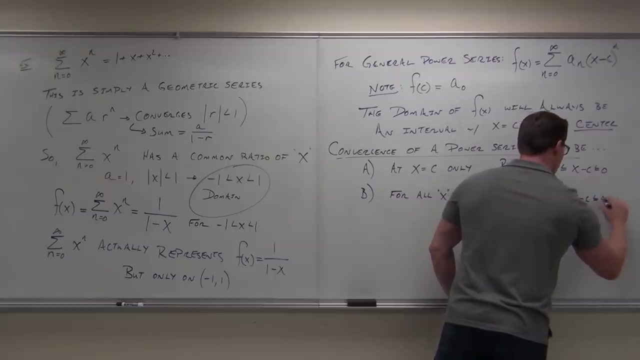 what's the radius of convergence? I would say Infinity. The infinity. It says: hey, you know what? I converged for any number. therefore the radius goes positive to negative infinity and therefore we would get an interval of convergence from negative infinity. 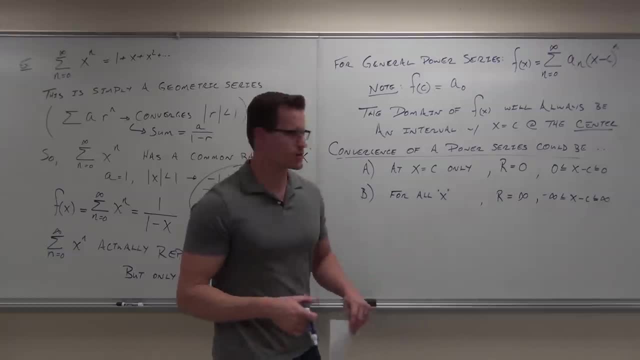 to infinity, centered at c, wherever that is. You guys, okay with that one? This one's not all that interesting. it just converges all the time. okay, This one's not all that interesting because it has no radius of convergence. 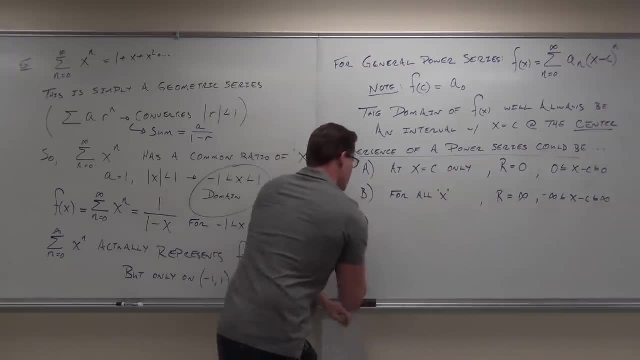 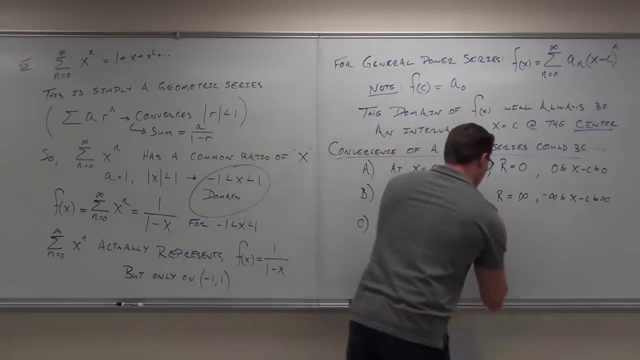 it converges at the center. cool C's where we like, I like. these are the more interesting ones to me. I like to spend most of my time here. We can have convergence for values that are within a certain radius, Where this is mathematically how you say this. 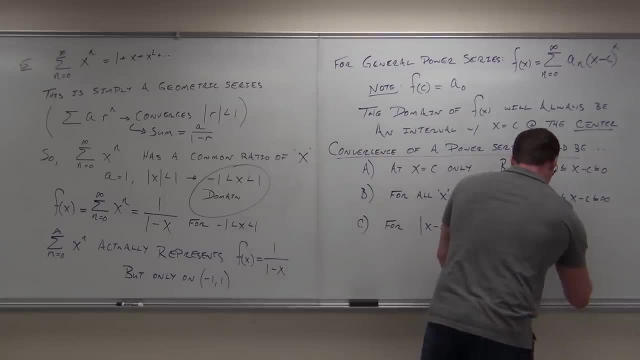 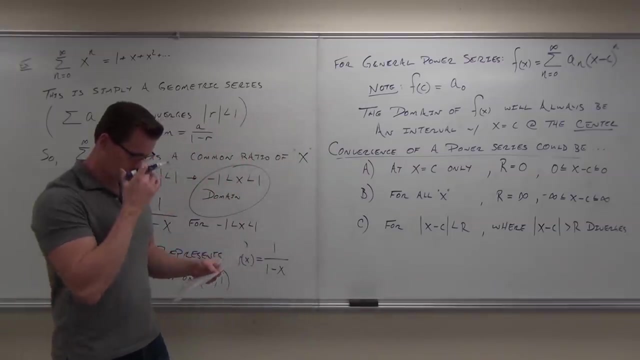 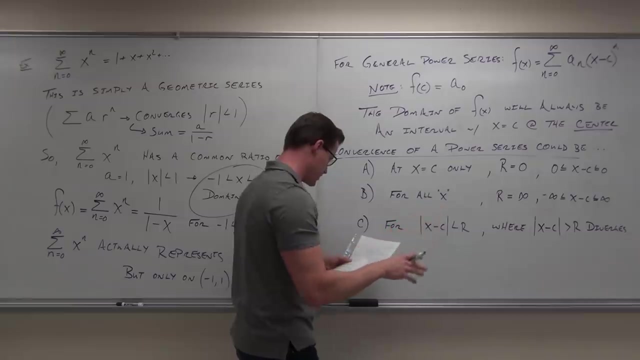 where, if you're outside of that radius, you get divergence. So let me let me make a couple notes on this one, because I haven't defined this yet. First thing, that r is called your radius of convergence. What it means is: how far is the radius of convergence? 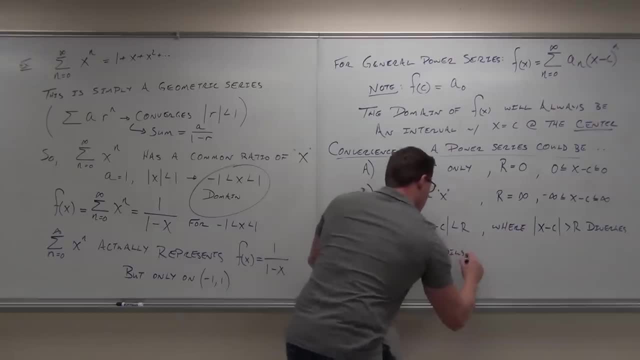 It's the radius of convergence, of the radius of convergence. So if you're outside of the radius of convergence, you're not going to get the radius of convergence right. You're not going to get the radius of convergence right. How far can you go above and below your center? 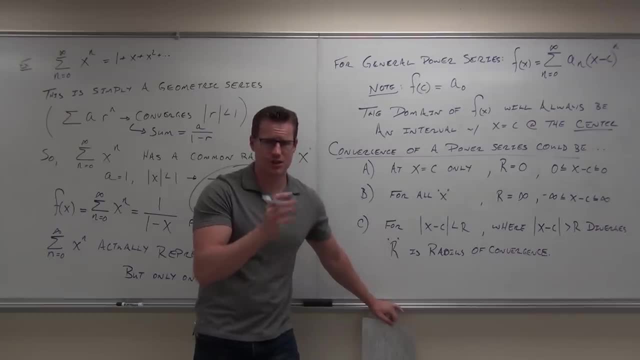 Remember, the center's always the center of your interval of convergence. okay, Always the center. So this is: how far can you go above and below that center of convergence and we'll still have a power series that works for you, Still has a defined power series. 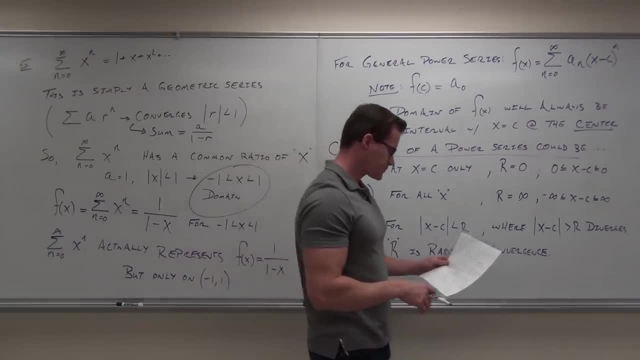 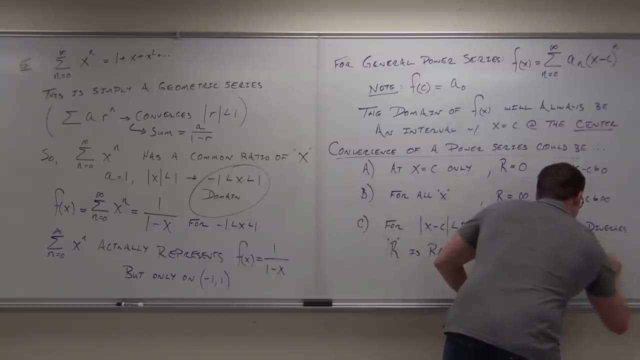 That's what the radius of convergence is, above and below. Now we can do this with the, since absolute value of x minus c is less than zero, which is less than r. what that means is that negative r is less than x minus c. 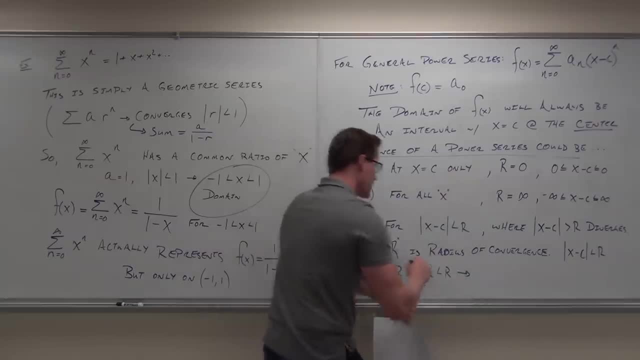 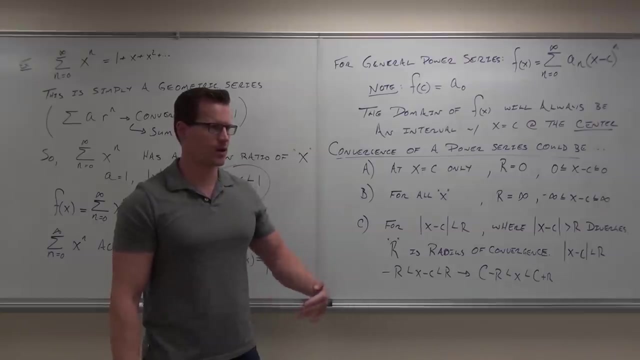 which is less than r, which means that if I solve for c, what we get is c minus r and c plus r. That, right, there is your interval of convergence. That tells you how far down and how far up you can go. Keep in mind whatever these two numbers are. 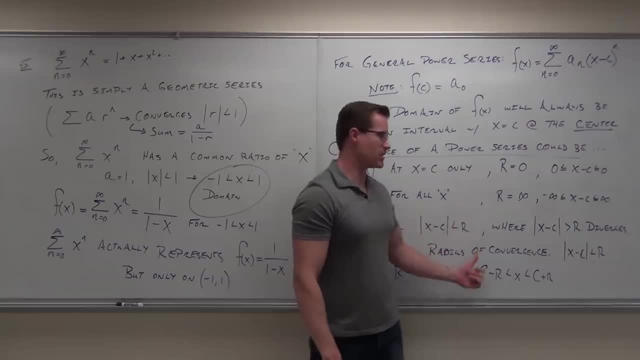 c will be in the middle of those, because you're adding c to a. c's going to be in the middle of these, right here. c's going to be in the right middle. So c's going to be in the middle of this. 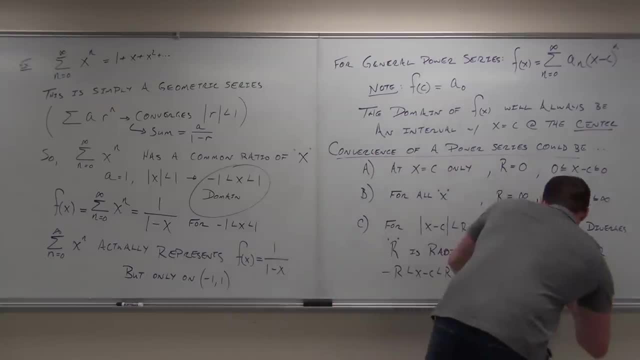 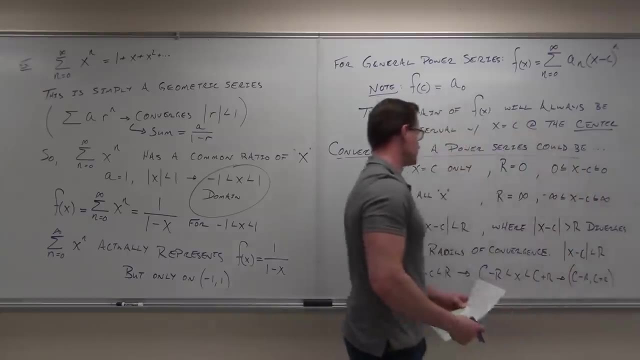 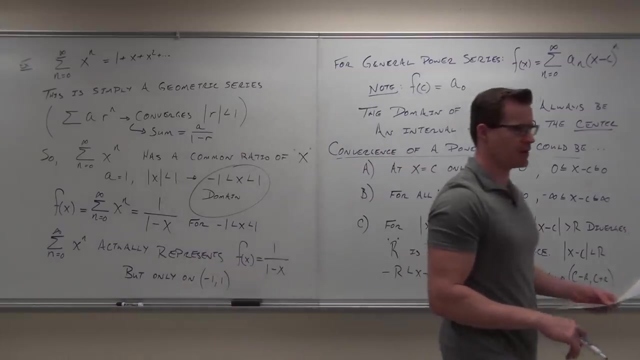 whatever your constant is, You can also write it this way: c minus r to c plus r. Now, last little comment. before I give you an example on this one, I want to get through at least one. Do you notice anything about this? 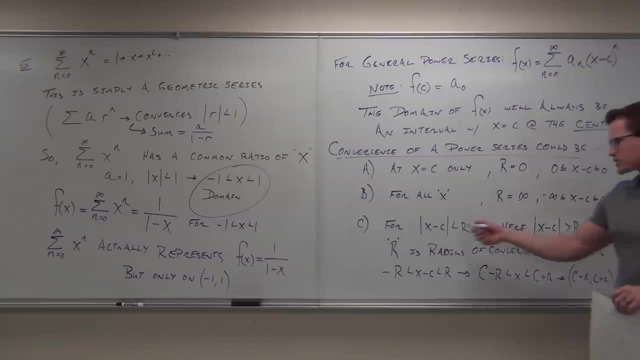 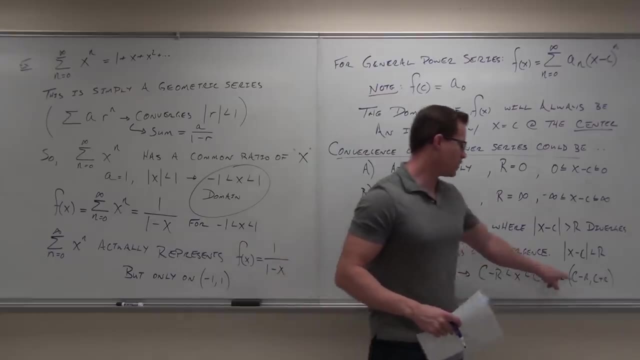 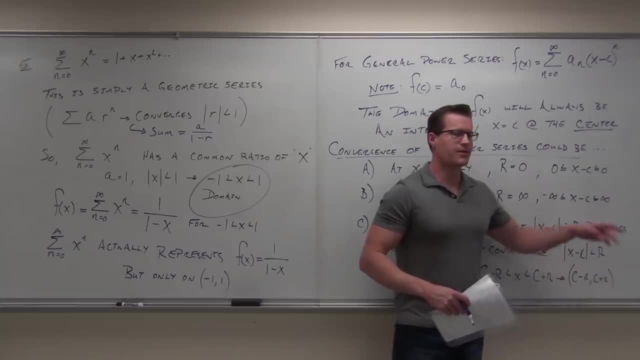 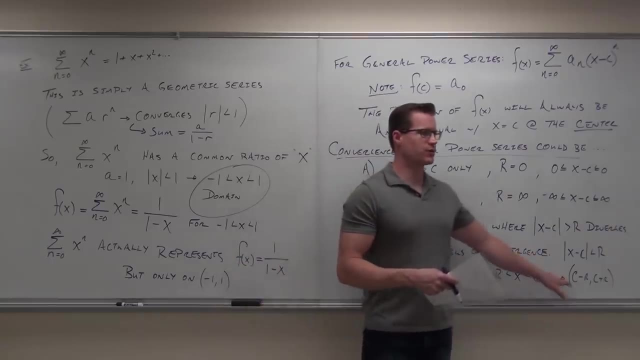 Do you get that? Now, I'm not saying anything about the endpoints. The endpoints must be checked individually. so the way we go through these is: we find first the interval of convergence. We find this, Of course. we find the radius of convergence before that. 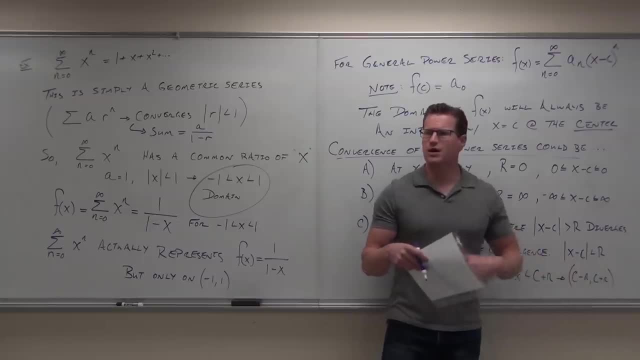 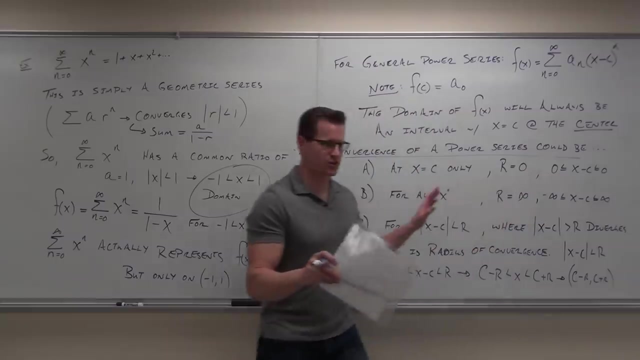 That's going to lead us to our interval of convergence. After that you must check, check whether each endpoint is included or not. Does that make sense? And to do that we use convergence tests because we've already done that. So we plug in a value for x. 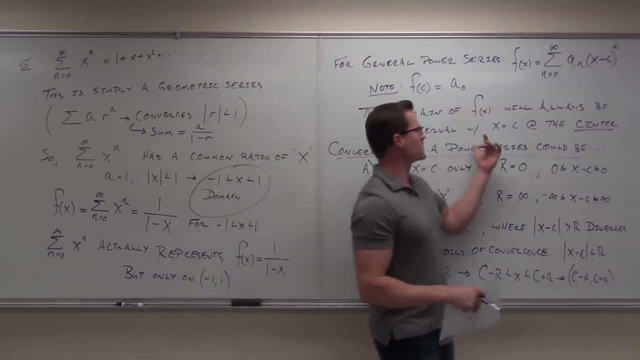 Listen, I'm trying to give you everything, without an example, I know. but if you had this one, I said: okay, we have a power series. Now plug in a value of x. What that value of x does is: it gives you a legit series. 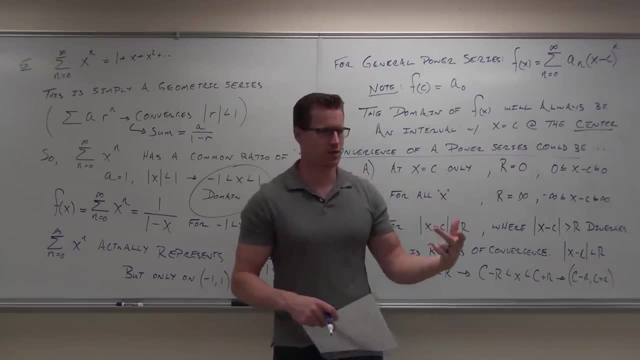 doesn't it Not a power series anymore, but an actual series which we can check with a convergence test? So to discover whether endpoints are included, you use a convergence test. You might want to write that down. So four endpoints use a convergence test. 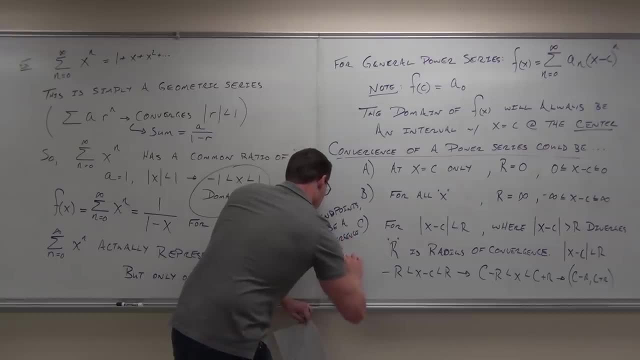 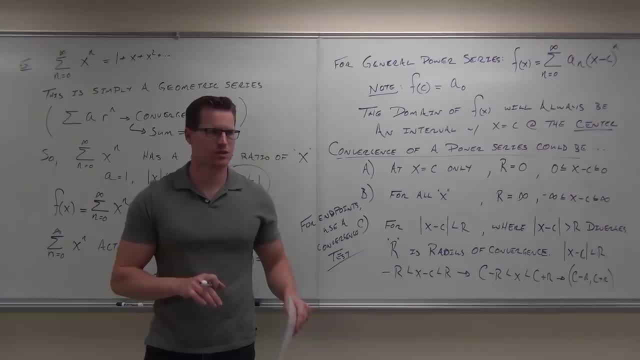 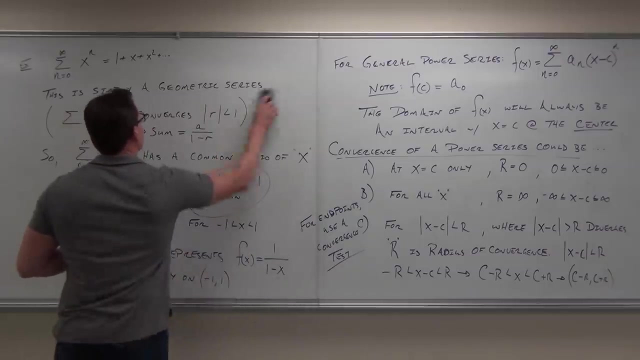 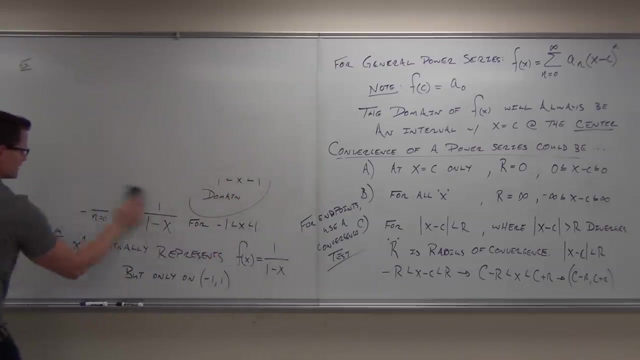 Four endpoints. use a convergence test. Would you like to see an example? I'd like to give you one before we head out, just so this is not all abstract for you. Yes, no, That clock's fast. Go for the gold, Mr Leonard. 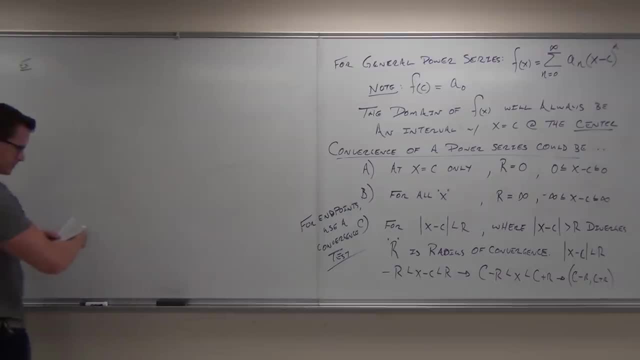 Go for the gold. That's what the relay for life is. Okay, so here we go. You find convergence first. This is going to give you the interval of convergence or divergence, or oh, sorry for the interval of convergence. 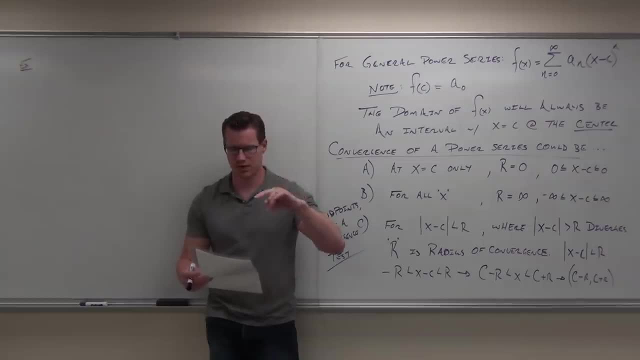 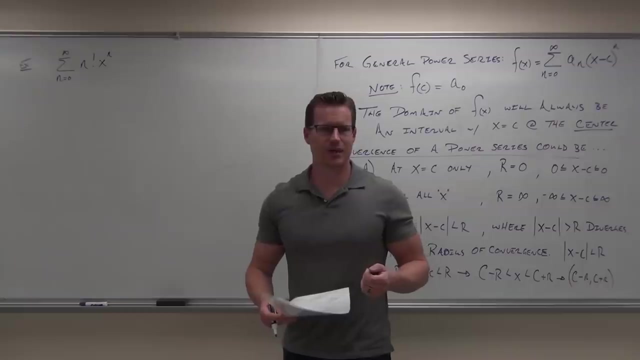 And then you use your endpoints and use whatever you can to find out whether those endpoints are included with a different convergence test. Let me give you this one. So, firstly, what type of series? Power, Power series, of course. What's in there that would probably help us? 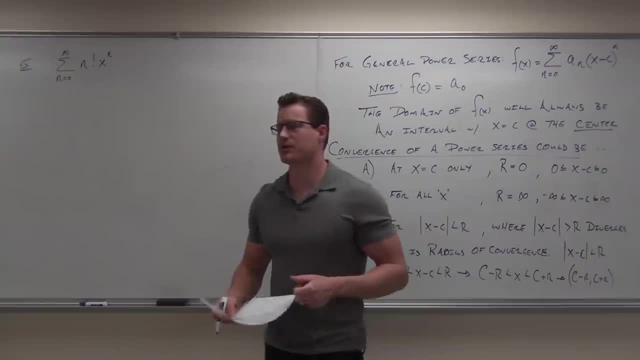 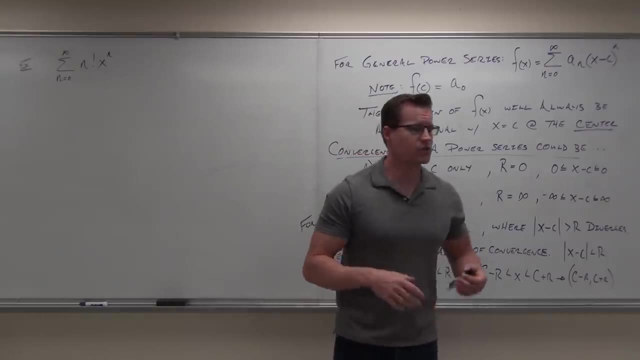 on what to do first. What do you see up there? Vectorial tells you to do something up here. Now listen, what we're going to do is we're going to do the same test that we've just done in our last section, because we still need to find out the interestingly enough, what we're going to do is we're going to do the same test that we've just done in our last section, because we still need to find out the interval of convergence. We need to find out when this thing converges. 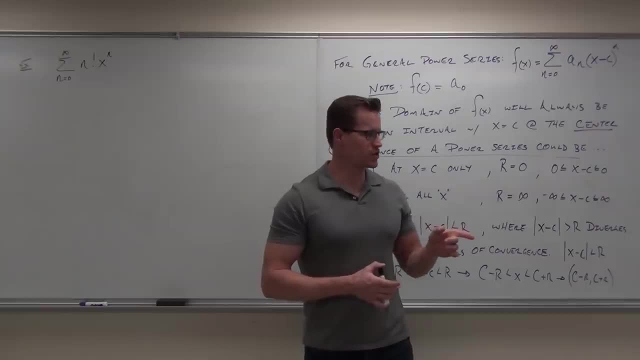 So what are we going to do with this problem? Ratio: We're going to do the ratio test. Now, keep in mind, when we do the ratio test, the ratio test says convergence, absolute convergence. actually, when the limit of our ratio is less than what number? 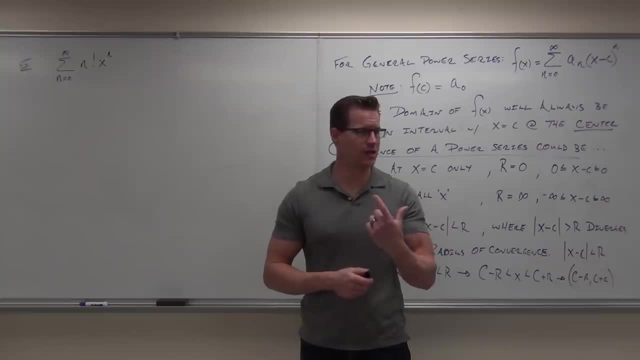 One Shows divergence when it's greater than one. It's inconclusive when it equals to one. Does that make sense to you? Yeah, We're going to use that here. So I'll be upright and straightforward with you. You're going to be doing the ratio test- an awful lot for this stuff. 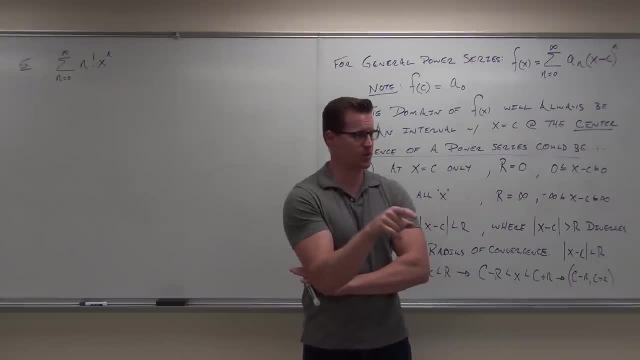 And the reason why is because the ratio test has a number associated with it. It says that it converges when something happens. Does that make sense That when something happens, that's going to give you your interval that you want? So let's go as far as we can in the next couple minutes and see if we can do it. 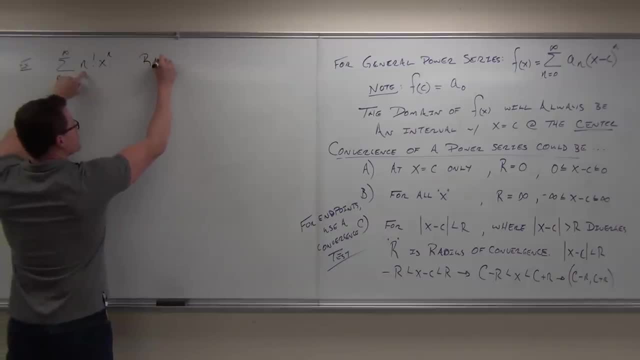 So, because we get that factorial, we're going to do the ratio test. Listen, I'm going to go quickly. I'm going to go quickly through the ratio test because I want to get to the punchline of this problem. So, ratio test. 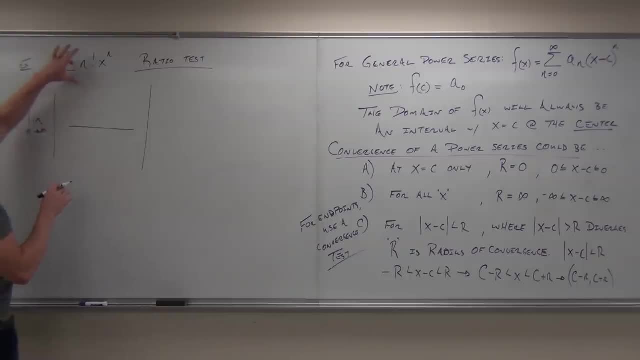 Ratio test would do. this Ratio test would put which one A sub A sub n plus 1.. Over A sub n plus 1. So we'd have n plus 1.. Bacterial X to the n plus 1.. 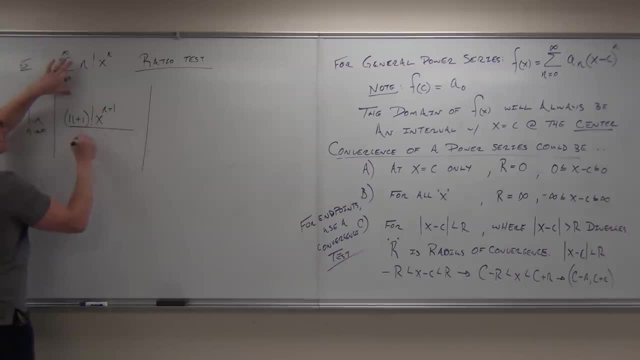 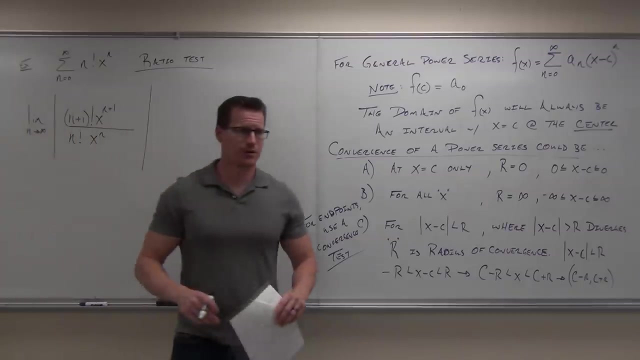 Okay, Uh-huh Over what? The same thing. sorry, The n, factorial of x to the n. Very good, That's exactly right. So let's do it. Can you simplify this stuff? Firstly, tell me something about the absolute value. 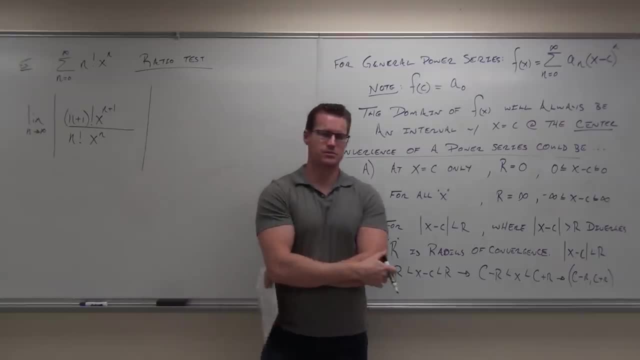 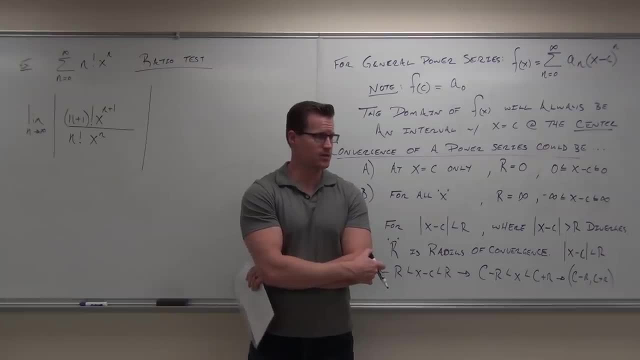 So be careful, You better keep it, You better not just arbitrarily get rid of this thing. Does that make sense? So be careful, Don't just jump to. don't create your own math, Don't. don't. don't jump to conclusions here. 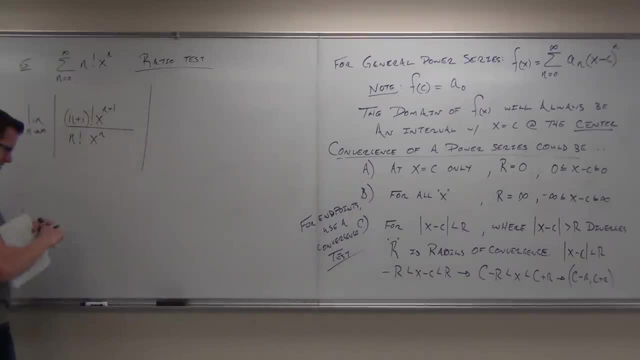 That would be bad. Now can we simplify this? What simplifies Lots effectively? Yeah, lots. We can do the x. Where's the x going to be? The x would be here. This is x to the n times x. 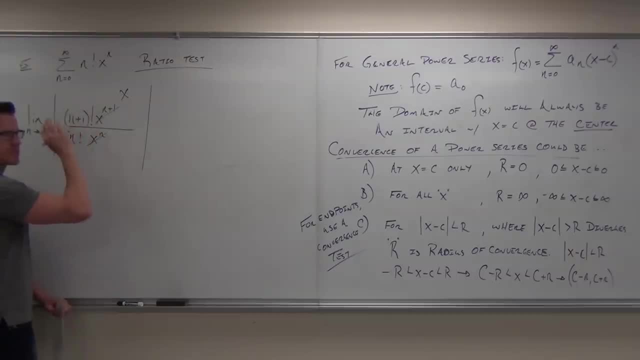 X is on the numerator. This Do you remember doing. we've done this several times. You're going to get it several times more. If this is n factorial, this is n factorial times, n plus 1.. So when I simplify that, I get an n plus 1.. 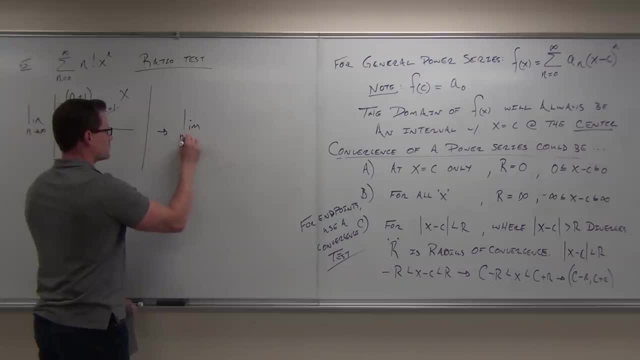 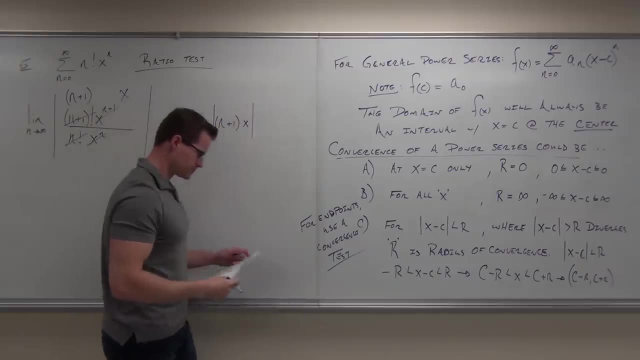 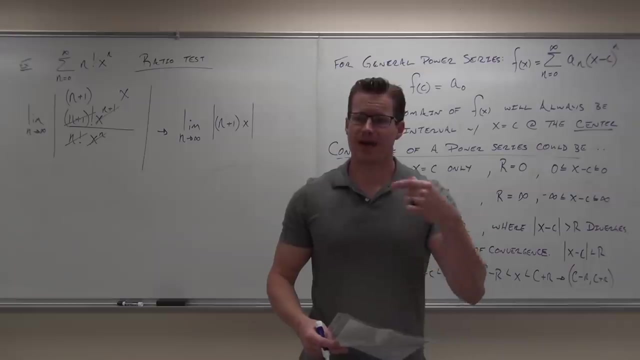 So what we get is a limit: n approaches infinity, n plus 1,- in parentheses, times x. Are you okay with that one? Yeah, Now strip off everything besides your x's, outside of the absolute value. Here's why you can do it. 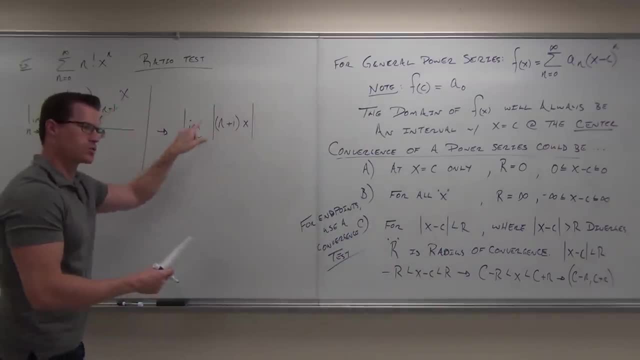 Is n plus 1 always positive? Yes, Yeah, that's what we're going to do. That's what you guys probably meant. when you said absolute value, You were thinking of just the n's. So when we go, okay, well, that's always positive. 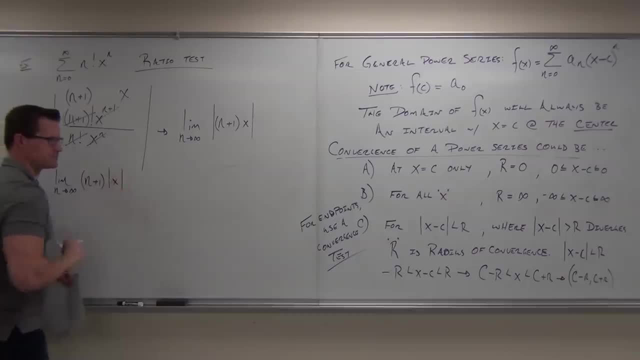 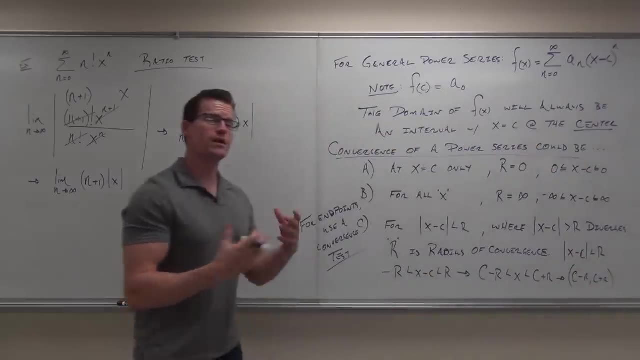 I can do n plus 1 outside of my absolute value. And now we're going to talk about this for a second. We're going to talk about when: When this will converge and when this will diverge. So real fast, I'm going to write this twice. 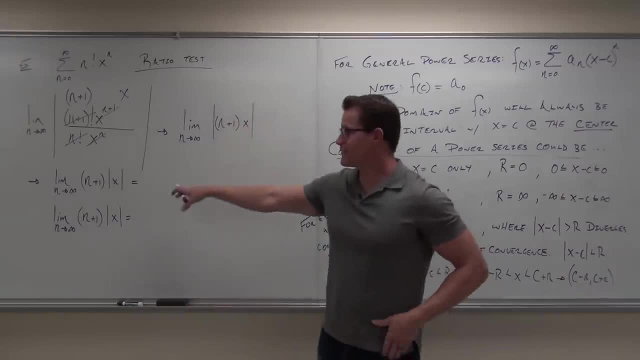 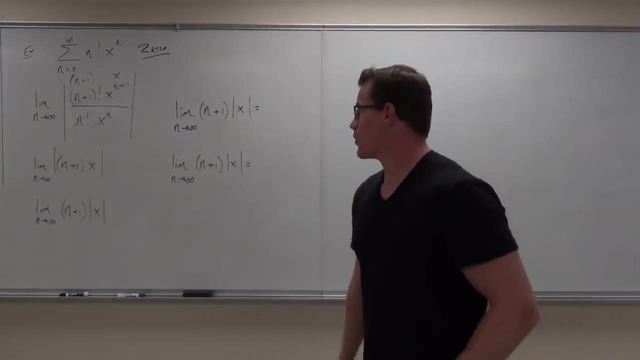 You know, actually, would you remember if I gave this to you tomorrow, Because I want to stop right now and I don't want to keep you any longer. So we're working on our very first power series And try to show when this thing is convergent. 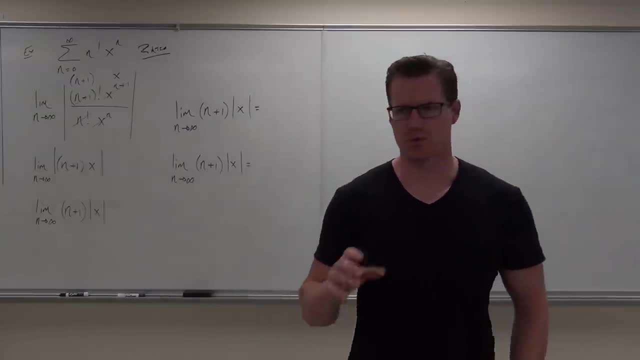 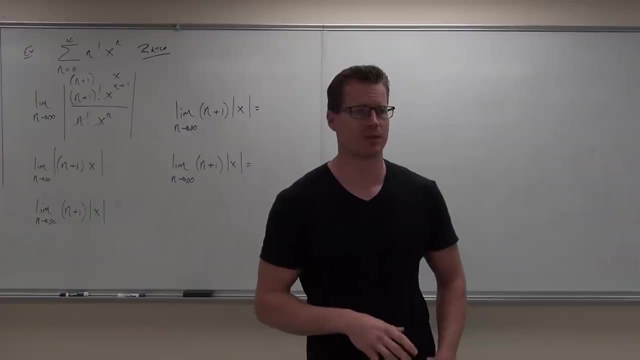 Now the idea is use some sort of a test- typically it's going to be the ratio test- to find out where this series is convergent. You see, the idea was- and I'm not going to repeat the whole thing, but the idea is this power series represents some sort of function, but only where it converges. 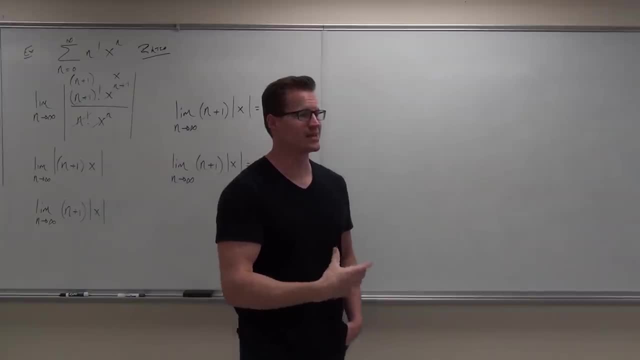 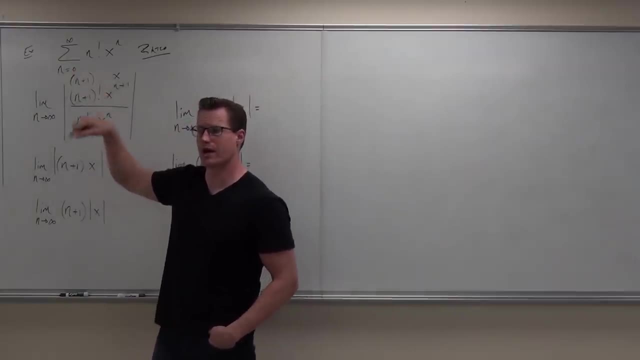 So we're going to find out where this converges, what our domain is. Basically, the domain is the interval of convergence, because therefore we can define our function as this series on some domain where our x makes the series. That was all practically our last time's lesson. 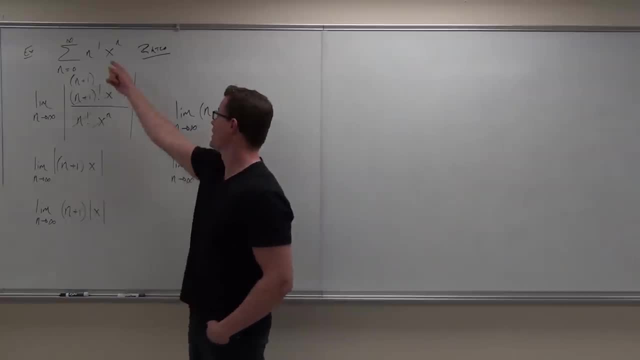 Did you guys? you got all right with that so far, Yeah, So what we've done is said: hey, you know what that's got? factorials, Let's use a ratio test. So we're going to work this down. 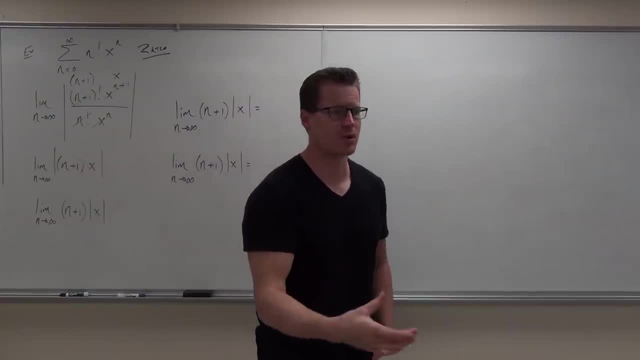 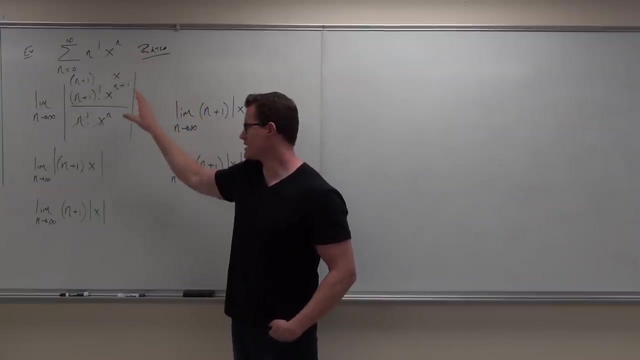 The reason why we like the ratio test is because it compares it to some number. It says this thing is going to converge when the limit is less than what number? Let's try this again. The ratio test says that this series will converge when the limit is less than what number? 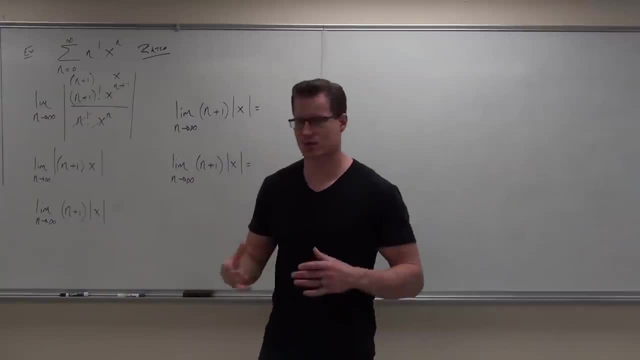 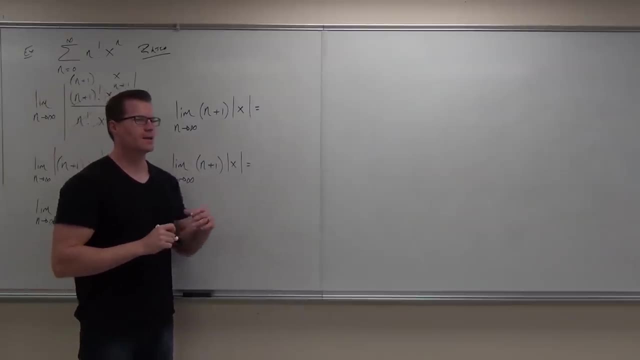 Now here's the deal. Please listen carefully, because this is where it's coming from. N's approaching infinity, right Yeah? So let me put in any number for x. What is what's infinity plus one? by the way, 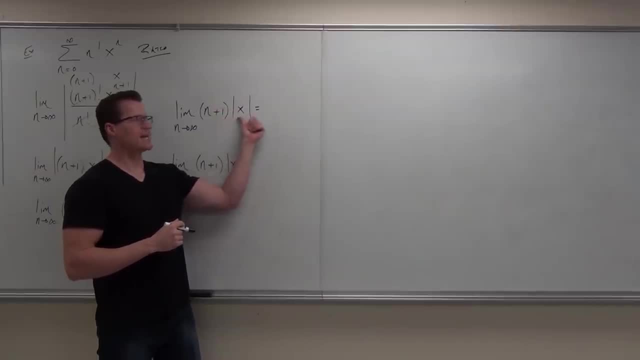 Infinity. So this is going to be infinity. If I put in any number for x, take an absolute value of it and multiply it by infinity, what's it going to be Infinity, Unless that number is Zero. I don't care if it's negative, because if I take the absolute value of the negative, it's going to make it positive, right. 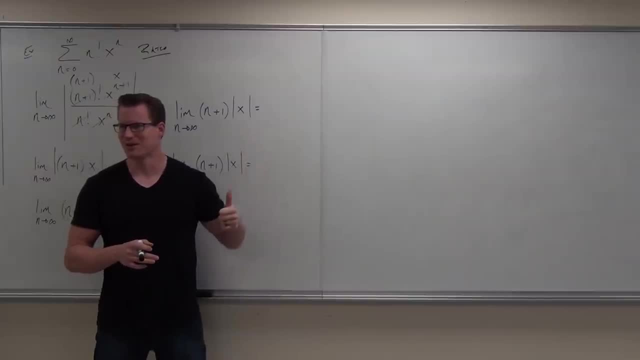 So if I put in negative a billion, well then you're going to get positive a billion. Hello, it's going to still be infinity. What's the one number that you can multiply by and get zero? Now, if you're thinking: well, wait a minute, isn't that an indeterminate form? infinity times zero. 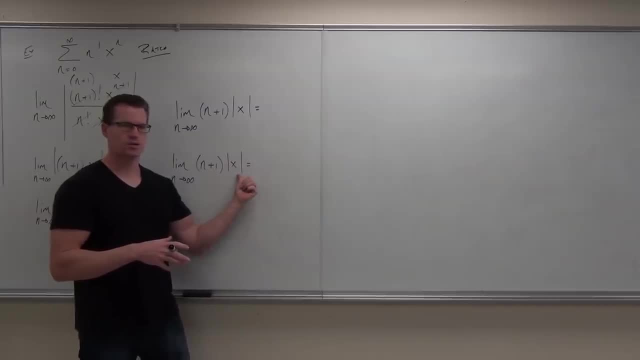 Not really, because this is x, It's not an n, It's not in terms of what this is. So this is legitimately zero. all the time zero. all the time zero. Does that make sense? Yeah, It's different. 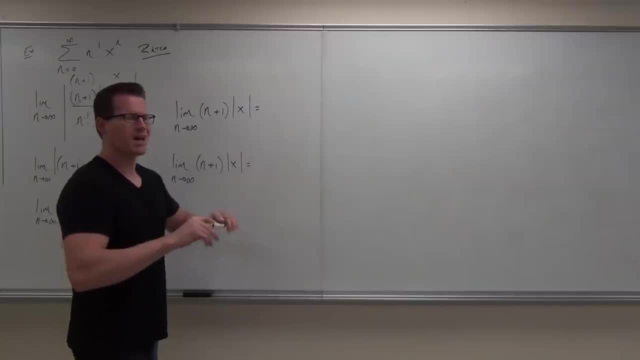 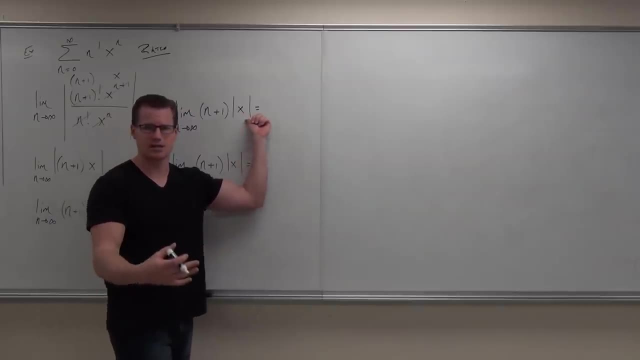 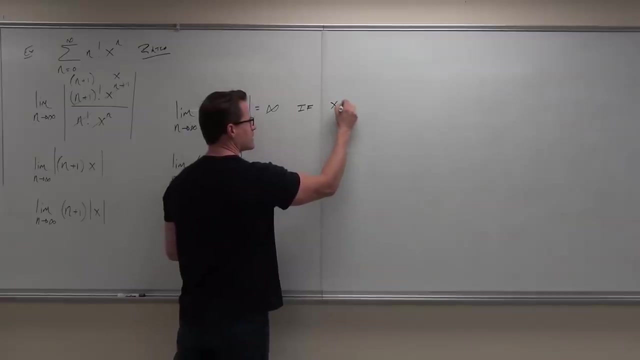 So we have two situations. We have a situation where if x is any number besides zero, if x is any number besides zero, I take an absolute value of it. it's positive, It's some number. I multiply it by infinity and what I'm going to get is infinity if x is not zero. 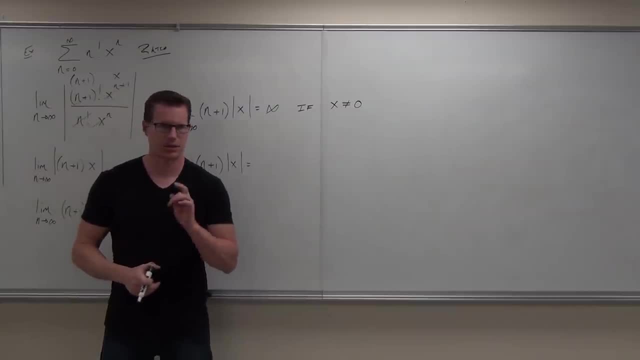 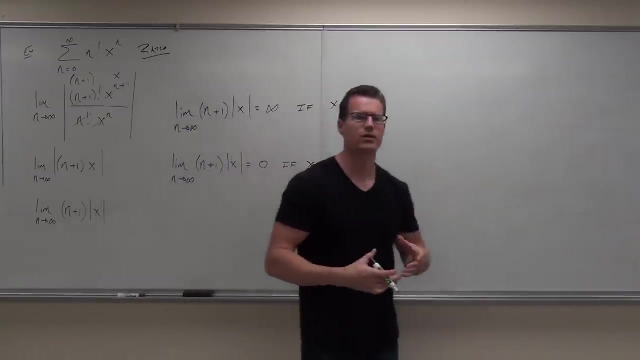 Does that make sense to you? Yeah, Are you sure? Yes, Okay, So if x is zero, I don't care what this is. how much is this going to be Zero? Zero If x does equal zero. Now here's where the type of test we use comes into play and why it's so important. 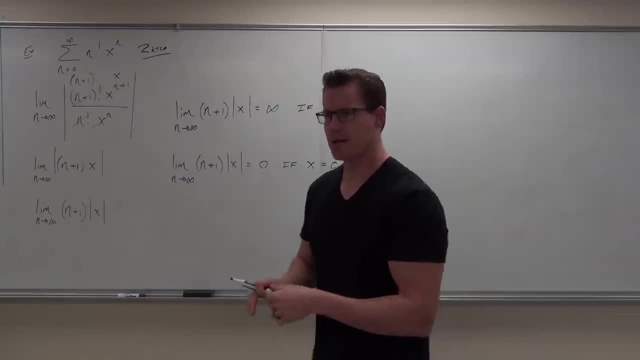 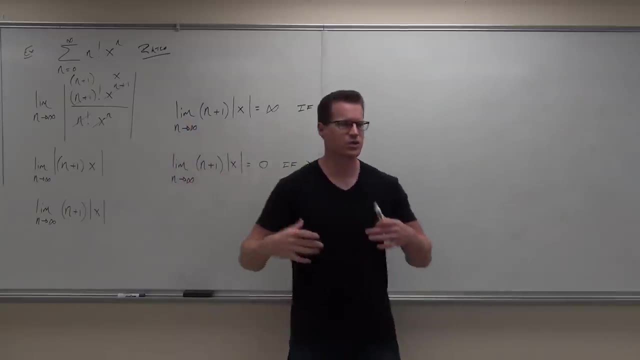 Are you listening? Yeah, The ratio test says that we're going to get convergence or divergence based on what number we get. So when we get infinity, all you've got to do is compare these things to one. So is infinity more than one or less than one? 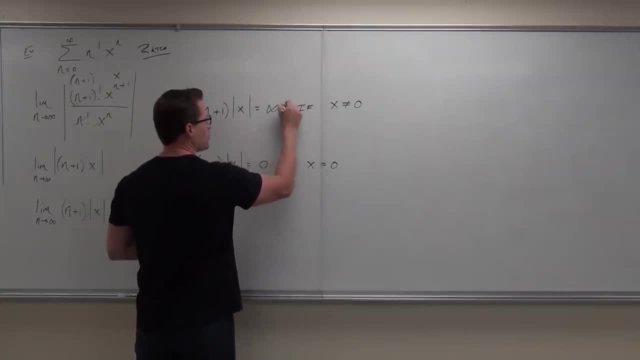 More than one, Of course it's more than one. So by the ratio test, because infinity is greater than one, by ratio test we get what is it when it's greater than one? Divergence, Divergence. 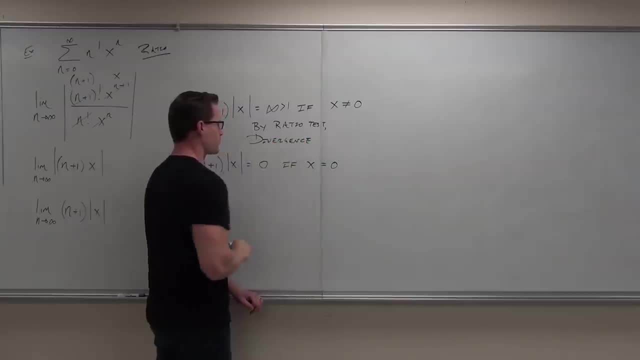 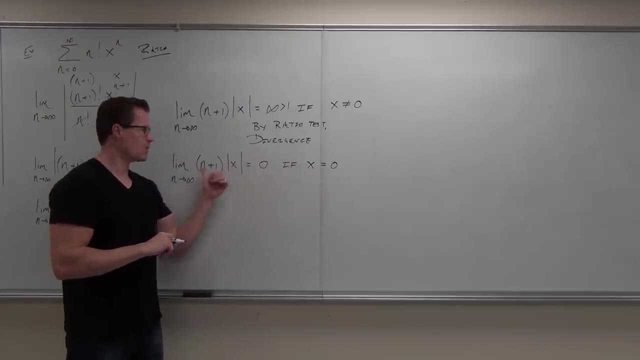 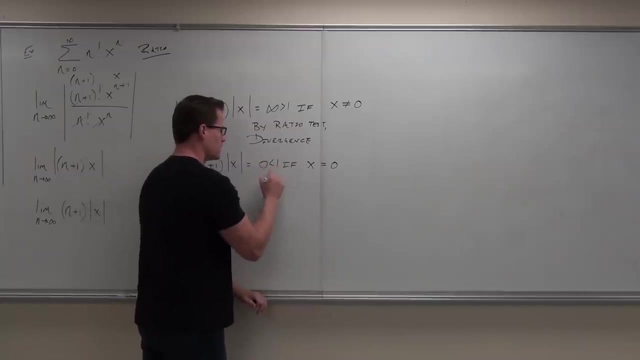 We get divergence. Now what about this one? When x does equal zero? when x does equal zero, we get our limit equals to zero. Well, how's that compared to one, Greater than or less than Less than So, by the ratio test. 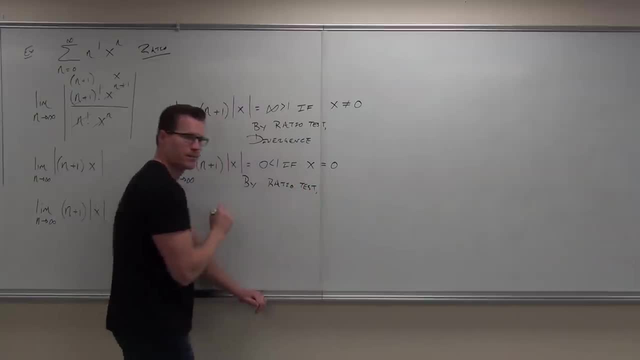 Absolutely convergence. We get what: Absolutely convergence, That's right, Absolutely convergence. I don't really care so much about the absolute part, but we do have convergence. You see, we said nothing about the function. has to the domain is where the x values make it absolute. 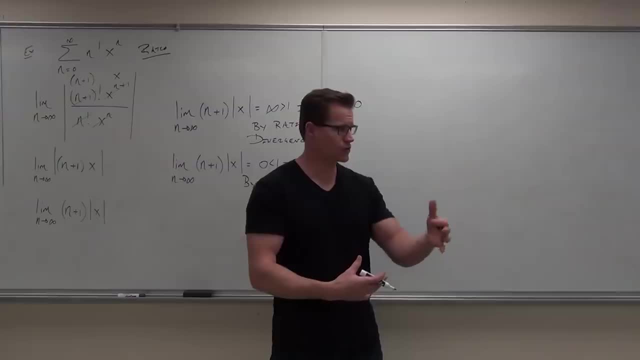 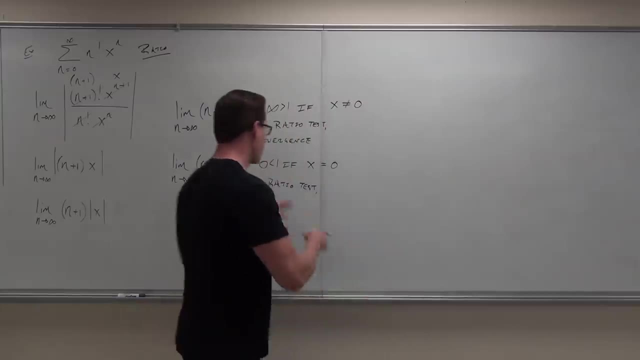 Absolutely convergence, It's just convergence. So where it does say absolute convergence, you're absolutely right, because ratio test gives us absolute convergence, We care more about the convergence itself. Does that make sense to you? So by the ratio test, this thing is absolutely convergent. 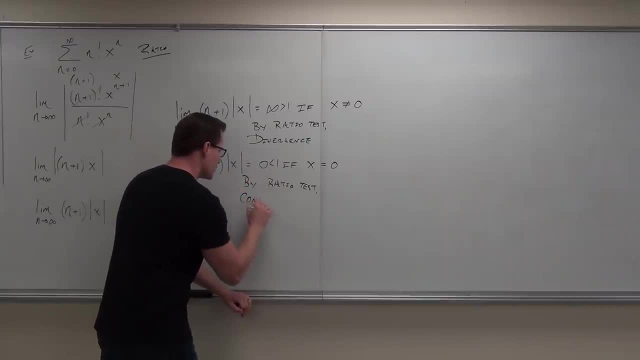 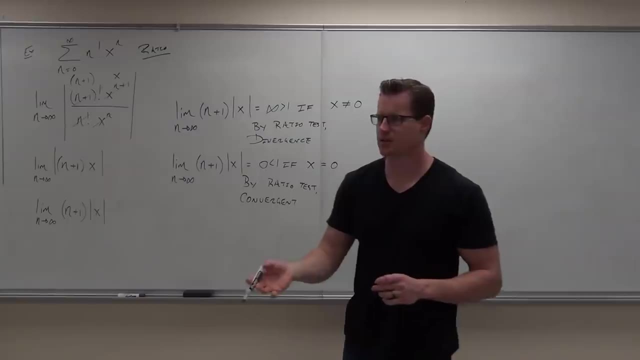 Therefore, it must be convergent. Do you feel okay with that so far? Now, here's what this says to you, and we're going to do a few more examples to illustrate each type of case that you can have. okay, So here's what we've done. 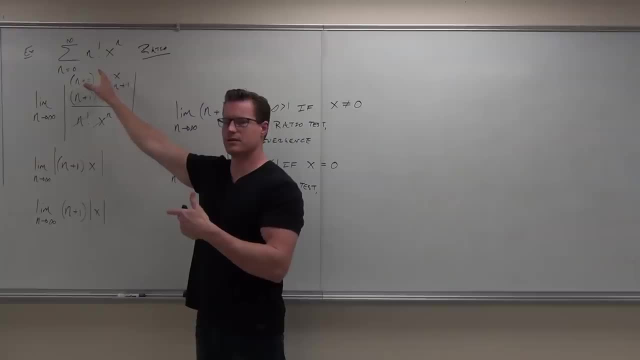 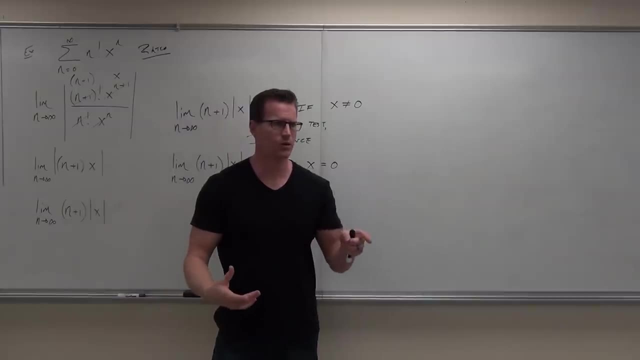 We said: how are we going to? how in the world are we going to find the domain for this? We already know a couple things. We already know: a power series represents a function. What we don't know is where The where is the domain? 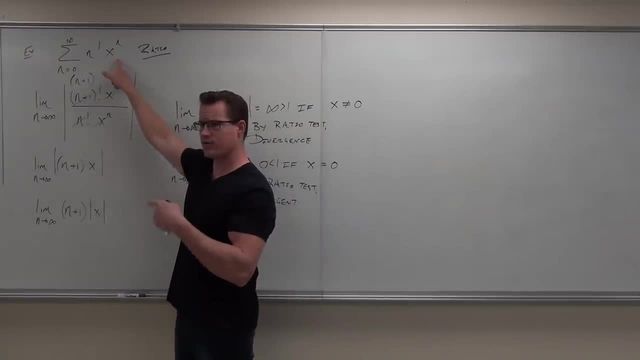 That's what you're trying to find, So you go. okay. what we find out with this is where this function is defined, So where a function which represents a power series is defined. Well, all right, Well, cool. 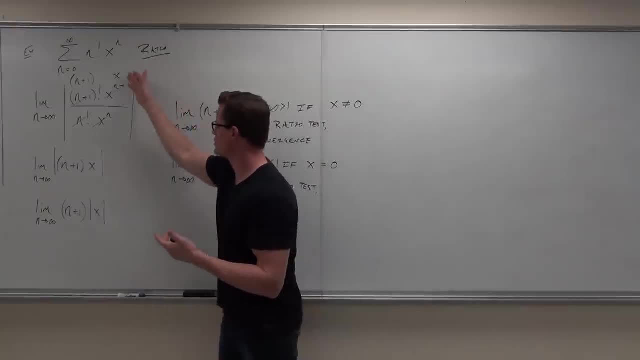 Use a ratio test, because the ratio test will tell you where. So we work this down. We've got a ratio test, No problem, Pretty easy. We've got absolute value, but n is always positive, so absolute value is gone here. 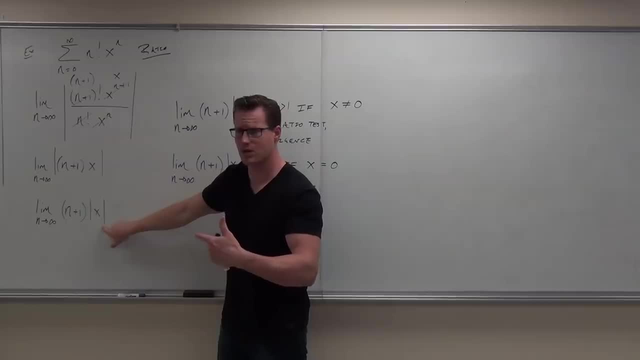 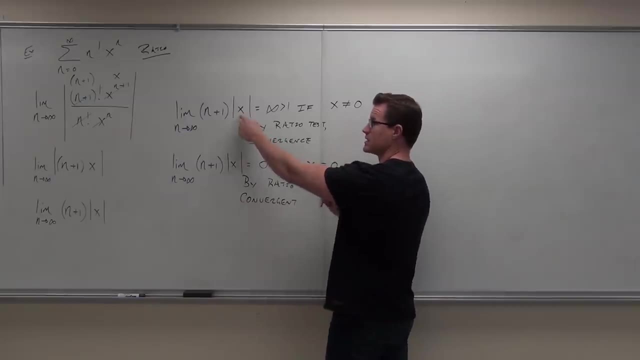 We have absolute x. This is not gone, because x can be negative. x is any number, All right. Well, there's two situations We have. if x does not equal 0, doesn't equal 0, that's a number. 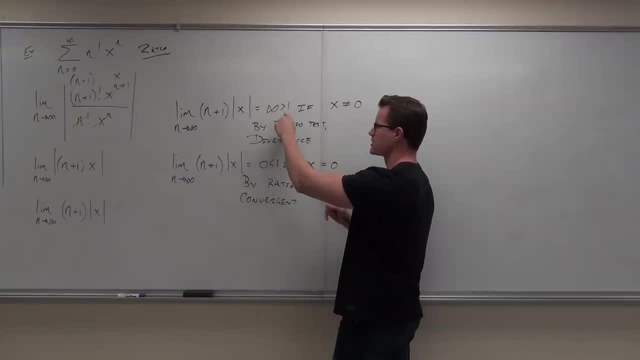 A number times infinity gives you infinity, Because infinity is greater than 1, we say, hey, you know what? By the ratio test, that's diversion. Here's what that means If I plug in any. listen carefully because this is a big deal okay. 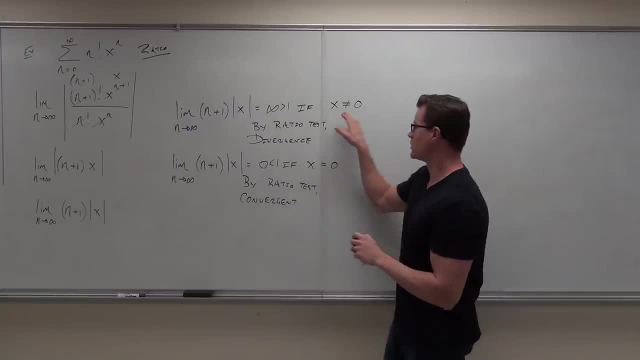 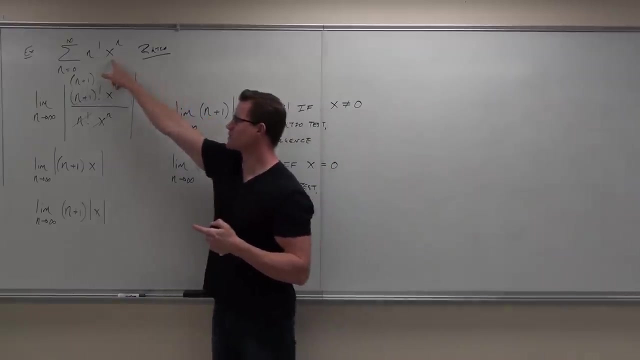 If I plug in any number besides 0, do I have convergence or divergence? Divergence? Therefore, our function is not defined for any number that is not 0. Does that make sense to you? So you go all right. if I plug in x does not equal 0, a half, a third negative, 1,. 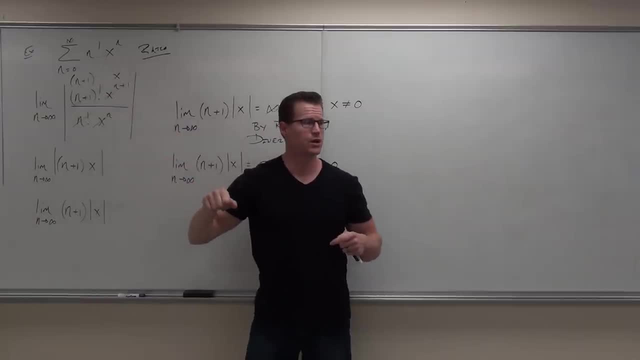 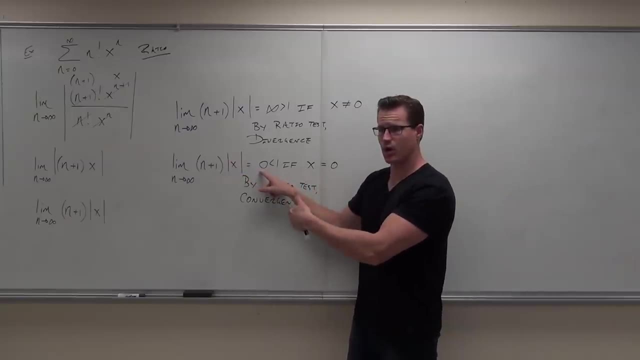 I don't care what it is. this thing is going to diverge. Now the other thing says: okay, what if x does equal 0? If x does equal 0, then our limit equals 0.. By the ratio test, that's less than 1.. 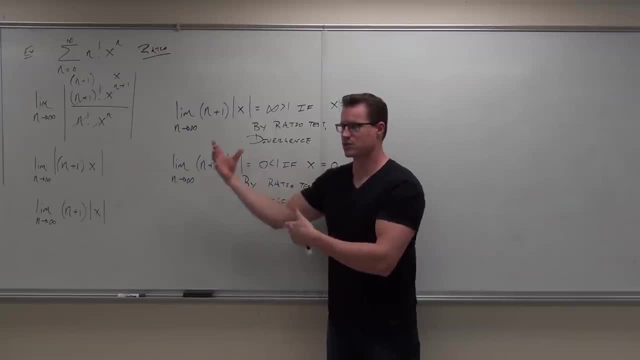 So by the ratio test that is convergent for our series convergence And since our domain for our power series, the function of our power series is all x's that make our series convergent, we only have one value that does that. 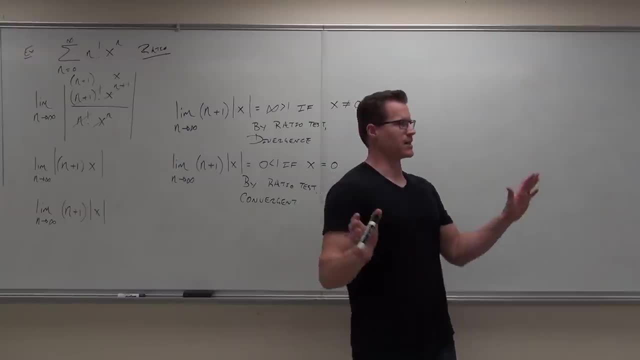 What's the one value of x that makes this thing convergent? That's the idea. So this is one of those cases. Remember, I gave you three cases of what you can have in your power series. I gave them to you last time. 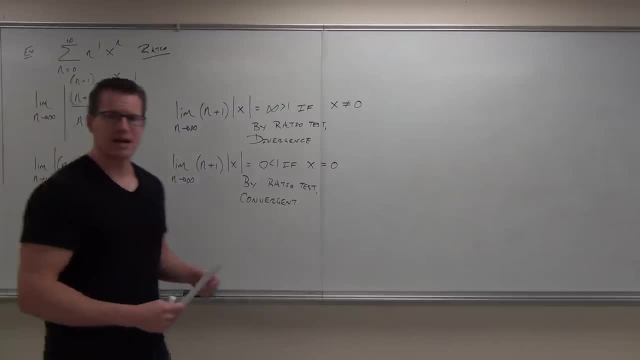 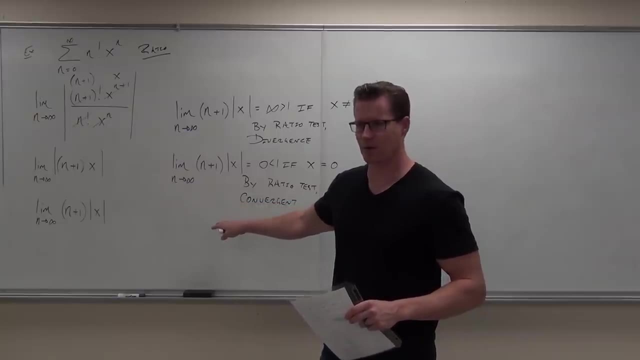 What I said was that your power series could be at the center only only at 0. That's this case. There is no radius of convergence. The radius is 0. There's no space there. It says there's only one number you can plug in to make this series convergent. 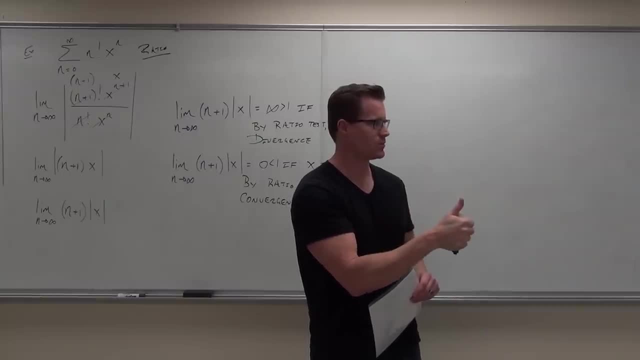 and the one number you plug in is 0. That's it. There's no radius of convergence, There's no interval of convergence, It just happens to be 0. You sure you're okay with that. And it happens to be at the center itself. 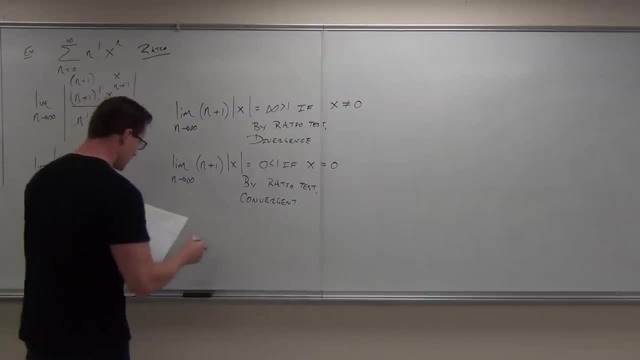 So what we get out of this? we go, okay, cool. So by the ratio test, our domain is simply: x equals 0. It says so right here. Also, little side note: the ratio, sorry, the radius of convergence is: 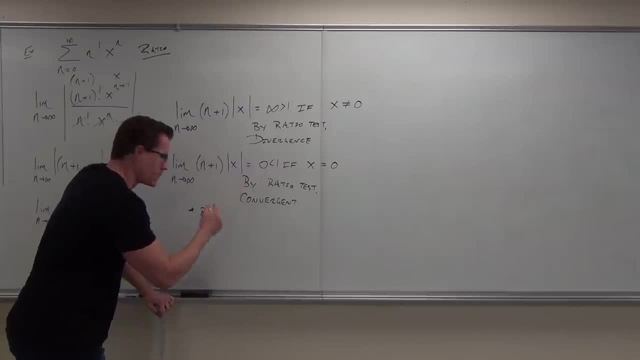 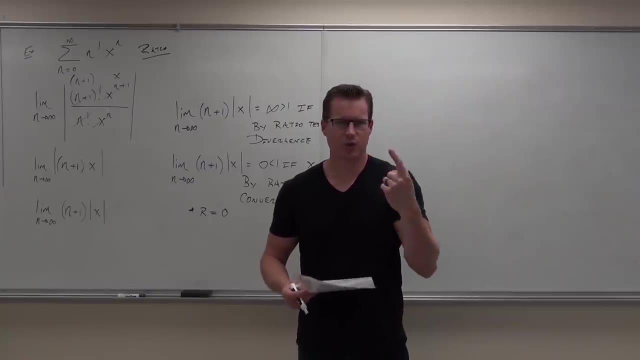 what's the radius of convergence? 0.. It's only one number. Radius of convergence is 0.. Would you like another example that's a little bit different from this? This one has only one number that you're good at. It's only at 0.. 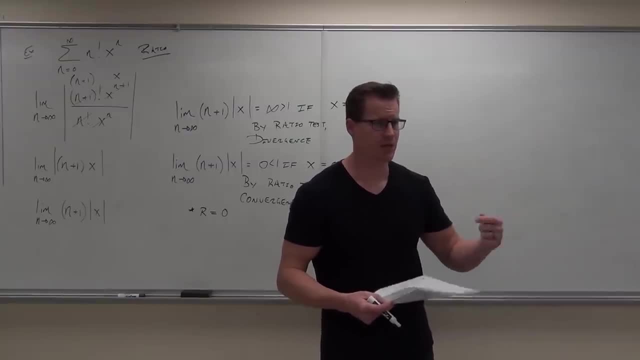 There's no other number that works. Therefore, our radius of convergence is 0.. It's nothing. It doesn't go above 0 or below 0. It's exactly at 0.. Show of hands. if that made sense, Let's continue. 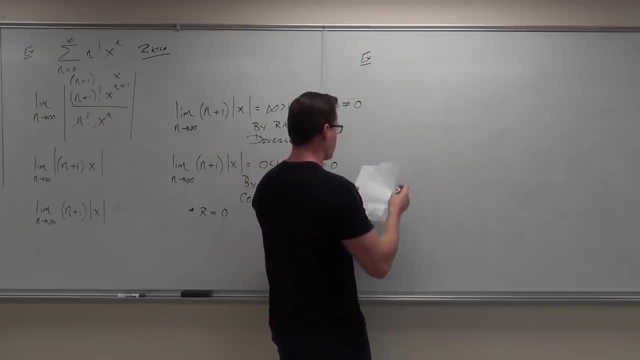 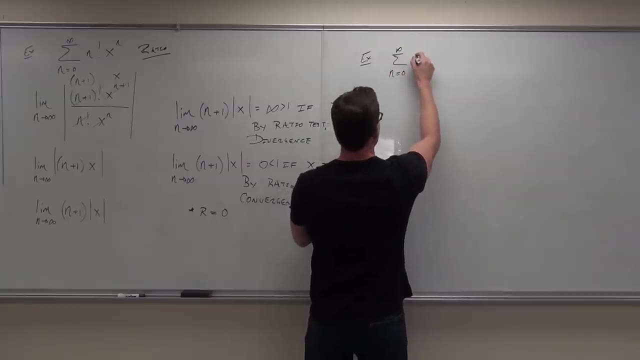 I want to do as many examples as I can to give you every type of scenario here. Okay, true or false, This thing is a power series, True or false? Absolutely. What tells you it's a power series? It's right there. 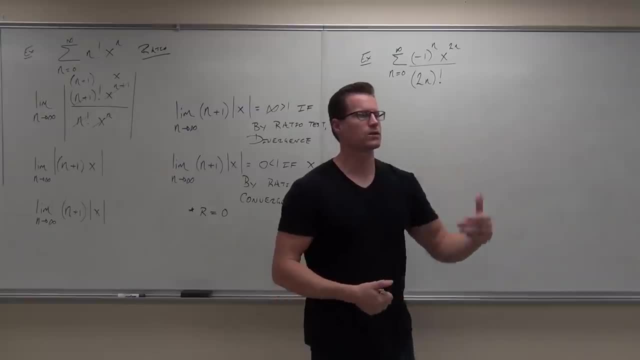 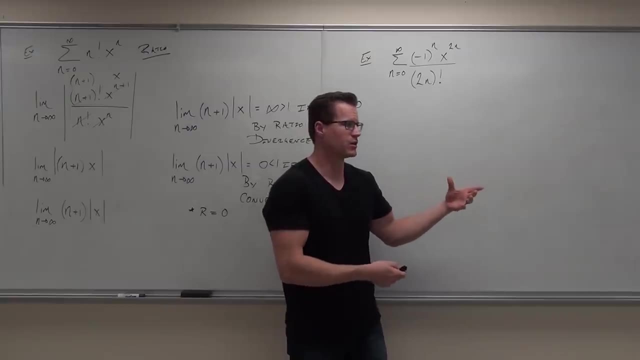 Right there, That's a power series, Not a problem. Now, talking about our power series, does it represent a function Or can we represent this as a function? This is a function in terms of x. For sure, it's a function in terms of x. 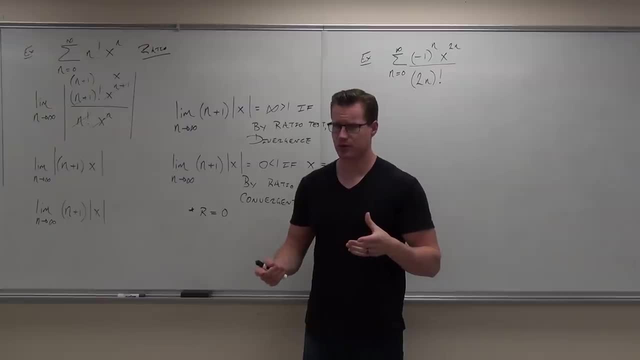 Now, do we know the domain for such a function? No, but we're going to find it. That's the whole idea. So what we know is that this thing is a function of x. When I write it out, it's a function of x. 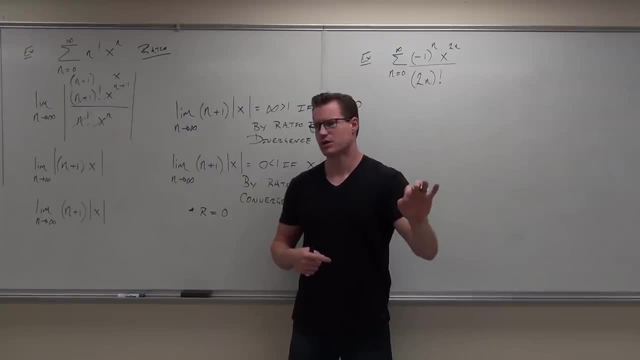 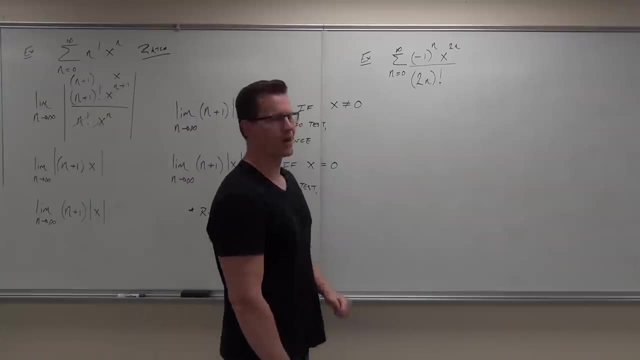 But it's only a function of x where it converges The. where it converges is our domain, So we're going to find out where the thing converges. Well, let's try it. How do we do that? Take the ratio test. 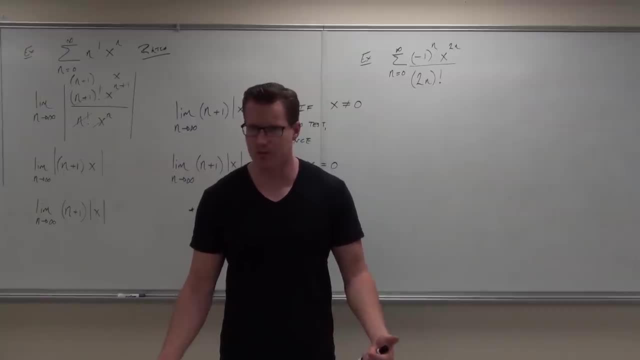 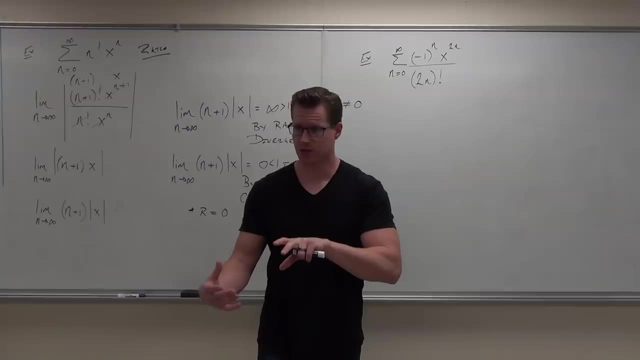 Let's do the ratio test. The ratio test is great for us for a number of reasons. Firstly, it gives convergence and it gives divergence right. Yeah, It tells you where your series is convergent and where it's divergent. What that means is you can find your domain from that. 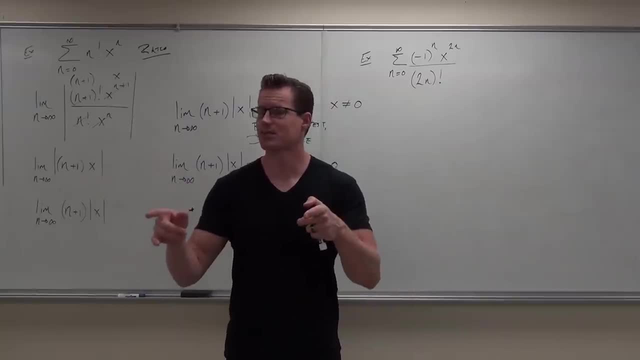 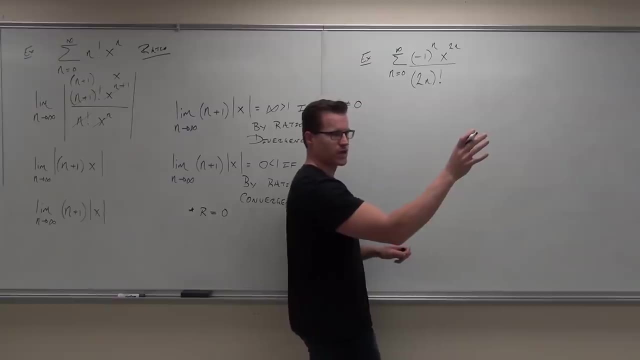 That's why we use the ratio test so much. That's why I said it's so powerful. So let's set up the ratio test. I want you to set up the ratio test right now, See if you can do it. So you're going to write out what you're doing, okay. 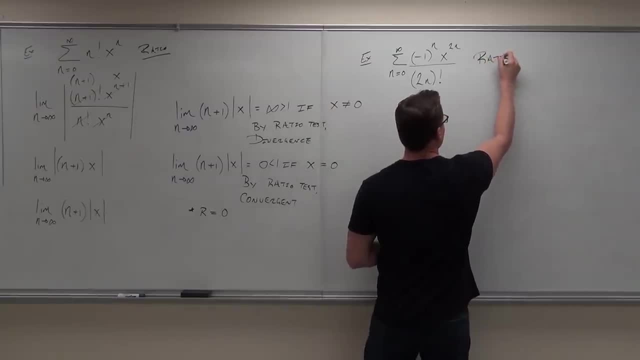 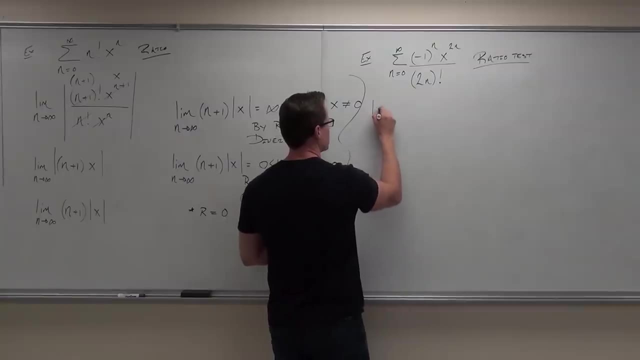 Write out ratio test. Don't forget your absolute values, because ratio test always has absolute values. Don't forget that one of these goes on top: a sub n plus 1 or a sub n What goes on top? a sub n plus 1.. 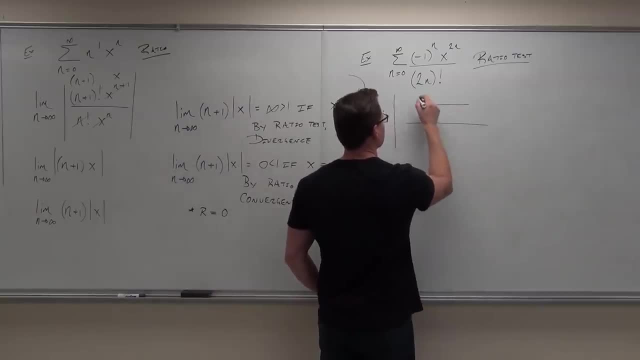 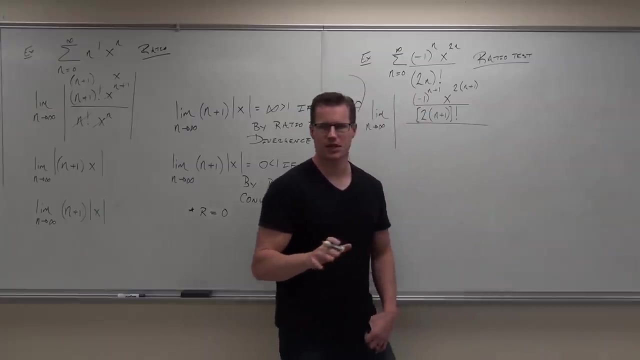 Okay, I want to stop you right there. I want to make sure that you've got this. Let's see, I'll have you do the rest of it kind of on your own, but I want to make sure you got at least this part right. 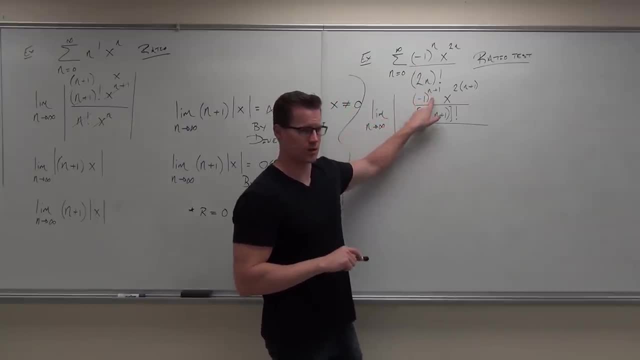 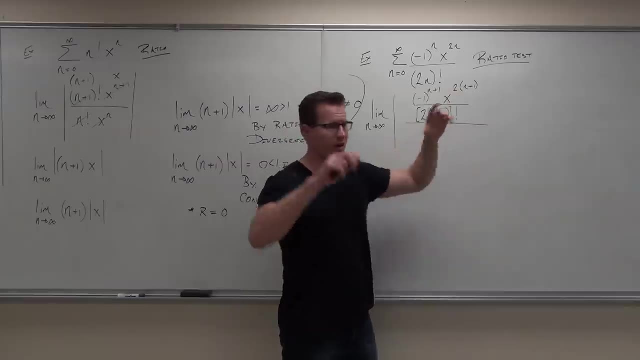 Did you get negative 1 to the n plus 1 here? Yeah, Did you get x to the 2n plus 1 or the 2n plus 2?? Yeah, You got n plus 1 in parentheses or you did 2n plus 2.. 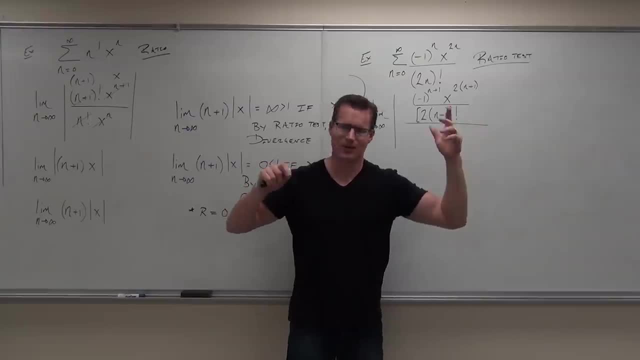 You distributed it correct. Yeah, You didn't get 2n plus 1, did you? No? Okay, Good, And you got the same thing here 2 times n plus 1.. Of course, we're going to distribute that. 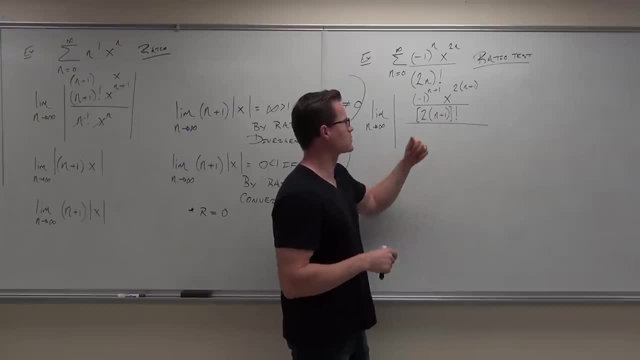 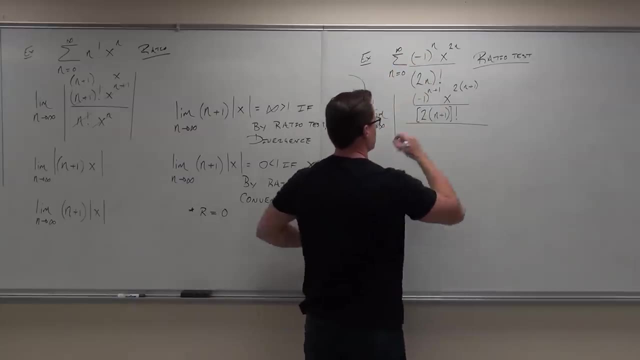 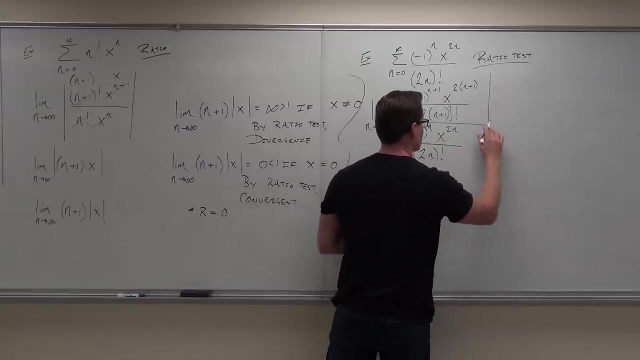 No problem, We probably could. And then factorial: How many people got that one? Now, the main denominator is pretty easy. It's just this thing again. Okay, That's quite a problem, isn't it? What's the next thing that you would do? 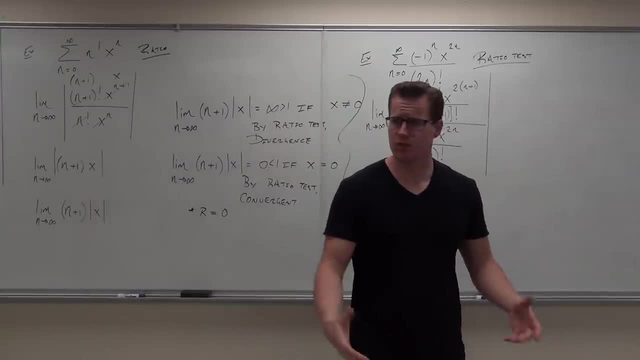 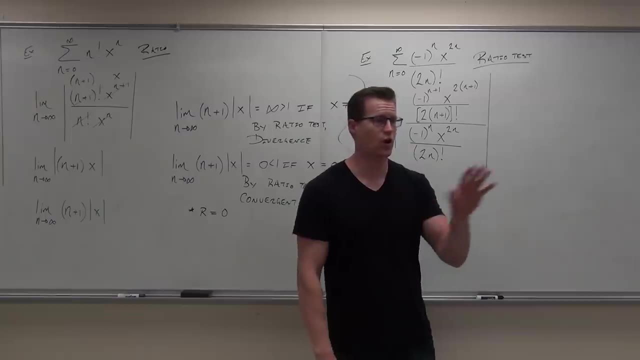 What would you do If you had this problem in the test which you're going to get something real similar to this? what would you do? Very good, Yeah. The absolute value is nice for a ratio test because the negative ones are gone. 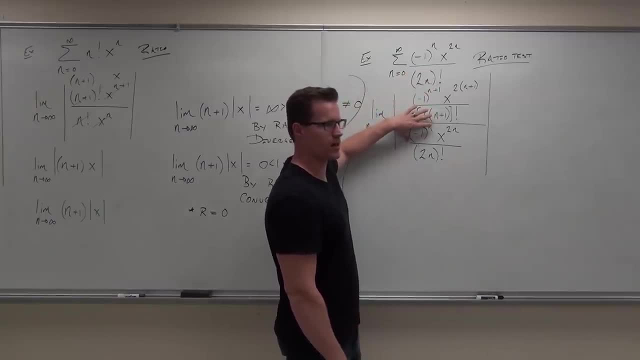 So this Gone, This, I don't care what it is, It's gone. It gone Because negative 1 to absolute. It's going to give you 1, no matter what it is Or 1. It's going to give you 1 anyway. 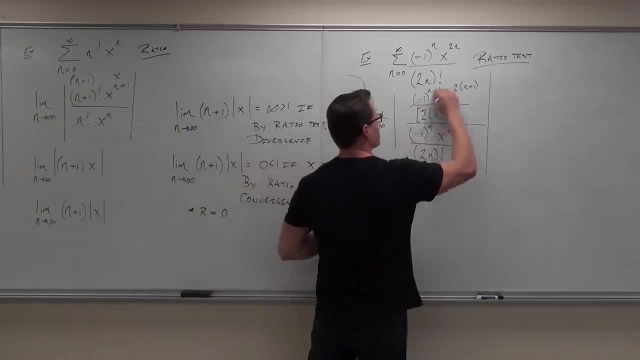 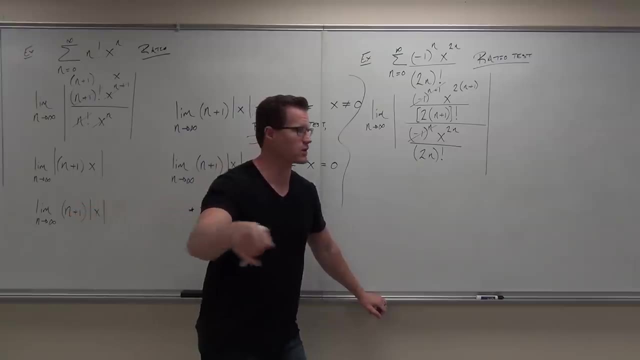 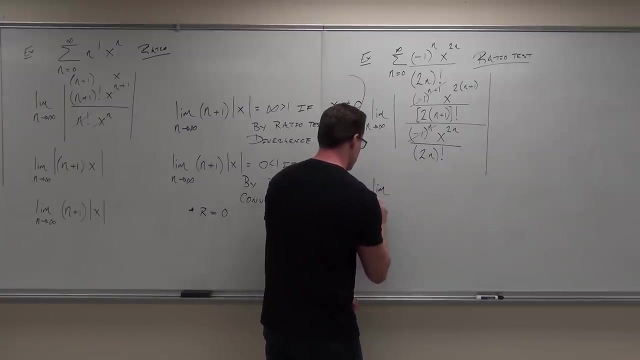 So these things, Those are gone. So in terms of absolute value that does not matter. What else would you do here, please? I'd multiply by the reciprocal changing division multiplication. Very good, Let's do that step. If you haven't done it already, go ahead and do it now. 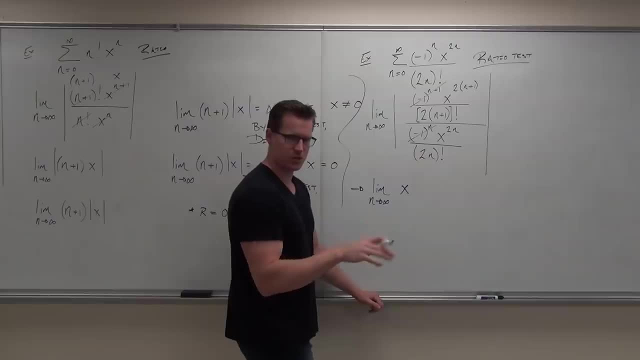 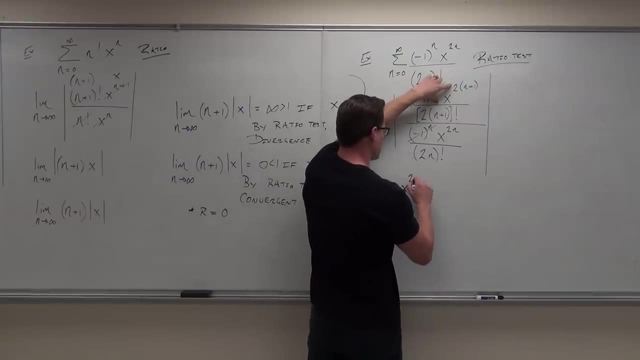 Also what I'm going to do at this point. you can do this too. I'm going to do my distribution. If you haven't done it already, this would be a good spot to do it. So here I'm going to get my x to the 2n plus 2 over my 2n plus 2, factorial times 2n. 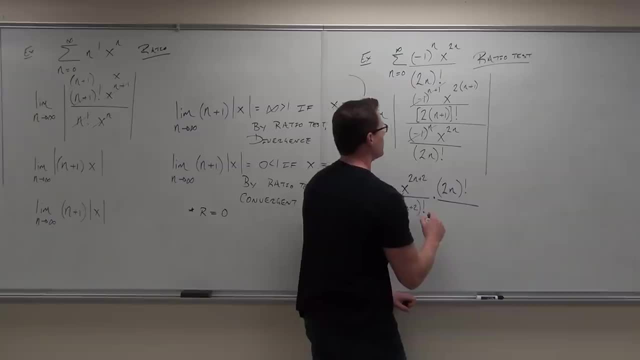 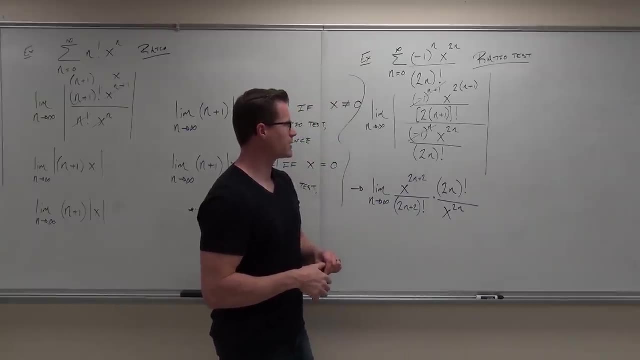 factorial. over x to the 2. Over x to the 2n. True or false? I can drop my absolute value from here to here. True or false, True, False, True, True, True, True, True, True. 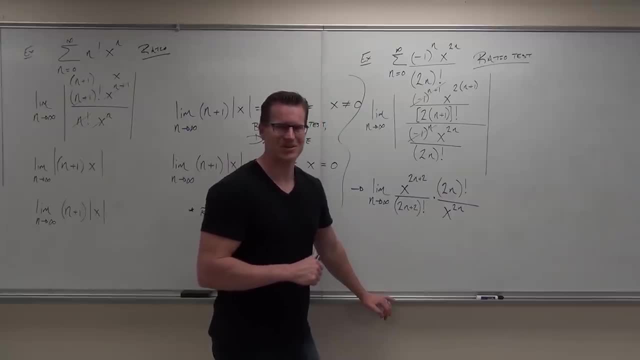 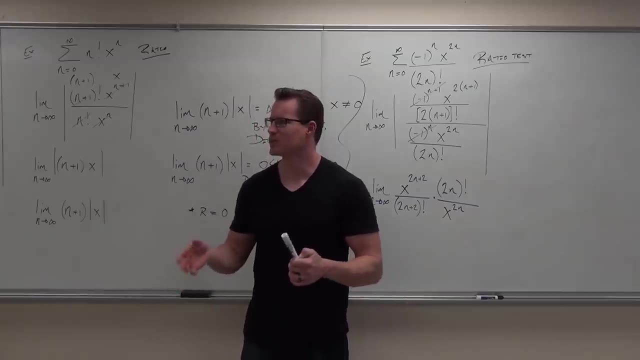 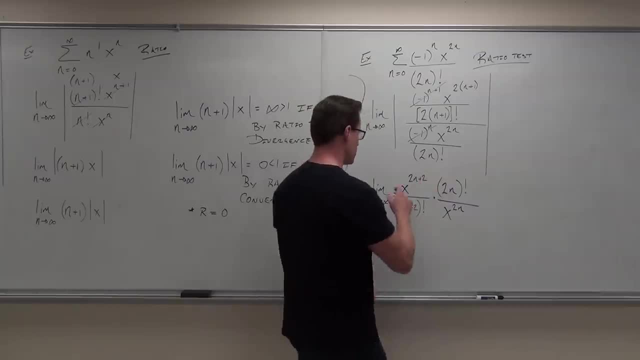 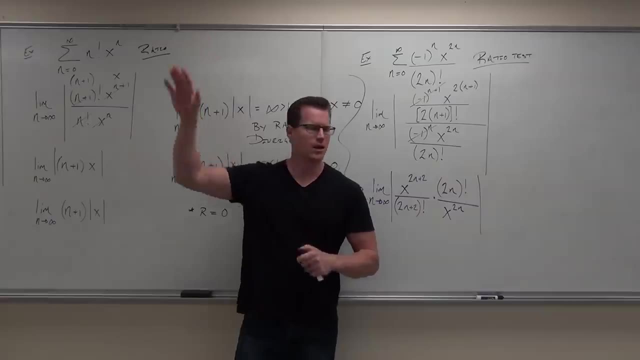 Do you see it? You could do it, You're just fine. I'm going to put them just in case. If you think you can make it that far, you'll be ok with it. Now, what would you do? Simplify. 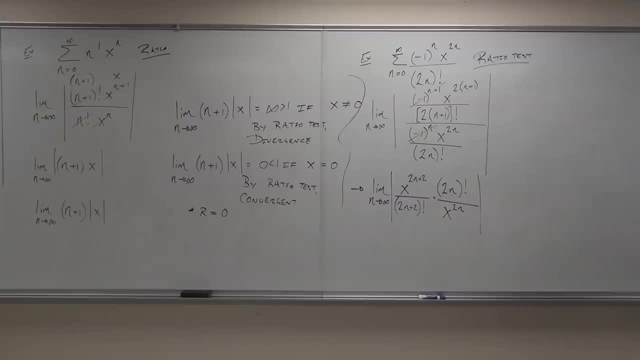 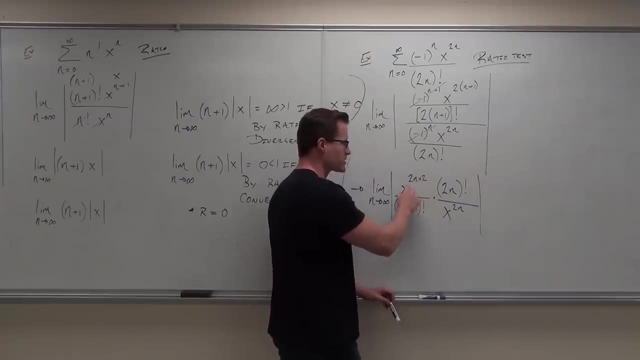 Simplify. Simplify as much as you can Now when we simplify this thing. this is something you're going to have to be pretty good at being able to simplify: x to the 2n, x to the 2n plus 2.. 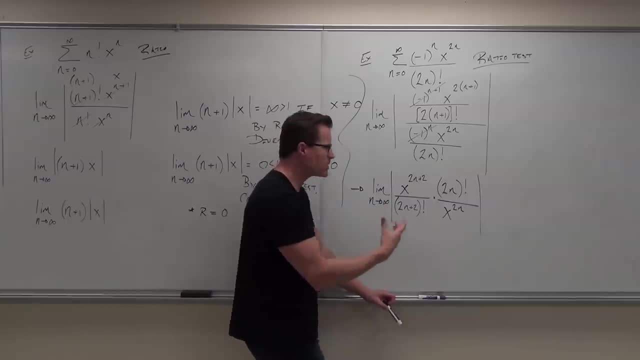 You've got to know what that plus 2 actually means here. okay, You've got to be good at simplifying: 2n factorial and 2n plus 2 factorial. You've got to know what this means. So I'm going to go through it one time with you. 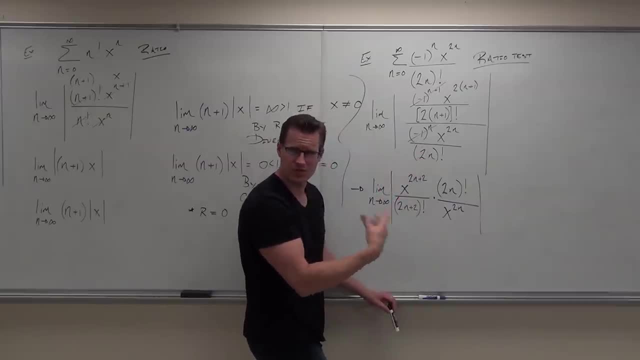 From here on out, I'm probably just going to kind of simplify on my own, because I'm going to expect that you understand this. Let's consider this first. This is the easier of the two. I'm going to write it over here and then I'm going to erase it. 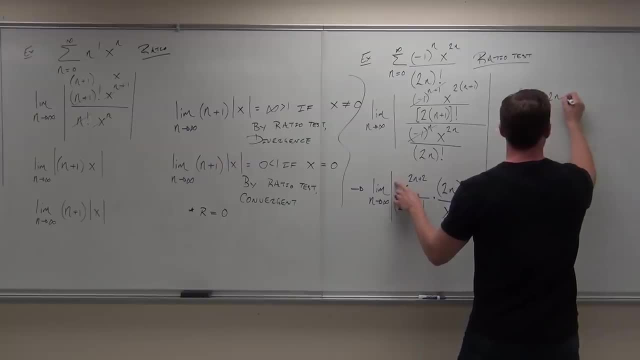 So if you're going to write it down, write it down quickly: X to the 2n plus 2, if I could even write it down, geez x to the 2n plus 2 over x to the 2n. 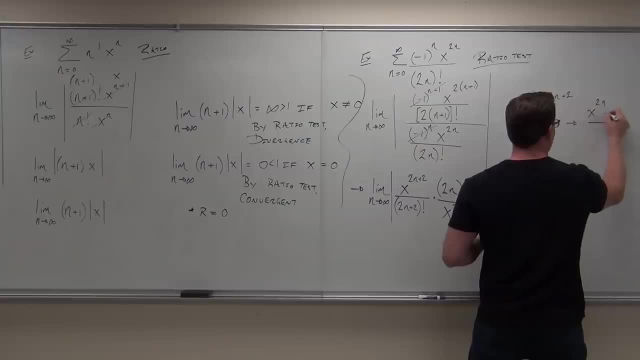 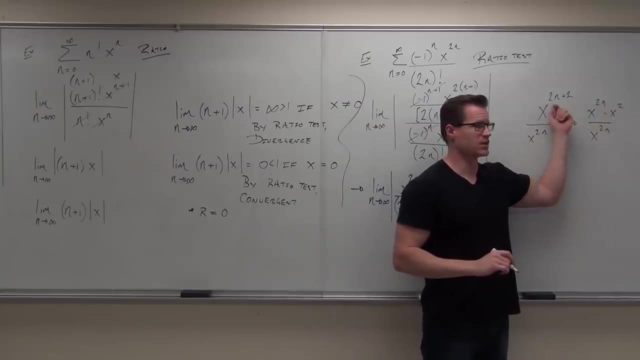 If you know what this is. this is x to the 2n times x squared over x to the 2n. When you multiply com bases, you add powers. therefore, I can split up any addition of powers by multiplication of com bases. 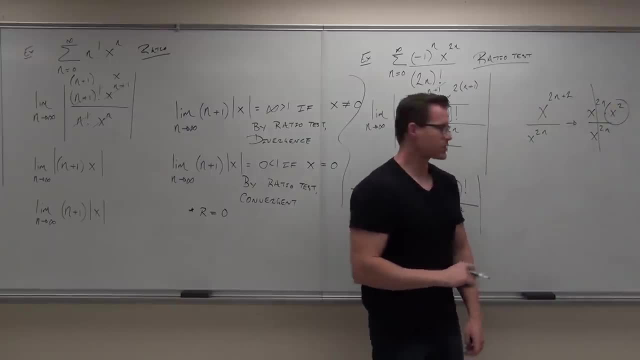 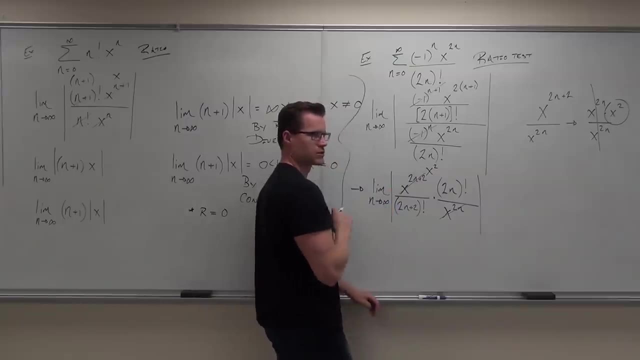 That therefore gives you x squared. Feel okay with that one. So when I do this, I'm going to go okay. well, boom, Boom, Boom, Boom x squared. So far, so good. Now this one's a little more tricky to think of. 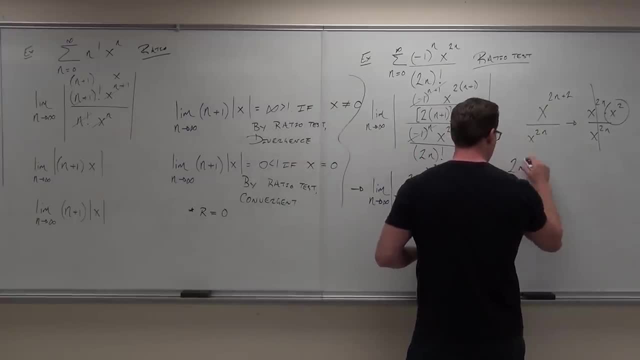 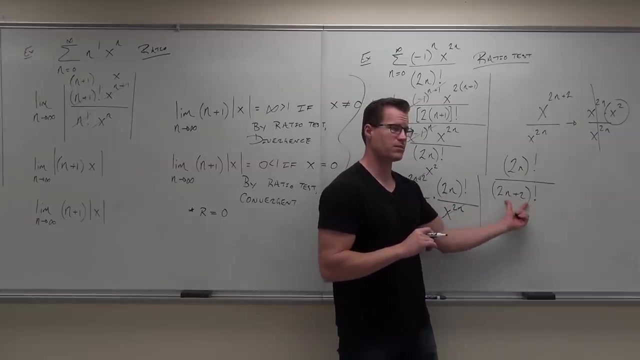 It's not hard. It's a little more tricky to think of 2n factorial over 2n plus 2 factorial. But think about what 2n plus 2 factorial would be. Do you understand that when you're doing factorials you take the first term and then you multiply? 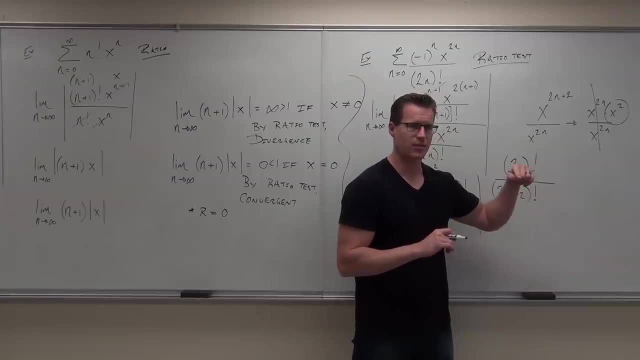 it by the term right below it. So basically you multiply it by x, the number 1 less than it. So if I had 5 factorial, it's 5 times 5 minus 1, times 5 minus 2, times 5 minus 3.. 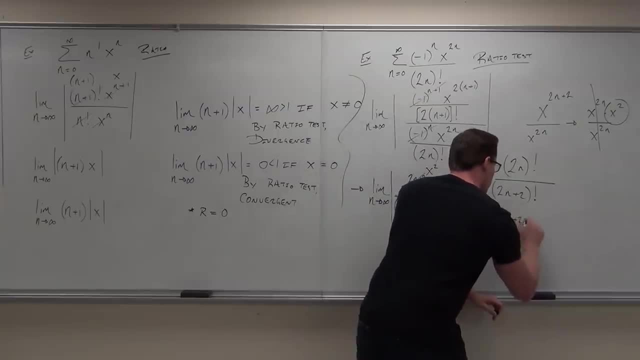 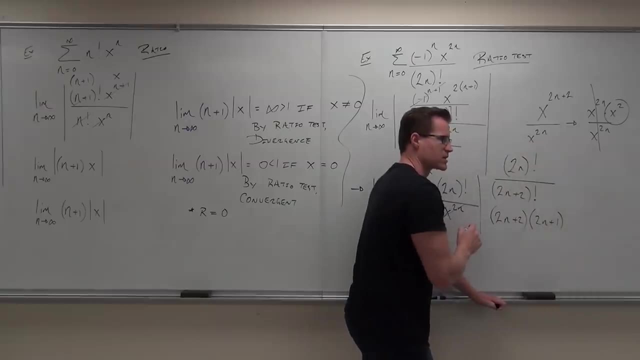 So this would be 2n plus 2.. That would be the first term. Does that make sense? Then I would have 2n plus aha. Does that make sense? Then I would have 2n and then I would have: oh, but wait a second. 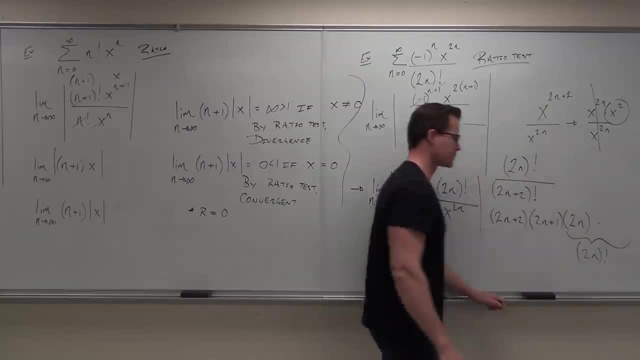 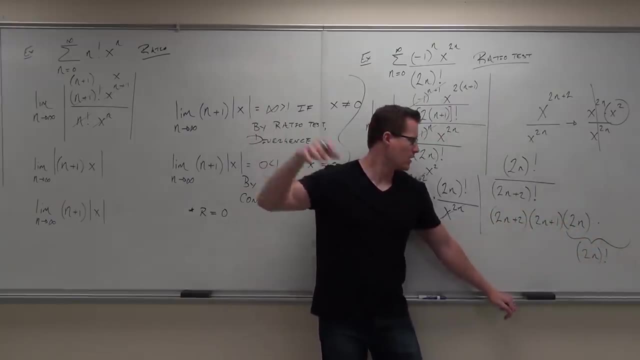 This is 2n factorial. All the rest of that stuff is 2n factorial. So if you understand that concept, We've used it before, but now we've never had a plus 2.. So let me assure you you can do. 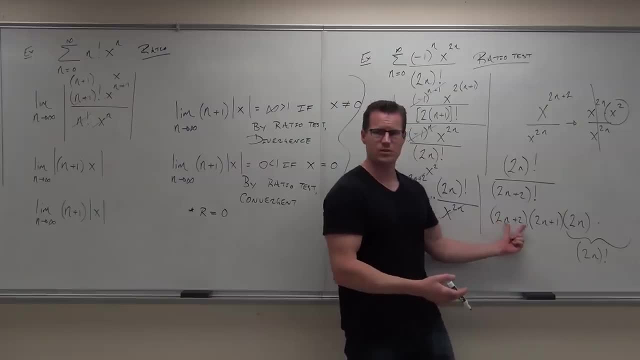 this with a plus anything. It just says 2n plus 2 times 2n plus 1 times 2n times 2n minus 1 times 2.. But that's this, That's exactly what this is. So basically, 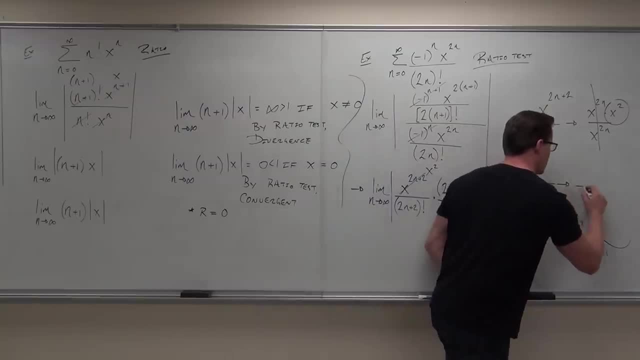 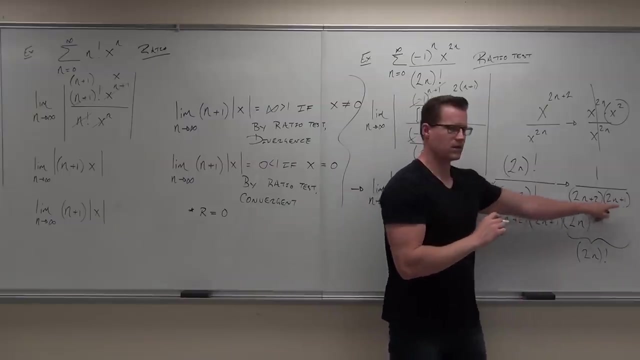 this gives you 1 over 2n plus 2 times what Times? what 2n plus 1.. And that's it. Are you with me on that one? That one's kind of tricky for people. I want to make sure that you're okay with that. 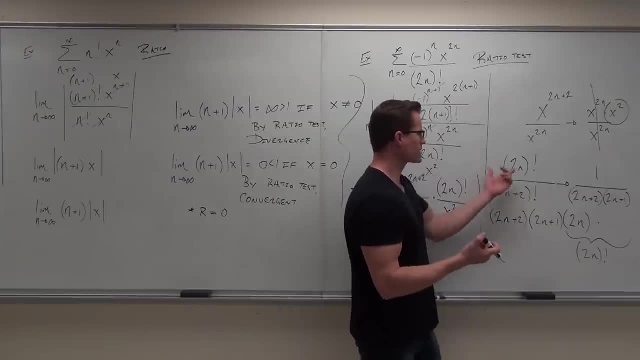 Are you sure? So when you simplify something like this, you go: okay, what's here, what's here? Well, this is 2n factorial. This thing right here is 2n factorial with a little extra, With two extra terms: The 2n plus 1.. 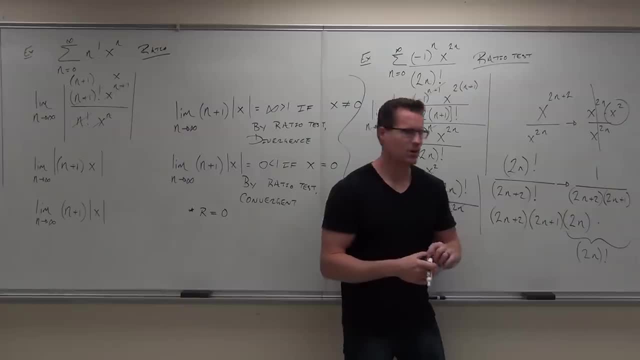 And the 2n plus 2.. And that's it For sure, you're okay with that one. Say what now You split it up. You split it up, You go. well, what is this thing really? It's really 2n plus 2. 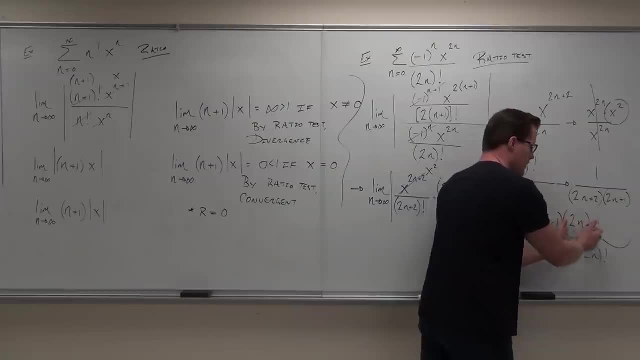 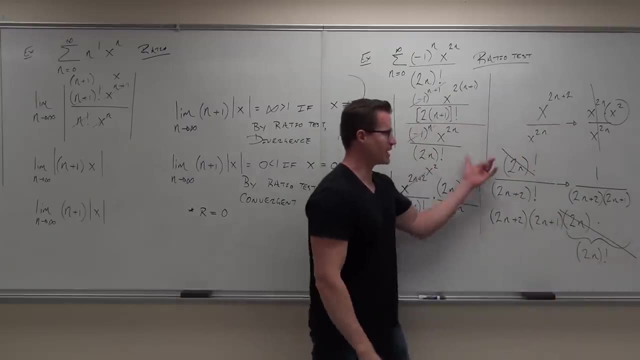 times 2n plus 1 times 2n. Oh, but this, the rest of this, is 2n factorial, So I can cross out all of this with this, And then I get 1 over 2n plus 2 times 2n. 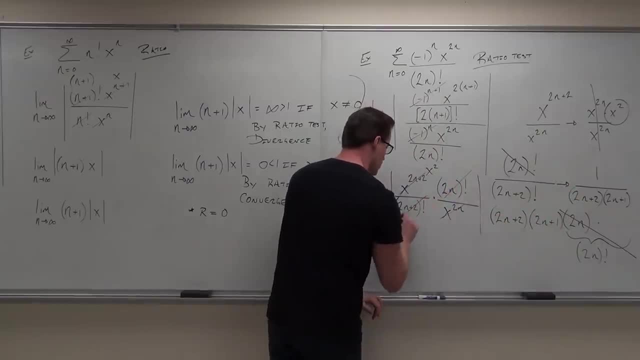 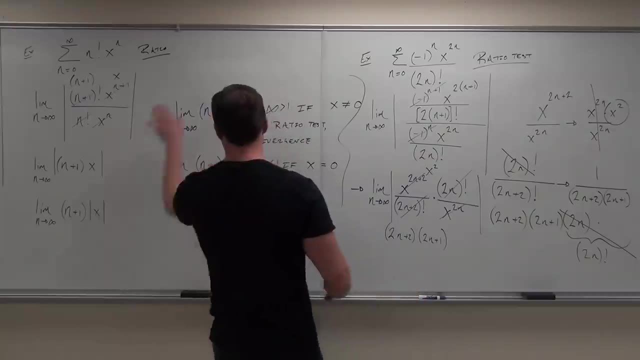 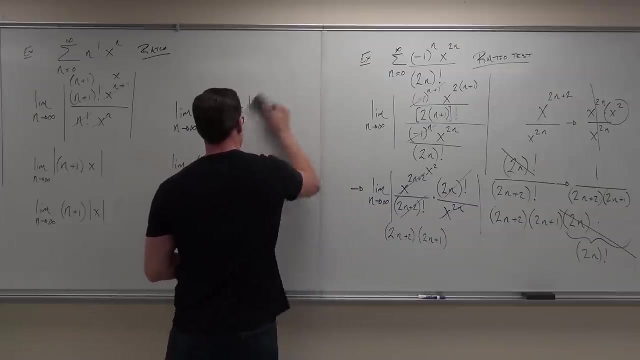 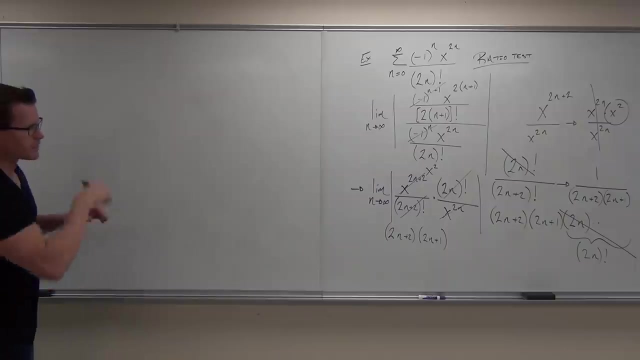 plus 1.. And that's what we're going to do here. Now I've got to move back over here, So let's see what we have left over. Can you tell me, Because I'm going to get lost over there. 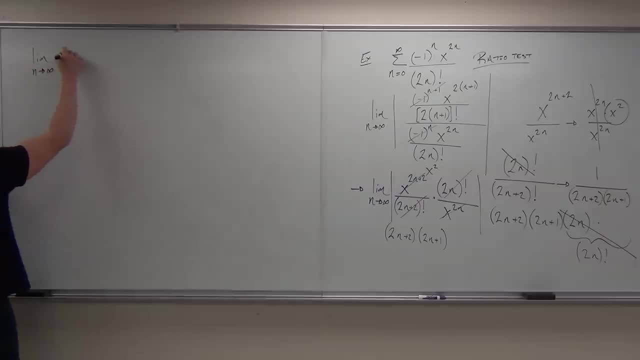 So what do we got X squared, X squared over 2n plus 2.. Uh-huh, 2n plus 1.. Okay, Absolute value. Sure, Do I need the absolute value anymore? No, For sure I don't. 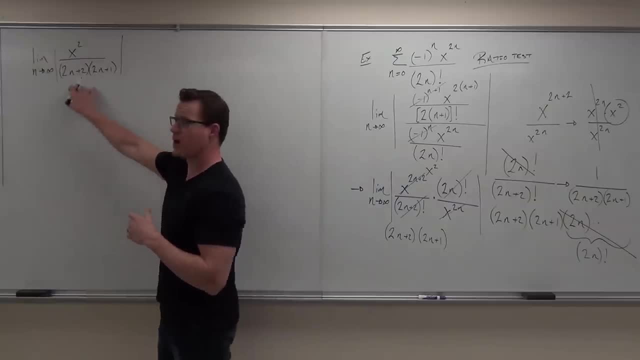 That's an X squared. There's no way it's going to be negative. This is both positive. There's no way that's going to be negative. So I can drop my absolute value right now, if you want to. Now, here's the deal. 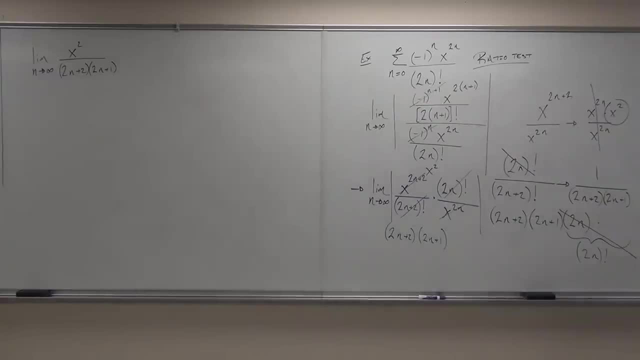 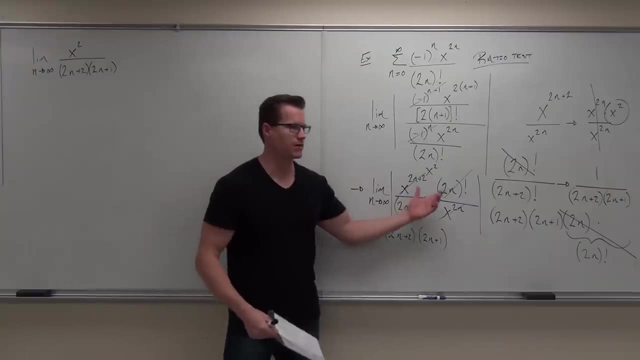 Here's the deal At this point. at this point, we're going to see what happens when we let our n go to infinity. We've already simplified everything we can right. If we go, let our n go to infinity, what are we going to get? 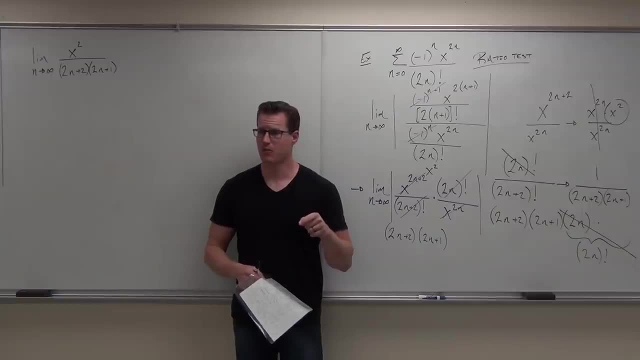 Now remember something about this: You're going to give me a number for X, right? So pick any number. I don't care what it is, but it's a finite number. Does that make sense? It's anything. Take any number and square it. 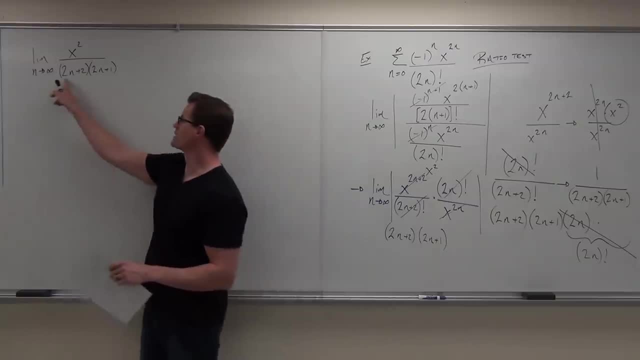 Do you understand? it's still a finite number. Now divide it by what this is going to be. What's this whole thing going to be? Infinity, Infinity. So what's this? What's this? divided by this: Zero, Zero. 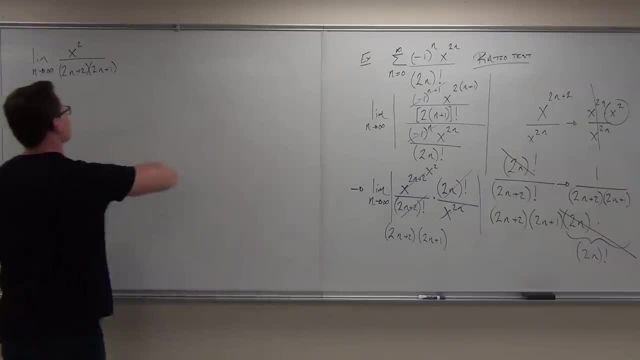 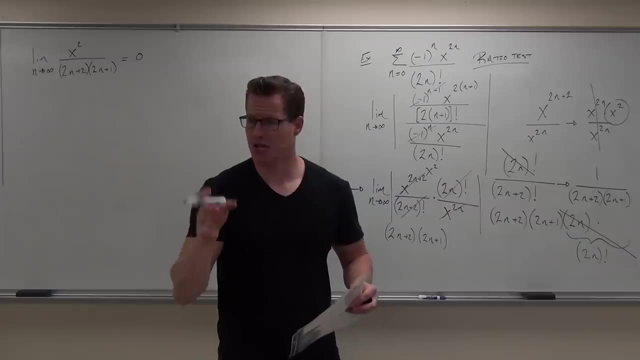 Zero. For no matter what X is right, Zero Equals zero. Do you understand why it's? for no matter what X is? Because X is not changing. as n is changing. N is going to infinity. X is not. X is not based on n. 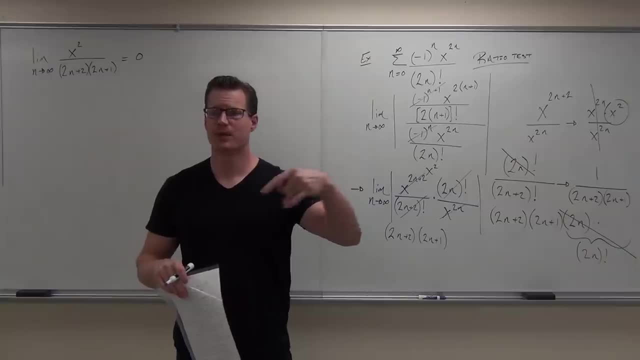 X is, X is this, X is. Pick a number, but it's one number. It's not going to be a variety of numbers. It is called a variable. I understand that, but you pick one number, You say X is. now, let's see about three-fourths. 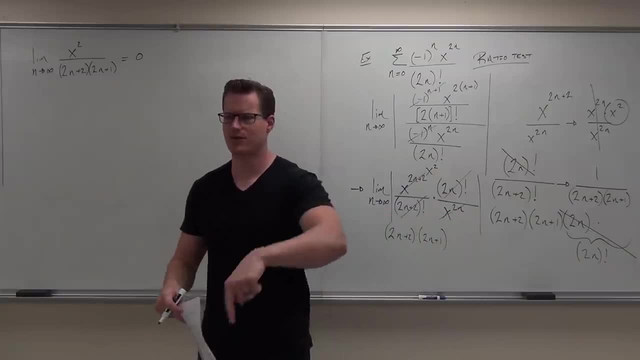 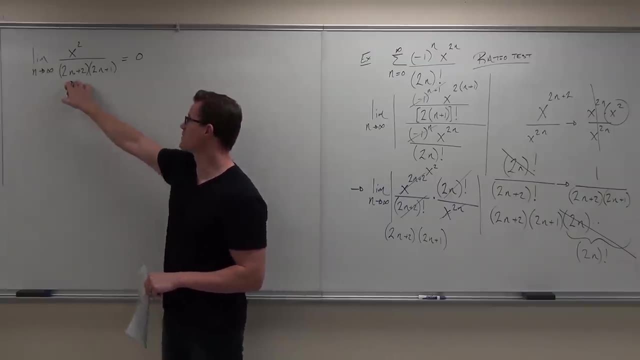 Okay, X is now one million. Okay, X is now negative five. Okay, But no matter what it is, you're going to stick with that number. You got it, Then you square it, You stick with that number, Then you divide it by something that's growing to infinity. 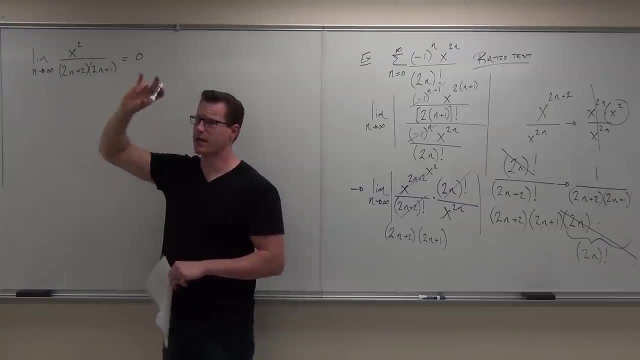 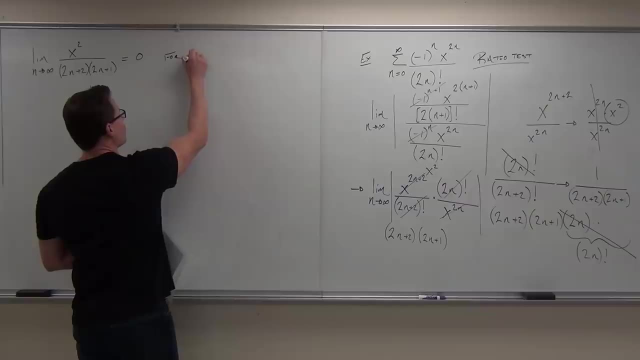 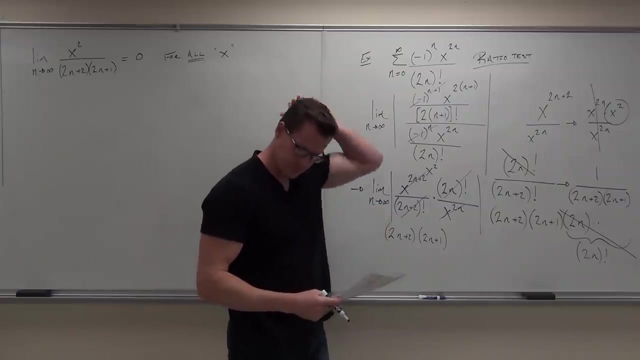 If you divide it by something that's growing to infinity, you have a finite number over infinity and that idea is zero, And this works for all X. Here's my question: If this works for all X, what that says is that: 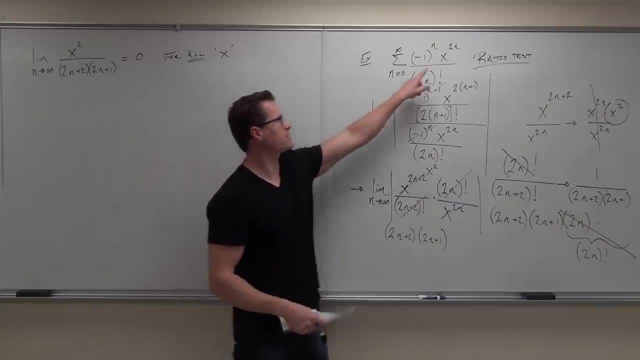 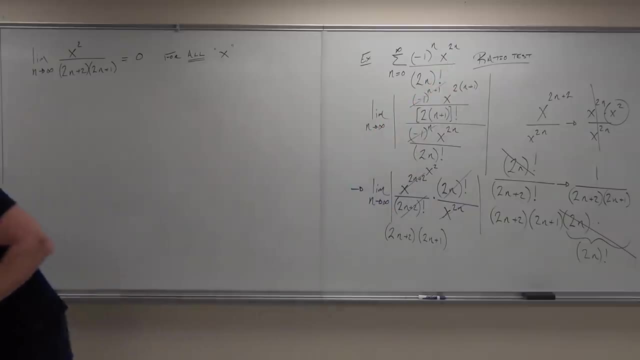 are you with me? Yes, Because I don't care what you plug in for X, this series will converge. Does that make sense to you? Yeah, Now how do I know that this thing's going to converge? How do I know that? 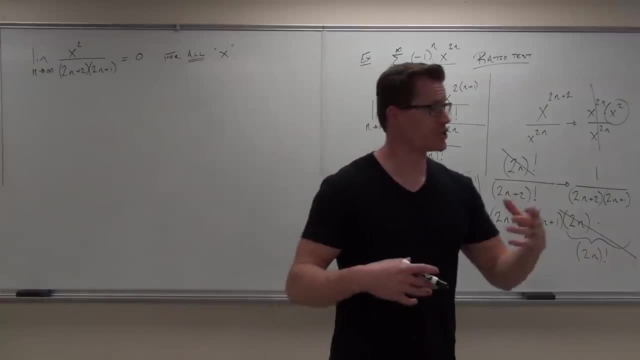 What test did we use? A ratio test And what answer did we get with a ratio test? Zero. And that is less than one, Less than one, Perfect. So we say this is less than one, so therefore it converges. 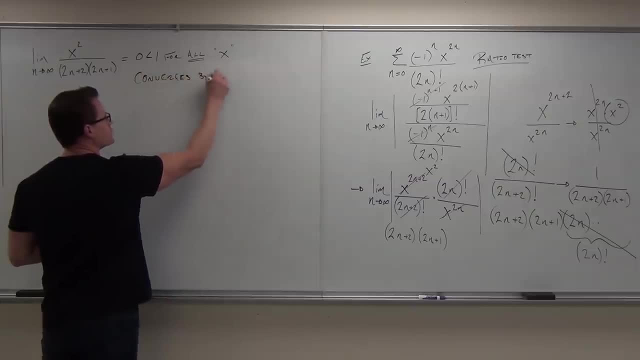 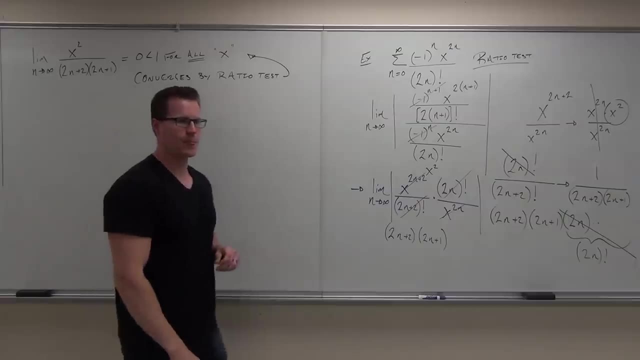 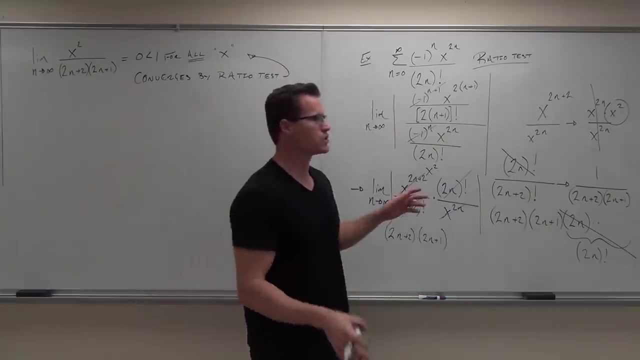 Yes, By the ratio test And what we've made. our determination is that this is for all X. Now, if you have something that converges for all X, what that means is that I don't care what you plug in to right here. 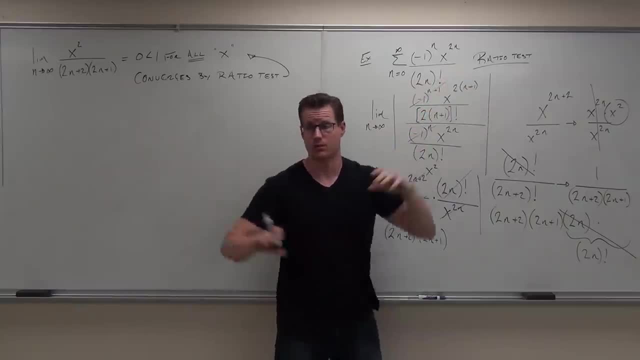 this power series will converge for anything. We've just proved it. Does that make sense to you? Does it matter what you plug in? Hey, guess what? It's going to be zero, Cool. Well, that means that we converge for all X. 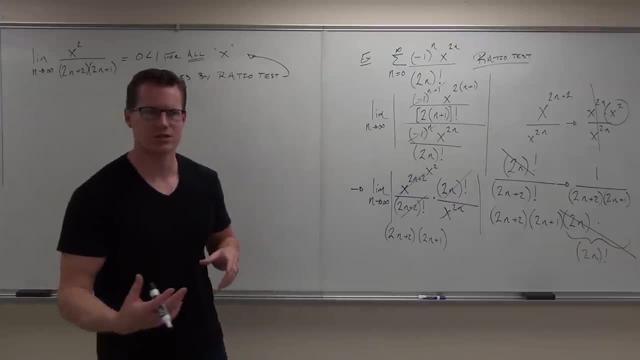 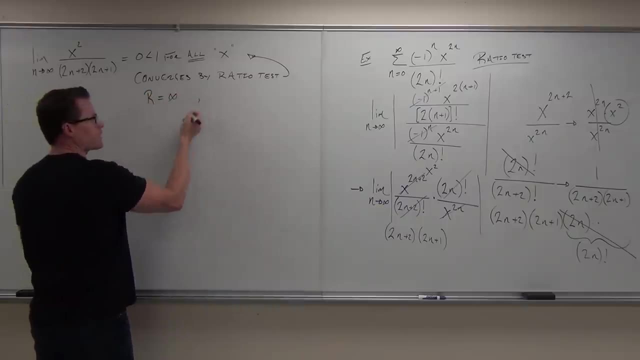 If we converge for all X, our radius of convergence says Infinity, Infinity. So the radius R would be infinity And our interval of convergence would be well, this is hopefully pretty common sense. It says: if you can plug in anything, right. 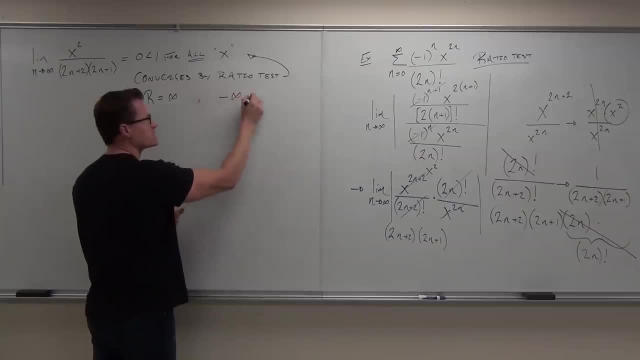 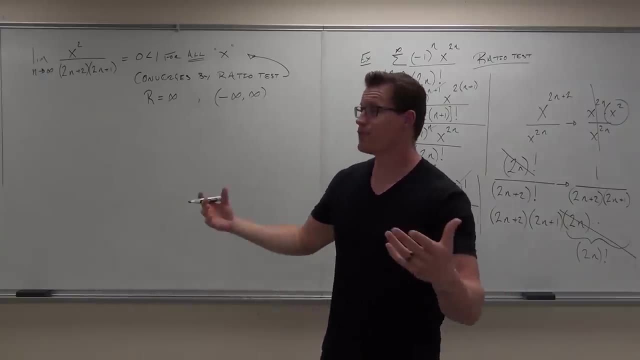 your radius is infinite. If you can plug in anything, our domain is negative: infinity to infinity. Remember that the domain is all X's that make our series converge. If we can plug in anything to make our power series converge, then our domain is infinite. 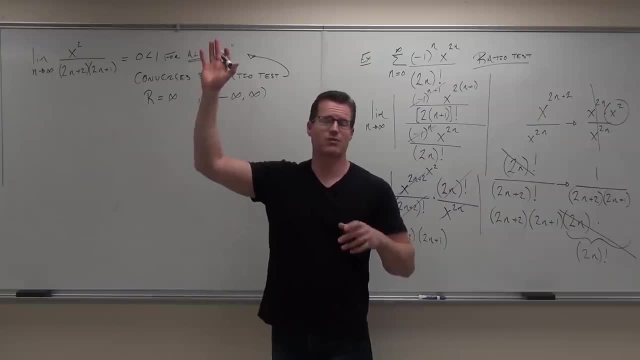 Negative infinity to infinity. So if you can just be okay with that, Okay, we've covered two out of three scenarios. We've covered one where we just converge at one number, just at the center, and that's it. The radius would be zero. 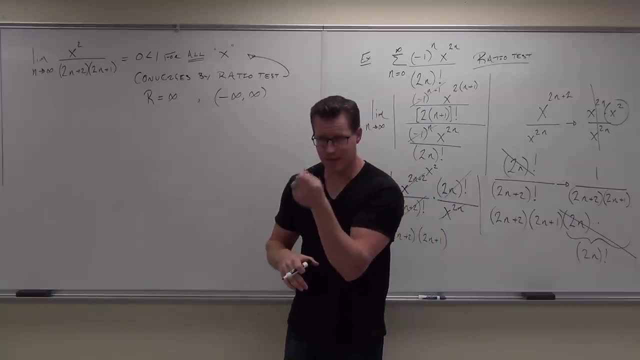 We've covered the next one, where we converge at any number, I don't care what it is. Our radius would be infinite and we'd have negative infinity to infinity. Let's talk about the third example question: If you can plug in infinity into X. 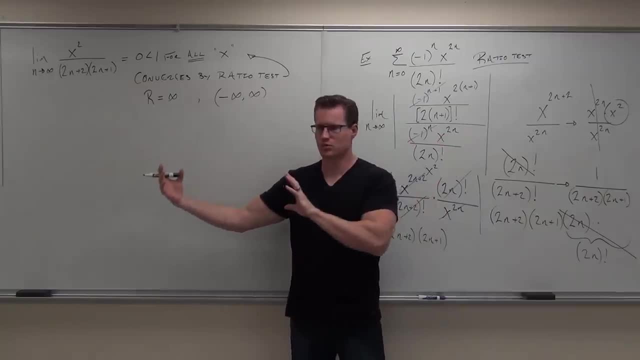 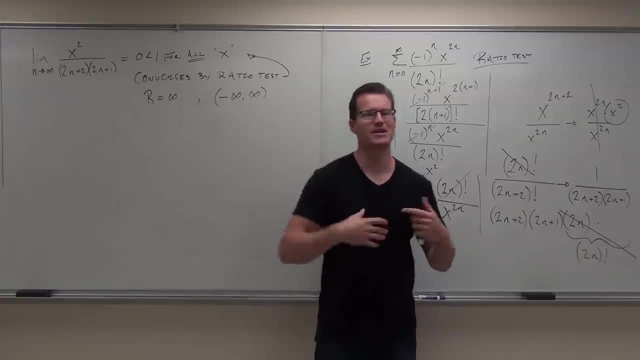 Well, you define X to be any number. right, But you can't say infinity for X, because that's not a number. We say: plug in anything Negative, infinity to infinity. of course you can't get to here. That's why we use our parentheses. 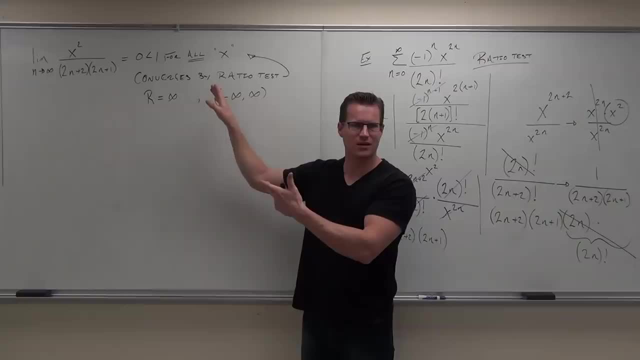 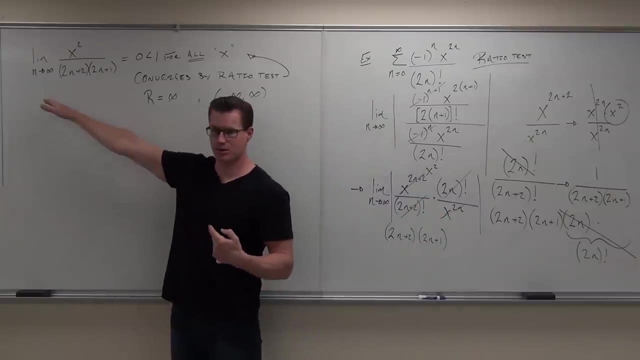 That's why on our interval notation you don't use a bracket, because the idea of going to infinity is a limit right Before we kind of accomplish that. X does not get to go to infinity. in this case, N is going to infinity in this case. 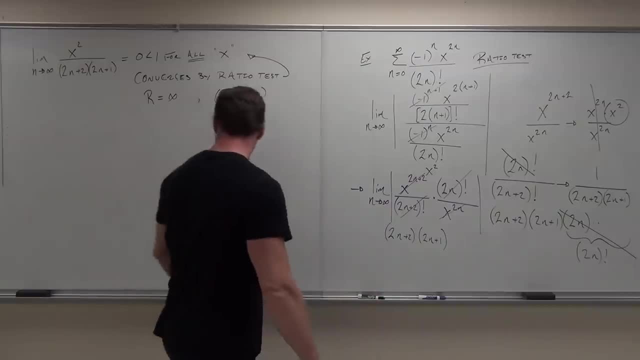 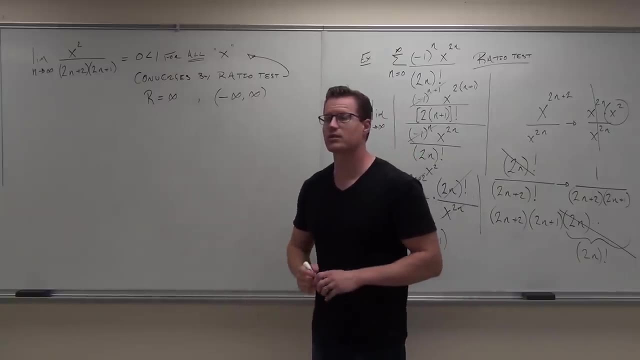 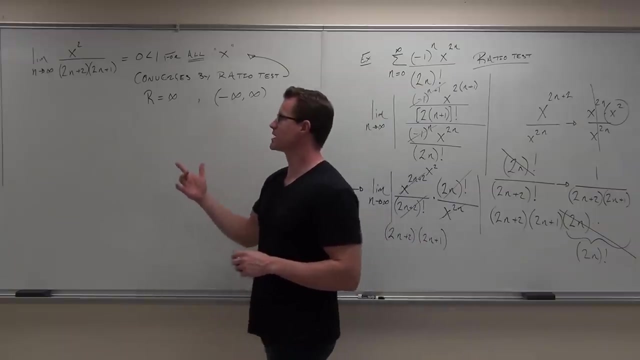 Does that make sense? Yeah, Yeah, Any other questions before we do our next example? We're going to do several more, but I want to make sure you're good with it. And infinity is different for n, because The idea of our limit here is saying that our n is growing. our terms are going to infinity. 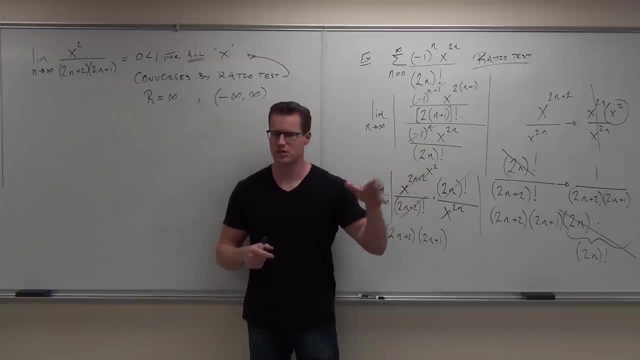 Our x doesn't change though. So once you start this, you pick an x, you stick with it. So it's first term, then first term times an x, then second term, times an x to the second. third term, times an x to the third. fourth term times an x to the fifth. 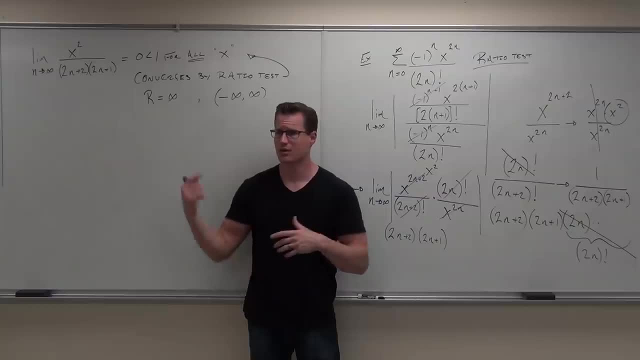 But the x doesn't change. The x is one number. So if we say, I don't care what number you pick, stick with it, the series is going to converge. That's what's going to happen here. No matter what x is, no matter what x is, that power series converges. 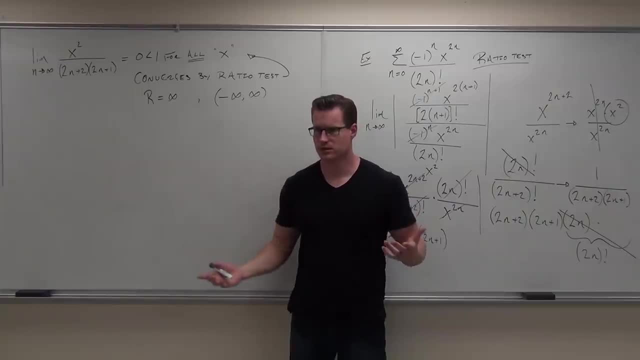 Therefore, this represents our function for all x. Are you sure you're with me? You want to do one more? Yeah, So the first example we had today, the one we just ended- a function represents that for only one value of x. 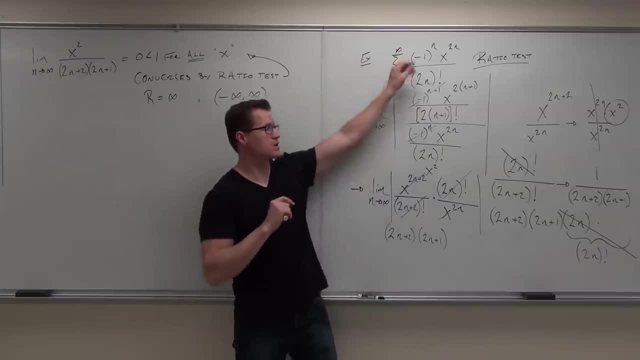 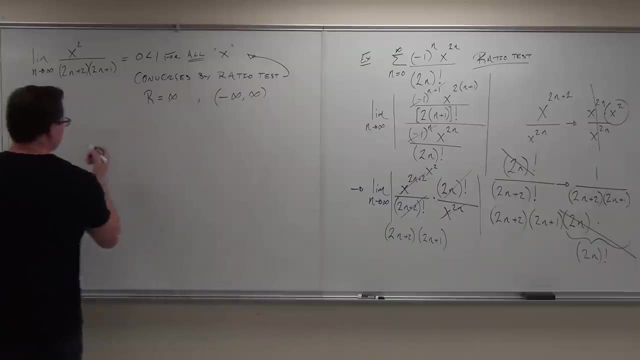 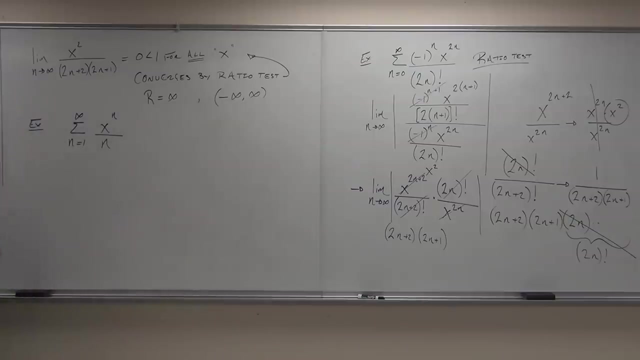 That value of x would be 0. A function represents this power series for any value of x. all the time It's going to converge for anything. Let's look at our third and final scenario, I suppose A seemingly harmless example. These are a little more fun though. 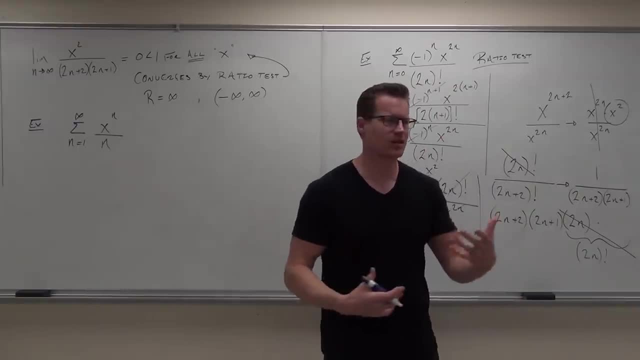 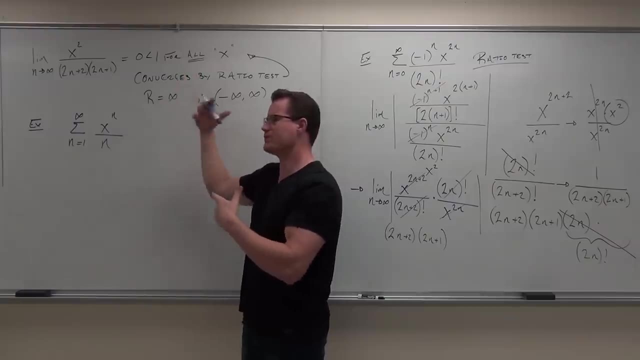 These are the ones that I like. The first one: well, it's always going to equal. well, the only time it equals 0 is if x is 0.. This one equals 0 all the time. It's less than 1 all the time for any value of x. 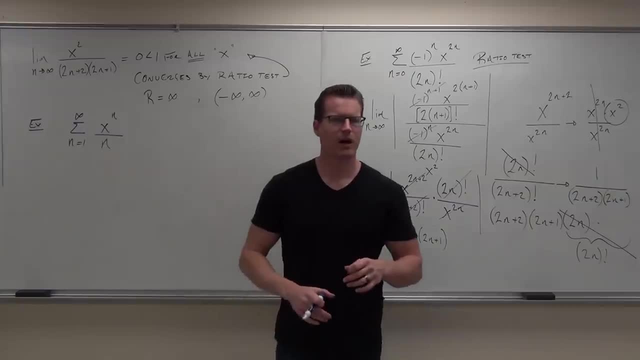 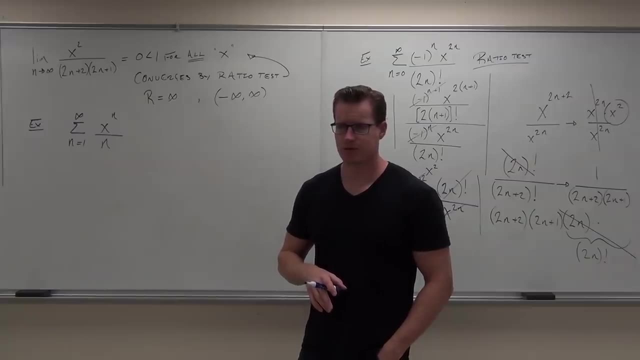 That's kind of boring. Let's look at this one. Let's look at what happens here. This thing, What type of series is that? Power Power series. That's right, It's a power series. So if it's a power series, 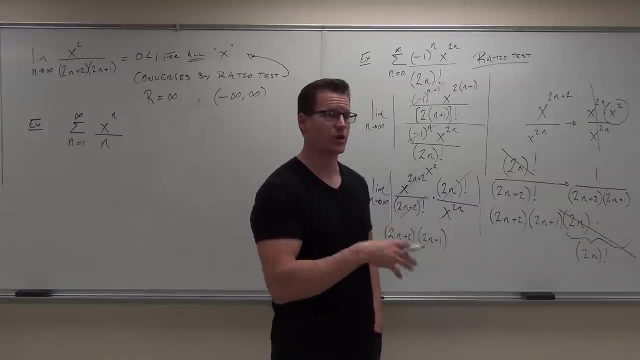 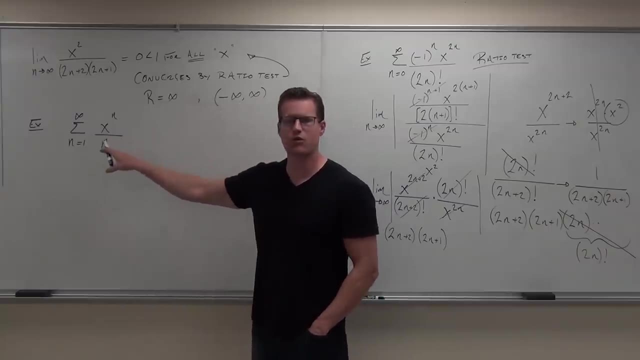 well, we need to find out where this series is going to be convergent. In the first example it was only at 0. In the second example it was anywhere In this example. we've got to discover where this thing is convergent. 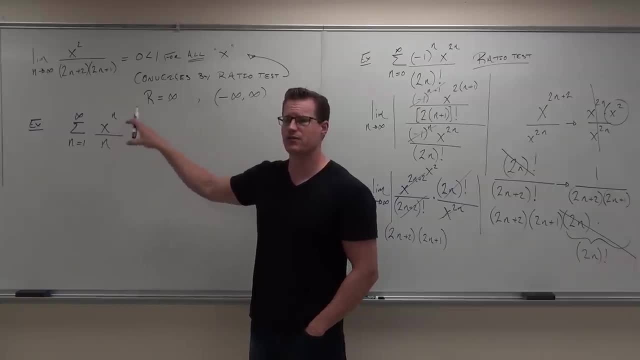 because only where our series converges is where we can define a function for it, Only on the domain. First example domain was: x equals 0.. Second example: domain is negative infinity to infinity. Third example: we're going to discover where that is. 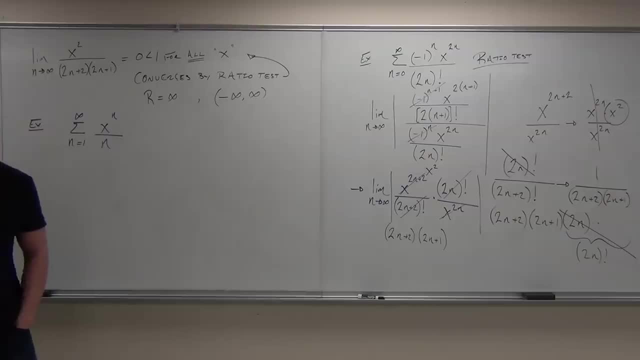 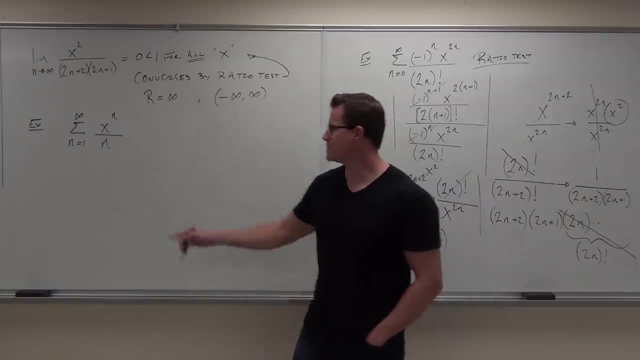 It's going to take us a little bit of time on this one. So what would you do first? Root test. You could maybe do the root test if you wanted to. I'm going to encourage you to stick with the ratio test. This is going to be a little hard to do, the root test. 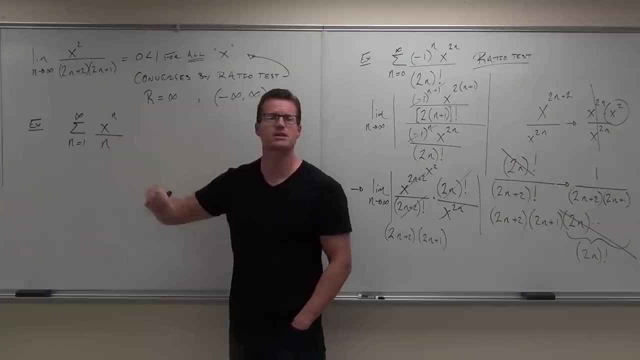 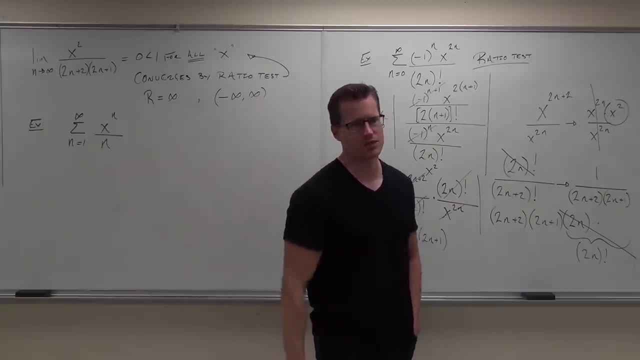 because you don't have a power of n there. So it would be a little difficult, So I'd probably stick with the ratio test. still, Ratio test works for powers of n as well, So try out the ratio test. Go ahead and set up the ratio test, if you would. 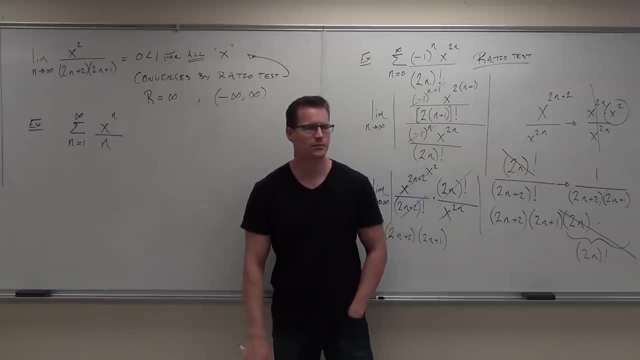 Question: You don't want to use the limit test because you don't know what x is. No, The ratio test right there, will give you where this converges and diverges, which is why it's so nice, right, Because it says: well, it tells you whether it converges or diverges. 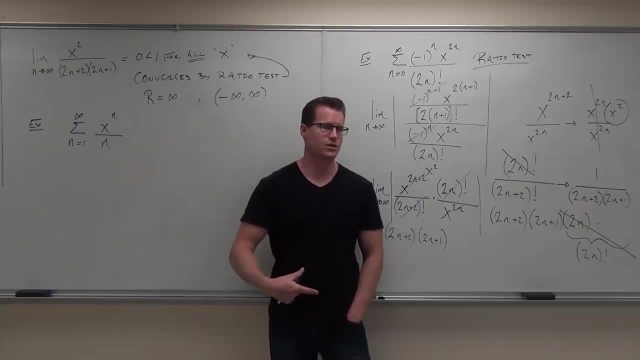 Therefore it will give you the interval here of convergence and divergence. So we can't do really like the divergence test. You wouldn't use that here. You'd use a ratio test to tell you where it's going to be convergent and where it's going to be divergent. OK, 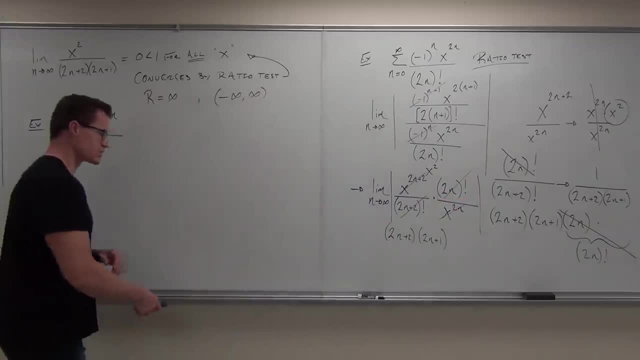 Now, after we do that, I'll show you when you can use something like the divergence test. OK, so we're going to use the ratio test and I'm hoping you're already working on it. Ratio test says that. Hey, do we need absolute value for a ratio test? 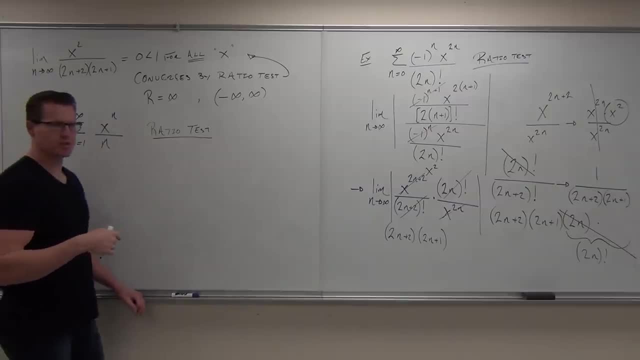 Yeah, Yeah, Because that n is changing. this is going to be, possibly, if you give me a negative x, a positive and a negative, you need the absolute value On the numerator. you need to have x to the n plus 1?. 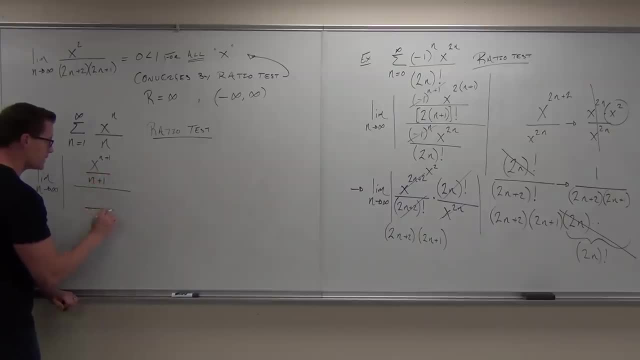 Over n plus 1.. That's right. And the denominator: you need to have x to the n over n. That's it And your absolute value. This one's going to be kind of nice. We have a limit. We have n approaches infinity. 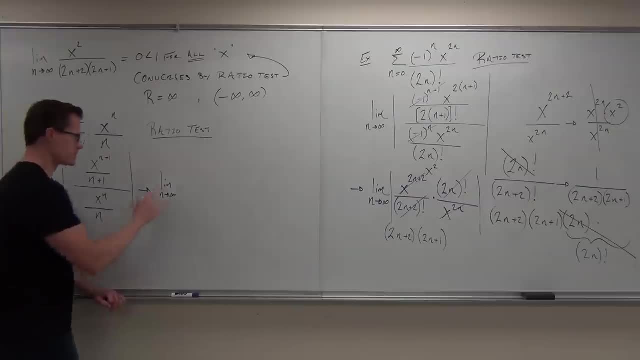 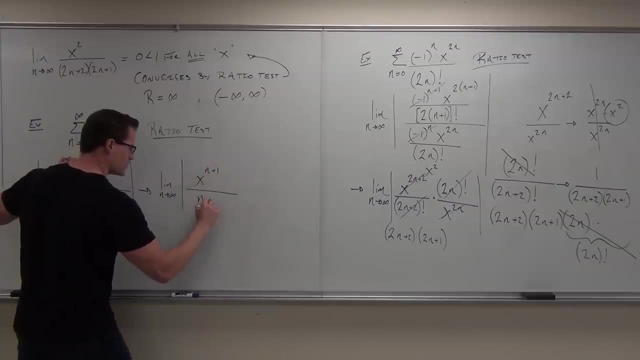 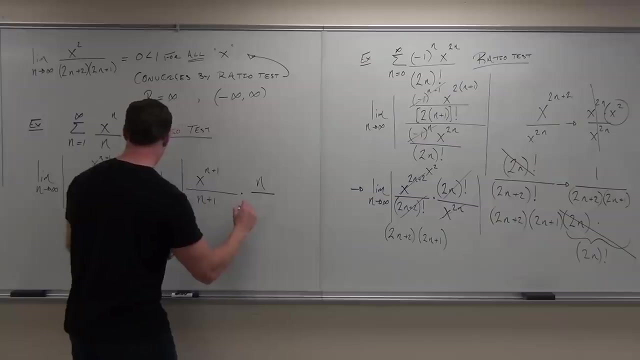 Are we still going to have our absolute value? Yes, Absolutely. Yeah, that's right, And we got x to the n plus 1 over n plus 1 times n over x to the n. Did I get that right? Yes, 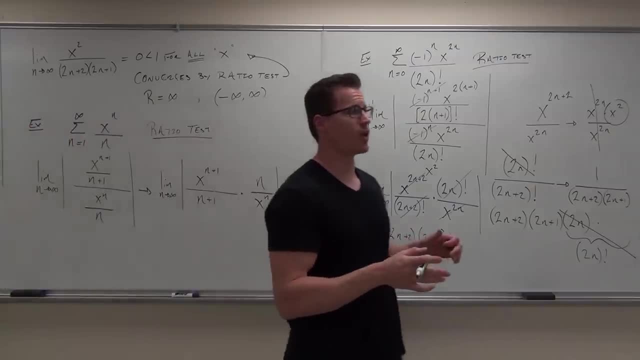 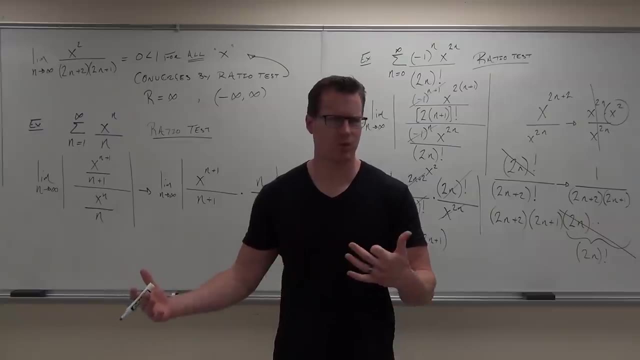 OK, What would you do now? Simplify as much as you can. Also collect your n terms and collect your x terms. You'll simplify. Simplify the x terms. OK, There's going to be only one x left. Collect your n terms. 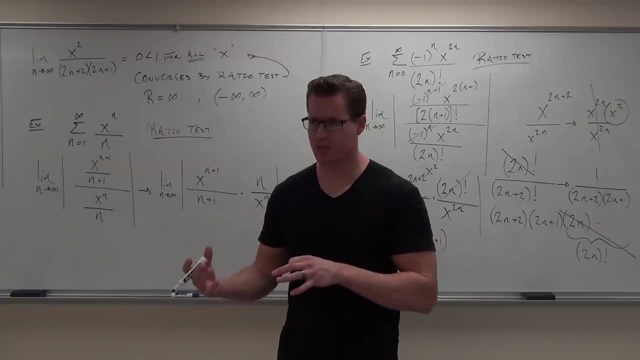 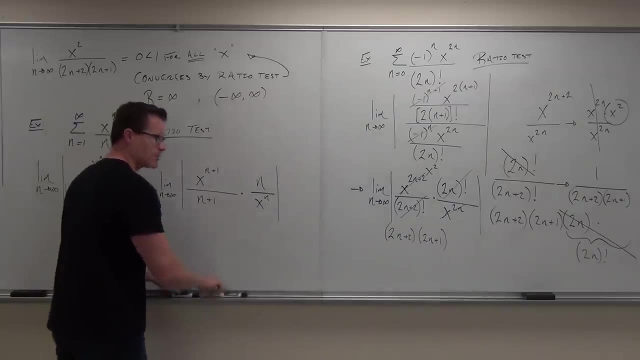 Pull those outside of your absolute value, because they're always positive anyway. Does that make sense to you? So what I mean by this is, well, simplify what you can, but don't do stupid things, Don't go. oh well, n and n. 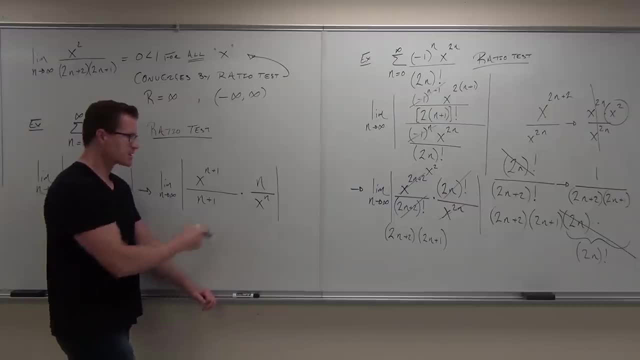 Cross out. I'm done. Don't do that. Don't do that. Simplify this Sure: x to the n, x to the n, plus 1 gives you one extra x. That's what the plus 1 is. It's an x to the first power. 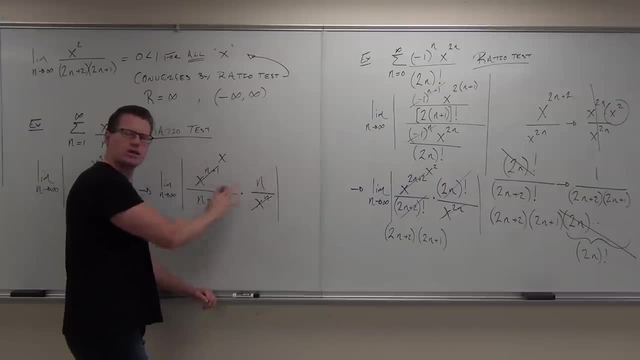 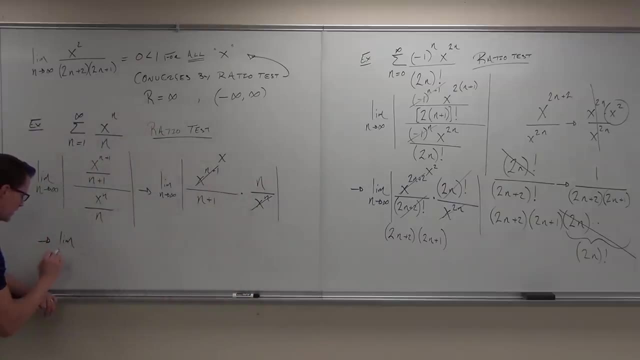 This you don't simplify right now, This you're going to do a limit with in just a minute. What I mean is: collect this, Collect it and say OK, well, that means that we've got a limit, as n approaches infinity, of n over n plus 1 times x. 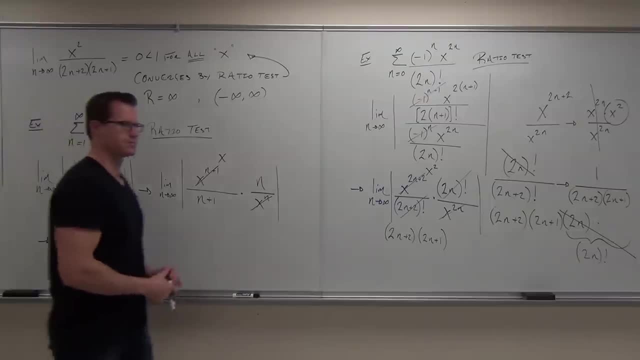 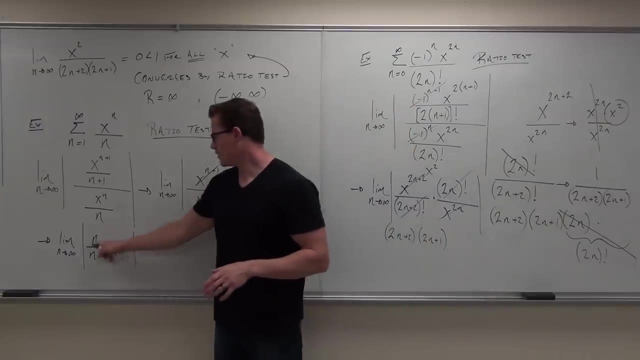 in absolute value. Are you still OK with that? Yeah, You sure. Yeah, Now is n over n plus 1 always positive? Yes, Because n's growing from 1 to infinity? Yes, it is. Is x always positive? 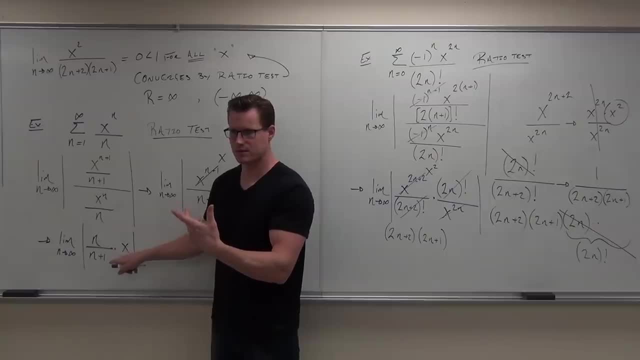 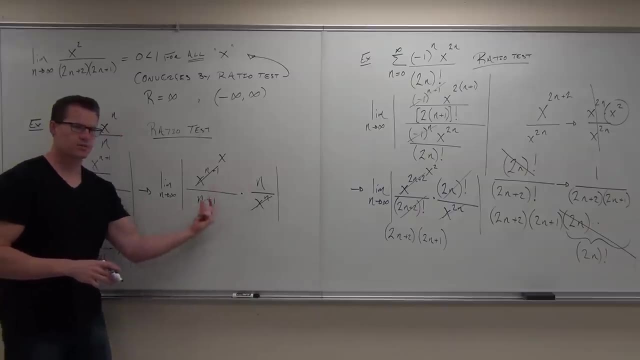 Yeah, No, We can't make that jump. I know what x is, Oh. So what I can do is what I've been telling you: Collect your n terms, Pull your n terms out of your absolute value, if they're all positive. 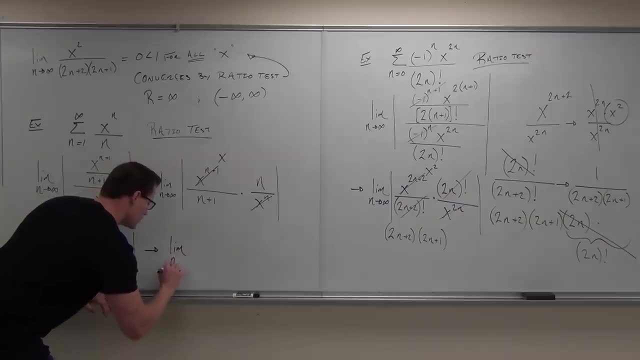 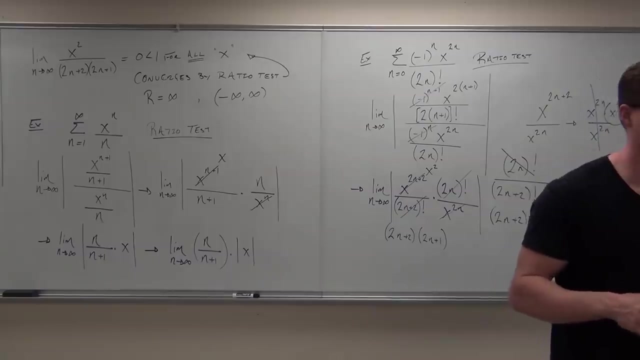 They generally will be. So we're going to have n over n plus 1 times the absolute value of x. Now, this is why I like these. It's a lot more interesting. You've got to do a little bit more work with it. 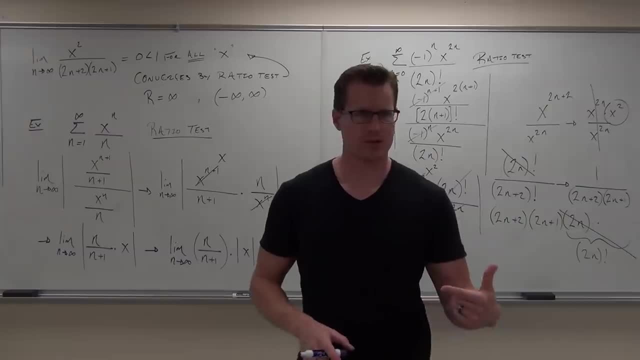 Is it super hard? No, it's not super hard, But you get to do a little more work with it, So please pay attention, This is how you do the rest of them. The first two are kind of our basic ones, OK. 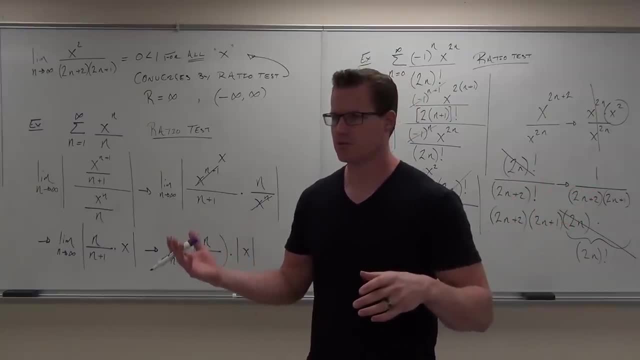 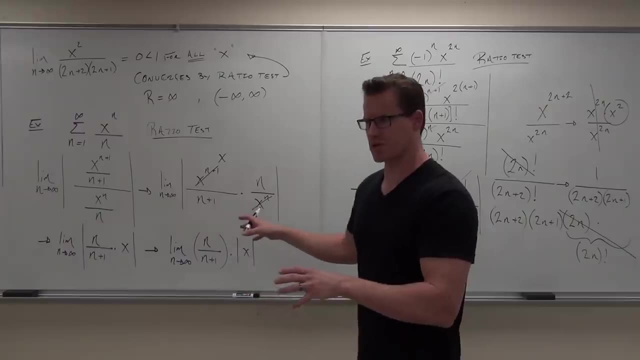 x is 0,, only for 0,. no radius. x is infinity. radius infinity, I'm sorry. x is 0 for all. x, Therefore radius infinity, no problem. This is more interesting. You limit as n approaches infinity of n over n plus 1.. 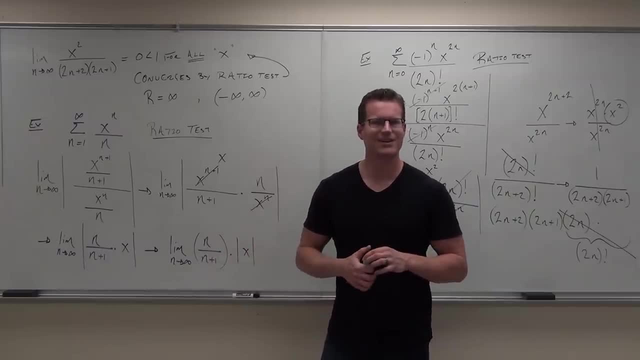 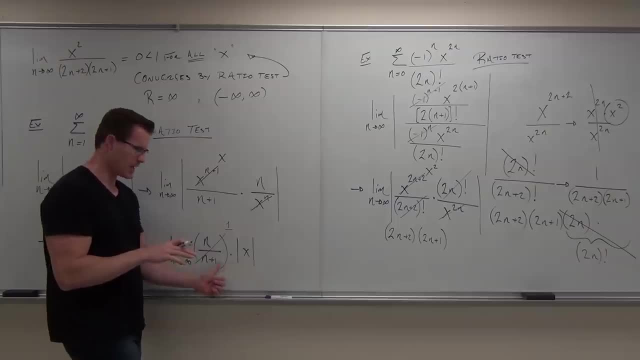 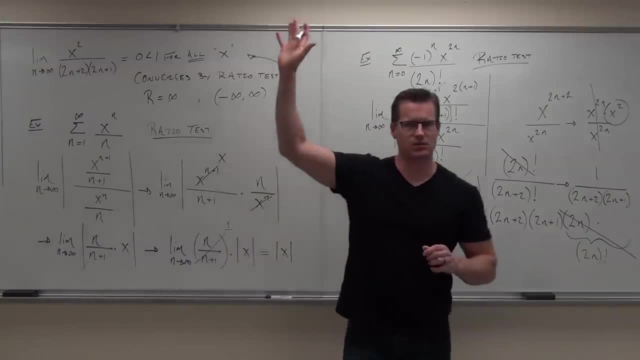 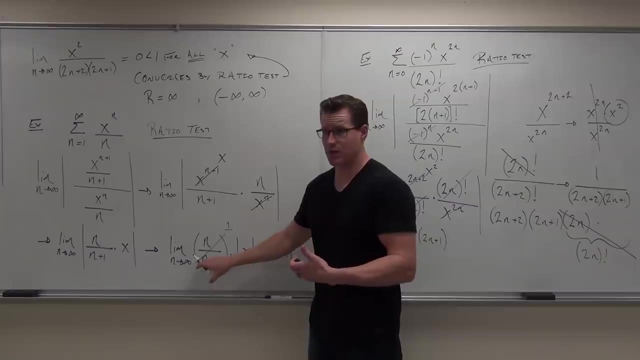 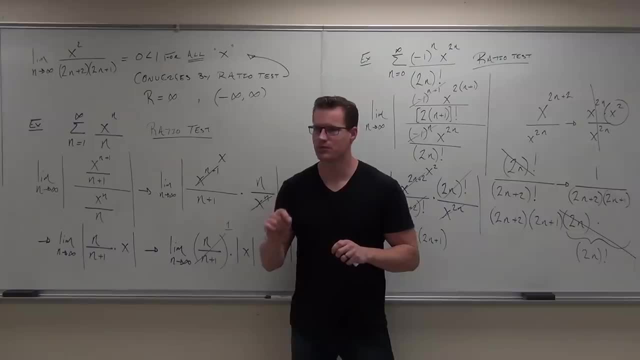 1. 1. 1. 1.. This is the whole deal. so if you get this, you're gonna get the whole thing. okay, The ratio test tells you when you're gonna be convergent. When does the ratio test tell you? 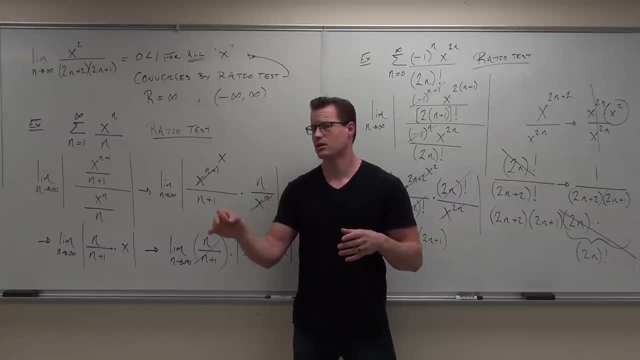 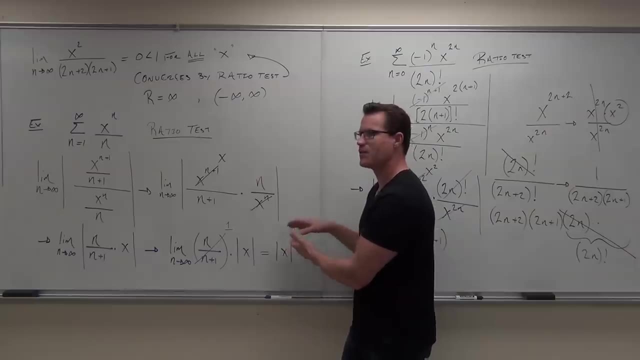 that your power series is going to be convergent. When the limit is less than what? When what's less than one? This, not x, the absolute value of x. So did you guys catch that We're using the ratio test, right? 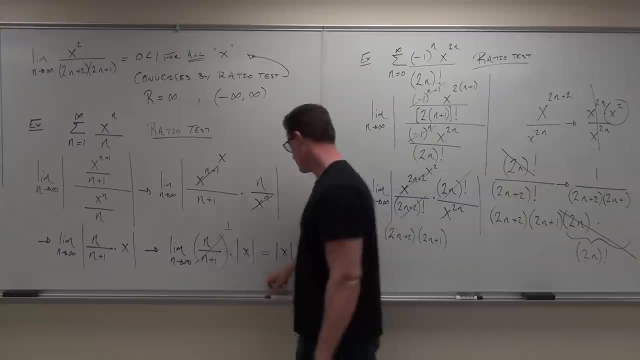 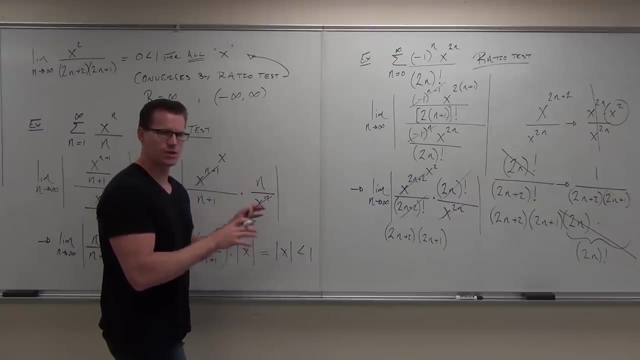 Ratio test says they go through all this crap and, at the very end, if this thing is less than one, then you will have a convergent series or you'll have a convergent power series. in this case, The reason why this is here, why the less than one is here, 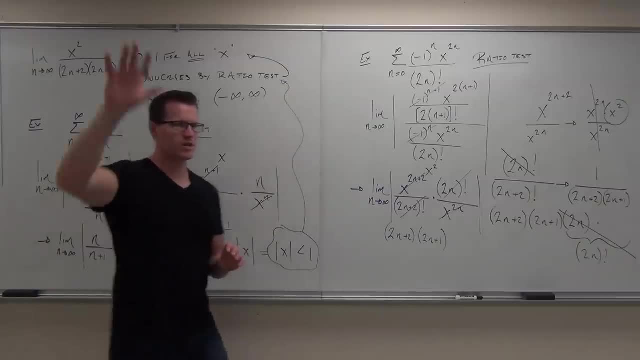 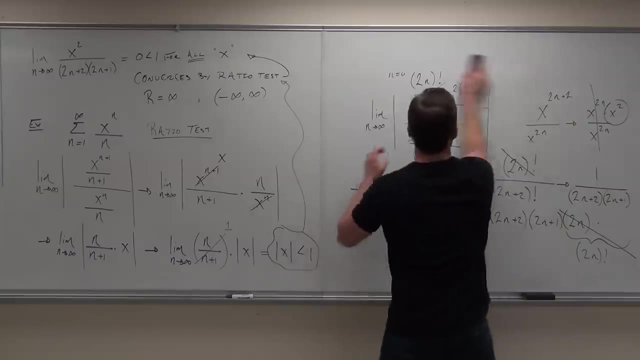 is because we just used the ratio test Show of hands. if that made sense to you, That's why we're doing it, folks. Now this is kinda cool. It's just very cool. Give me a specific value of x that you could plug in. 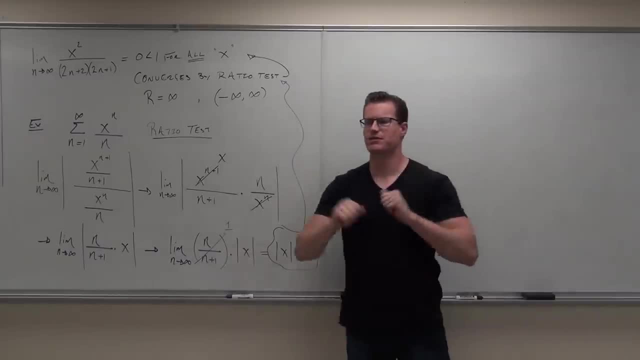 that you know that this series is gonna converge, for Give me a specific value. One-half would be great, Zero would be fantastic. What else Negative? one-half? How about two? No, Because that's bigger than one. How about one itself? 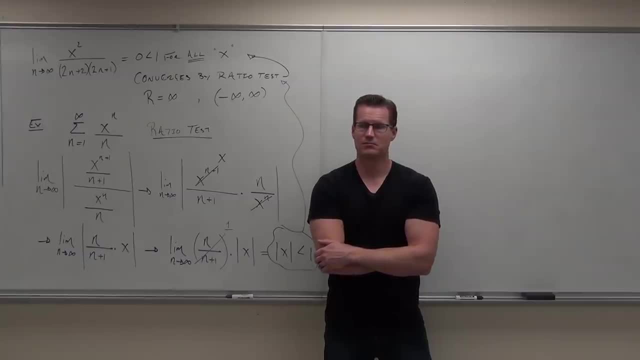 How about negative one itself? No, Yes, No, no, I don't know. I don't know. The ratio test does not tell you. So here's what we need to do. Here's what we know so far. Did you guys catch the whole idea about? 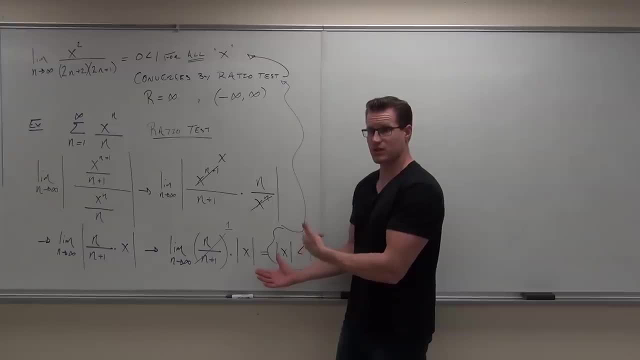 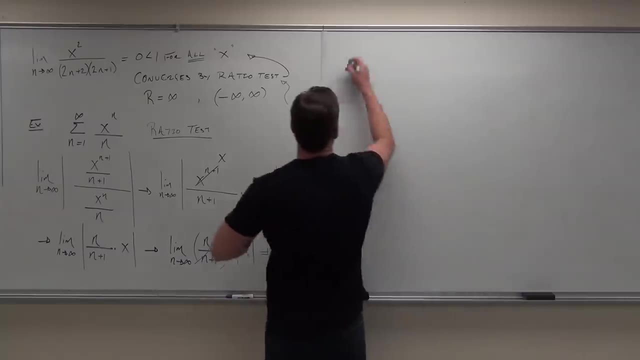 if you have a value between negative one and one Between- not inclusive, but in between, You will for sure have a conversion power series. Then here's what we know already Because of this case, because absolute value of x has to be less than one by the ratio test. 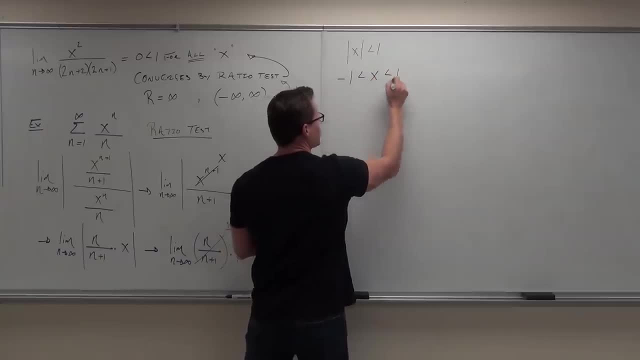 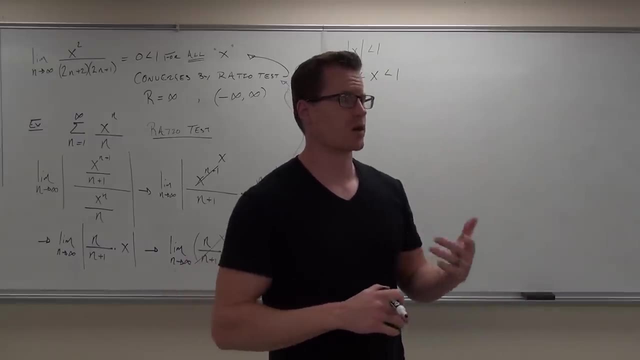 we know that negative one is less than x, which is less than one. We know x basically has to be between negative one and one. Now let me tell you something Right. here is where you find your radius of convergence. It's really easy to do. 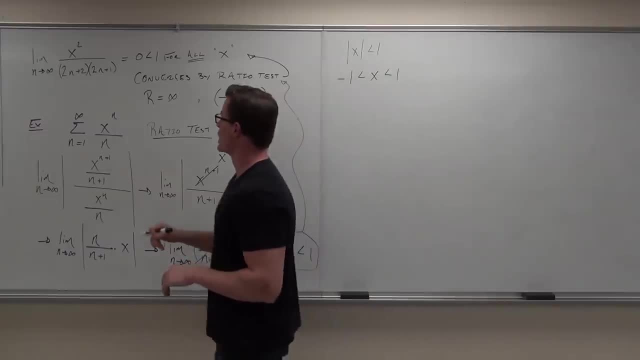 Please listen carefully. What you should find your radius of convergence is whatever is being raised to the nth power, x in this case. if it was x minus one to the nth, you'd look for x minus one. That's looking really nasty, I know. 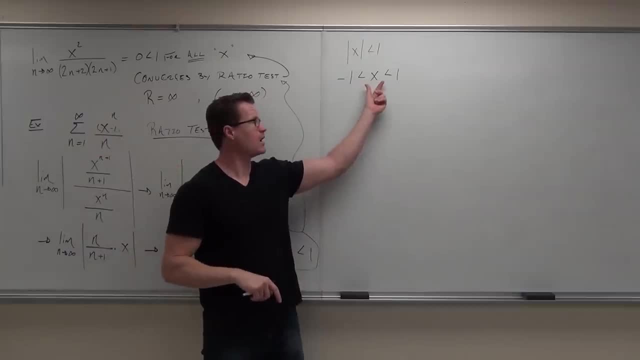 but if you had x minus one in there, you'd look for x minus one here, and whatever that number is, that is what your radius of convergence is. So in our case, your radius of convergence is One. What number is this? 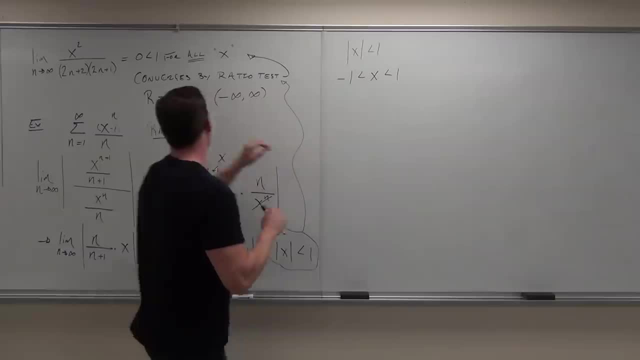 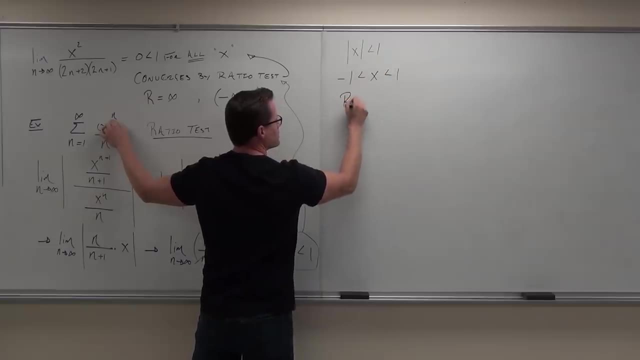 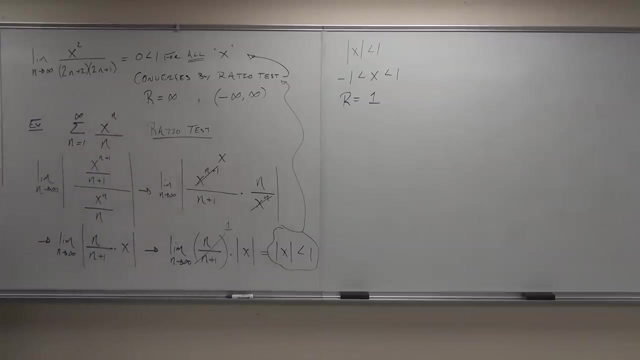 One. What's the radius of convergence? One, There you go. So you look for whatever's being raised to this power right here. When you get that, that is your radius of convergence. So the radius of convergence is one. So so far, what we know is that 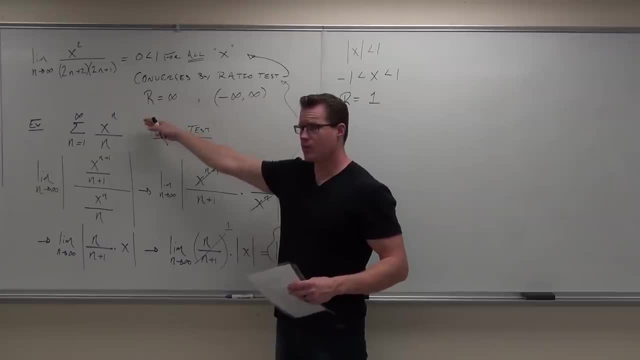 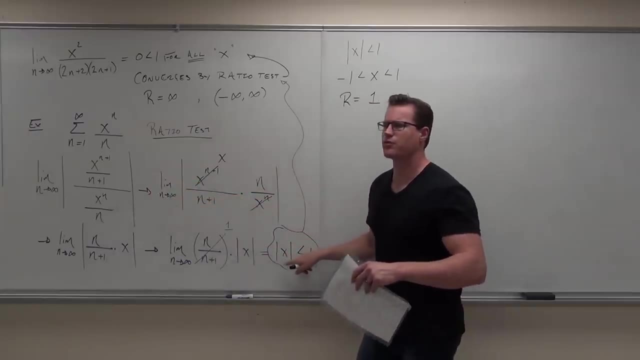 yeah, our power series represents a function, no problem. We've used our ratio test to say that this thing, this power series, is going to converge when the absolute value of x is less than one for sure. So basically when x is between negative one and one. 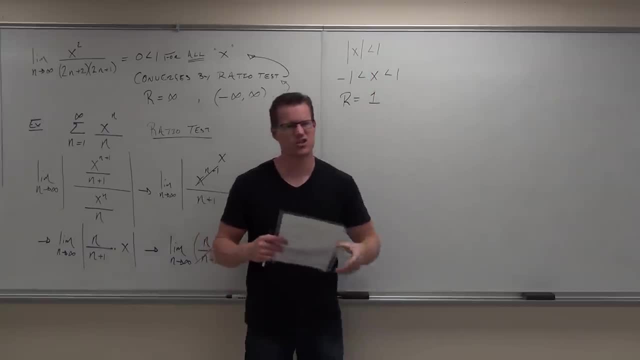 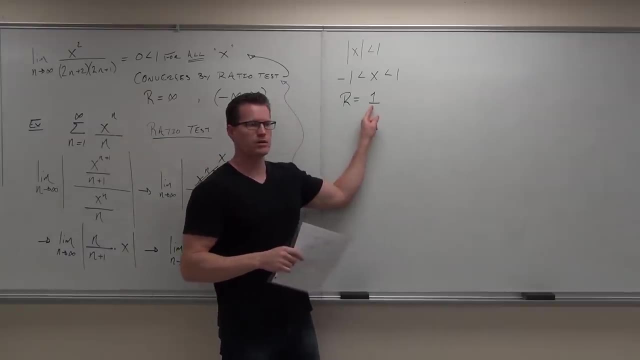 what that says is the radius. By the way, what's the center? What's the center of this? Zero, The origin. Zero, The origin, OK, zero. Hey, add one to zero. what do you get? One. 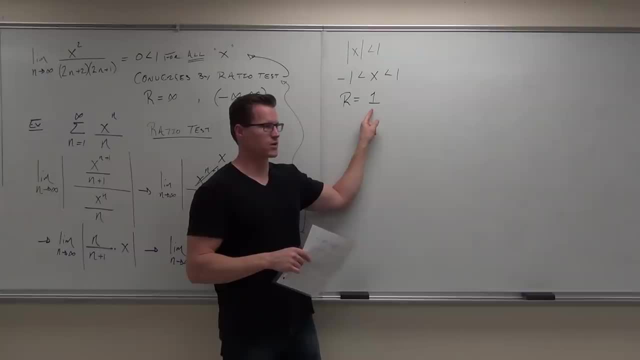 Subtract one from zero. what do you get? One. That's why the center's zero and the radius is one. OK, And the way you do this is you find out the thing that's being raised to n, that's your radius. 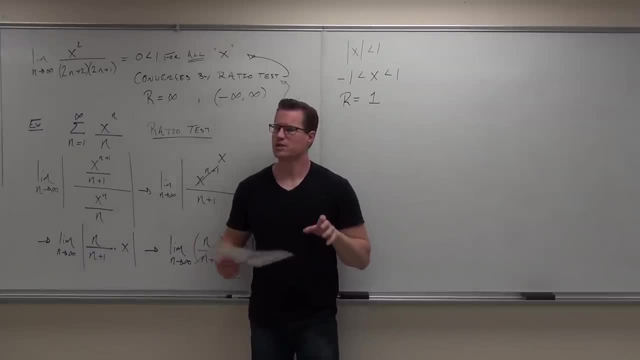 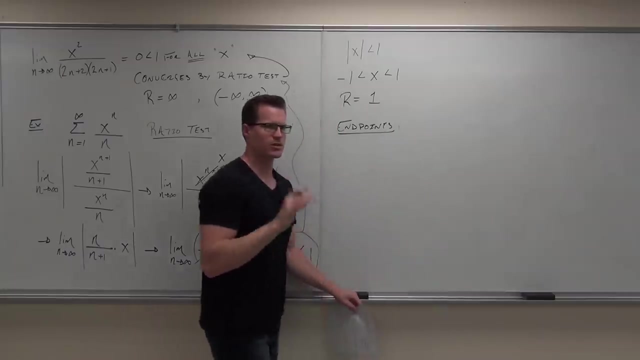 That's what it is Now. the issue is: are the endpoints included or not? Well, the ratio test does not tell you that. You have to determine that. So now for our endpoints. It's not hard, in fact. It's all that stuff that you learn about series. 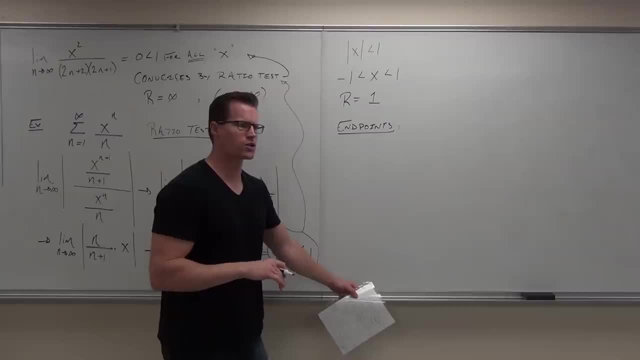 which is kind of cool. So now for endpoints. Can you tell me what are our two endpoints that we have here, Negative 1 and 1.. You've got to check both of them. There's only two things you've got to check. 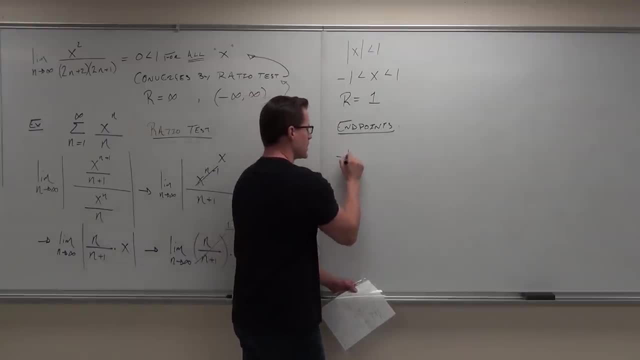 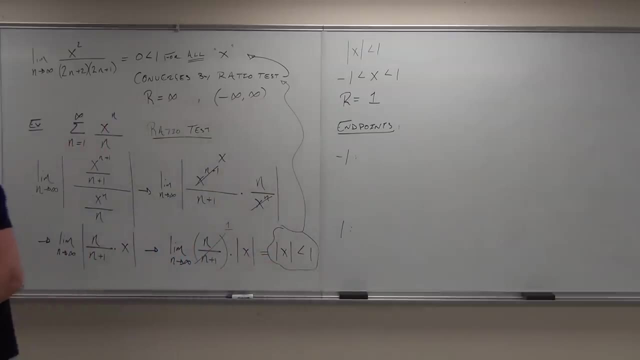 Two things you've got to check. There's only two endpoints, So we're going to check negative 1.. And we're going to check 1.. Wait a minute, How in the world can I check my endpoints? Well, let's plug it in. 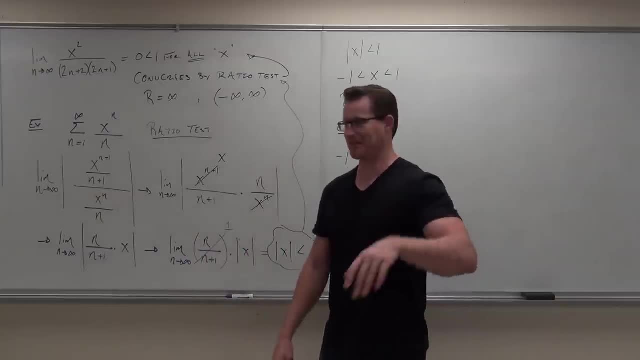 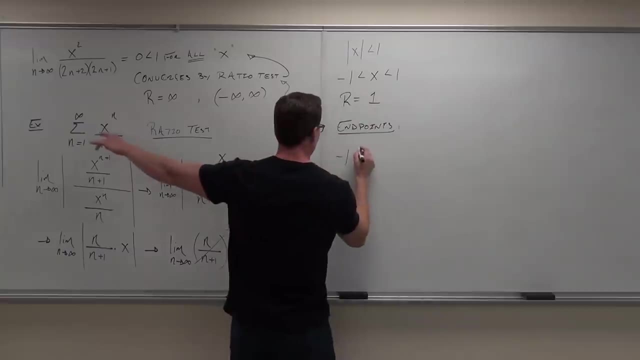 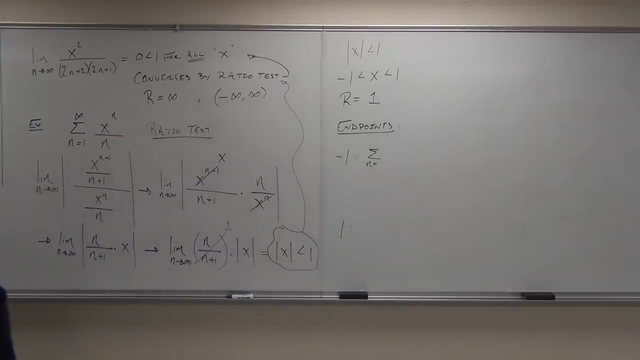 I just spit all over it. Do you see that It's on the tip of the gross? Plug it in here. So here we go. So if we have our series n equals, I say 1.. Shouldn't it be 0?? 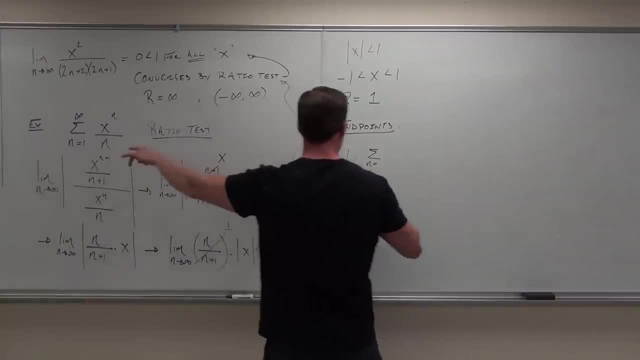 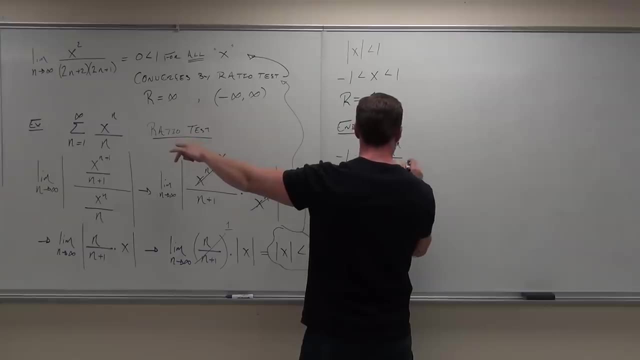 That one is 1.. Interesting. So if we have our series going from 1 to infinity, of x to the n over n, What am I putting in here? What am I plugging in for? Am I plugging in for the n or am I plugging in for the x? 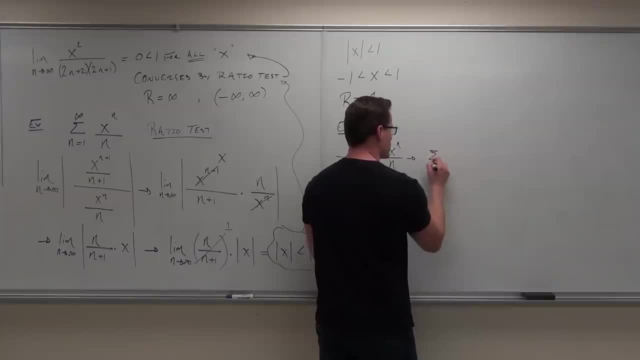 X. It says x. So what we get is a series from 1 to infinity of: oh, it can't be 0.. We divide by 0.. Oh, I'm sorry, What's our x? going to be Negative 1.. 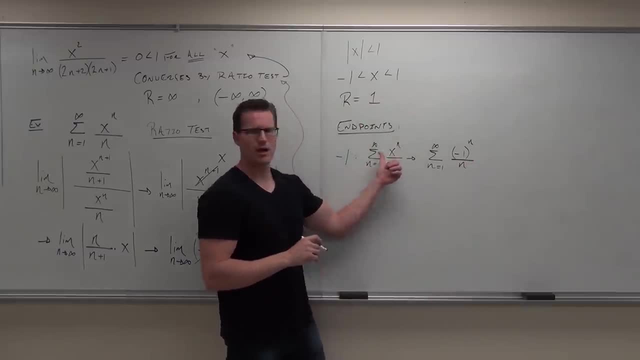 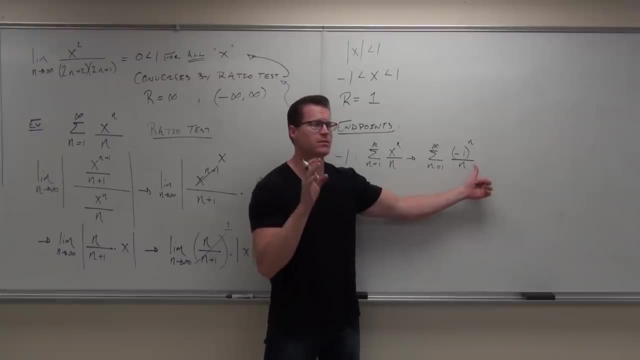 Wait a minute, Look at that. OK, so if we plug in negative 1, what's it do? It changes our power series. It's just a typical series that you have seen before. This will change into something you've seen before. 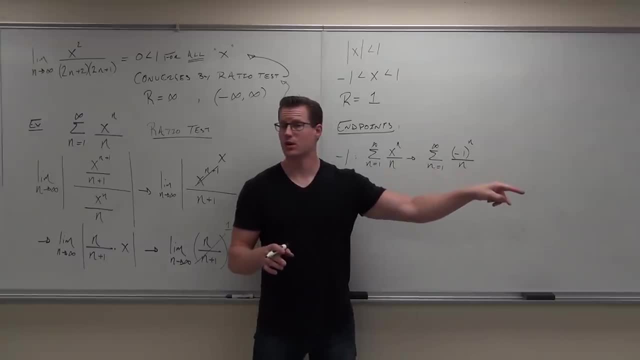 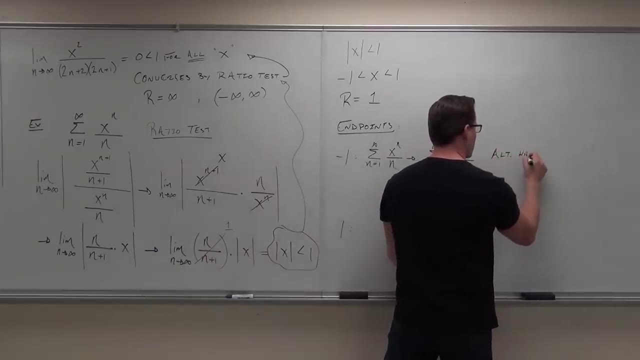 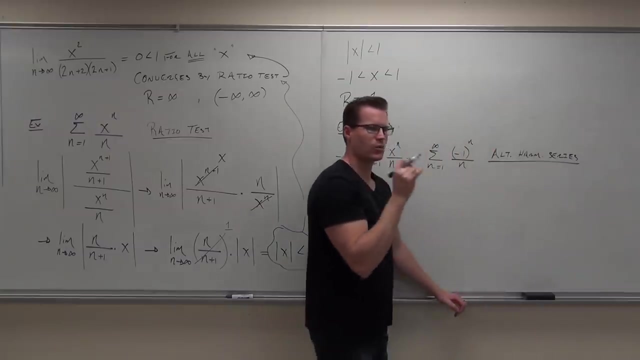 Tell me about that one Alternating harmonic. Alternating harmonic- We've done alternating harmonic before- It converges. It converges, So this is an alternating harmonic series And because we've done this already before, we know this thing converges. 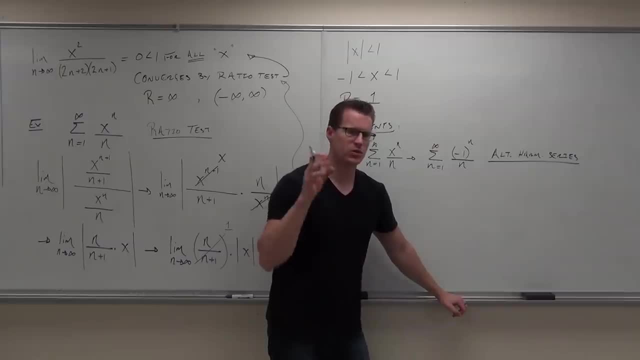 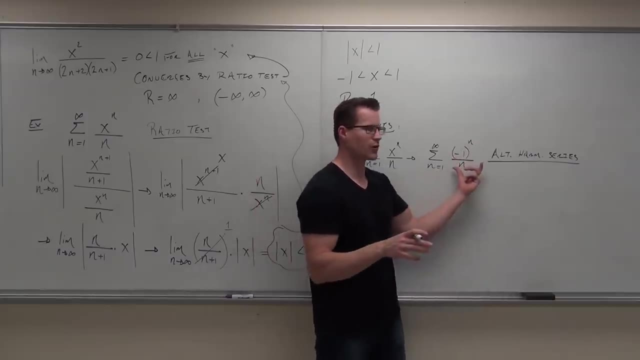 Listen carefully. If you didn't know, it converges. you would do one of the tests you've already done. You would do absolute convergence here, Because if you do absolute convergence you get 1 over n And that would be divergent. 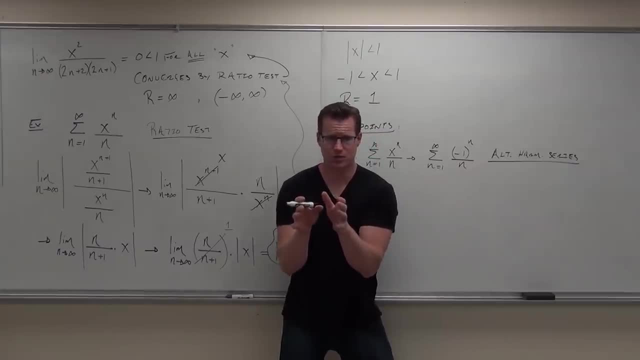 But remember that when you're doing absolute, listen carefully to this one. OK, When you're doing absolute convergence, if you take the absolute value and the series you get diverges, it doesn't mean the whole original series diverges, It means that it just doesn't absolutely converge. 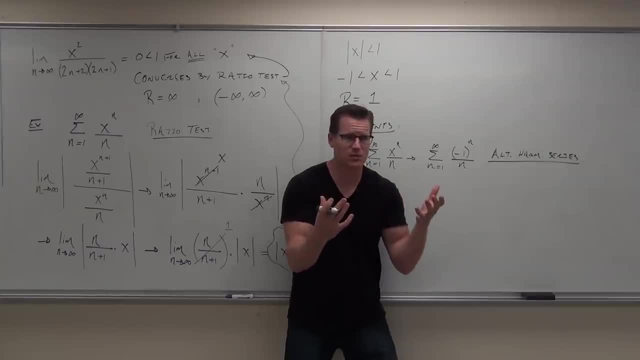 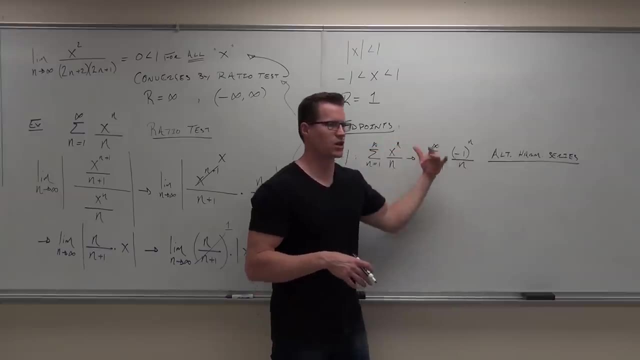 Remember that idea about conditionally convergent. It was the first thing that we talked about. OK, so here you go. Well, let's do the alternating series Alternating series test. The limit is 0. It's clearly decreasing. 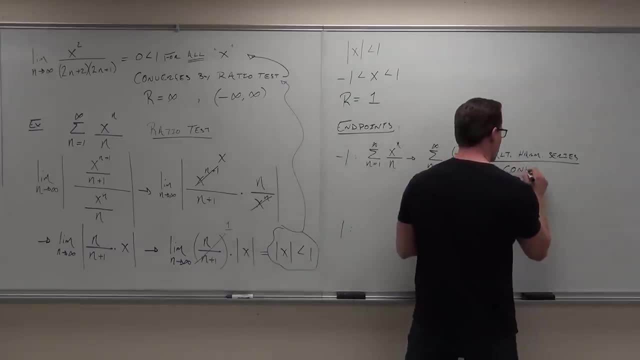 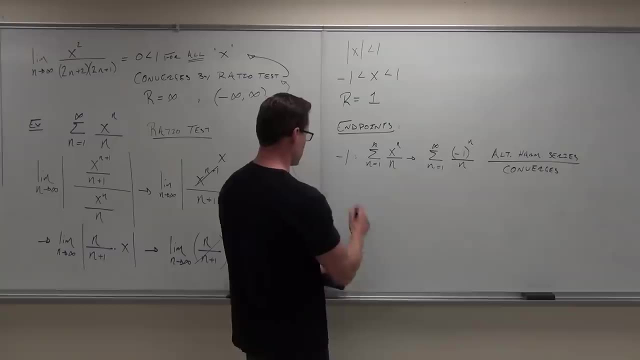 Alternating series test says converges. So even if you didn't remember this, we get a convergence. Now the next one. I'm going to move it up here, It didn't take a lot of work. The next one: If we get a series, n equals 1 to infinity, of x to the n over n. 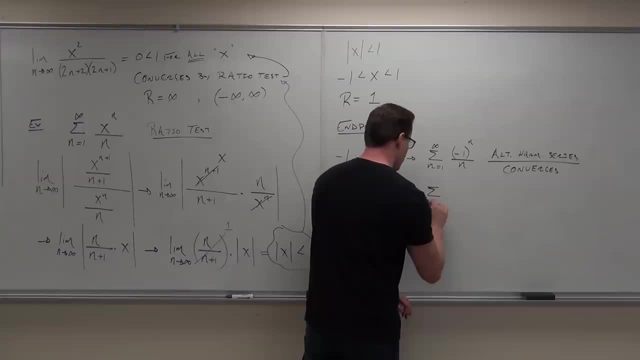 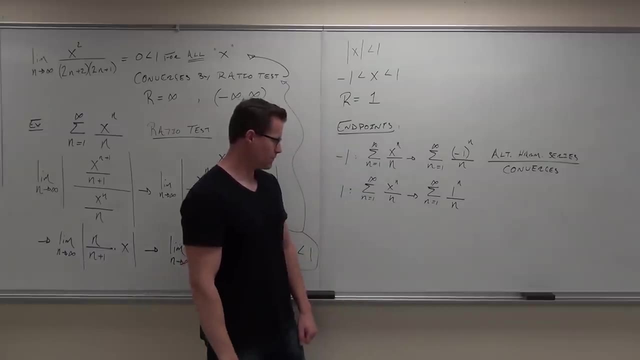 and we say: let's let our x equal 1, then we get the series from n equals 1 to infinity, of 1 to the n over n. What's that Harmonic series? 1 to the n is always 1, isn't it? 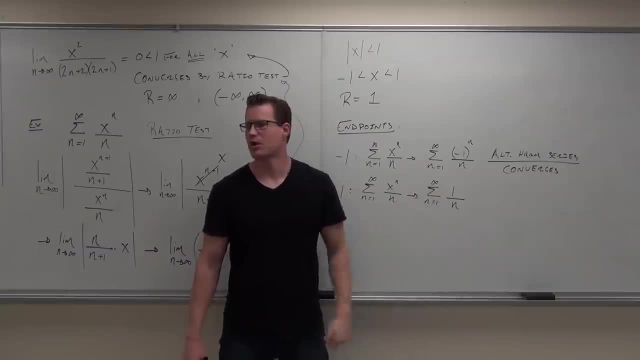 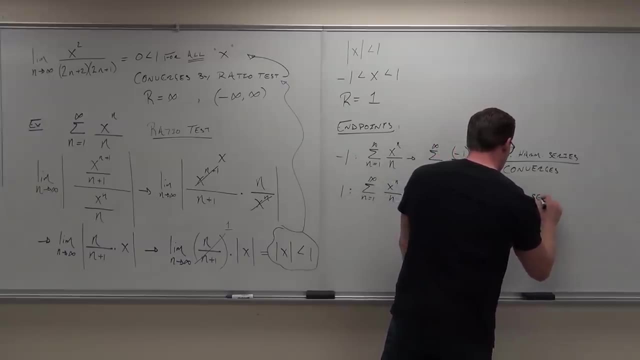 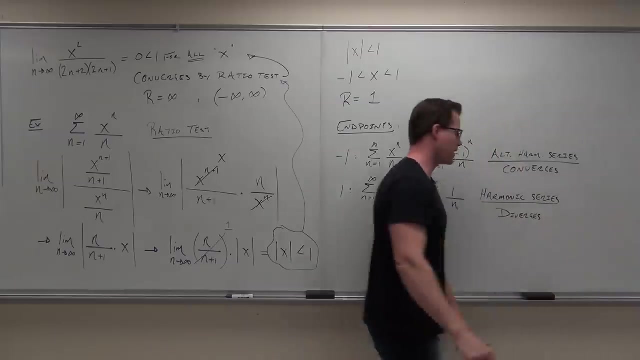 Yeah, What's that again? Harmonic series. Tell me something about harmonic series Divergence. So we only include the negative one. That, my friends, is how you find out whether or not your endpoints are included. So here's what you do for the most part. 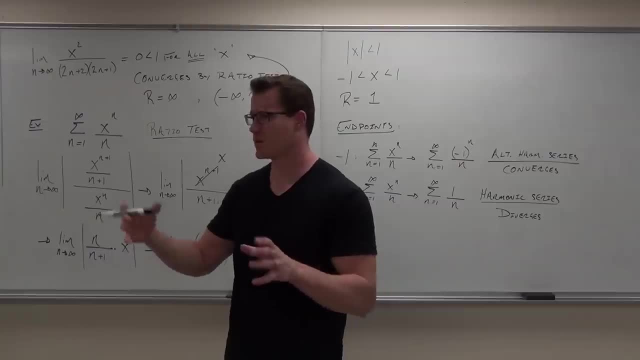 on all these problems with your power series. It's not that hard. I know it looked originally like: oh my gosh, what are we doing here? It's not that hard. Honestly, what you're doing, you're taking your power series. 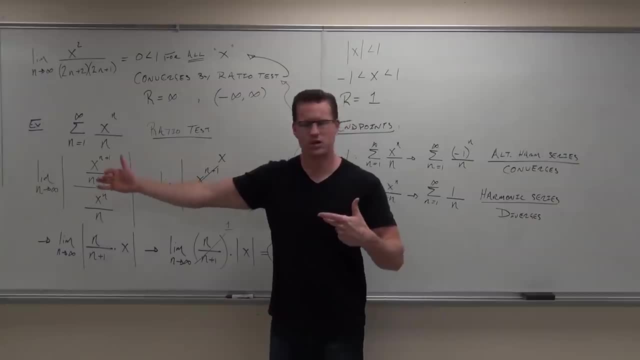 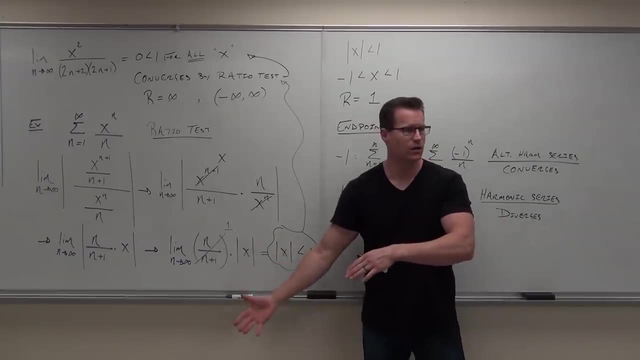 You're going. OK, I know that represents a function Where Use a ratio test. The ratio test will tell you where. Remember, ratio test only converges, for whatever you get here is less than 1.. So ratio test is cool, man. 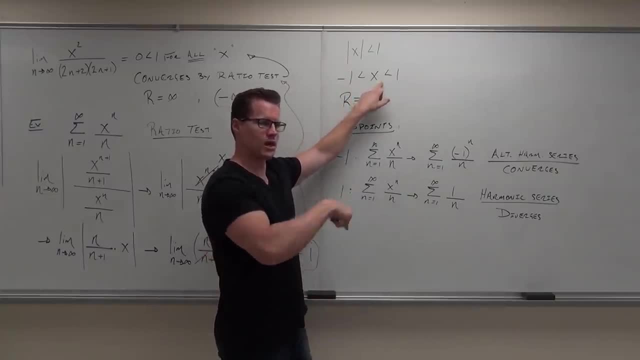 You know where that's going to converge, You just don't know the endpoints. Use those endpoints in your original power series with some of those tests you already know Alternate, harmonic converges, Harmonic diverges. What endpoint will we include? What endpoint will we not include? 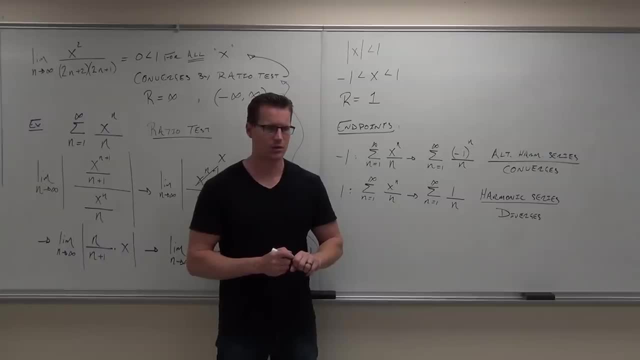 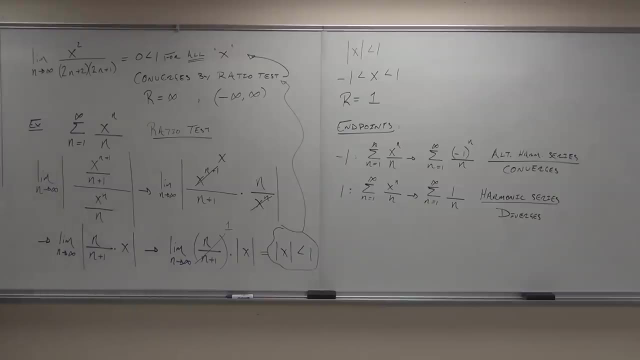 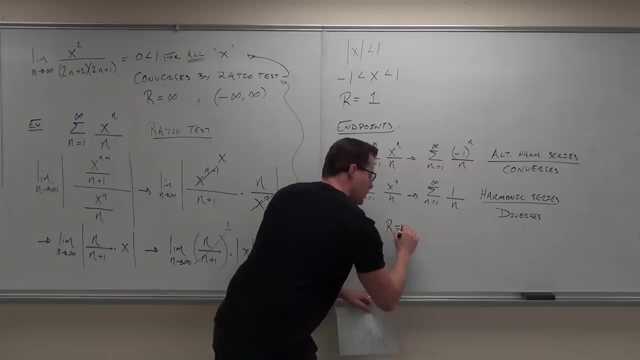 Negative, 1 we include Good And 1 we don't include. OK, so now, the last thing we're going to do here. So the last thing we're going to do: our radius. what was our radius of convergence 2 and 1.. 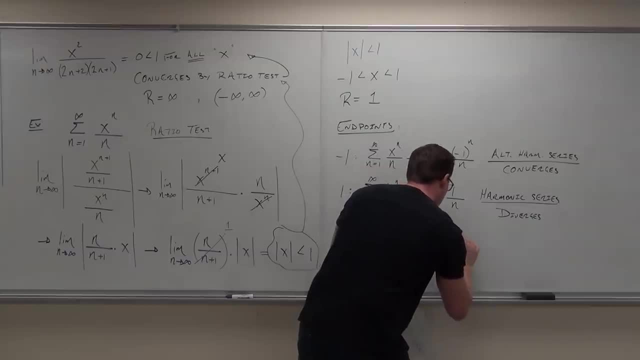 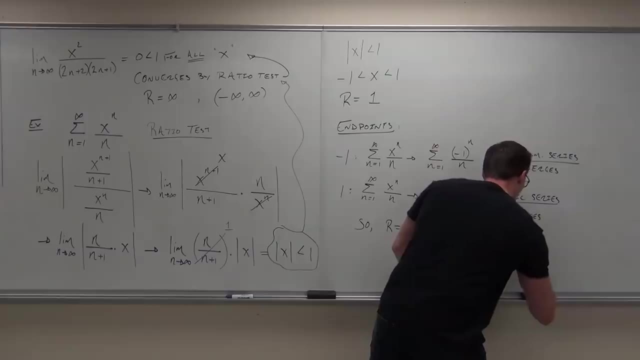 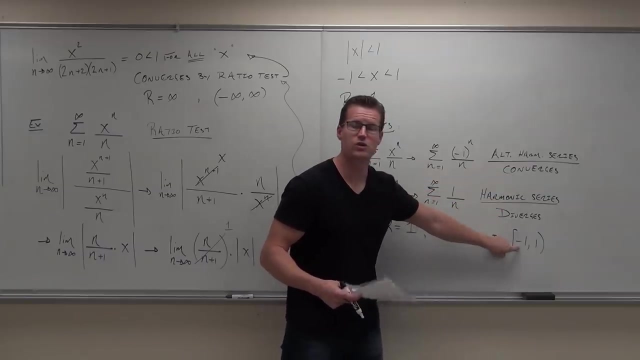 And our interval of convergence is: what's our interval of convergence Bracket: negative 1.. Why is there a bracket there? It includes negative 1.. Negative 1 makes that series converge. Remember our domain is all the numbers that make our series converge. 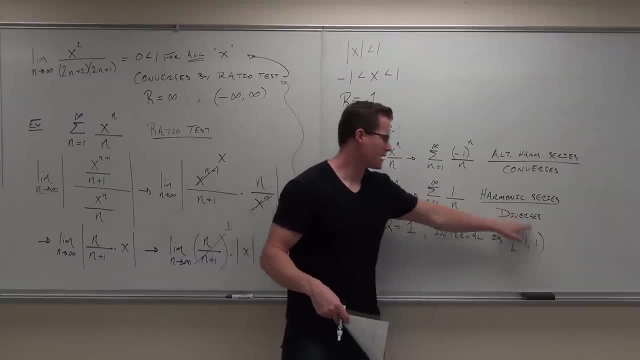 So if it converges, negative 1 is included. If 1 diverges, 1 is not included. We already had the rest of it right here. So we go negative 1 to 1 and just talk about the endpoints now. 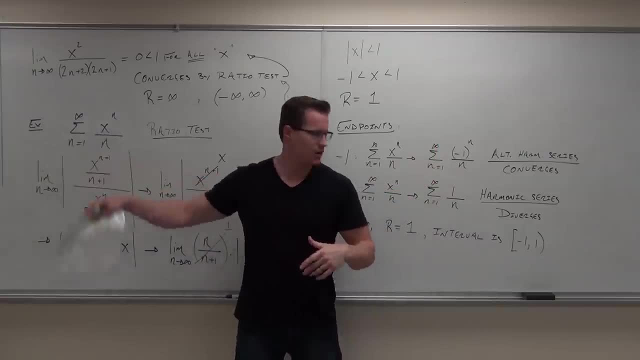 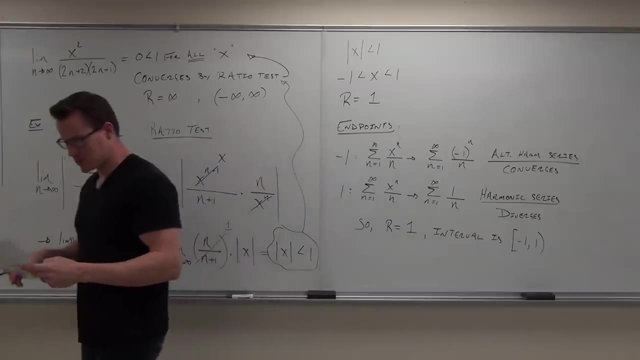 Does that make sense? By the way, what was the center for this 0.. Where's the center between this 0.. Does that make sense? Yes, Tell you what. let's go ahead and start with one more. This is practically. 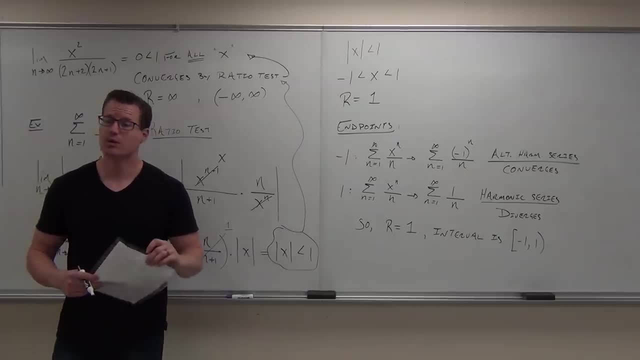 we have two more examples, and that's about it. Then I'll teach you how to do the calculus of power series, how to do derivatives and integrals of this stuff. Yes, you can. No, No, Yes, you can. 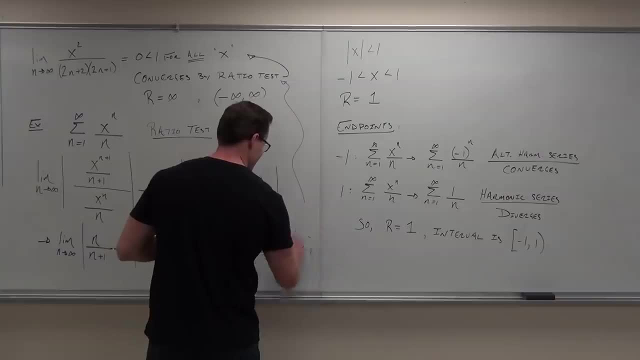 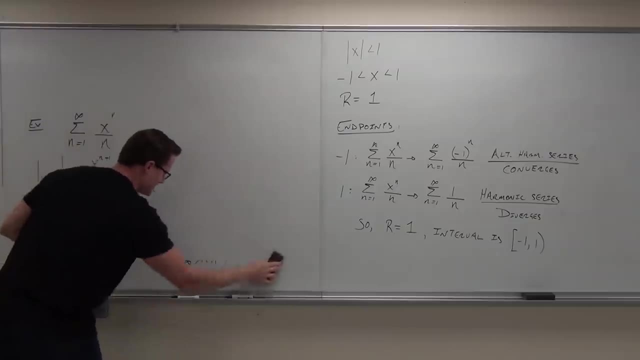 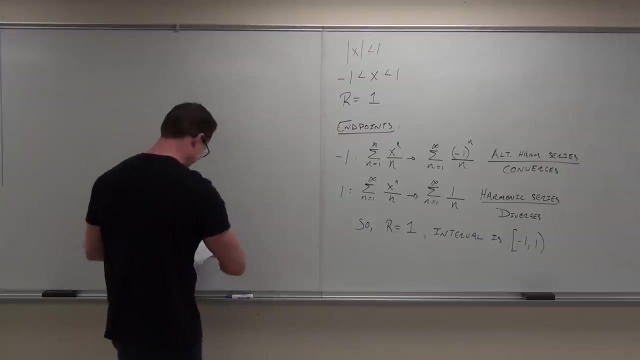 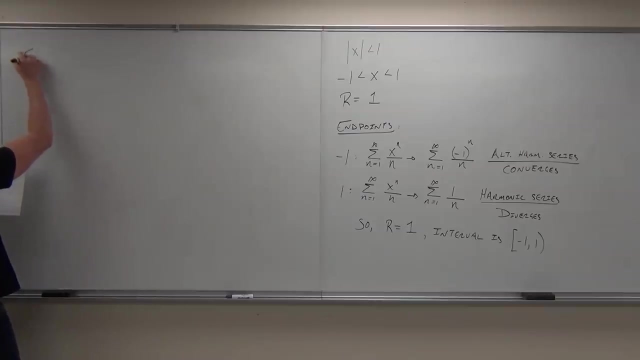 You can do it, Don't fret, Don't fuss, It's calculus, Let's do it. Doing so dorky, I can't help it. Oops, That can't be right. There we go, Oh dear, All right. 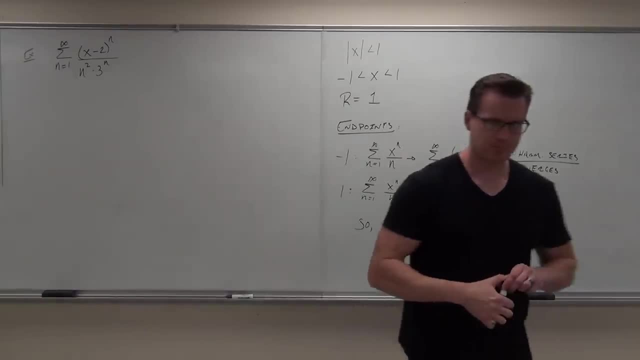 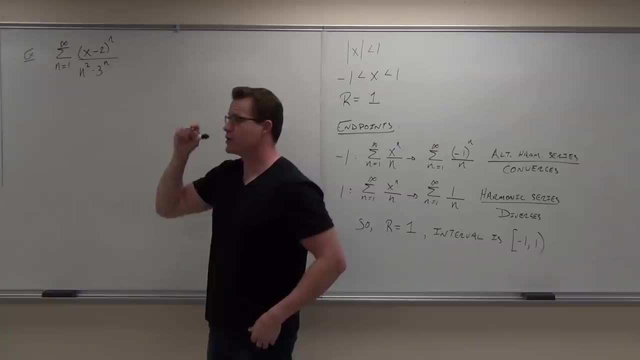 Let's do it, Let's go through it right now. Firstly, what is this Power series? You see something like that with an X raised to the end. Power series, Absolutely power series, For sure. Now you tell me. 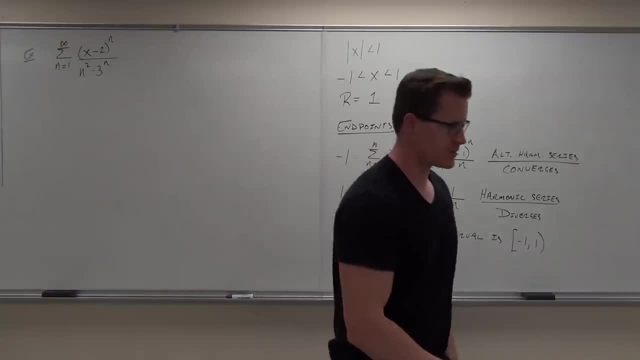 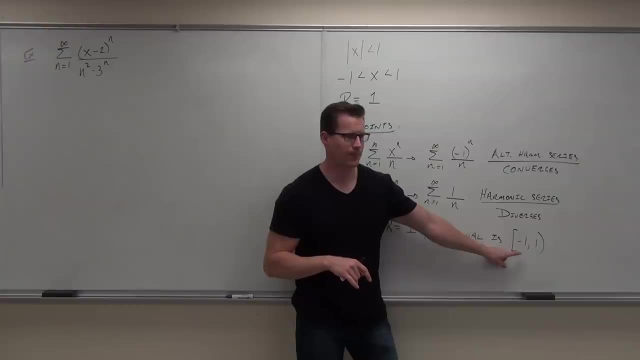 right now, where is this power series? centered At 2.. Very good, Centered at 2.. Which means this: When we get down to this part, our interval of convergence, the center, is going to be at 2.. It'll be 2.. 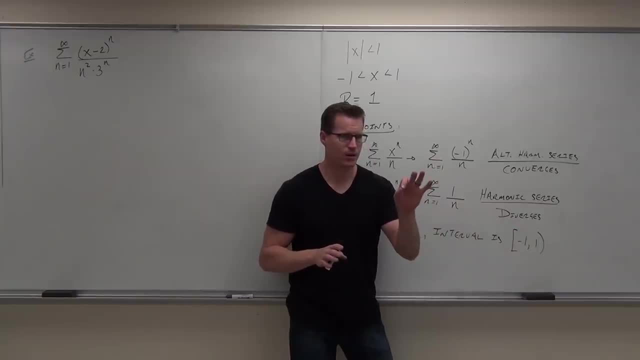 If it converges, it's going to be at 2.. If it converges at more than one number, it'll be 2 plus and minus the radius of convergence, whether that's infinity or that it's a finite number. Does that make sense to you? 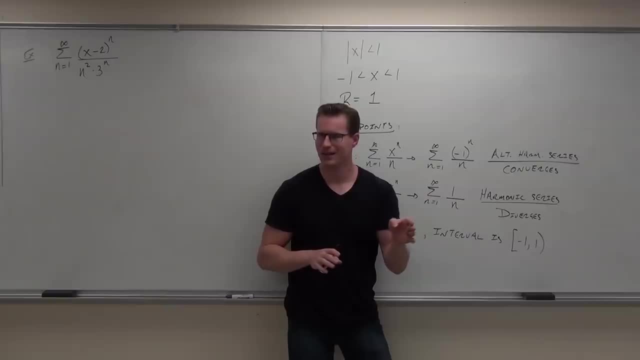 But 2 will be at the center for sure. Okey-dokey, Okey-dokey. What are you going to do? Ratio test, Ratio test, Do a ratio test. That's not any power Ratio test is going to give us. 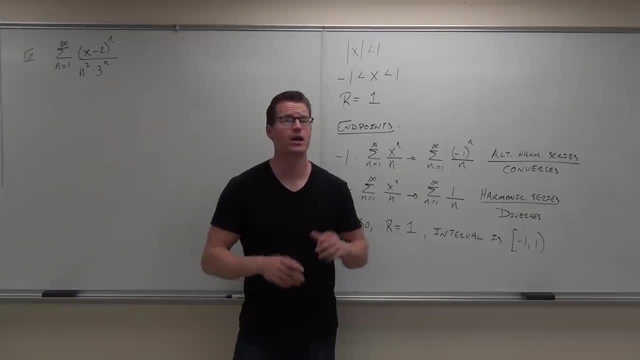 something less than 1. anyway, Do a ratio test. What are you going to use for most of these things? Ratio. Do you understand that ratio test works when the root test works as well? Yes, Do the ratio test. So we're going to do. 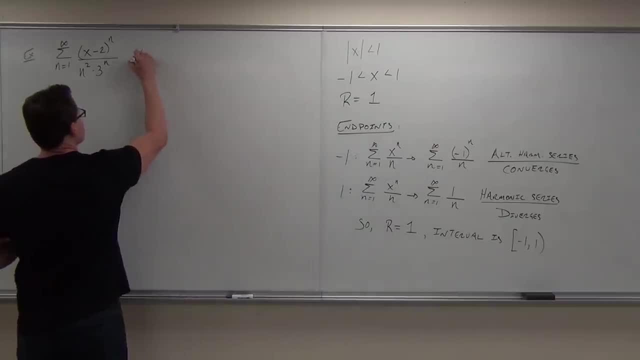 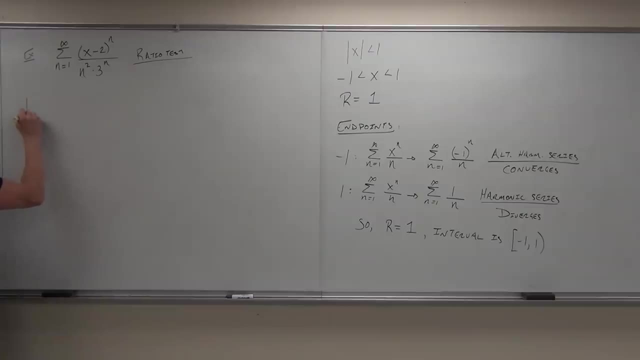 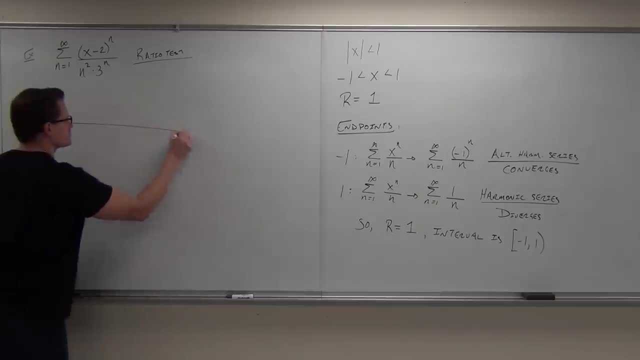 on getting these correct here. Be real careful. Of course, the ace of n is pretty easy because it gives it to you, but don't make a mistake on the n plus 1 idea. Remember the ace of n always goes on our main denominator here. 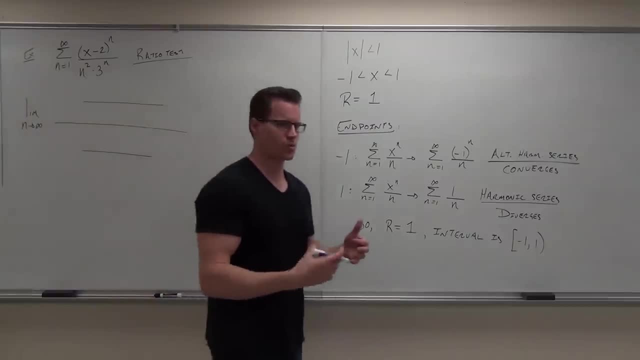 so we're going to have x minus 2 to the n over n squared times 3 to the n. You forget 1,. so we're going to have x minus 2 to the n over n squared times 3 to the n. 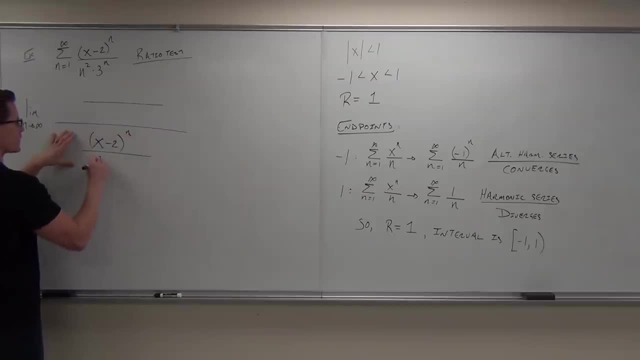 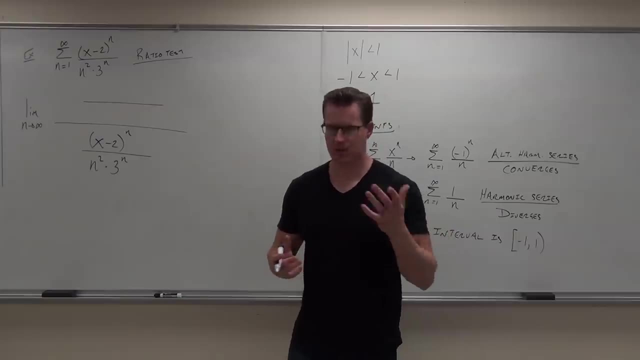 You forget 1, so we're going to have x minus 2 to the n, over n squared times 3 to the n. You forget 1, you forget that little thing and this problem explodes in your face. Okay, We're going to get. 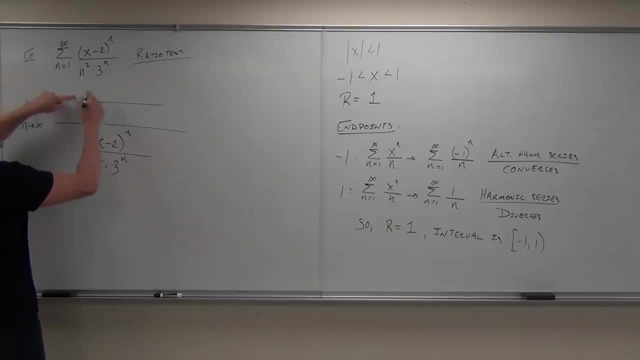 to that in a second. Okay, so up here we have. by the way, when you're doing the n plus 1,, does the x ever change? No, So this guy is going to be there, no matter what x minus 2,. 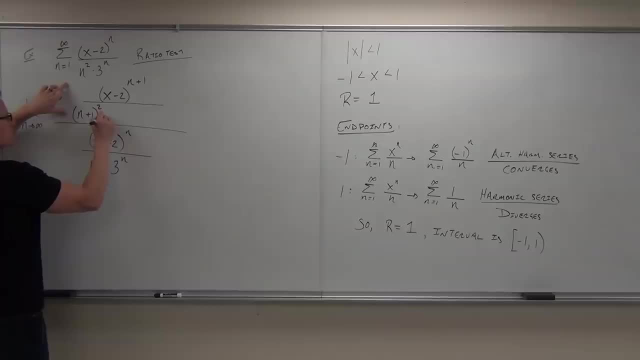 the n does, though we get n plus 1 over n plus 1 squared times 3 to the n plus 1.. Oh goodness, And I'm forgetting something. What else am I forgetting? Absolutely nothing. Yeah, you're right. 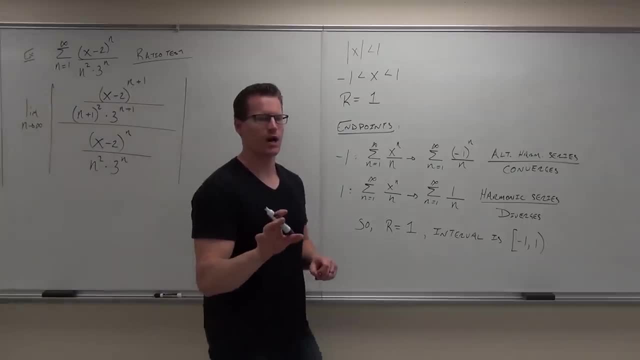 Is that important? If you forget an absolute value, forget your absolute value. look at what happens. Look at: if you forget absolute value, you lose this, don't you? You lose your other side of your interval. That's a problem. 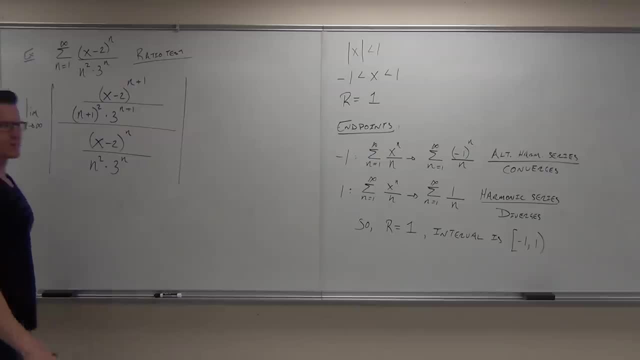 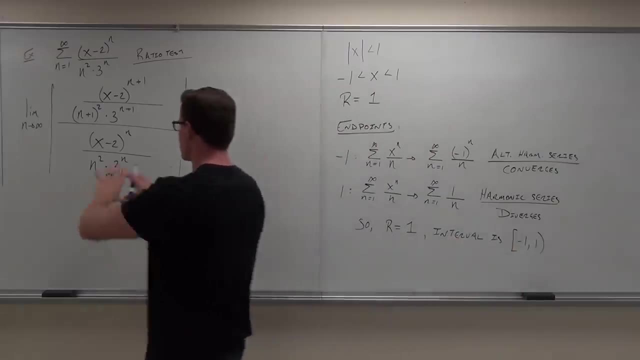 Okay. so, oh my gosh, from here. is there anything that we can get rid of automatically right now? No, There's no negative ones. it's not like that alternating idea. so we'd have to go through and multiply by the reciprocal. 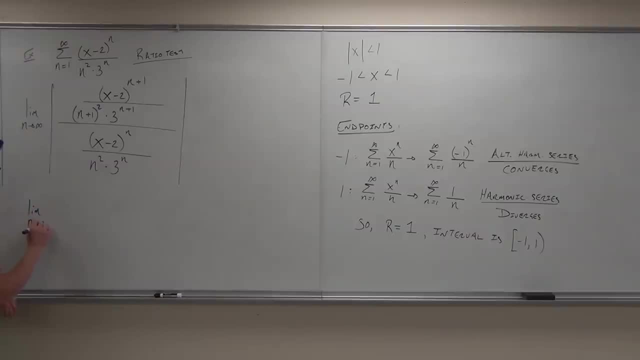 Simplify as much as you can. And yes, absolutely, you've got to simplify by the reciprocal. Do we drop the absolute values right now? No, Oh no, The x is for sure. we can't drop that, So we've got. 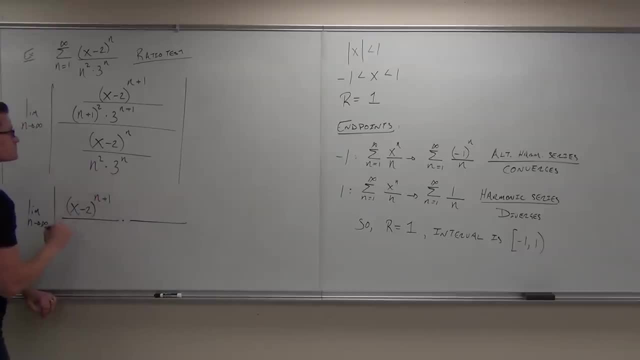 x minus 2 to the n plus 1.. We've got n plus 1 squared. We've got 3 to the n plus 1, no problem, Now multiply by the reciprocal. we've got n squared times 3 to the n. 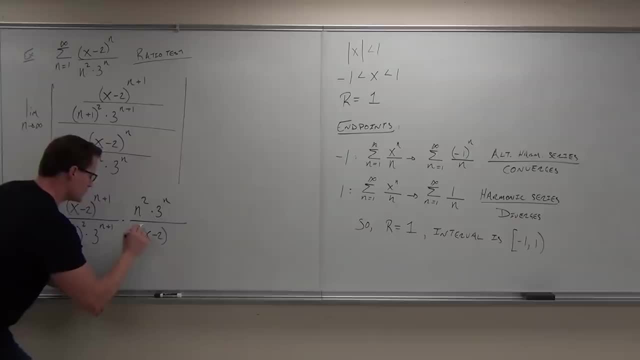 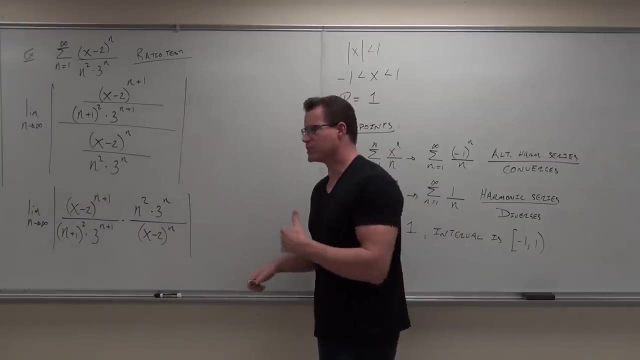 we've got x minus 2 times 3 to the n, and then we still have the absolute value. I promise you the simplification gets way easier when you get used to this. Right off the bat you're like: oh my gosh. 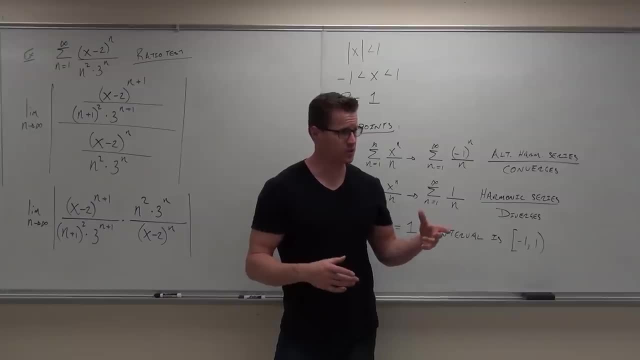 what are you doing? But when you get used to it it gets really quick. It's really nice. You get used to what a plus 1 and a plus 2 mean as a power and you can simplify stuff really fast. Have you ever done it? 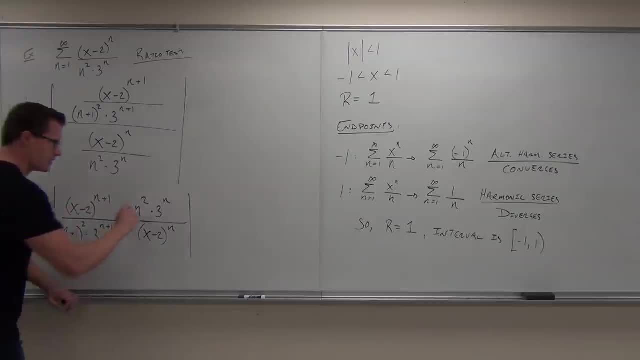 Yeah, Probably Tell me something that does simplify 3 and 5.. So if I simplify 3 to the n, with 3 to the n plus 1, I get the 3.. And it's on the denominator, yeah. 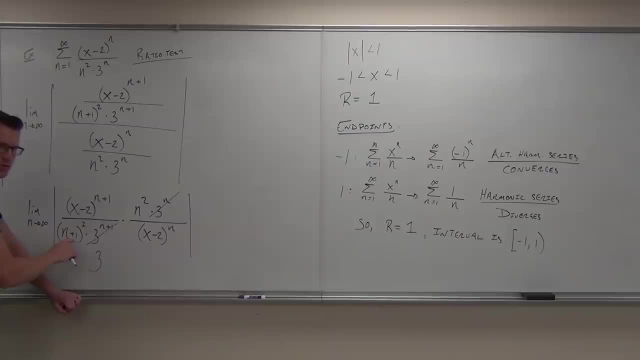 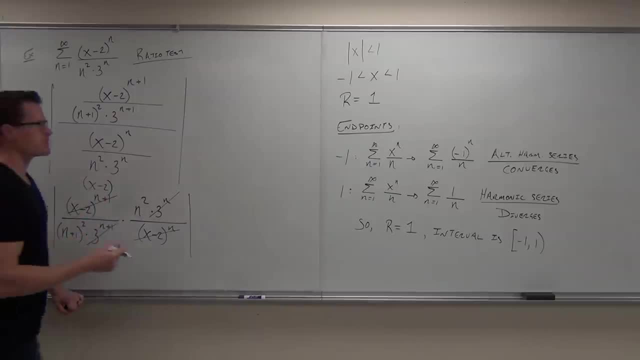 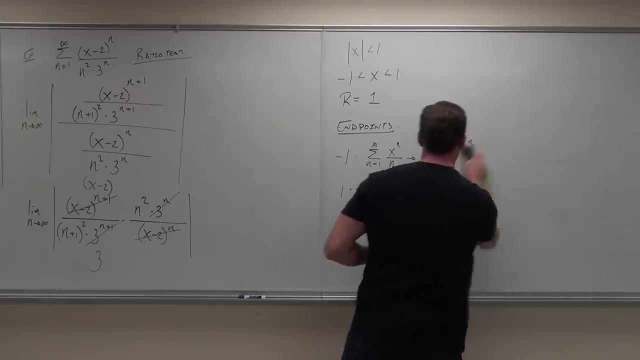 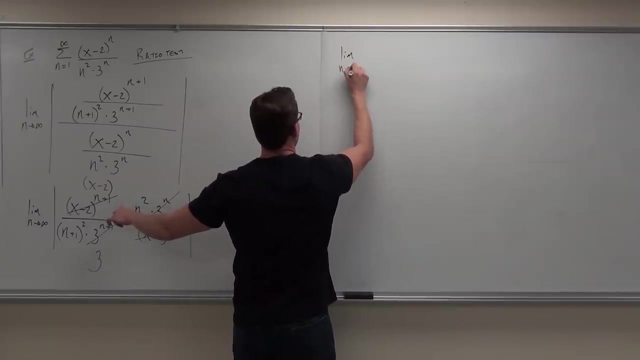 do, do, do, do, do. Do you know what? we end up getting? Dinner at Wells, and we're not gonna have much time after this anyway, so I'll erase this. What we end up getting is a limit n approaches infinity. 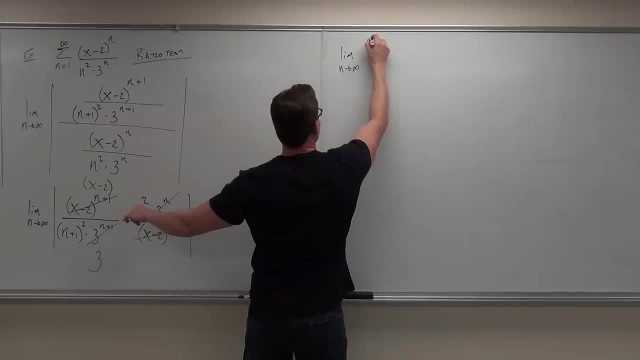 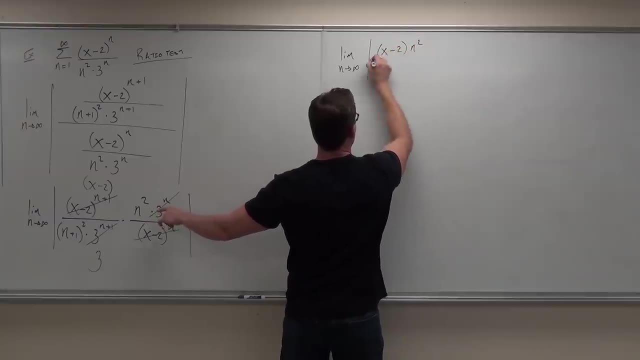 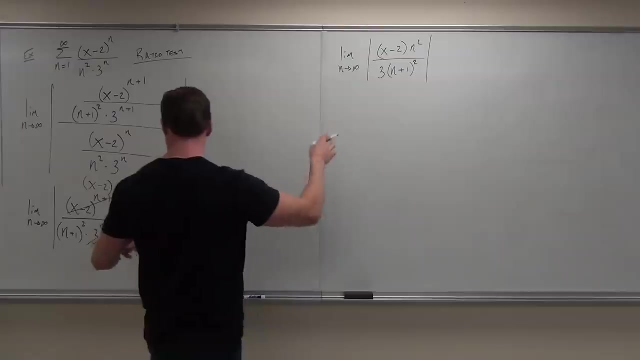 do I still leave the absolute value? Yeah, Yep. What's on my numerator, please? Over 3 and plus 1: squared, Okay. x minus two: no problem. N squared, no problem. Three: no problem. N plus one: squared, no problem. 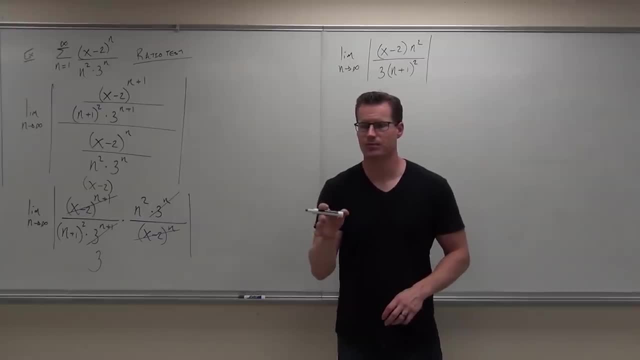 Chopin should be okay with that. Here's what you do now. please be careful. What you do now, you collect your n terms. You do not collect constants and x's. Those are important, So collect your n terms. What I mean is that this stuff? 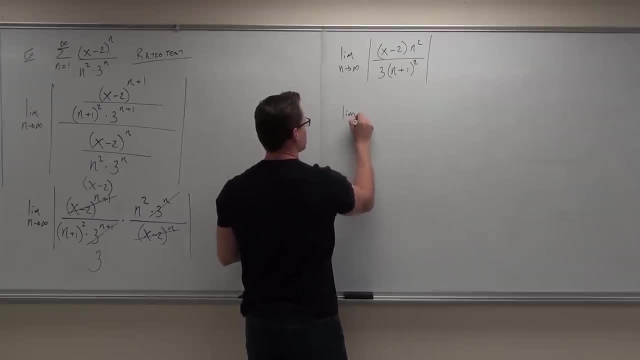 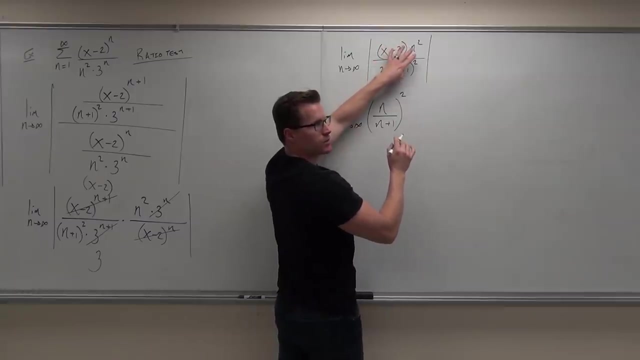 I'm gonna move this off to the side. I'm gonna get a limit. See if you can stick with me here. N over n plus one quantity squared. Do you see it? N over n plus one quantity squared. Notice how I don't have an absolute value. 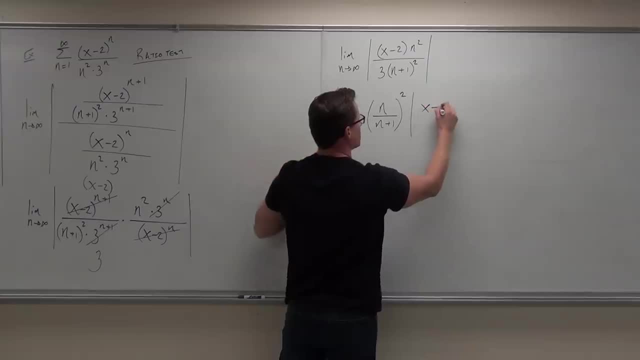 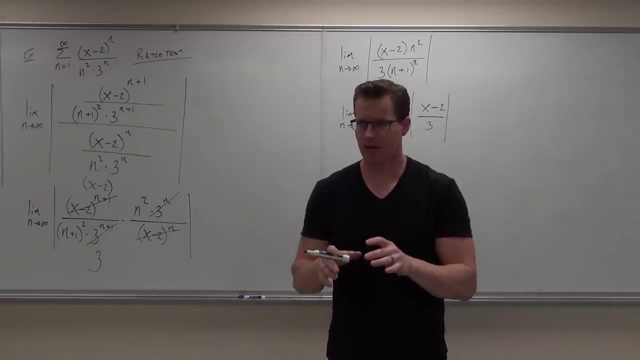 It's always gonna be positive. Then I have an absolute value of x minus two over three. Collect everything except for your x values and your constants. Does that make sense to you? Yeah, Honestly, are you guys okay with that one? Yeah, 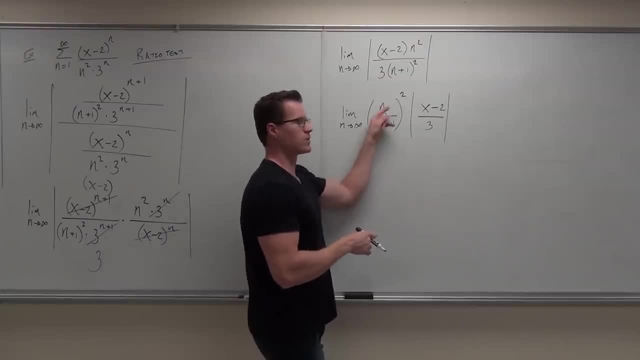 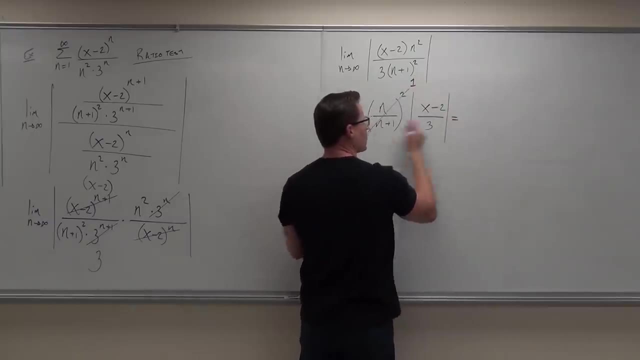 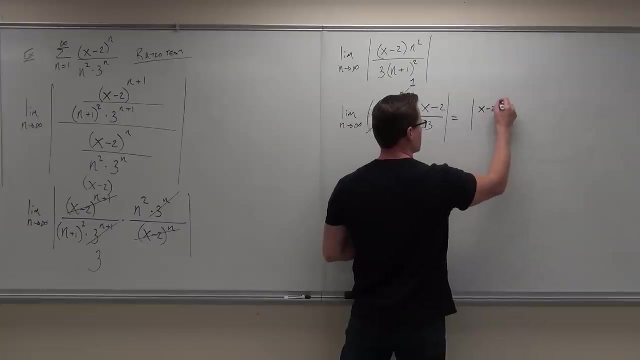 How much is n over n plus one? One, One And what's one squared One? So this whole thing is one, is that it Uno? So what is this whole limit equal? Two over three. Absolute value of x minus two over three. 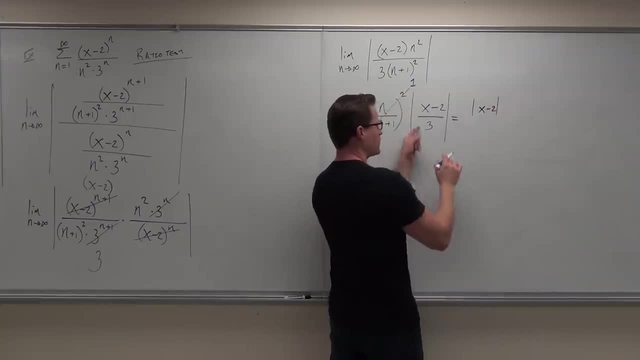 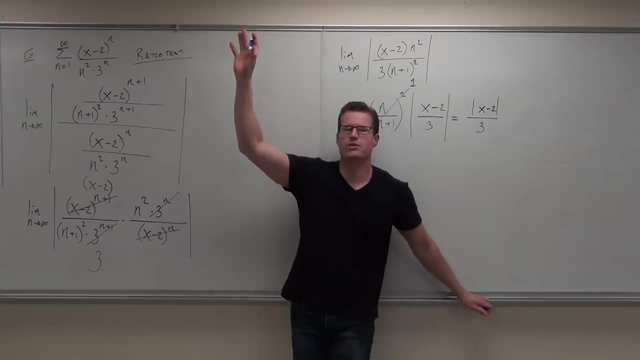 Actually, I'm gonna do this for you. Does this absolute value affect the three at all? No, That's what we get. Chopin should be okay with that so far. Now here's the question: What test did we just use? 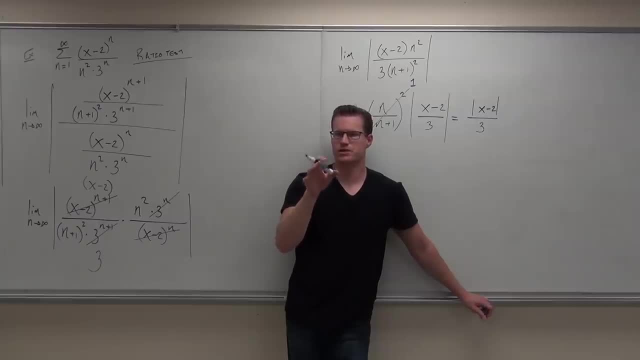 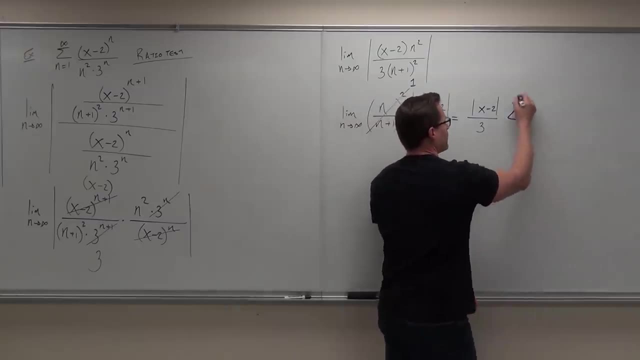 Ratio test. When does the ratio test show convergence? When the limit is less than one. Again, this is by ratio test. That's why we're doing it, because ratio test says that our power series, any series, converges if the limit is less than one. 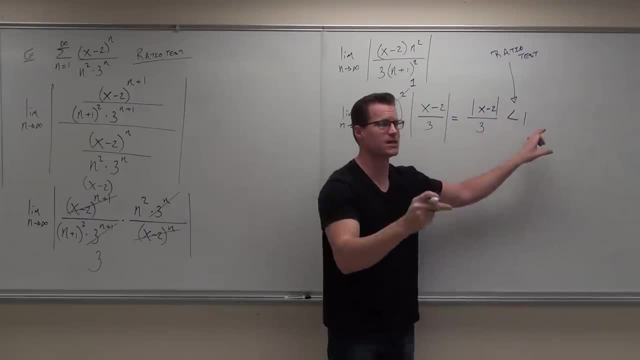 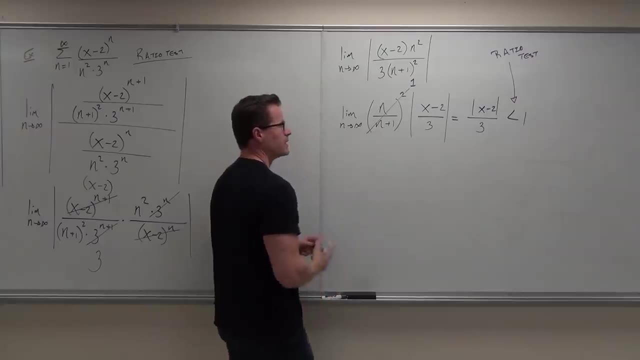 No problem. So this power series make the limit less than one. Therefore, you guarantee this thing is going to be converted. Does that make sense? Definitely have that, Okay. now what that tells us is that if I multiply by three, 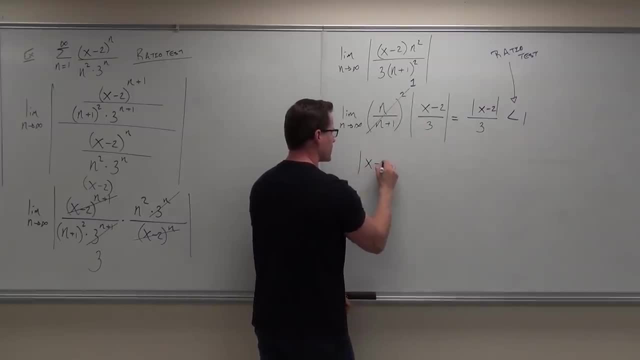 if I multiply by three, what I end up getting is absolute value of x minus two is less than three. You guys? okay with that one. If you're wondering, why are you multiplying by three? now Here's what I'm trying to do. 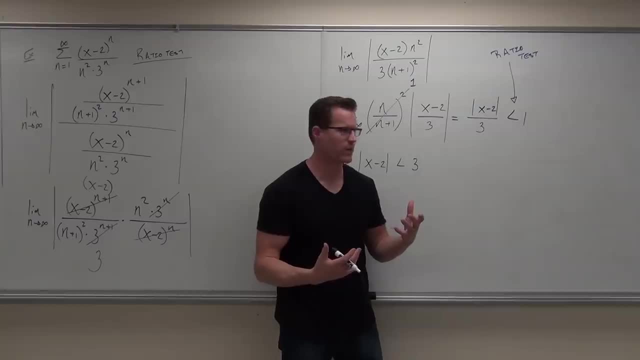 A lot of students get confused. How in the world do I find my radius of convergence? Is my radius of convergence one? No, Is it three? Is it five? Here's how you tell. See the thing that's being raised to the nth power over there. 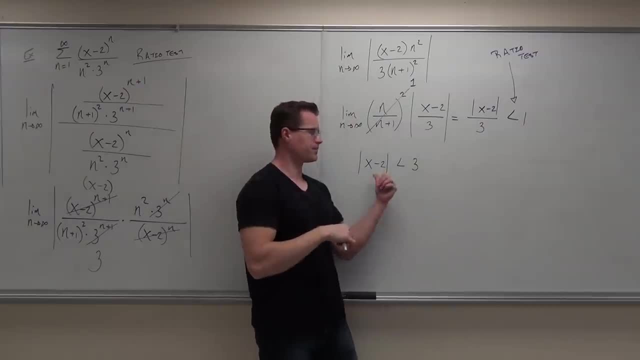 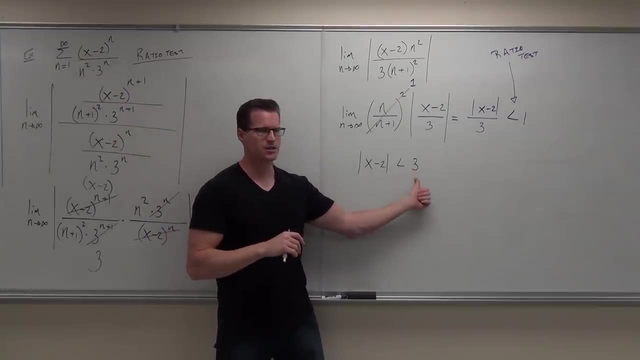 The x minus two. As soon as you isolate that, as soon as you isolate that x minus two, x minus two in absolute value, as soon as you isolate that, that is your radius. Does that make sense? Yep, So the radius is perfect. 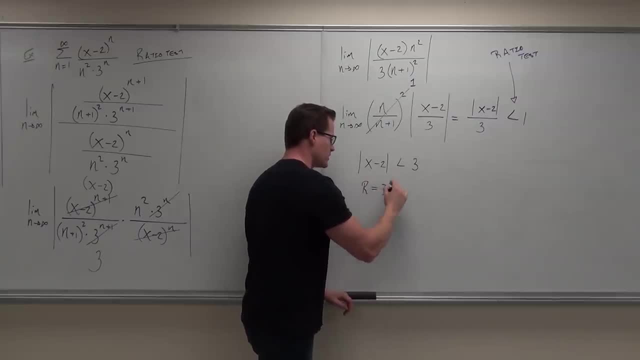 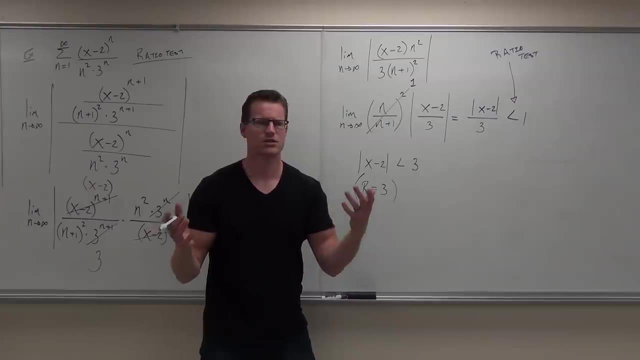 Radius of convergence is three. That's what this says right now, So I'm gonna put this right here. We already know the radius of convergence is three. Now, from here, all you gotta do is find the interval of convergence, and it's so easy, it's really easy. 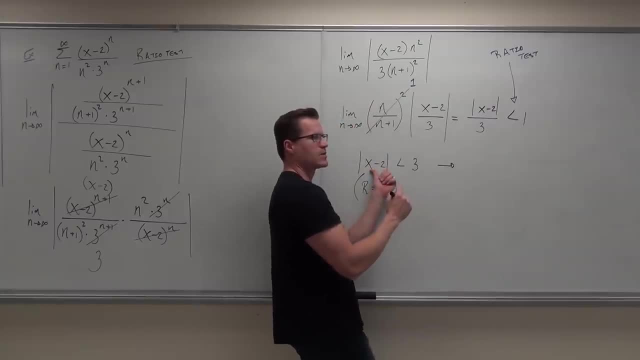 All you gotta do is solve for x. So if you solve for x, what an absolute value inequality means is you do? negative three is less than x. minus two is less than three. That's what an absolute value inequality is, right there. Then if we add two, we find our domain. 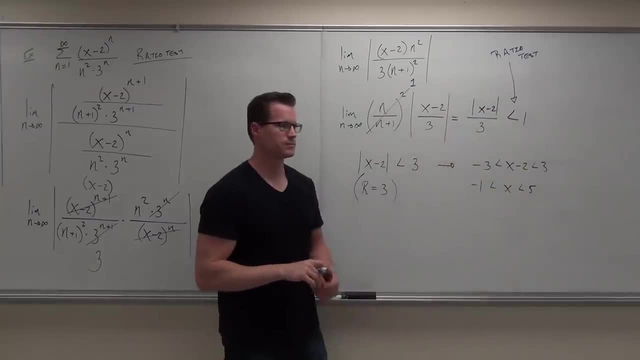 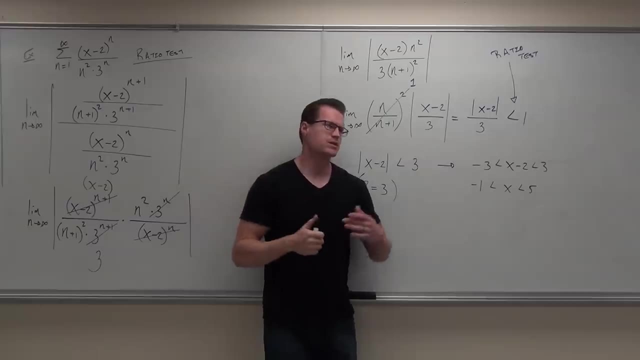 If you simply add two, So it seems to be okay with that so far. So this is why you do your radius first, because right now it's kind of hard to see. It's not super difficult, You can still do it. By the way, what number is at the very center of this? 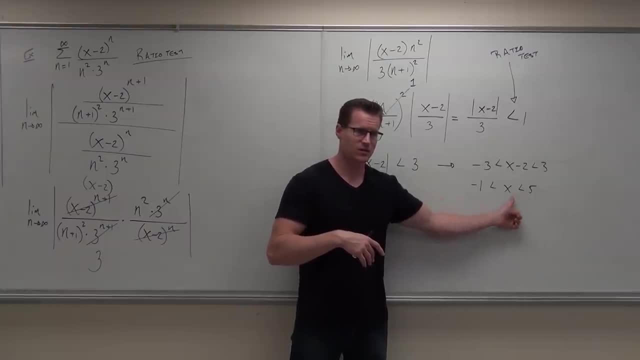 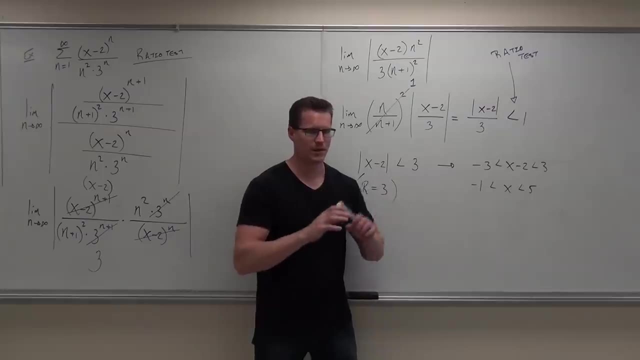 Two, Two plus three, Five, Two minus three, One. Oh yeah, Radius is three, center is two. Now what about the endpoints? That's the bottom end. Can we do that real quick? Yeah, go for it. 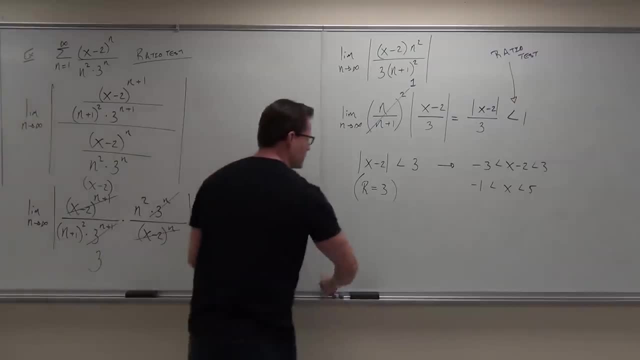 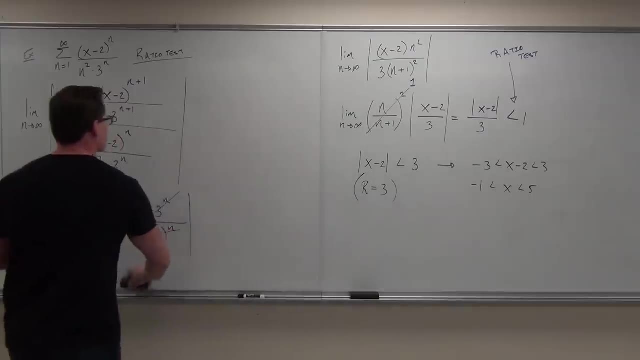 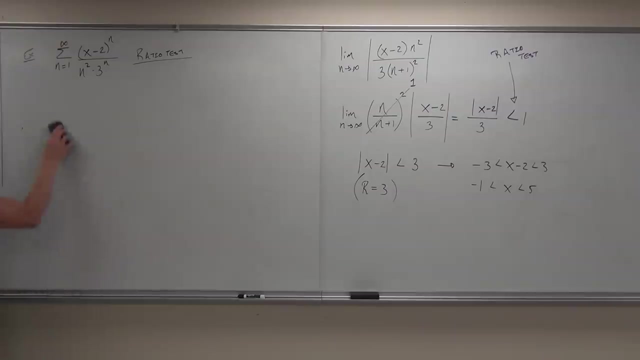 Oh, we don't want to do it. I'll do it here. You know what? I'm gonna erase this. I'm gonna do it over here. We're gonna test our endpoints here. So last little bit endpoints. So for our endpoints we need: 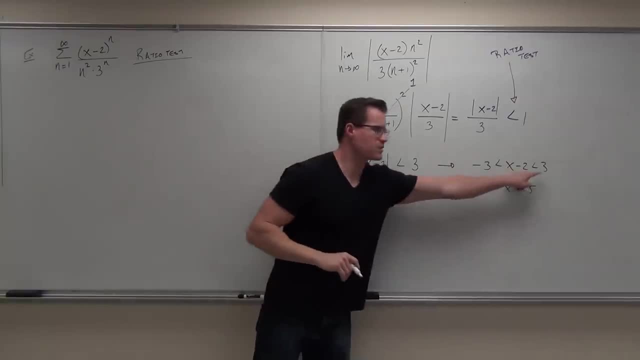 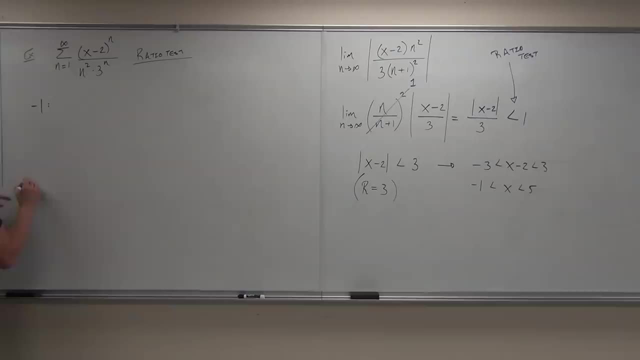 what's our first endpoint? we check Negative one. Don't be silly and check this. That's silly. okay, Make sure you solve for x to find your domain. This is the endpoints that are understandable right here. So we do negative one and we do five. 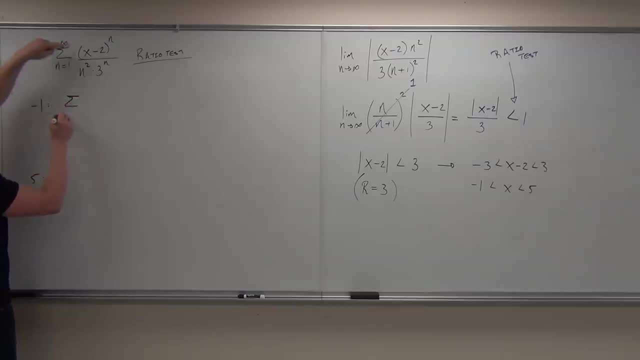 So if I'm plugging in negative one, what we end up getting- remember I'm plugging in negative one, right here we end up getting negative three to the n, over n squared times three to the n. What that gives you if you look at this real carefully. 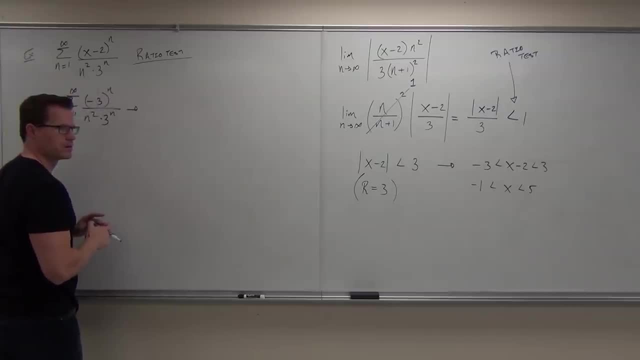 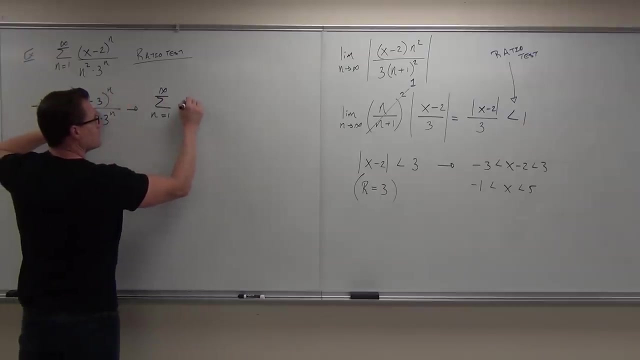 what this gives you is what One over n squared times negative three, Kind of Almost. You're so close. You said one thing wrong, Almost, Do you notice how they both have a power? So you could make negative three over three to the n right. 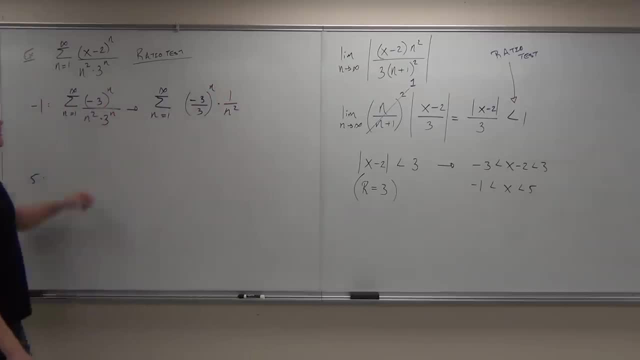 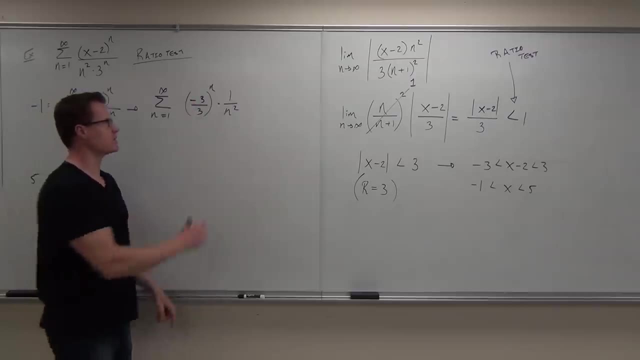 Times one over n squared. Nope, not geometric. Do you see that this is negative? three over three to the n Times one over n squared. Okay, it's not a denominator. How much is negative one over three? Negative one. Negative one to the n times one over n squared. 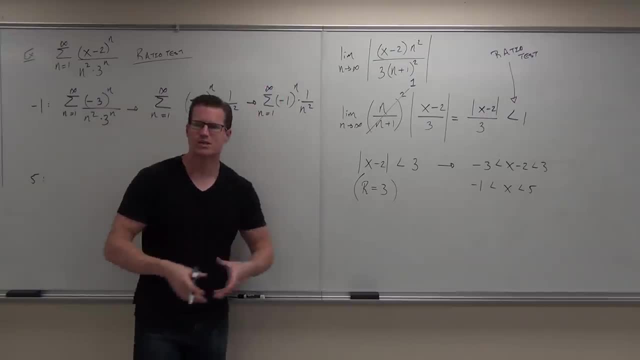 N equals 1 to infinity. Tell me something about this series. It's not a p-series. It's not a p-series, It's alternating series. You can do a few tests with this one If you want to be really quick about it. 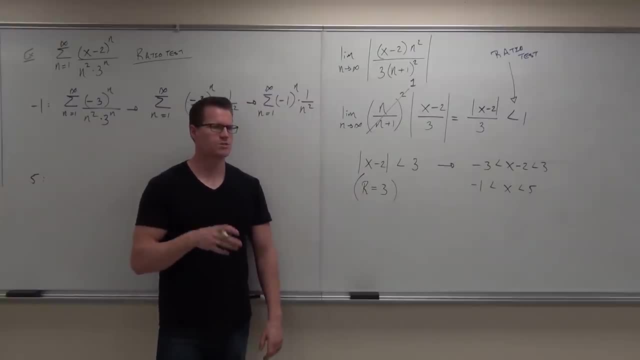 if you want to be real quick about it, do absolute convergence. Absolute convergence gives you 1 over N squared. yeah, P-series, booyah done. This series converges absolutely. If you don't need absolute convergence- which you don't- 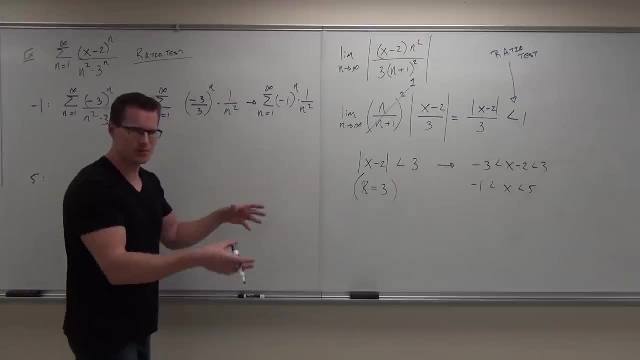 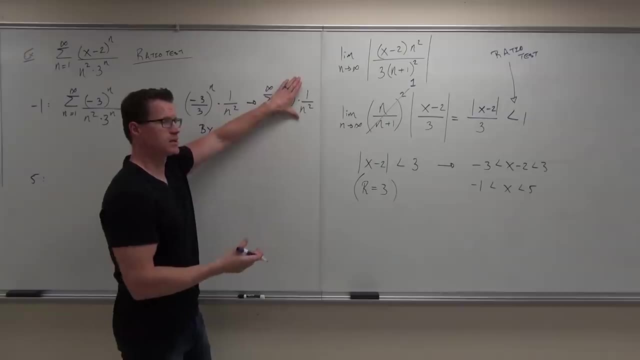 you just do alternating series tests. So that's what I'll do, because I don't need absolute convergence. I'll do by alternating series test. It's pretty clear that the limit is 0.. It's very clear that this is decreasing Limit 0, decreasing alternating series. 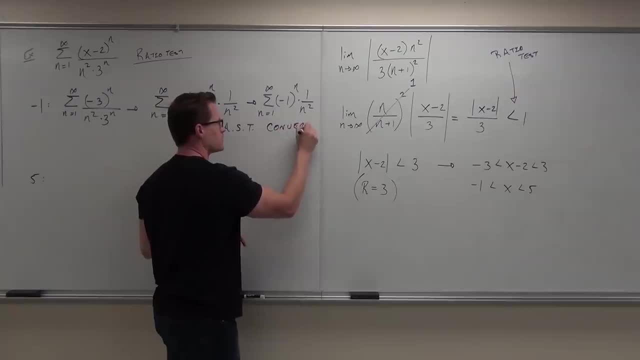 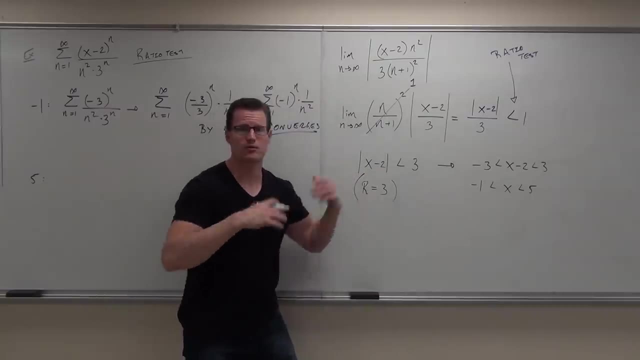 by alternating series test convergent. Are you guys okay with that one? Yes, Could you have shown it a different way? Absolutely, You could have used absolute convergence Done. absolute value: This is gone. 1 over N squared is a P-series. 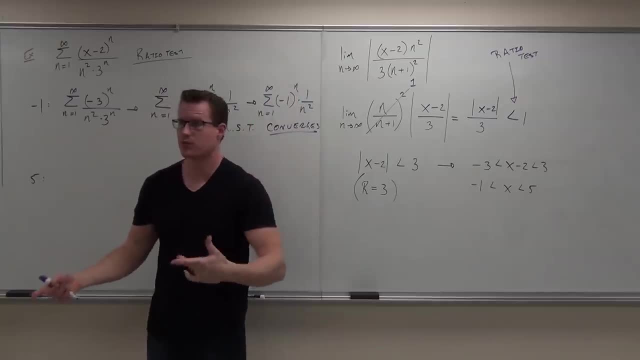 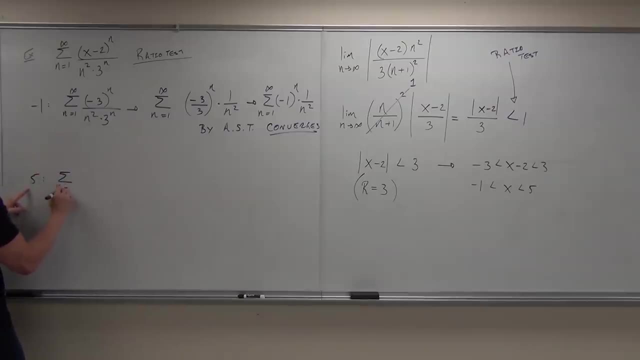 Because the absolute value of our series converges. our series is absolutely convergent. Therefore it is convergent Endpoint, no matter what is included, Number 5.. If we do that, we get N equals 1 to infinity, of 3 to the N. 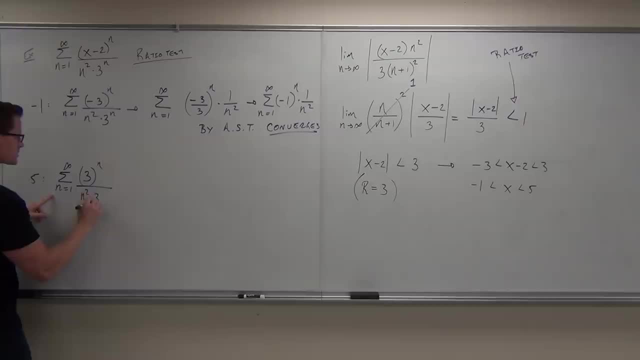 over N squared times? this one's even easier. How much is 3 to the N over 3 to the N? 1. Pshew, pshew, 1. 1.. 1 over N squared. 1 over N. Tell me something about 1 over N squared. 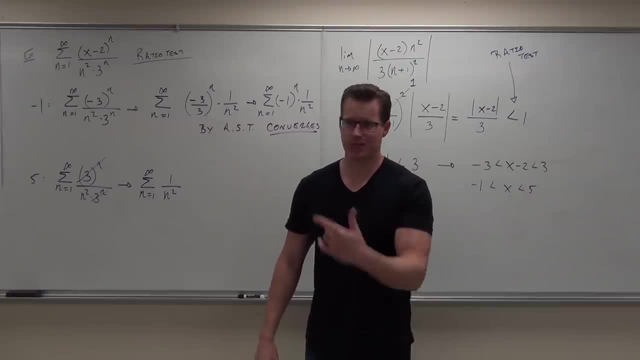 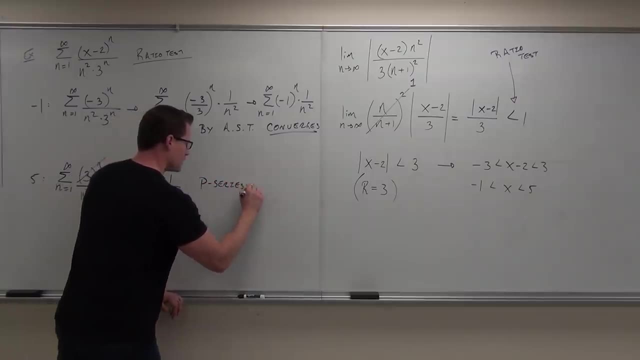 That's a P-series. That's a P-series. Say what now? That's a P-series. That's a P-series. Yeah, Tell me about the P-series. P equals 2,, which is greater than 1 minus. Oh, you guys are too fast. 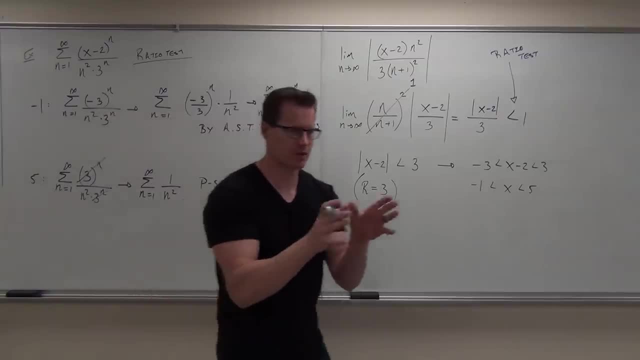 P-series. P equals 2, that's greater than 1.. Do you notice how what we're doing? Let's look at it- We're putting like everything we know together right. I'm going to go through it one time here, real fast, to show you what we're doing. 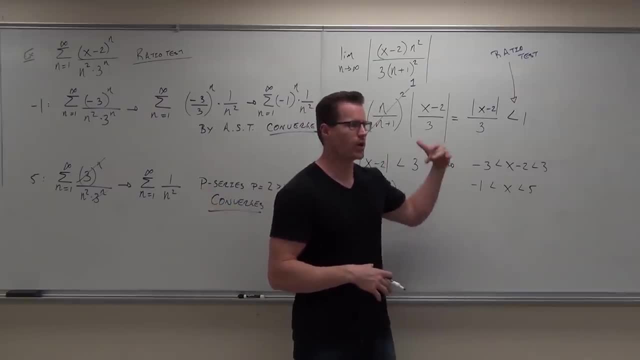 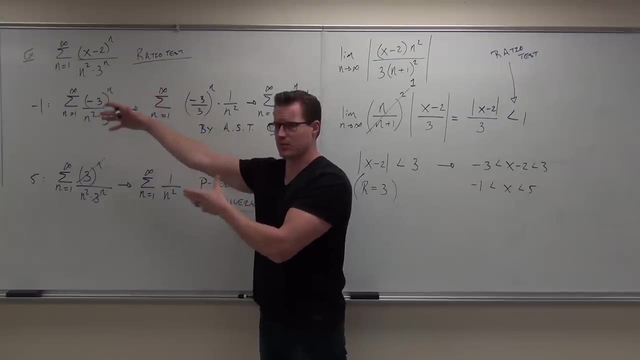 We're doing ratio tests to give us an interval that lets us know when our power series converges, when it represents a function. We're using all of the stuff that we've learned already to do our endpoints. We're saying, hey, alternate series tests, or absolute convergence, or a P-series. 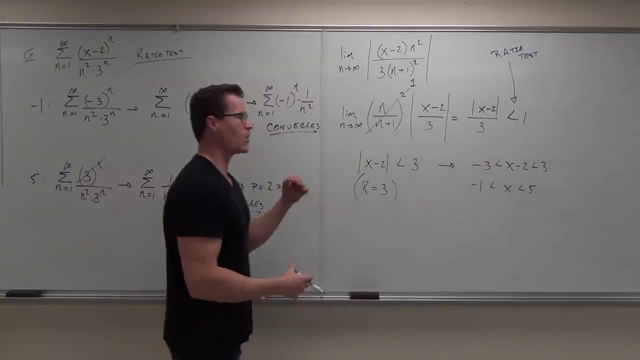 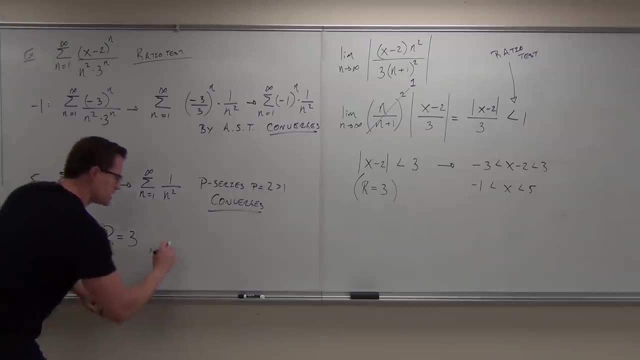 or a geometric or whatever. you have to show that our endpoints are or are not included. So here's what we got. The radius of convergence is 3.. The interval of convergence is negative: 1 to 3.. Negative 1 to 5, we've already had that. 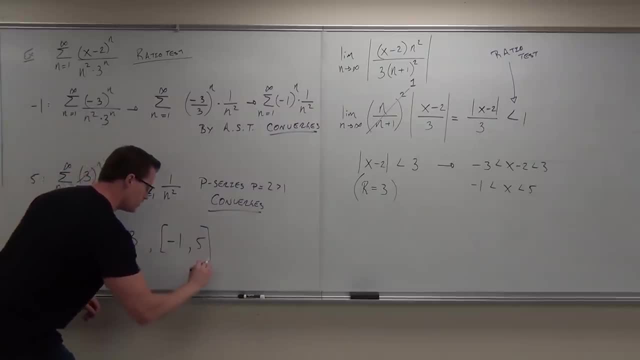 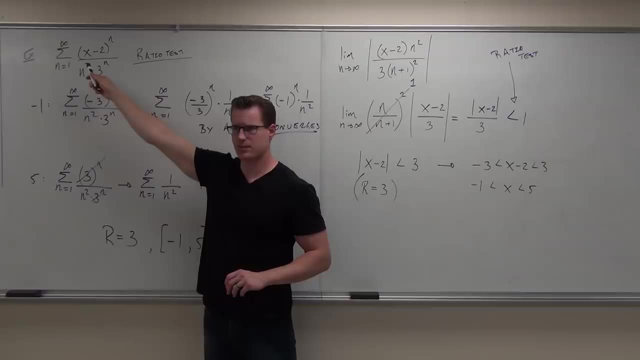 Now tell me about the endpoints. They're both brackets. That's what we're talking about. Here's what it means. It means that this series represents a function of X that converges for negative 1 to 5, and that's it. 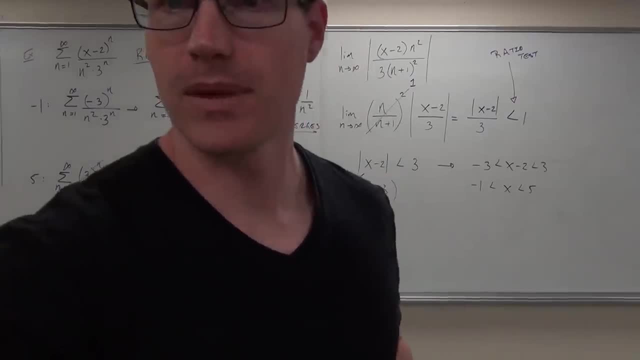 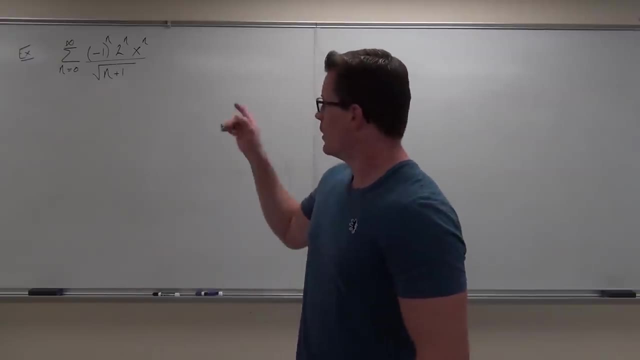 Make sense. Yeah, yeah, I'm sure, And that's what we're talking about. All right, so let's do it. The last example before we get on to the calculus of power series: from before we know that that right there, whenever we have an X raised to a power, 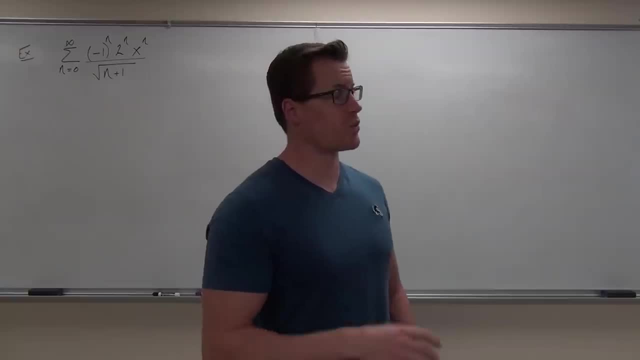 of X And we have this thing that creates a function of X. that's our power series. What we are focused on doing is how to find the interval of convergence, the raised convergence, where this thing converges. Firstly, notice something about this power series. 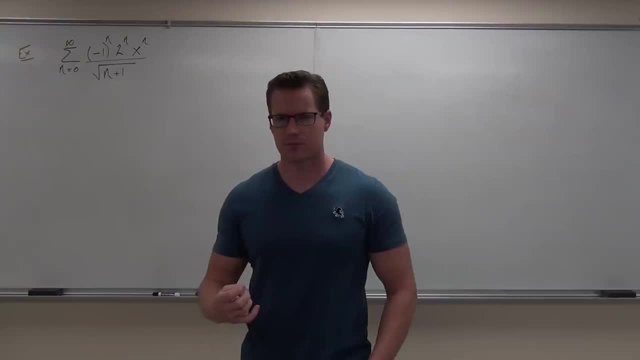 Where's the center? One right here. The center is at Zero, sorry, zero. Zero, that's right, Which means that whatever interval we get is going to be centered around zero, plus or minus some number, Whether that radius, that number is zero, infinity or actual finite number. 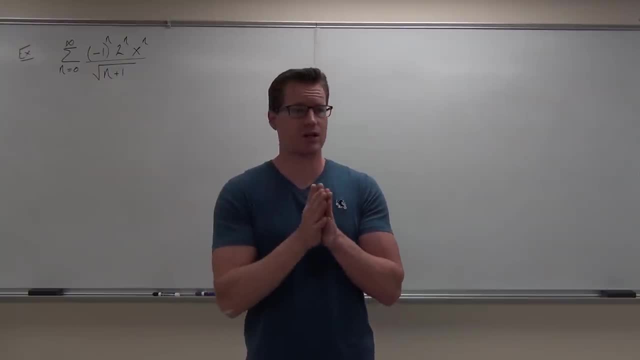 this interval of convergence is going to be centered right at zero And you found three cases so far- You found those cases on your homework- where it converges only when X equals zero and diverges elsewhere. That's the most limited, most limited amount. 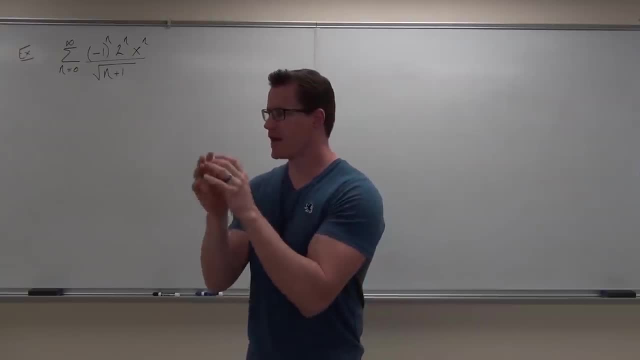 Does that make sense? You found the cases where it converges at the center and some radius around it, where that radius is a finite number, And then we'd have to check endpoints, of course, whether the convergence of endpoints or not. That uses the stuff we learned before. 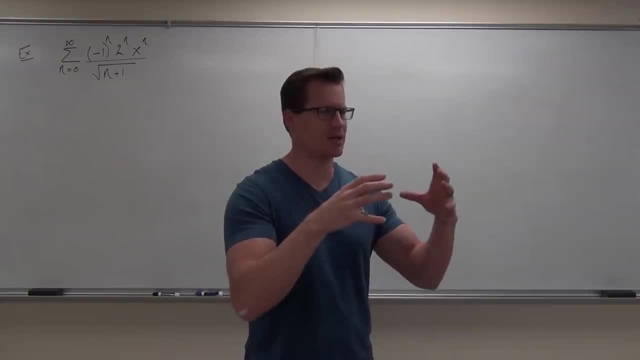 And then that's kind of the second case. The second case, The second least limited, And then the least limited is where it converges all the time for any X And hopefully, if you've done your homework or some of it, you've seen all three of those cases. 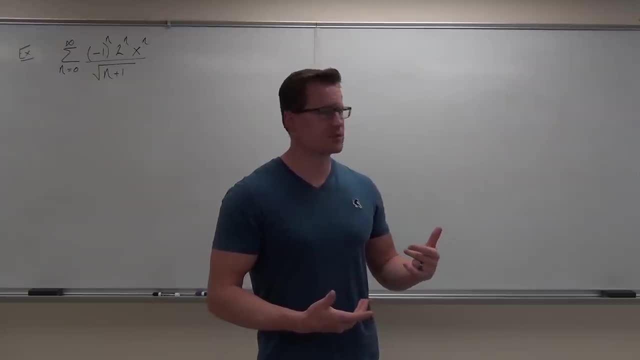 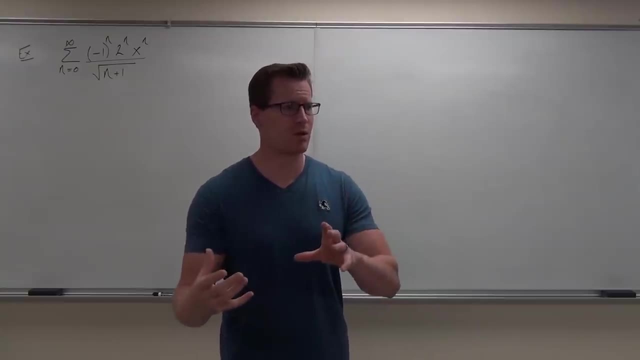 Have you seen those cases yet? By the way, I do want to see where these things converge. They will converge somewhere, Okay, I want to see that. I want you to, even if they go. it diverges when X doesn't equal zero. 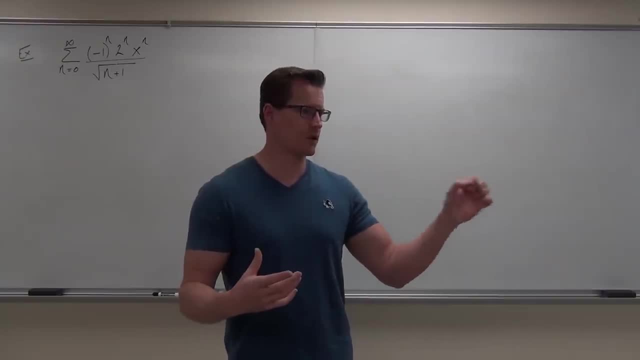 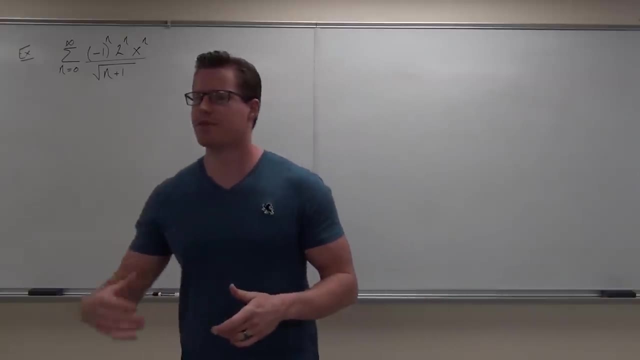 I want to see it converges when X does equal the center, wherever that happens to be. Does that make sense? Okay, so our last example says: all right, if that's a power series, let's go ahead. let's find out what the interval of convergence is, what the radius of convergence is. 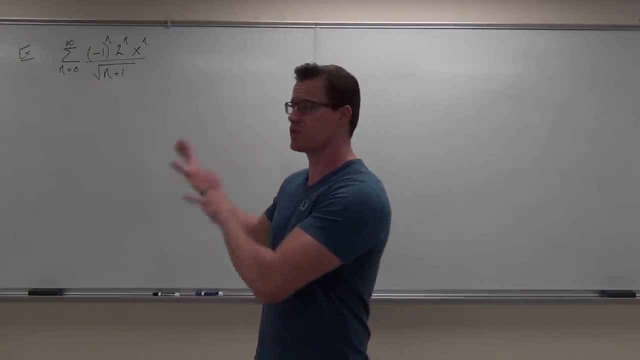 what's going on with this thing? How are we going to do that? most of the time with this, Yeah, usually it's a ratio test or maybe a root test, But you want some test that lets you determine the interval or the radius of convergence. 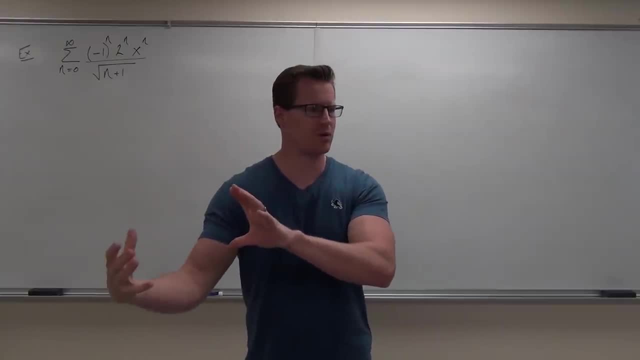 that says, hey, it's going to converge when this is less than some number, when this happens, Because that gives us that interval. So let's go ahead and let's start. Do you guys want to try this one on your own? 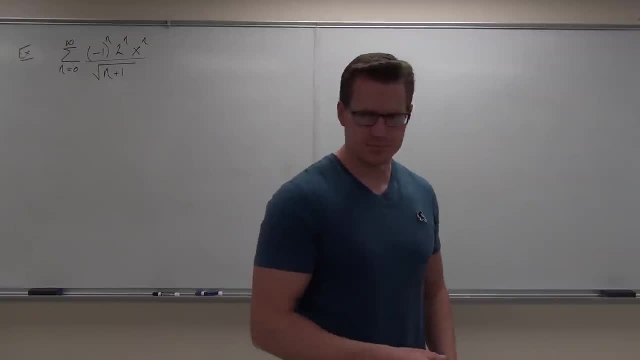 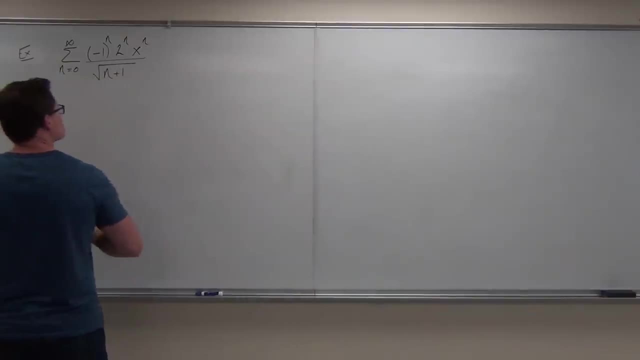 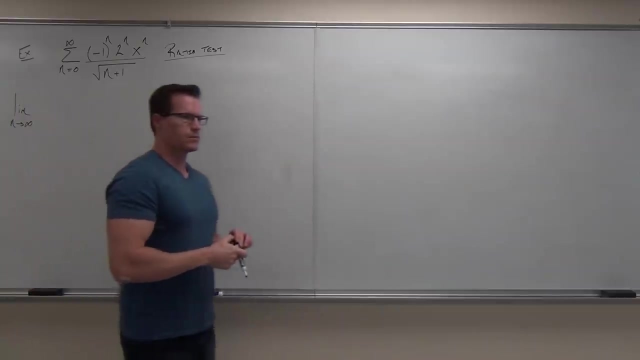 See if you can do it. Let's start with the ratio test. Write out the ratio test And see if you can do it. As you're working through this, can you tell me some of the key points about the ratio test that we need to know? 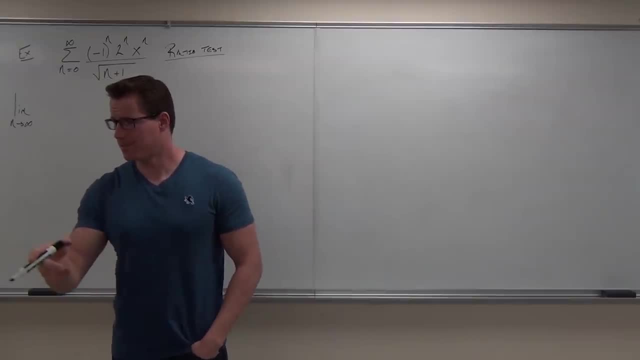 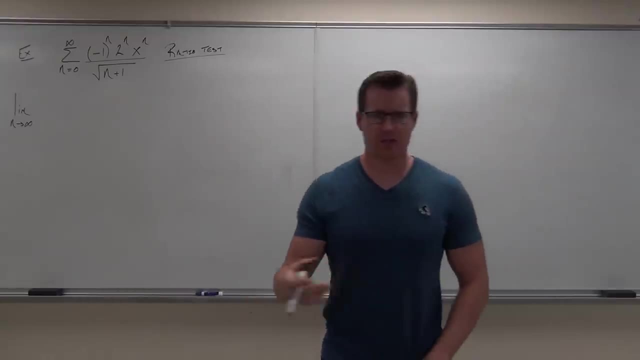 Yes, we need to know. Say what now It would take away the. It would. Why? What part of the ratio test takes away the negative 1? The absolute value? Okay, So the ratio test has absolute value in it. 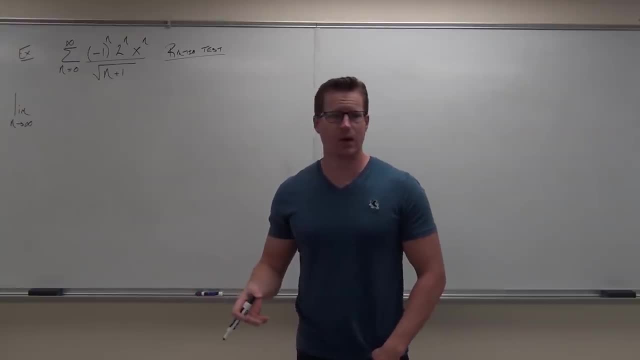 No problem. What are some other key points about the ratio test that we need to know Specifically what goes in the main numerator: The a sub n or a sub n plus 1? a sub n plus 1.. Okay, That's pretty good. 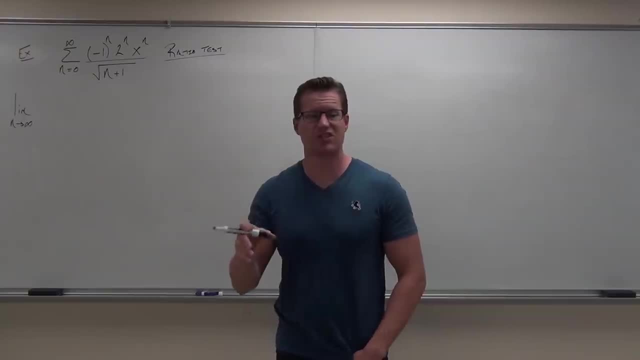 Do you know anything about the convergence of the ratio test? When does the ratio test converge? When the limit is less than 1.. Very good, When the limit is less than 1.. And it diverges when the limit is greater than 1.. 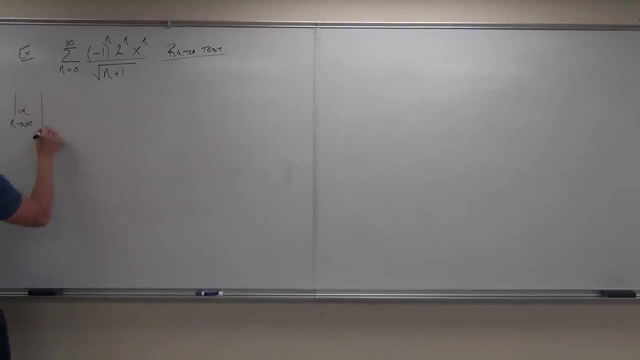 All right, this is going to be a nasty one, isn't it? Let's see if you all got this. We got negative 1 to the n plus 1.. We got 2 to the n plus 1.. We got x to the n plus 1.. 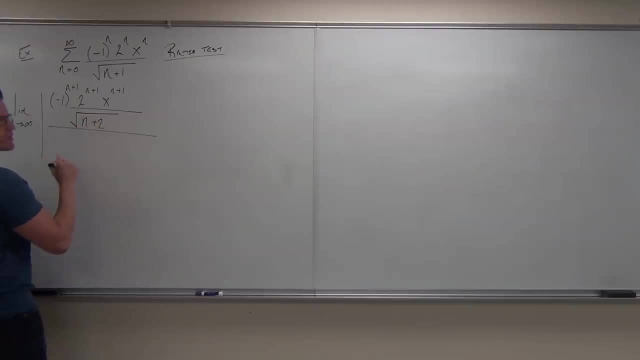 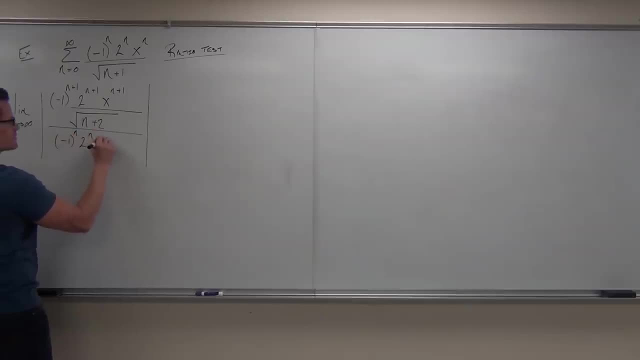 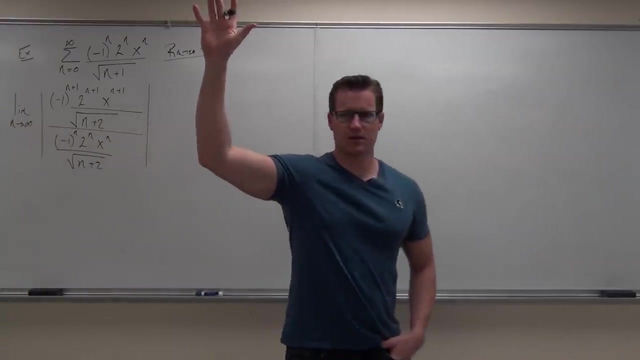 So negative. 1. Negative 1 to the n- not a problem. 2 to the n. x to the n, square root of n plus 2.. Show of hands, if you made it at least that far, I'm sorry. n plus 1.. 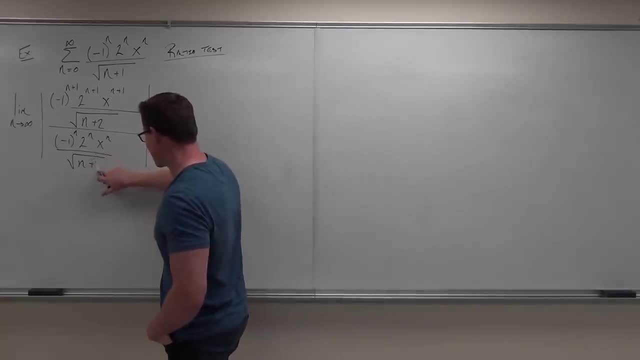 Hopefully you didn't make it that far. I just like 2's today, n plus 1.. Did you make it that far? Yeah, Fantastic, That'll let you know the ratio test. All right, So now, what do we do? 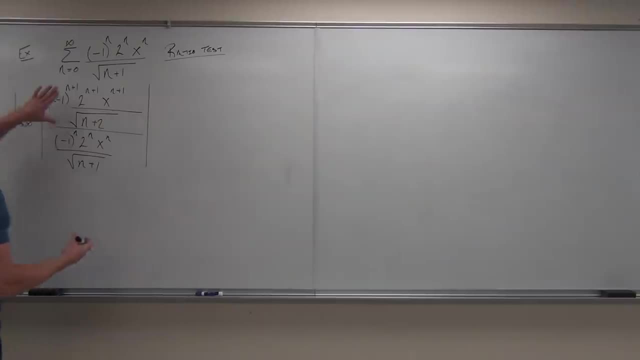 Simplification As much as you can. So simplification means get rid of your negative 1 to the n plus 1's, or negative 1 to the n plus 1's, All right. And then, because absolute value gets rid of those things, 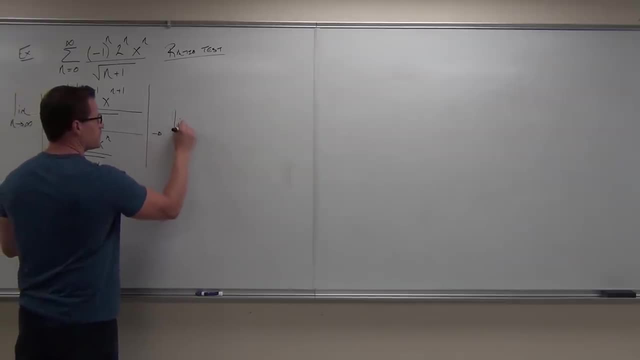 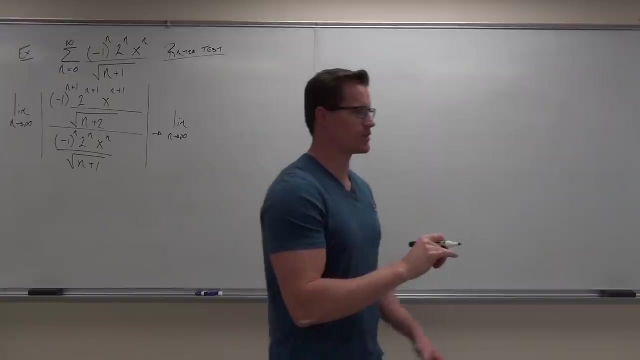 It also means take your complex fraction and rewrite it. Do I get rid of my absolute value with a ratio test in a power series? Not generally, unless you have something like x squared where it doesn't matter, Sure, But not generally no. 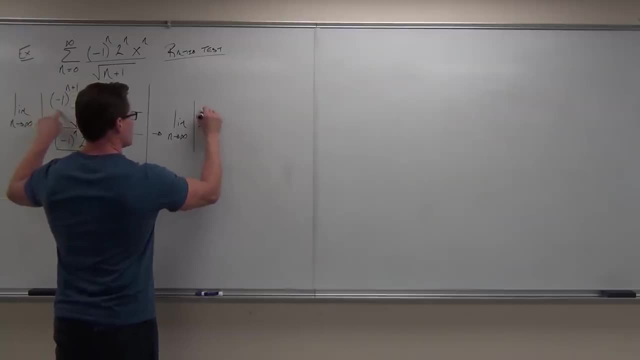 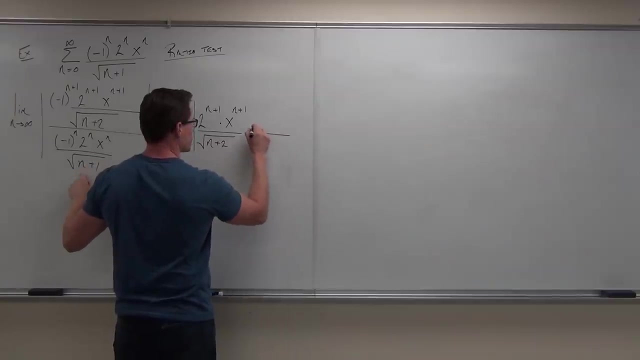 So we're going to have the absolute value. still, We'll have 2 to the n plus 1 times x to the n plus 1, all over square root of n plus 2.. Okay, times the reciprocal of our main denominator, That would be the square root of n plus one over. 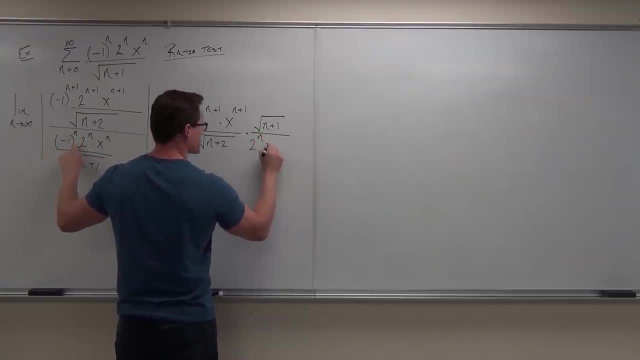 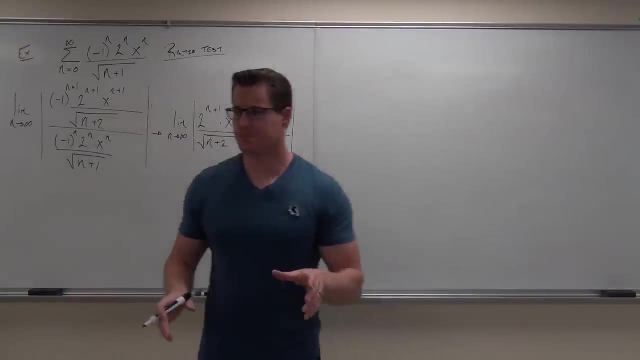 well, the negative ones, those are gone. Our absolute value does that for us. We get that. Did you get that far on your own? Yeah, Okay, now, before you go any further, what are we gonna do? Simplify. 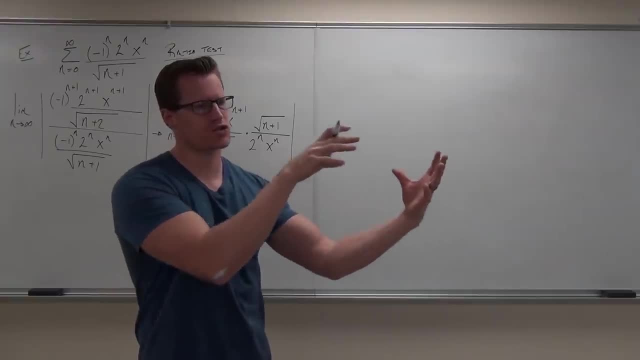 Yeah, as much as you can Simplify. and then, after we simplify, we're gonna strip off our n terms and leave our x terms. We're gonna separate those things. So when we do this, I'm gonna go through it quickly- 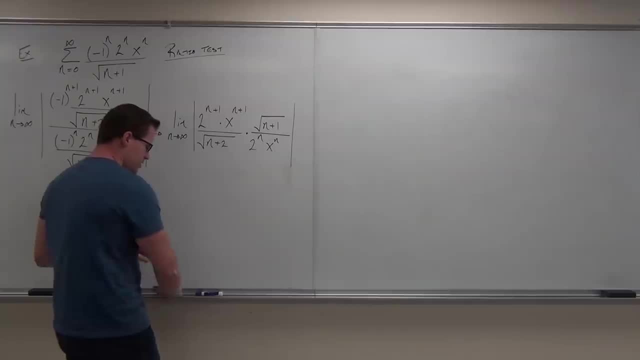 I've already explained it a few times to you. When we simplify, you're gonna have a lot of common bases raised to different powers. Just understand that a plus one simply means you're multiplying by two. A plus one here means you're multiplying by an x. 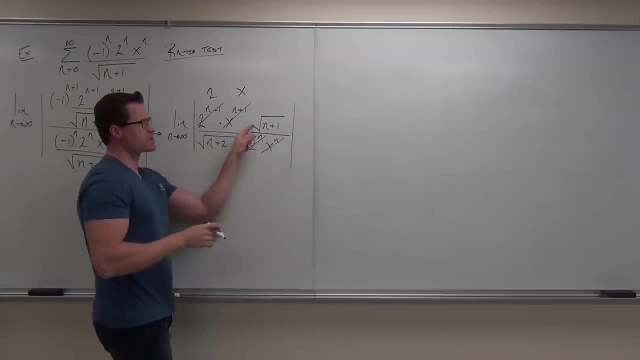 So what we're gonna do, we're gonna collect our n terms. If you notice this, there's a square root of n plus one over square root of n plus two. I can make a big square root of n plus one over n plus two. 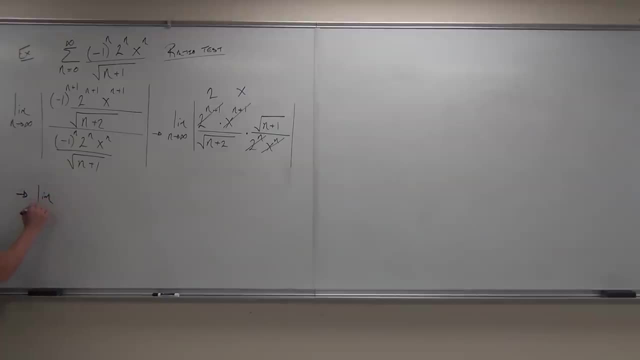 And we're gonna do that. So n plus one, n plus two as the radicand of our square root. And then we got what else is up there: 2x. Absolute value of 2x, 2x okay. 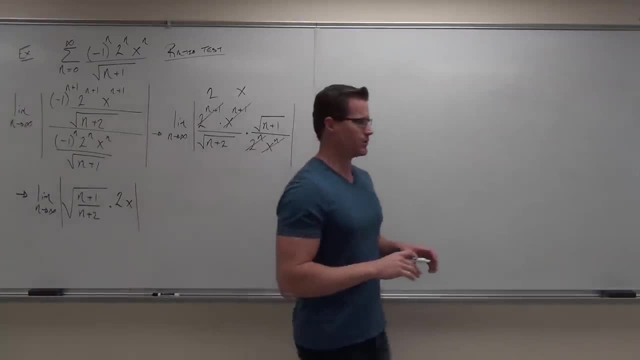 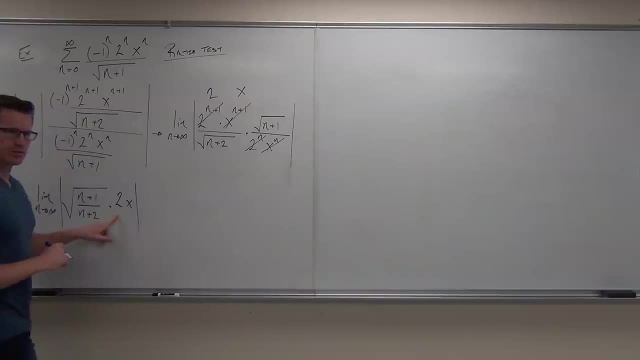 If this is all in the absolute value, tell me, what do I do? What can I pull out of the absolute value right now, because it'll never be negative? The square root- Good. How about the two? Could I pull that out? 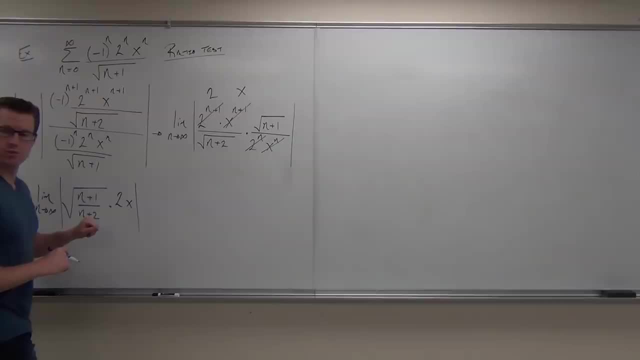 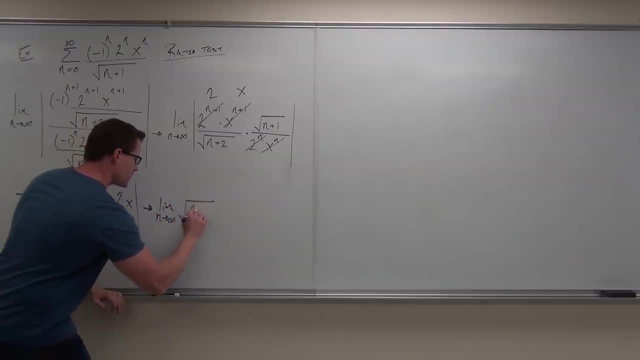 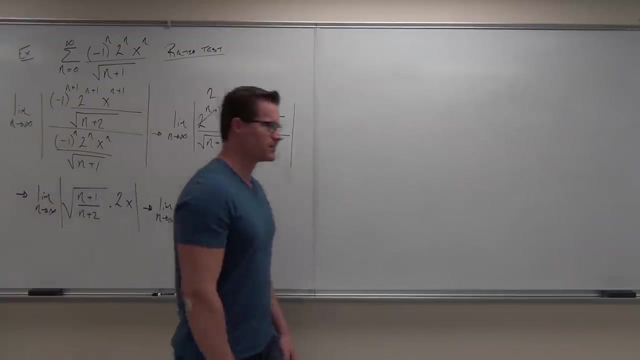 as n approaches infinity, of the square root of n plus one over n plus two times, two times the square root of x. I could do that, We absolutely can. Absolute value of x. What did I say? Square root of x. Oh man, sorry. 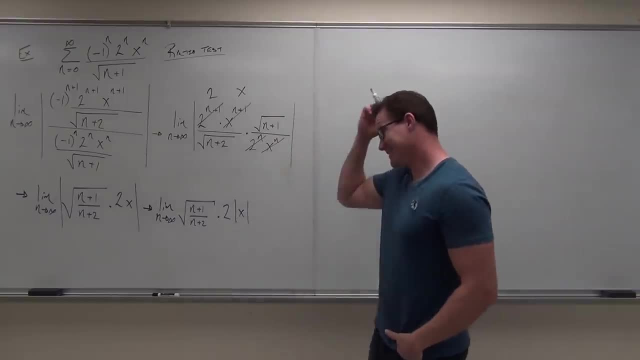 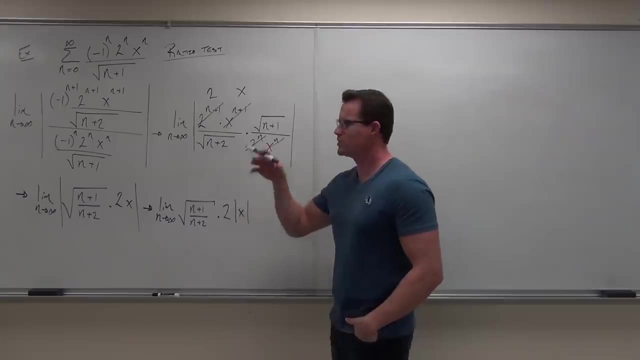 Too much painting, I told you, Frank, kinda Hm, My bad. So square root of n plus one. I just like square roots and twos today, Don't worry about it. Square root of n plus one over n plus two times two. 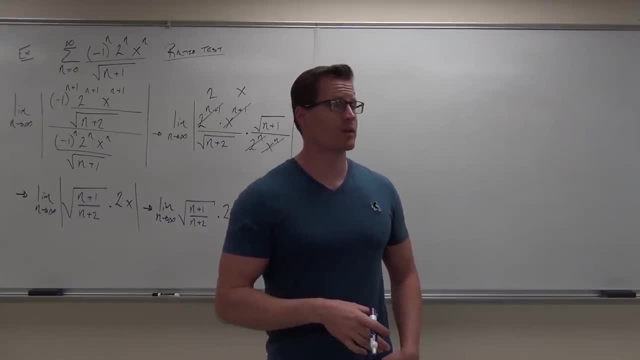 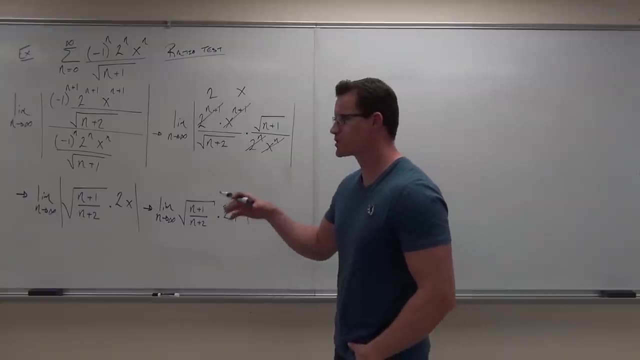 times the absolute value of x. Oh my gosh, Tell me one more thing that we got here. What's going on? The limit, The limit, What's the square root of n plus one over n plus two, as n approaches infinity inside of our limit? 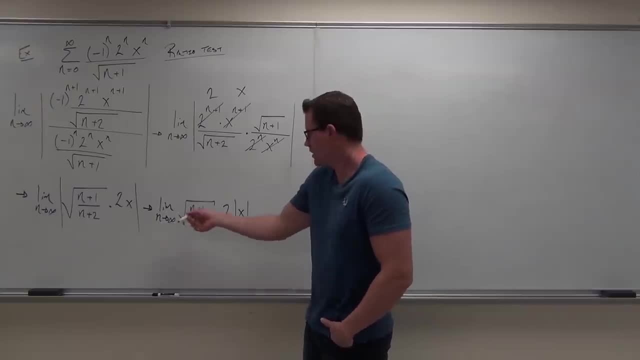 What's this? do One, Yeah, use all this stuff about limits that you know N over. well, if you divide by the largest power of n or you do a low B tolls inside your square root, whatever you want to consider this. 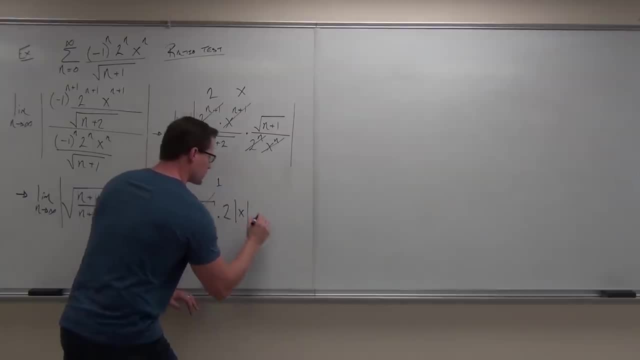 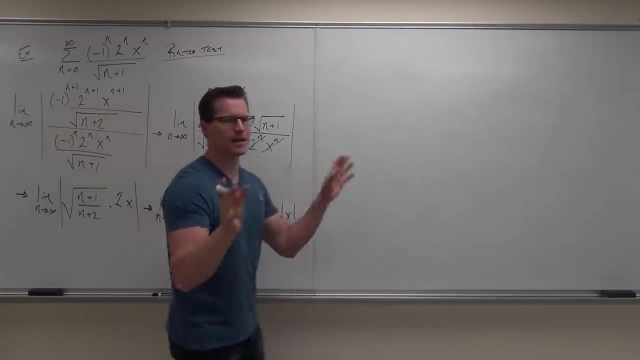 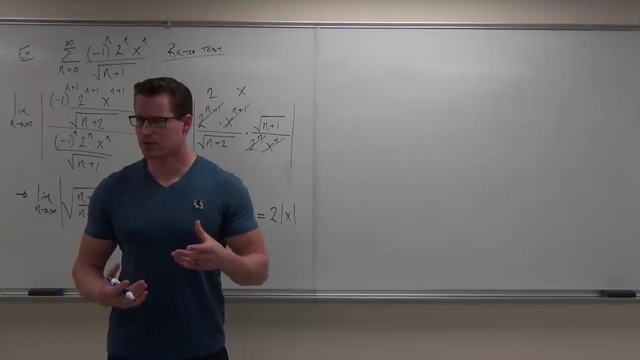 this whole thing goes to one. So what's our limit? equal, Very good. Okay, let's put the whole thing together now. What test did we just use? The ratio? And when do we know that the ratio test converges When the limit is less than one? 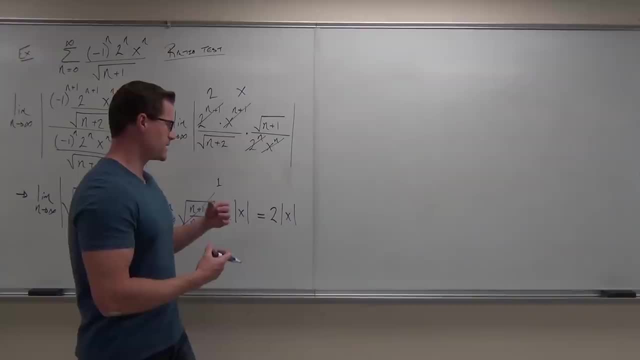 When the limit is less than one. So if we just use a limit and say, hey, you know what, We use ratio test to find our limit and we know that when the limit is less than one, we know that this power series converges. 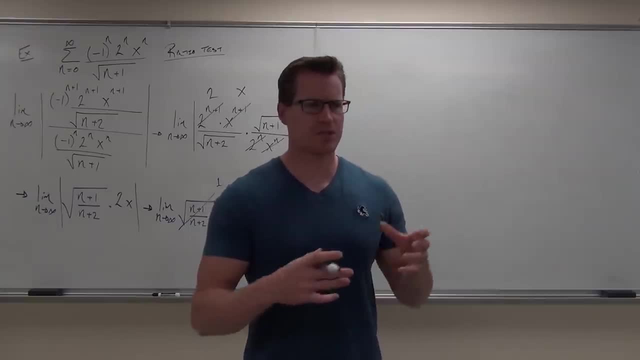 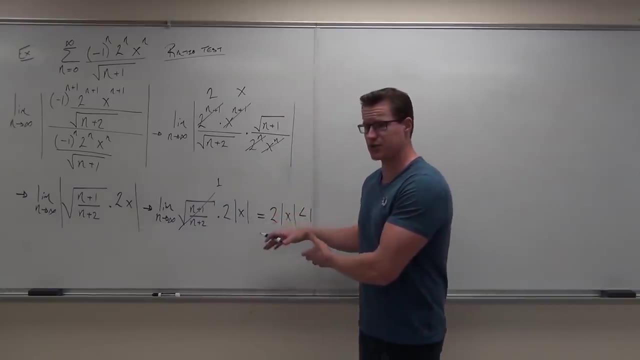 Remember that a power series represents a function only when that power series converges. So that's the whole idea here. behind you is the ratio test is we want to find out when that actually converges. so we know the domain of our function, the domain of our function. 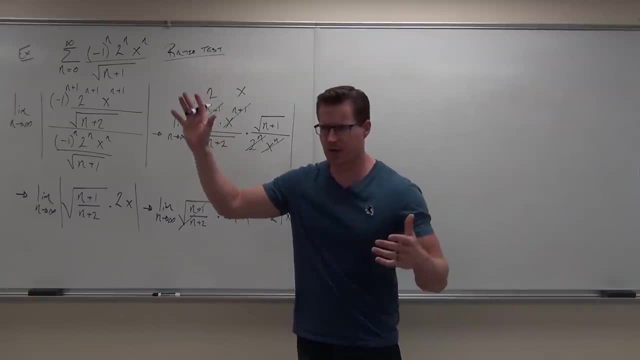 for which our power series converges. So if you guys feel okay with that idea- I know we've explained this a couple times- I want to make sure you're with it. Do I stop here? No, No, but we're getting there. 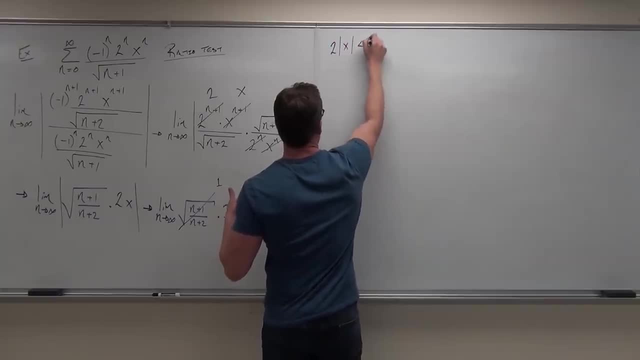 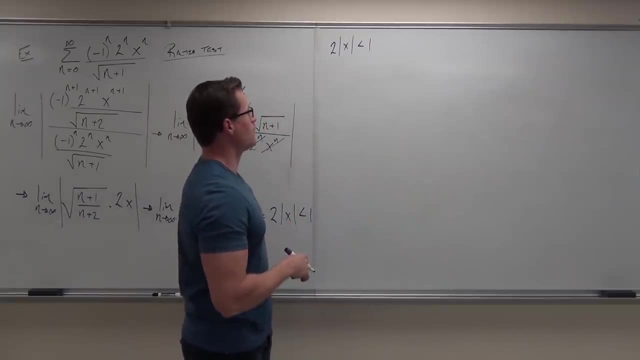 What we know is that two absolute value- of x is less than one- gives us our interval of convergence for our power series, for which our function will define that. That's our domain. Now, what we do here is we're always trying to find. 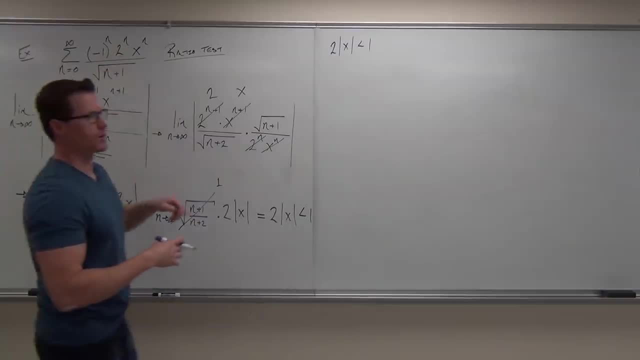 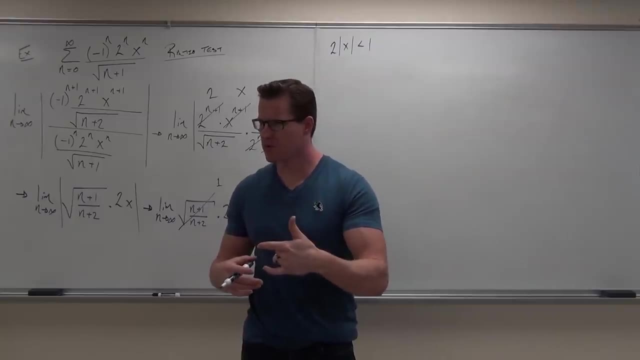 the absolute value of whatever is being raised to the nth power, isolated all by itself on one side of our inequality. What that does, that will give you your radius of convergence. Have I told you that before? Yes, So what you're looking for here is: 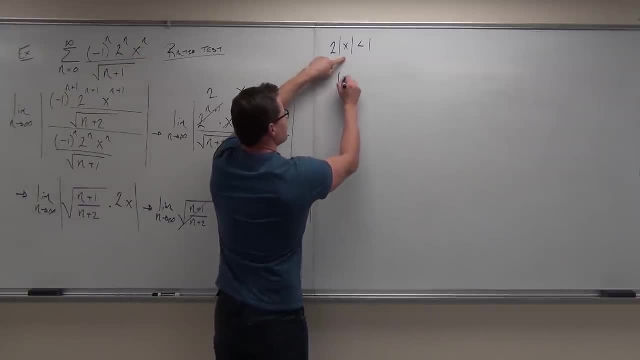 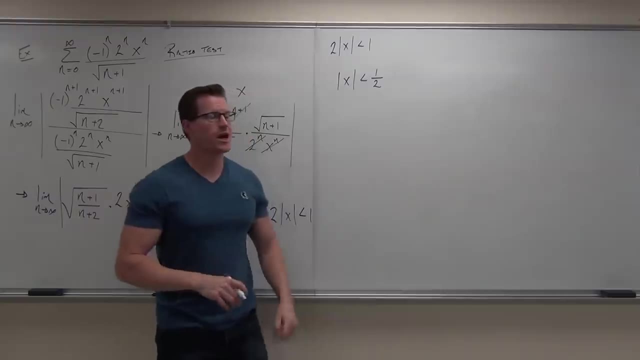 hey, if it's x to the n, I want x all by itself inside of an absolute value. on one side of my inequality I divide by two on both sides. That right there. as soon as you isolate, they go. oh cool, look at that. 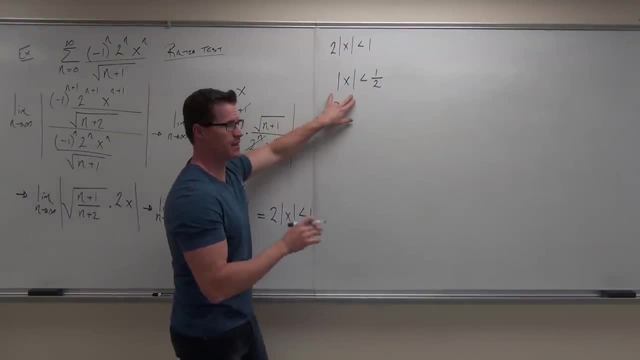 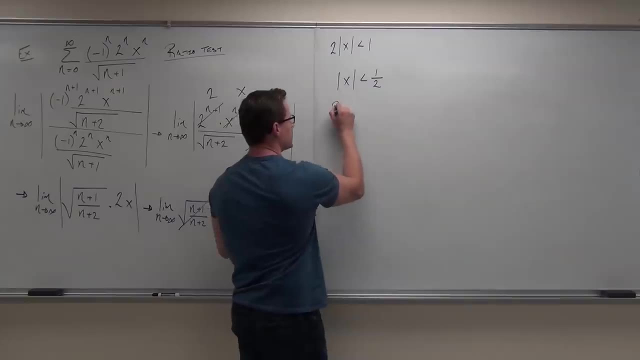 Hey, this is what's being raised to my nth power. It's isolated. since I'm inside my absolute value Right now, you should be able to tell me the radius of convergence. What is it? Very good. So this right here says: 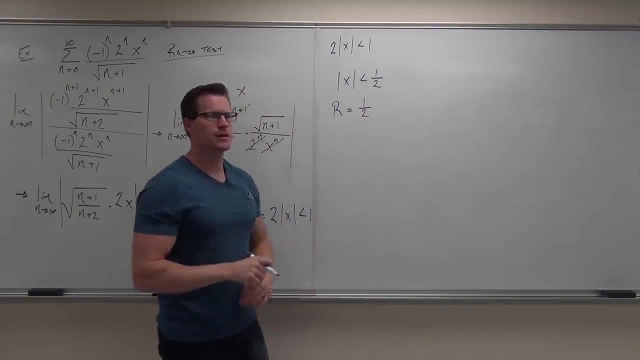 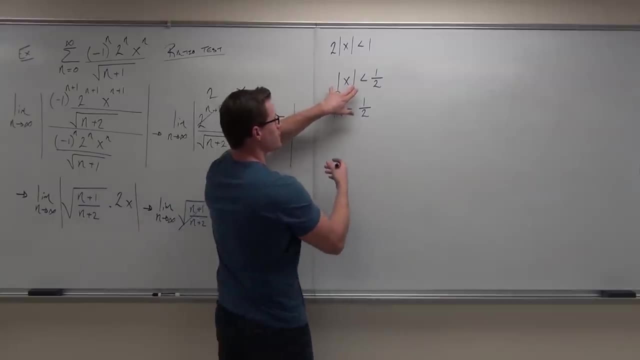 the radius of convergence is one half. Now we keep going a little bit. We write out the definition of what an absolute value inequality is. Absolute value inequality says if you have the absolute value of x less than one half, that means that negative one half. 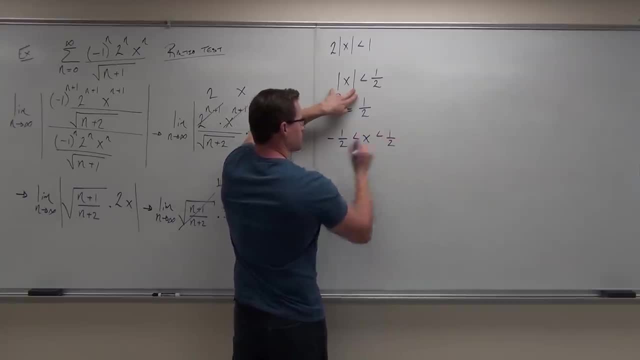 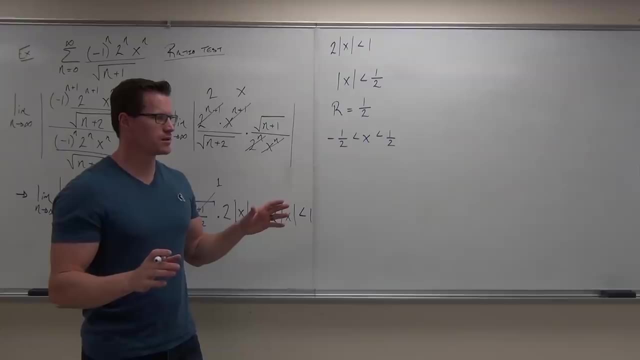 is less than x is less than one half, And we're almost done. Are you guys okay with that one? Yeah, Almost done. What do we do next? Check endpoints. We gotta check those endpoints Because right now, yeah, we have the radius. 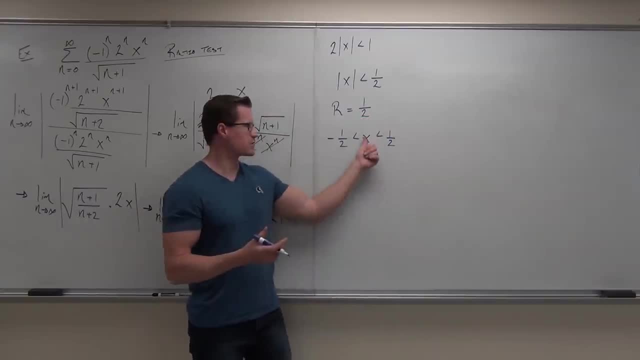 We know it's gonna be one half. We have the center. Notice how the center zero is right between negative one half to one half. What we don't know is whether these two endpoints are included or not. That doesn't give us this with the ratio test. 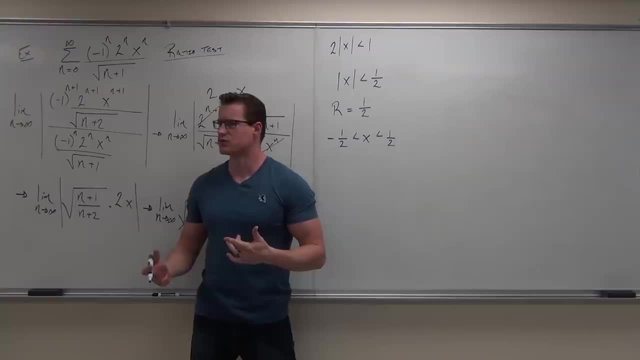 It doesn't give us it by just doing this simple mathematics. We gotta check the endpoints Individually. Where do we check the endpoints? Say what The original point? Original point. So plug it in. Let's see If we plug in. 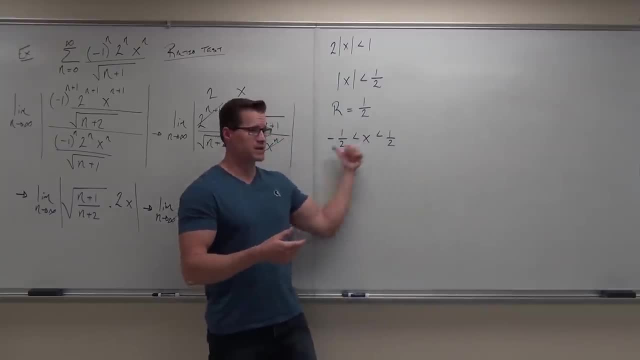 where do we plug in the one half and the negative one half? It seems that way right, Because x is between those things. So if x becomes negative one half, we're gonna find out whether that converges or diverges for that specific endpoint. 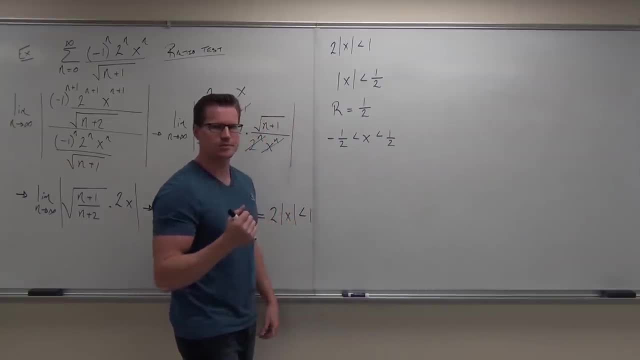 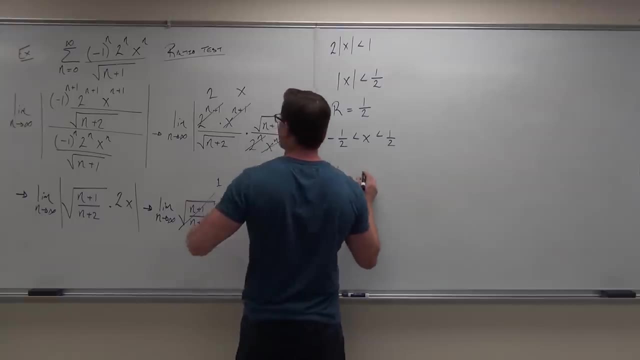 Same thing with positive one half. Which one do you guys wanna do first Negative, Okay, negative one half. Does it matter? No, No, We just have to go left to right. So if we're gonna check the endpoint, negative one half. 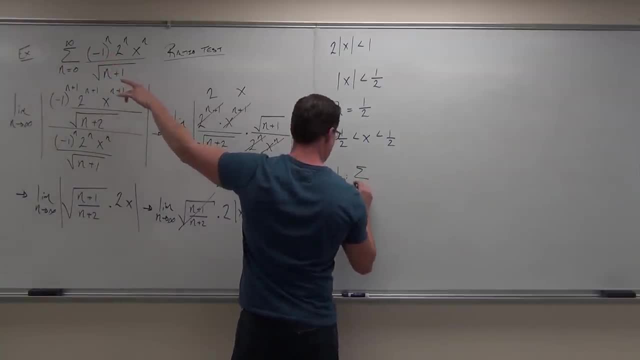 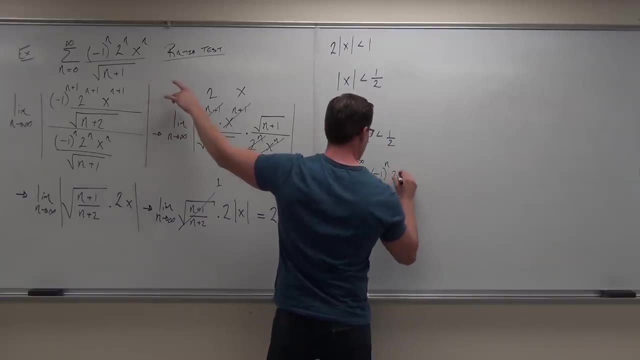 we're gonna plug it in here and get a series- n equals zero to infinity- of negative one to the n. We're gonna have two to the n And we're gonna- what's the next thing? Negative one half into the n. Yep. 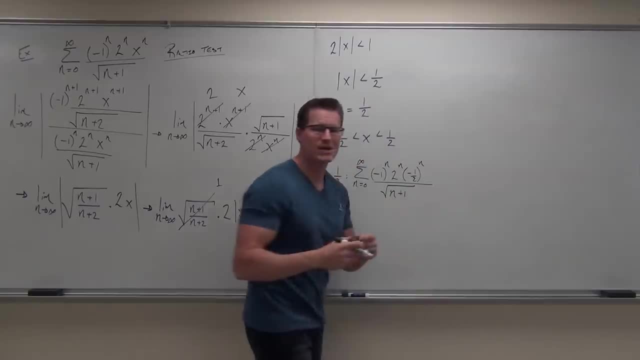 All over the square root of n plus one. Now, because you did all that stuff in the previous sections, these ones should be pretty easy. These are gonna be nice, These things that you recognize, You go, oh yeah, we can do this with it. 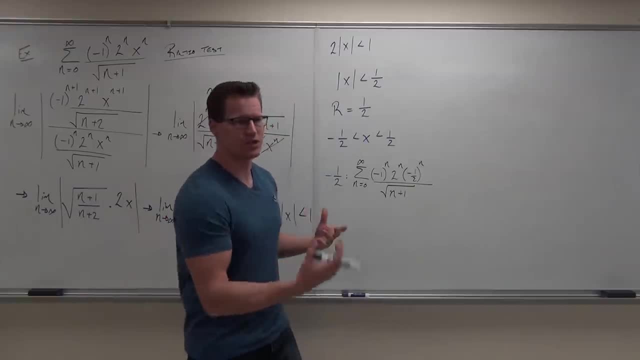 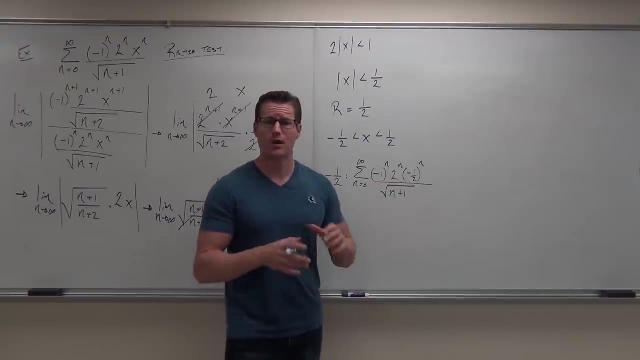 We can do alternating series tests or absolute convergence, or we can do another ratio test if you really really want to, Or we can do a p-series or a limit comparison test. All those things open up right now because we don't have any more x's. 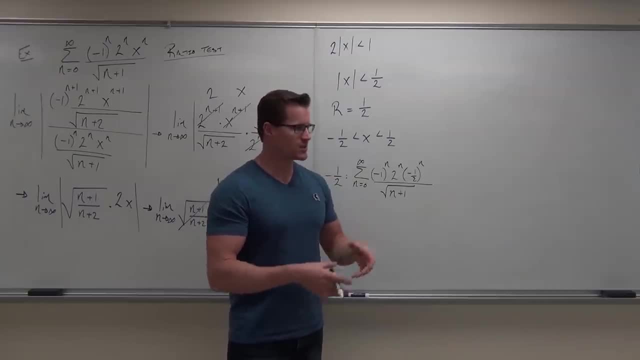 We have all constants, So simplify before you check them. but it's gonna be something familiar. So here's how I would look at this. one Nth power, nth power, nth power. Do you see if I can make all those things to one nth power? 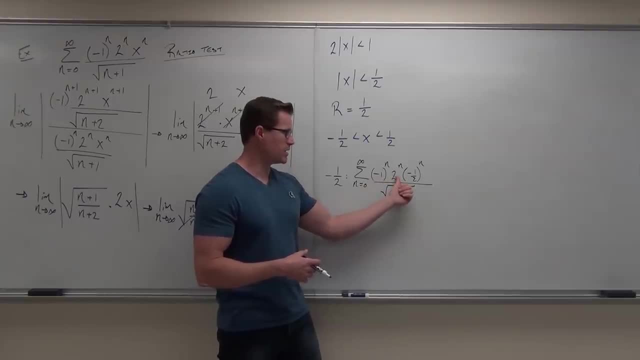 Well then we have negative one times times two times negative 1 1⁄2.. How much is negative one times two times negative 1 1⁄2? One Positive one. So this whole thing gives us a series from zero to infinity. 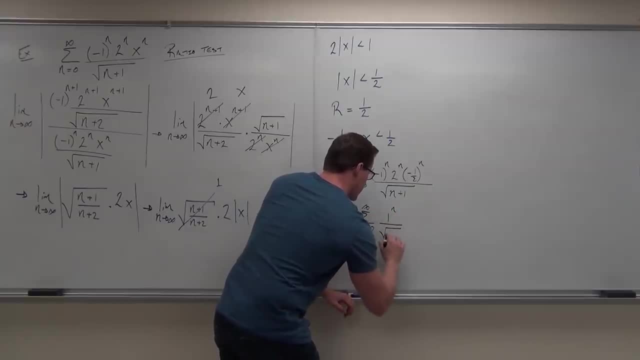 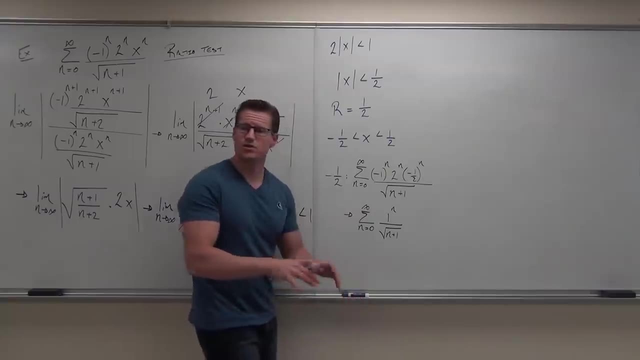 of positive, one to the n over the square root of n plus one. Okay, well, wait a minute. How much is one to the n One? So, no matter what the, do you guys notice that when I have a negative times, a negative that gets rid of that idea? 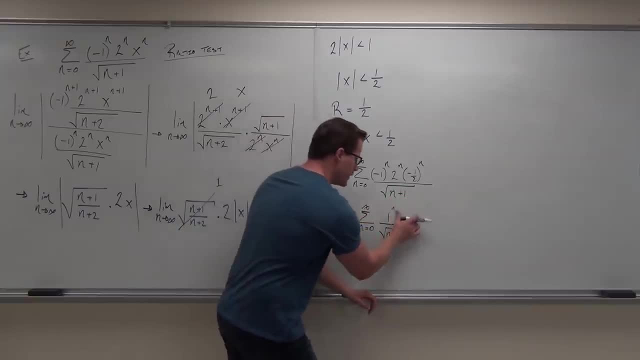 of an alternating series. This is not alternating, It's just one to the n or simply one all the time. So we don't need that n anymore. Now tell me something about this series. Can you work with it? Can you do something with it? 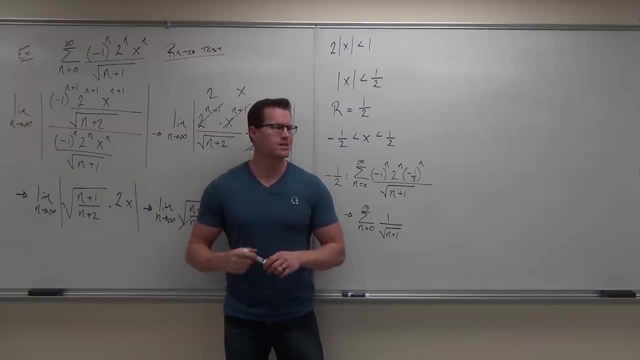 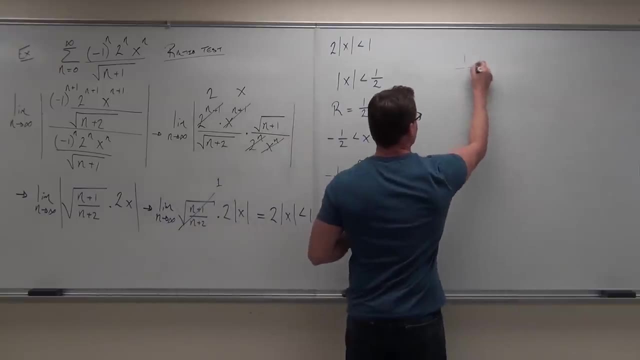 Okay, if we compared it. please listen carefully. I wanna walk you through this because I don't want you wasting your time. You need to think about it and I like that you're thinking about it. But if you compared it, this is less than one over square root of n, correct? 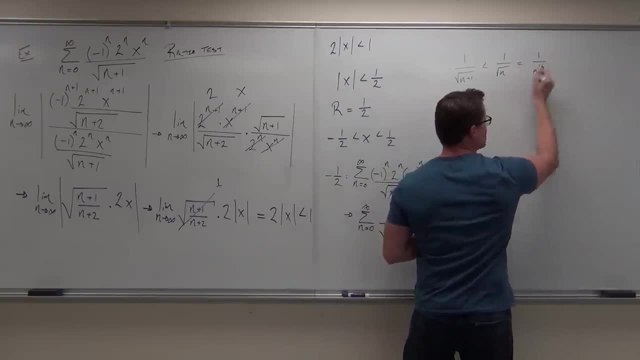 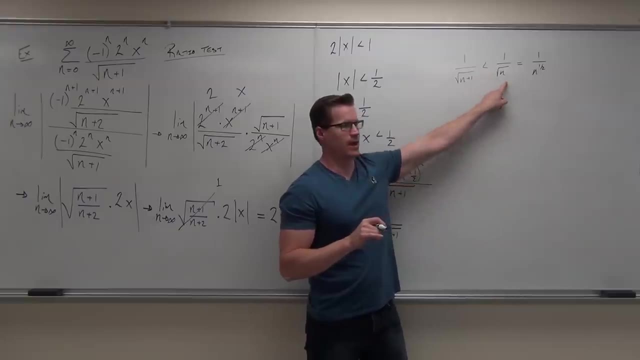 Yes, And this is one over n to the one half, which is a divergent p-series. Are you clear on that? Yes, This thing diverges. This is less than that. Does it tell you anything? No, This is inconclusive. 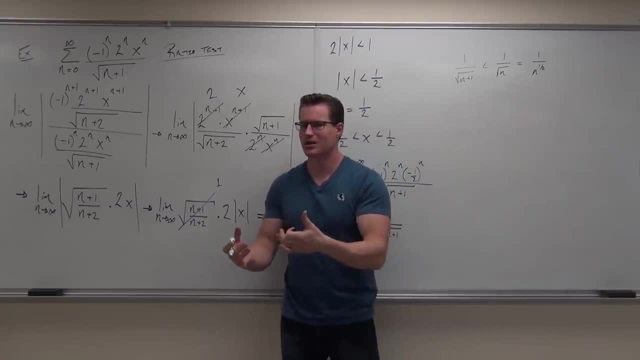 That does not help us at all. So even though we can compare it, we're comparing it to something that is bigger and divergent. That doesn't make sense. We want bigger and convergent. That would be great, But this is not that. 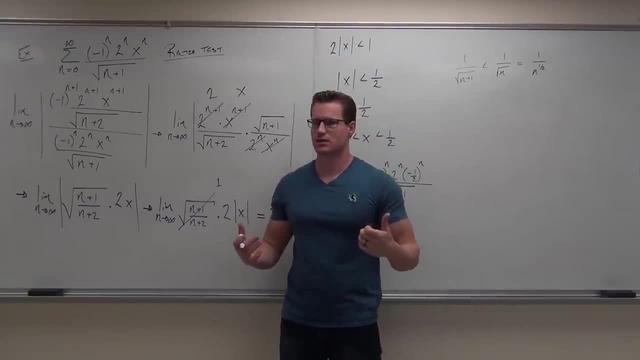 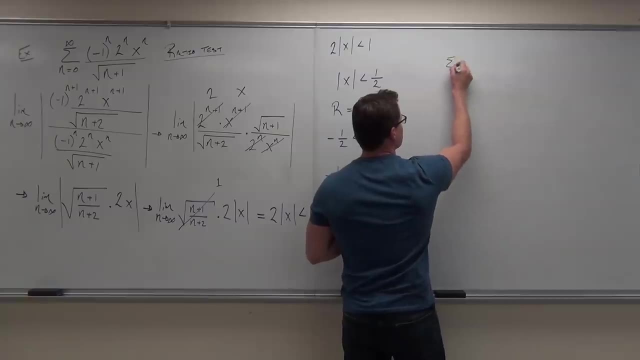 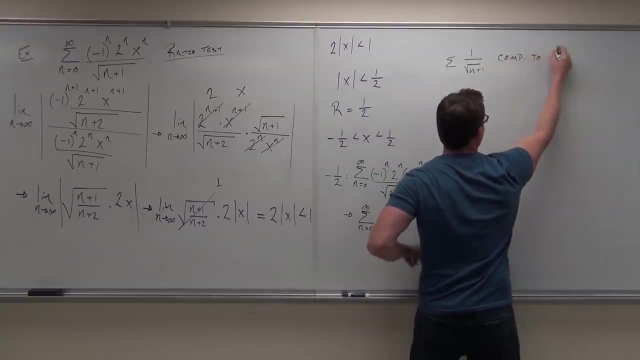 Does that make sense? Could you use a limit comparison test? That you could do. If you did a limit comparison test, then the series of one over the square root of n plus one compares to the series of one over square root of n. 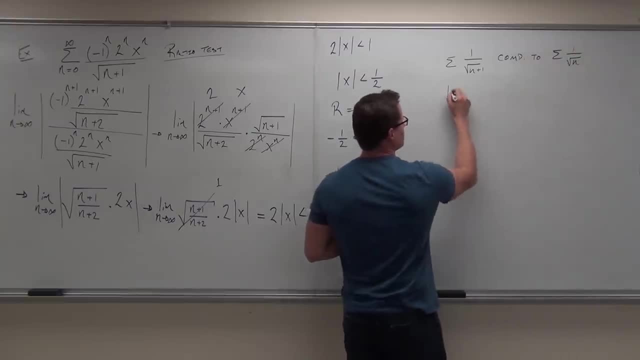 Sure, No problem. If you did the limit, since these both have positive terms, we'd have square root of n plus one over one, over square root of n, as n approaches infinity. This should kind of be old hat for you, right? 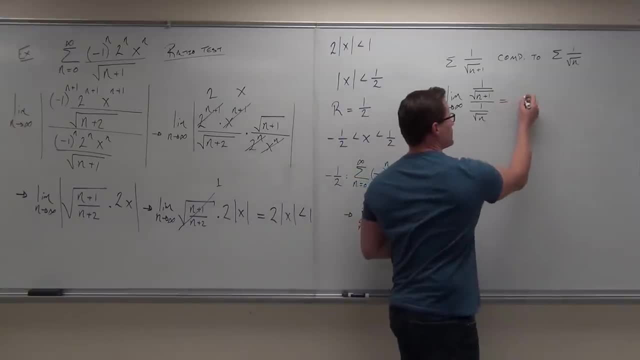 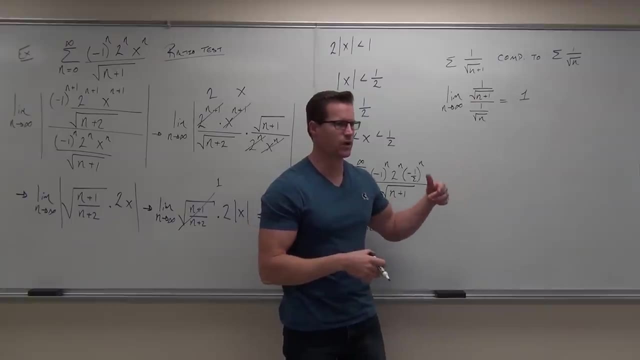 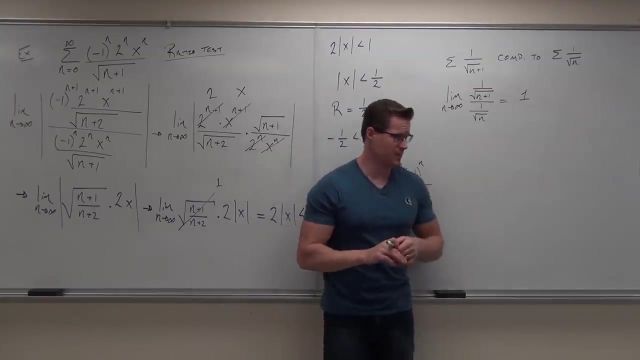 You guys have seen this before I know, And this would give you one When you work through it. that's going to give you one Quick head note, if you're okay with that one. Now next question: If that gives you one, this is a limit comparison test. 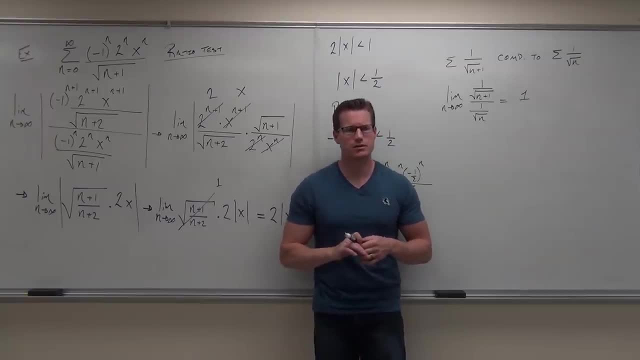 is that inconclusive or do you know something about this? You know something? You know something With a limit comparison test? if the limit equals a number, I don't care what it is, if it just exists, if the limit exists. 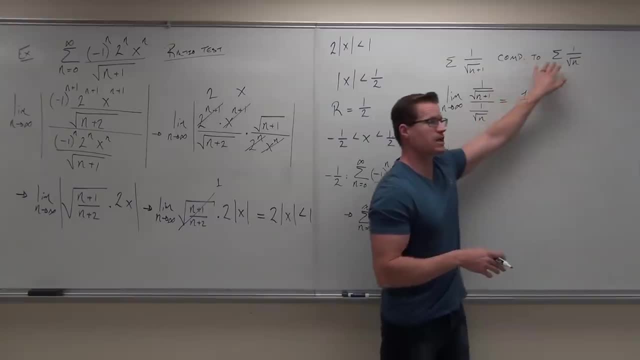 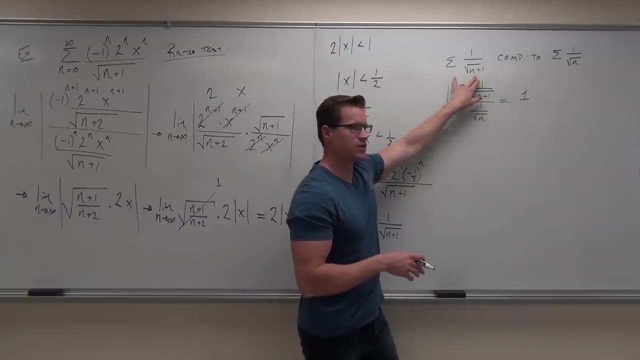 then it's a limit, Then both of these series have the same result. Tell me something about this series. Tell me something about this series then. So by the By the comparison, Very good. By the limit comparison test, we said this: 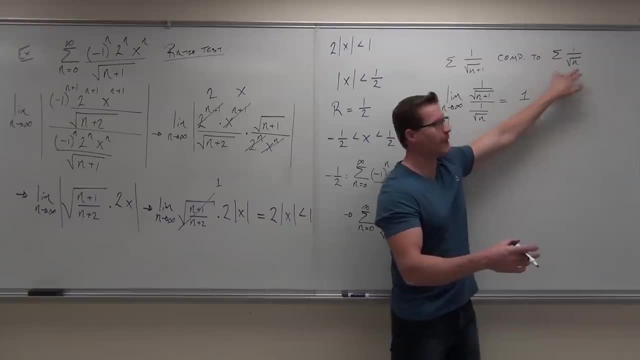 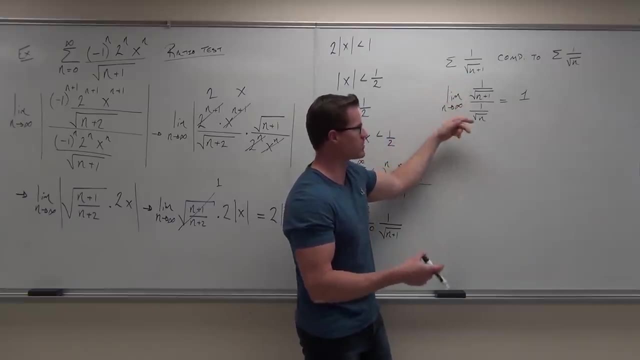 All right, This one acts just like that. Think of the end behavior of your function. This one acts just like this one. If I compare them in a limit, a limit comparison test, compare them in a limit and that limit exists. 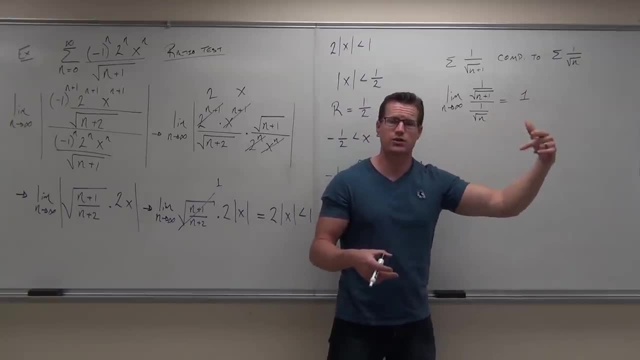 they both have the same result: If one diverges, the other diverges, diverges the other diverges. If one converges, the other converges. So we base this, our given series, on a series we already know the result for. 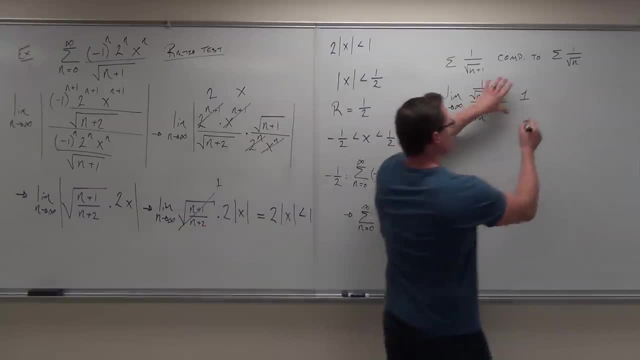 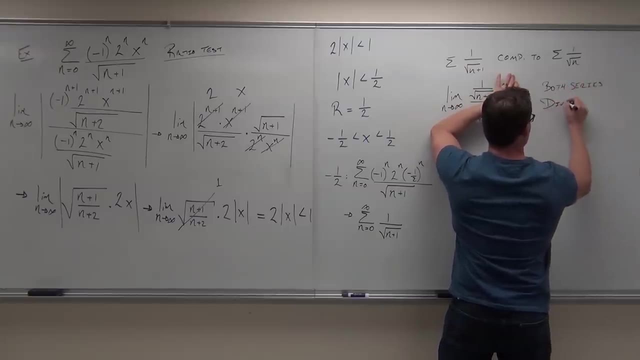 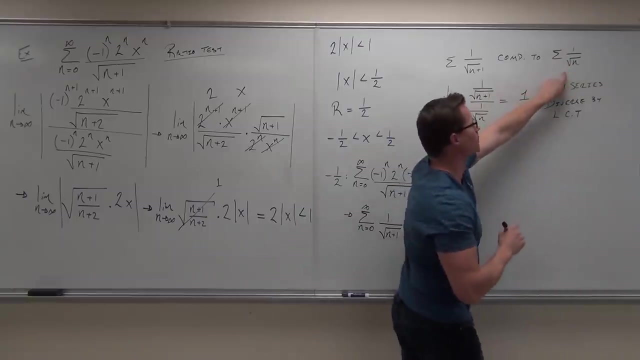 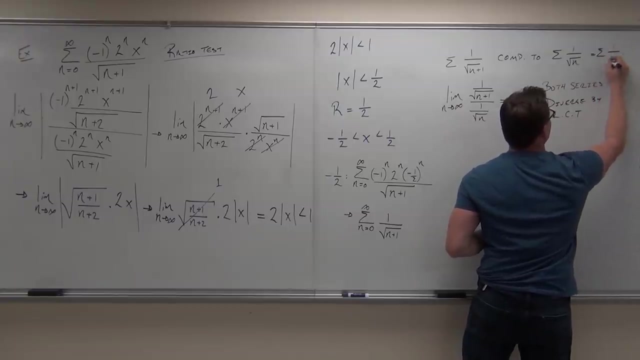 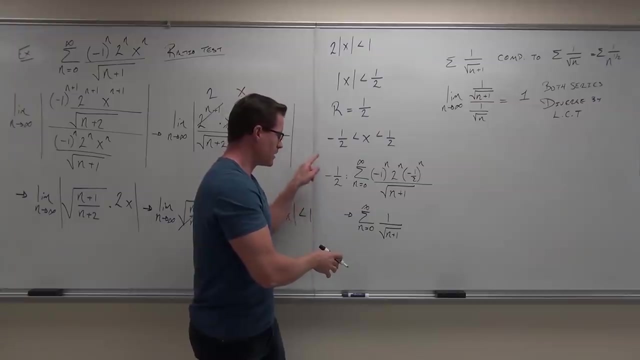 Whether it's convergent or divergent, it doesn't matter, They're going to have the same result. So both series diverge by the comparison text, Since that was a p-series, with p equals 1 half. OK, so let's put this into play here. 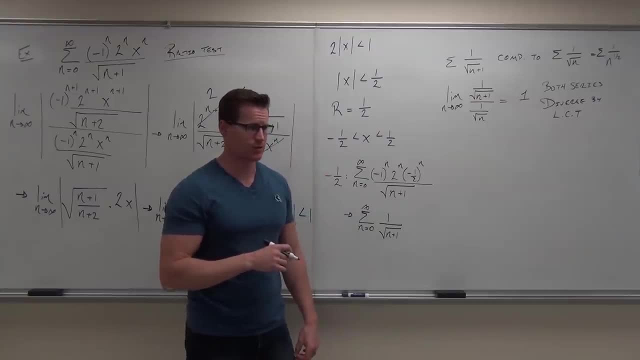 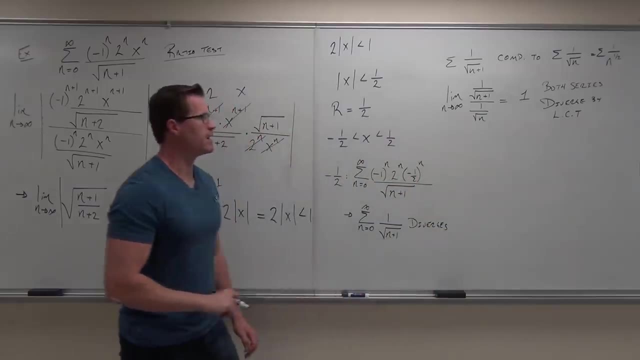 Is the endpoint negative 1 half going to be included in our domain of our power series? OK, so since this thing diverges, we are not going to include negative 1 half. Can I show you something else, a different way to think about this? 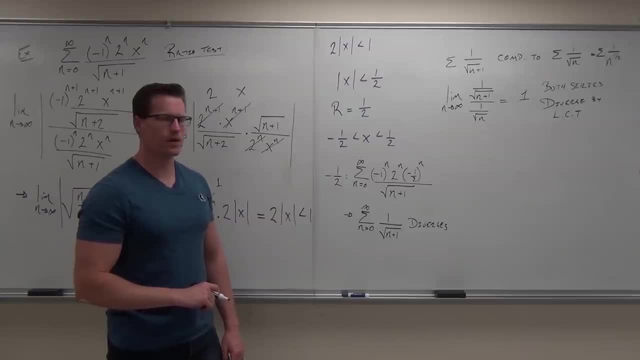 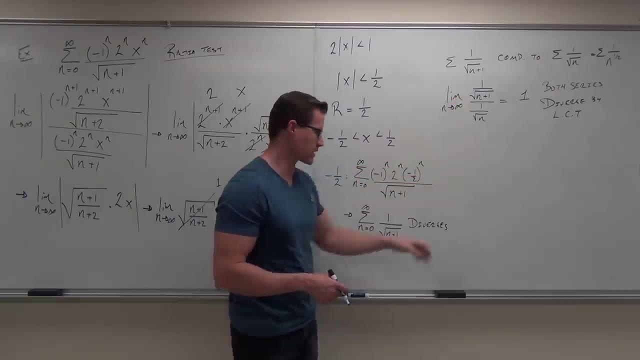 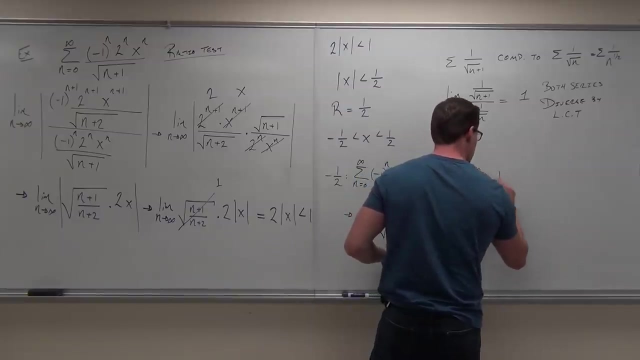 It's a little weird, but I want to open your minds to something a little bit different. You don't actually have to use a comparison test to do this. I'll show you this one. Check it. Sometimes you can manipulate your series in such a way. 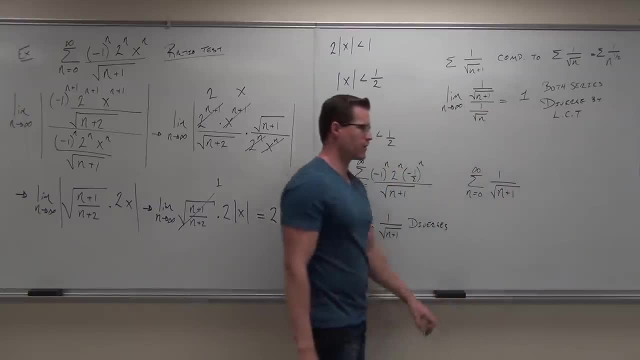 to change it from what it is to what you want it to be, And here's how you would do that in this case. So notice something: If we start with n equals 0,, what we're going to get is a square root of 0 plus 1.. 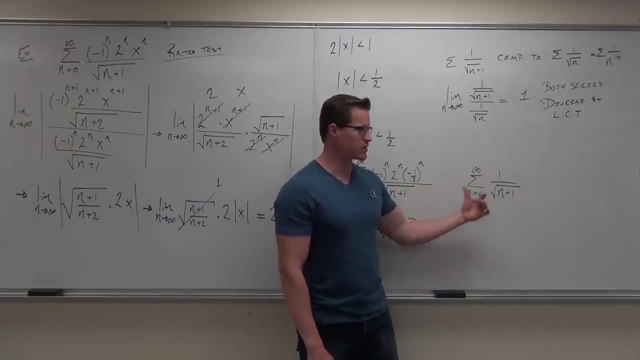 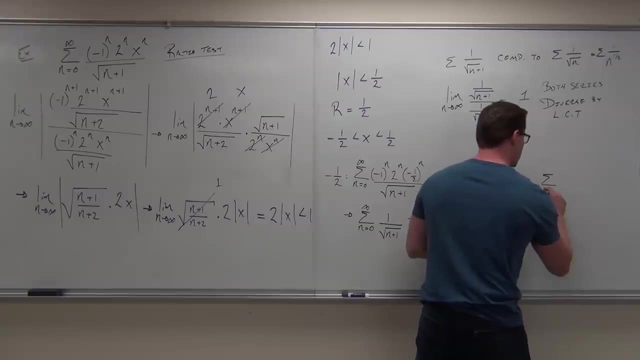 Do you get that? Well, you can manipulate these series, as long as you start with the same thing and it follows the same pattern. For instance, instead of doing a series from n equals 0 to 1.. Sorry, 0 to infinity. 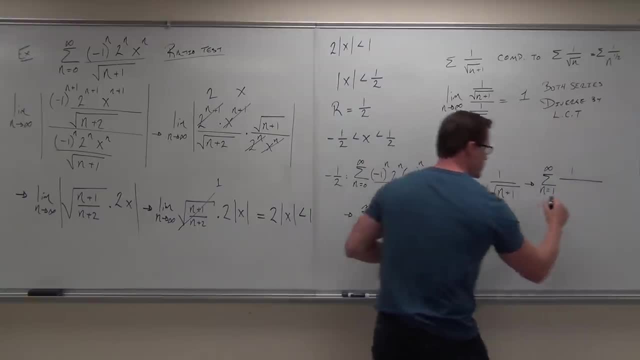 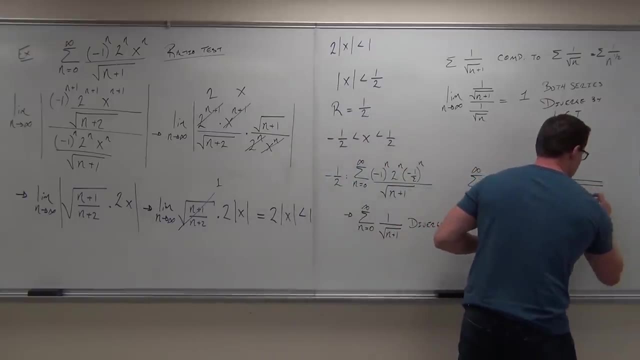 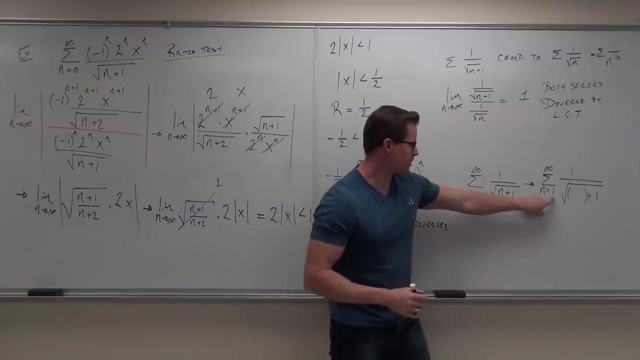 If I start it at 1, then what changes about this is, instead of having n plus 1 inside of my square root, all I need is something that takes this number and maps it to the same place that this did. So, for instance, here's 1,, here's 1.. 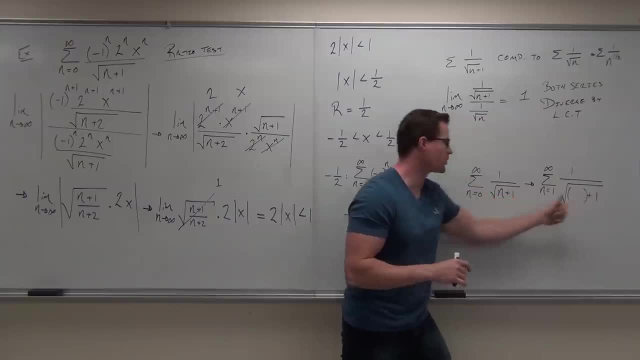 Here's square root: square root. Here's n. here's n. Here's plus 1.. OK, When I plug in my 0,, I get 0,. right, When I plug in my 1,, I need to get 0.. 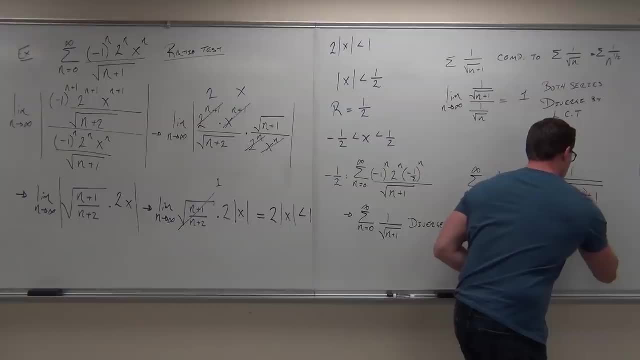 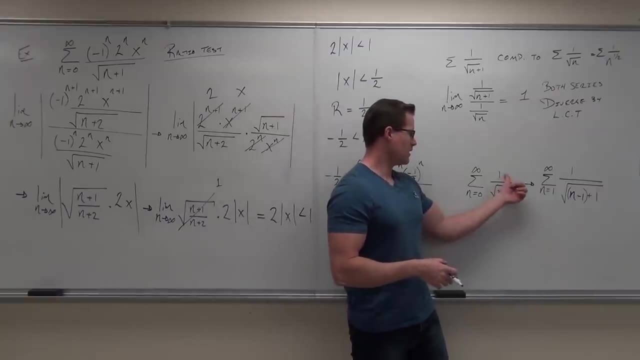 n minus 1.. Does that make sense to you? It's doing the same thing. Think about that. If I plug in 0 here, I get 1 over square root of 1.. If I plug in 1 here, I get 1 over square root of 1.. 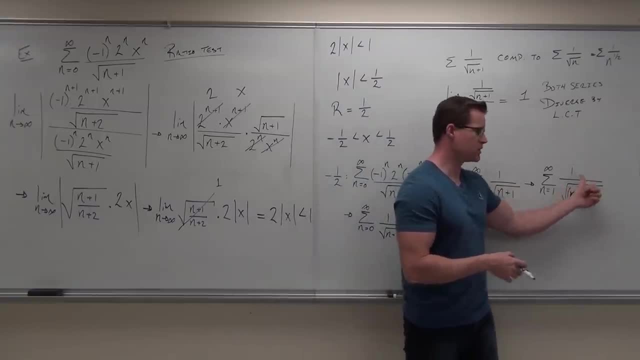 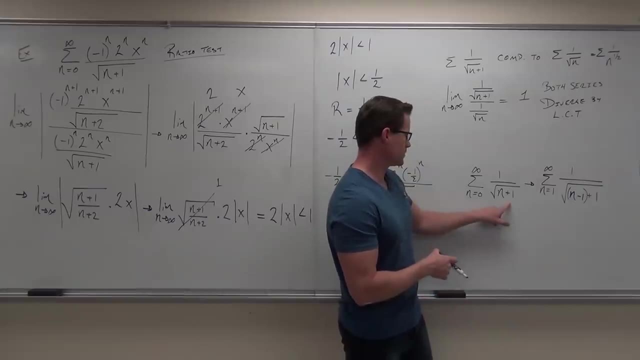 If I plug in 2 here, I get 1 over 3.. If I plug in 2 here, I get 1 over 3.. Sorry, what did I say? 2 here? Yeah right. So if I plug in the next one, it maps to the same fraction. 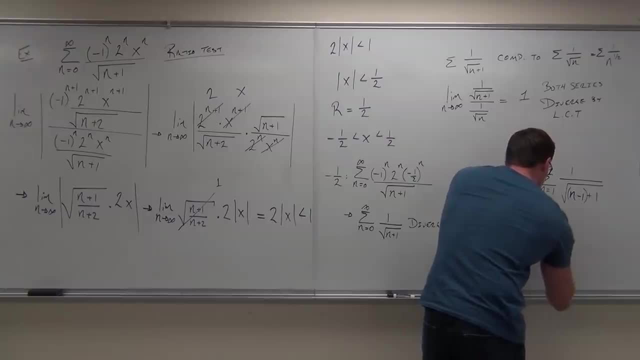 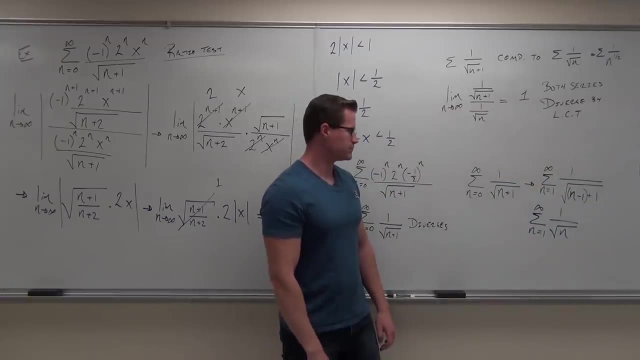 Well, if that's true, then this becomes the same exact series. This is a divergent piece series. You can do it a different way. I just want to show you that one. Is it super important? Probably not. You can do a linear comparison test and get the same result. 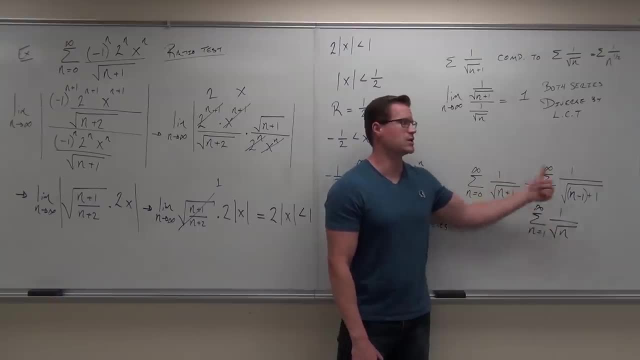 But I wanted to open your mind just a little to something else. Show of hands, if that one made sense to you. OK, cool, We're almost done. What's the last thing that we got to do here? One half, Yeah, let's do that one. 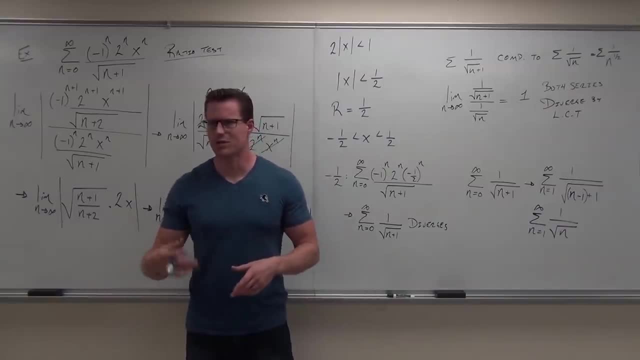 Let's do the positive one half. So if we do one half, we're going to get 1 over square root of 1.. So we're going to get 1 over square root of 1.. We're going to get 1 over square root of 1.. 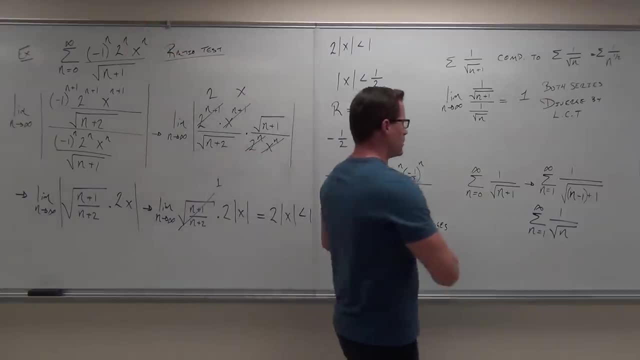 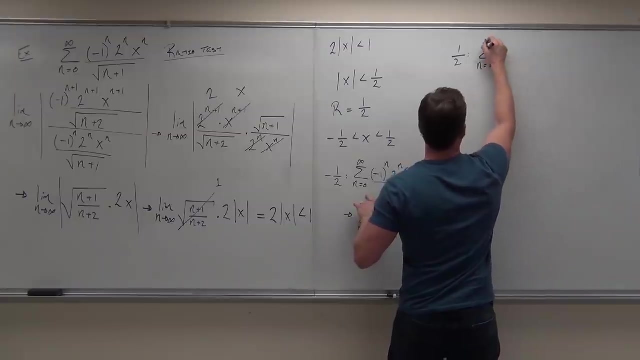 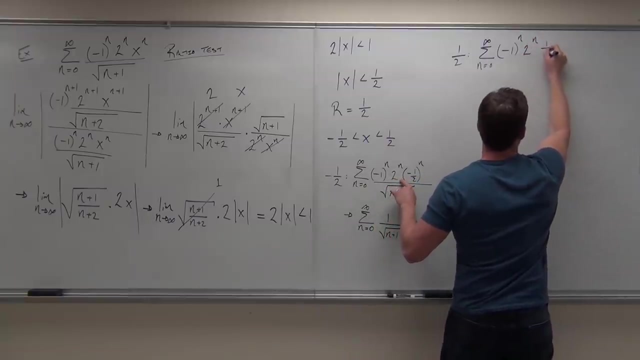 We're going to get 1 over square root of 1.. The series will look really similar, Except instead of a negative 1 half, we get positive 1 half. So if you do the same thing over here, we get a positive 1 half. 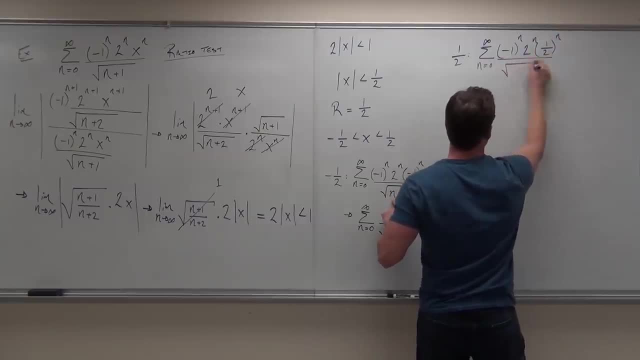 And then we'll try to find the series as simple as possible. So if you tried this one over here, it's going to be 1 over square root of 1.. So that's the first one. I'm going to try one here. 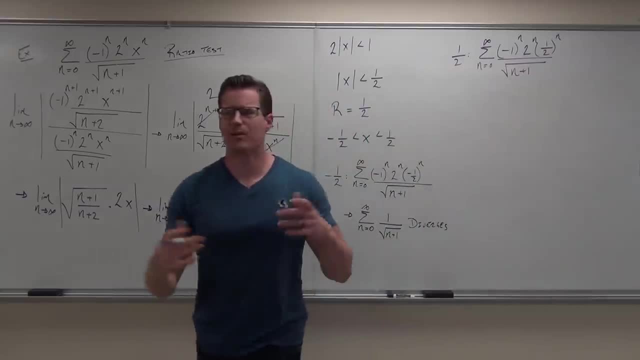 And then I'm going to try this one over here, and then I'm going to try just one over here. What's going to happen with our numerator? Let's simplify that. What do we get? A negative, negative, That's right. 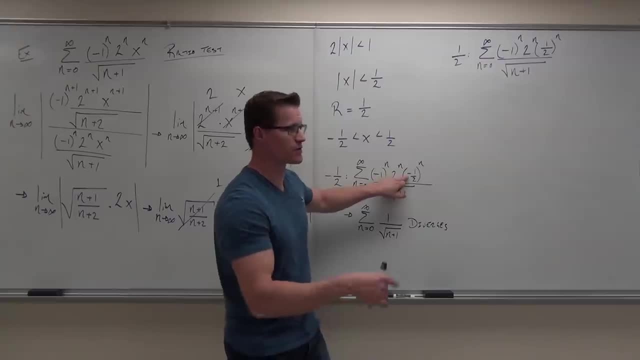 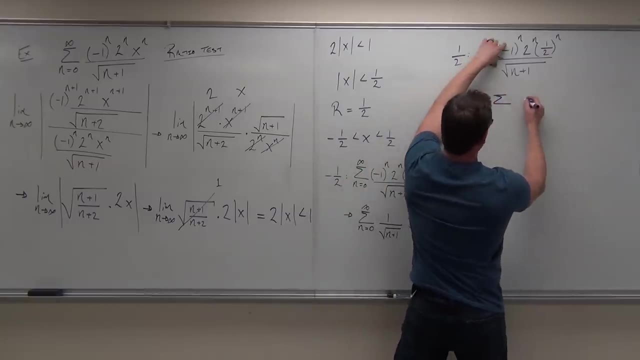 We don't have that negative we had here, So we had negative times. a negative gives us a positive. I don't have that here. So our series does look really, really similar. It's still going to be a 1, but it's a negative. 1 to the n. 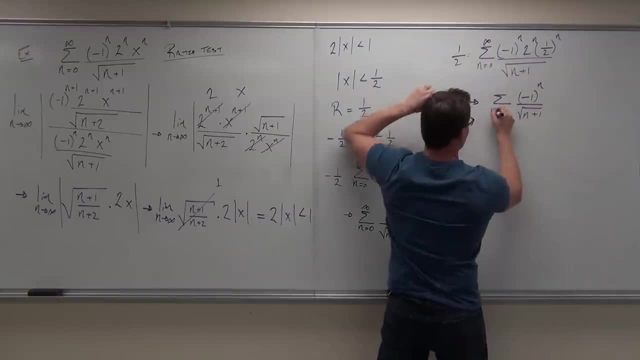 over the square root of n plus 1.. Now this one. oh man, this will be ringing some bells. Tell me something about this series that you know right now. Alternating, It's alternating, All right, so alternating series, So we take the limit. 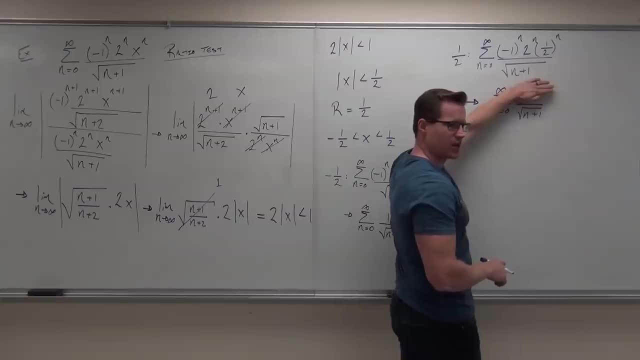 What's the limit of that series? Zero, Zero. Remember doing that. Limit is n plus infinity is zero If the sequence from which we get our alternating series goes to zero. that's like the divergence test for our alternating series. Next up is our series. well, what's the next thing? have to be. 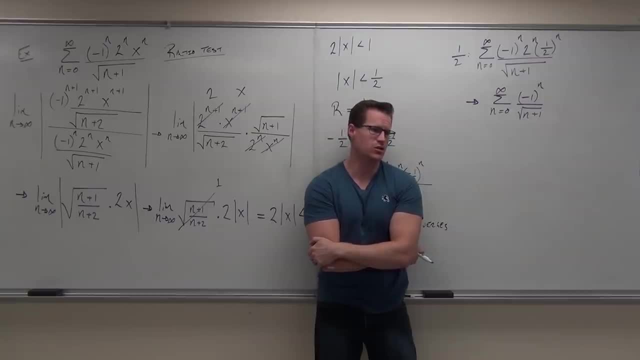 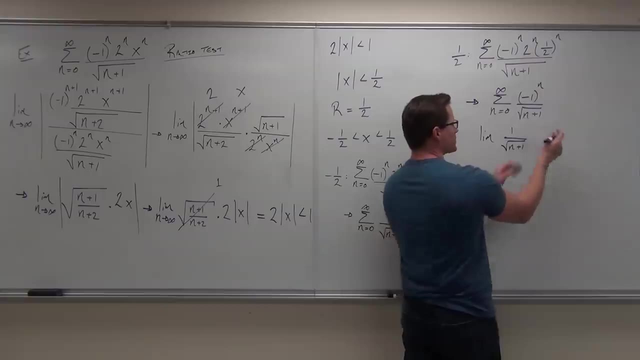 Is it decreasing term by term? Yeah, and it's really easy to show. So we'd say the limit of 1 over square root of n plus 1.. That's our a sub n. So to get our a sub n, you cover up this. 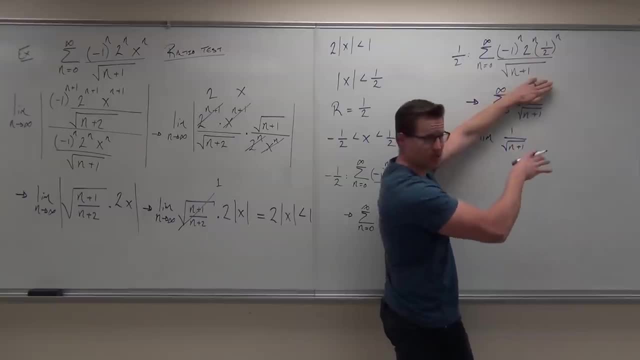 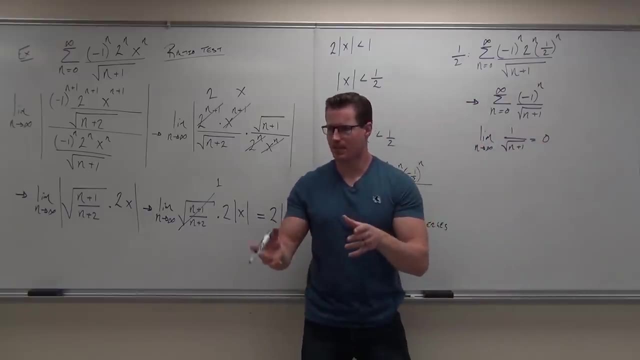 You go. okay, what's remaining after I take away the alternating part? That's our a sub n. If the limit as n approaches infinity gives you a zero. that's like passing the divergence test and saying, okay, it's not. 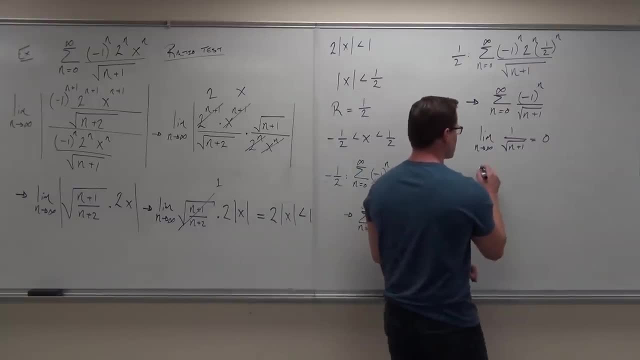 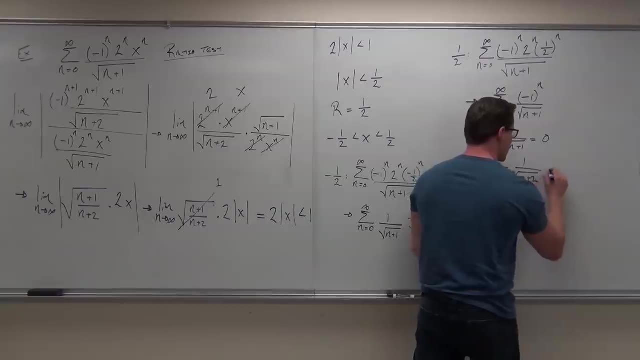 maybe not divergent. You keep on going. After that you say: is it decreasing? Is a sub n plus 1, which is 1 over square root of n plus 2, is that less than 1 over square root of n plus 1, which is our a sub n? 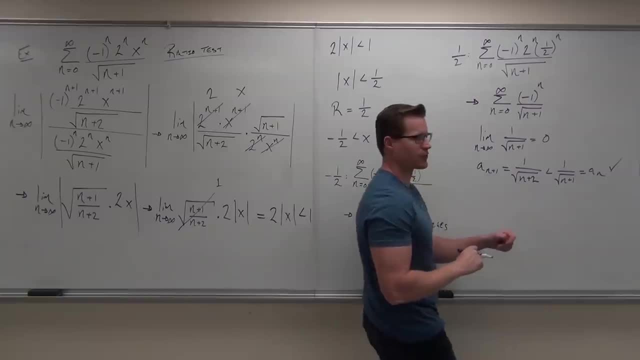 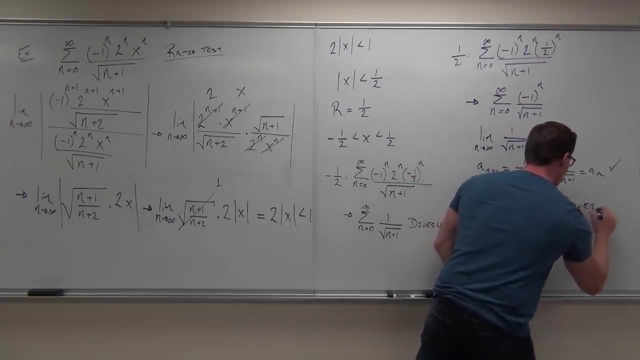 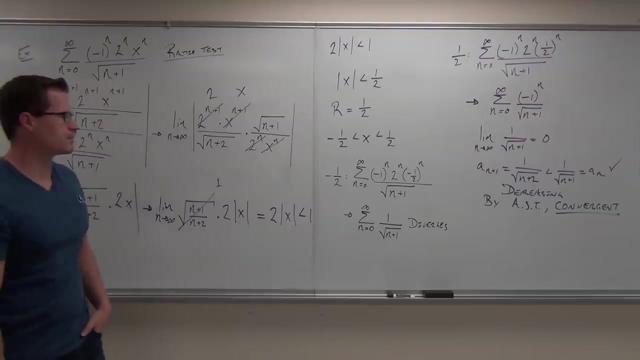 If that's true, which it is here, this is definitely less than that for n greater than or equal to 1. This says it's decreasing, So by the alternating series test we get convergence. Let's put the whole thing together then. 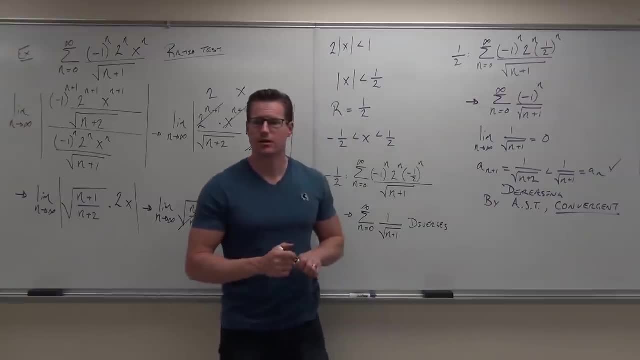 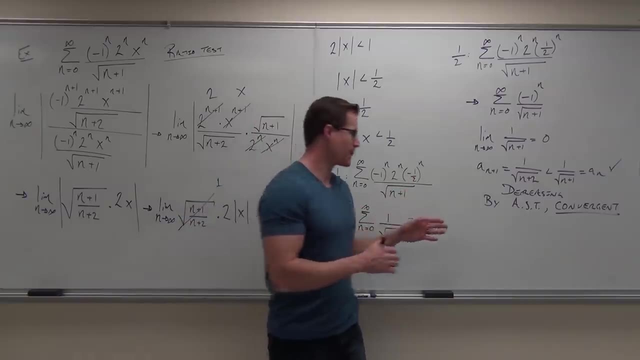 Do you know what your interval of convergence is? Oh, interval, Your interval of convergence. Do we know what it is right now? Yes, Where does it start? ladies and gentlemen, Negative 1 half: Is the negative 1 half included? 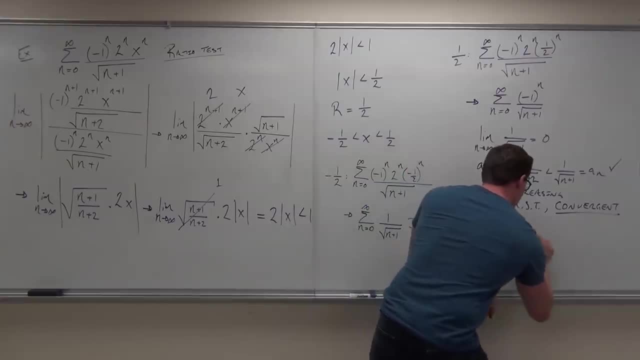 No, Where's the n 1 half? Is the 1 half included? Yes, So we know the radius is 1 half, We know the center is zero, We know our interval, We know everything about this. So for our last example, I want to make it real clear. 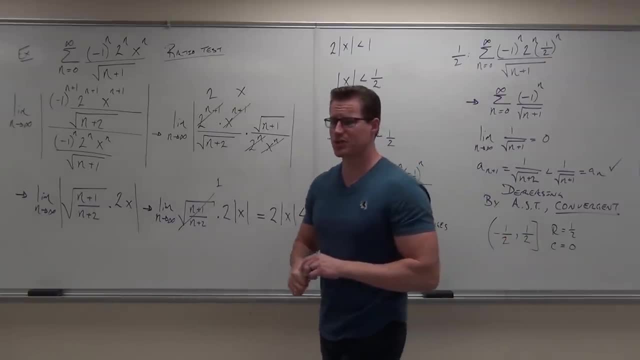 Make sure you guys are really good at this. We got these things called power series, which are functions Power series- how about it? It's a function of x in there, so when I write out the series, I get a function of x. 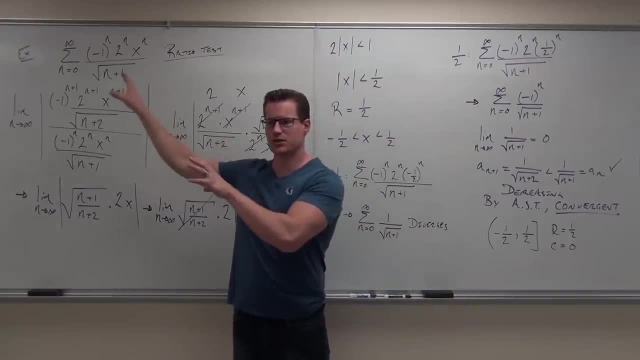 Now that function is only defined where that series converges. That definition, that's our domain. So what can x be in order to make this thing convergent? That's, when we go through all this mess, We go okay, well, what's x got to be for that to work? 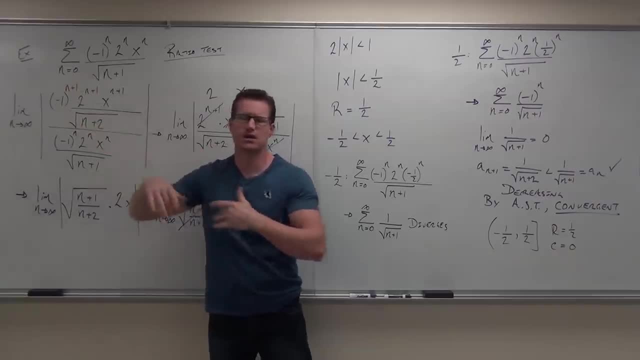 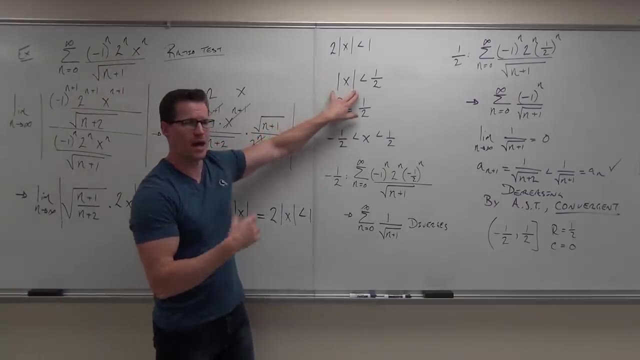 What's x got to be for our series to converge so that it defines a function of x. We get all the way down to here. We say okay whenever I have my whatever's being raised to the nth power, isolated inside my absolute value. 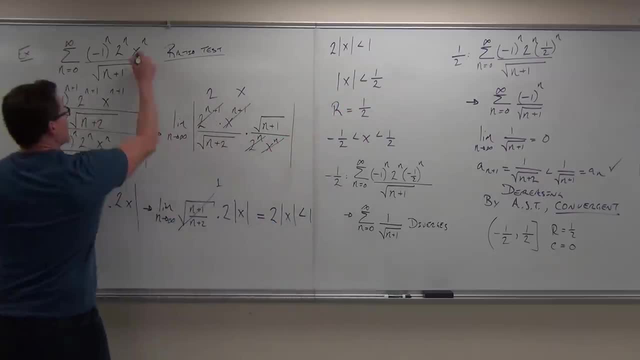 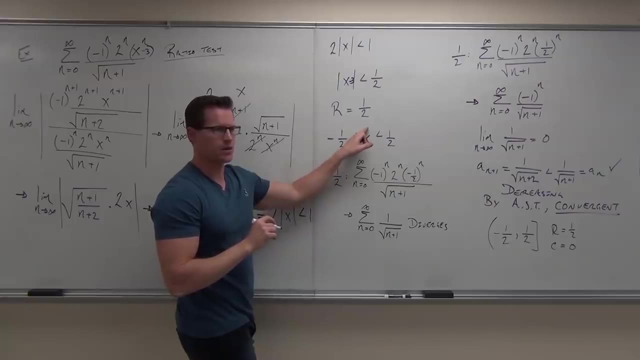 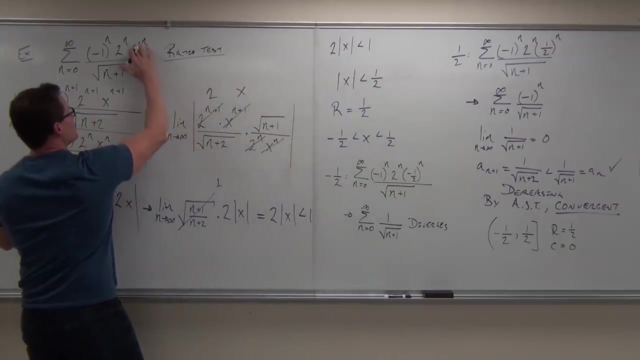 what I want to get out of here is your radius. If this had been an x minus 3, I would want an x minus 3 here, before I determine my radius. Does that make sense to you? Yes, After that, After we determine the radius, that's all fine and good. 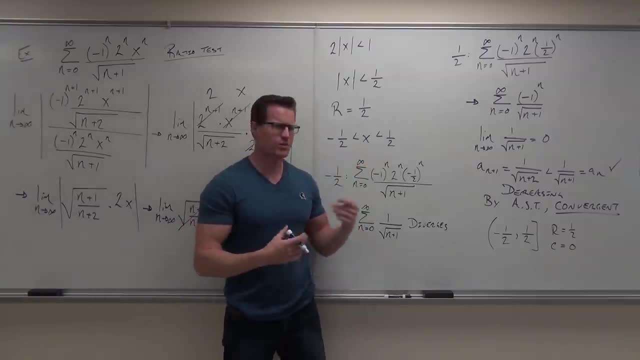 We get our interval and then we check our endpoints. The endpoints are going to be done with something you've done before in this class: either an alternating series test or a limited series test, Or a limited comparison test or another test that we have, integral testing. 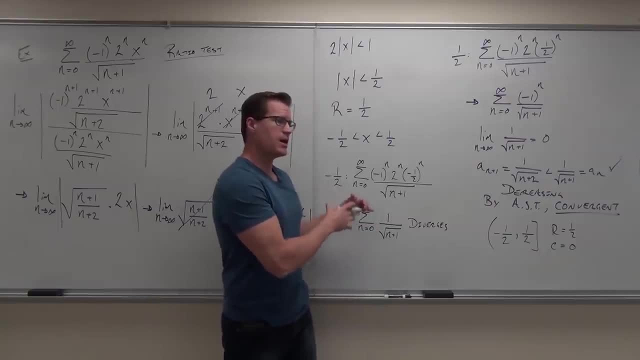 I don't care what you use, as long as you can test this thing out. If you get for an endpoint that a series diverges, that endpoint's not included in your domain. that makes this power series convergent. so defines our power series. 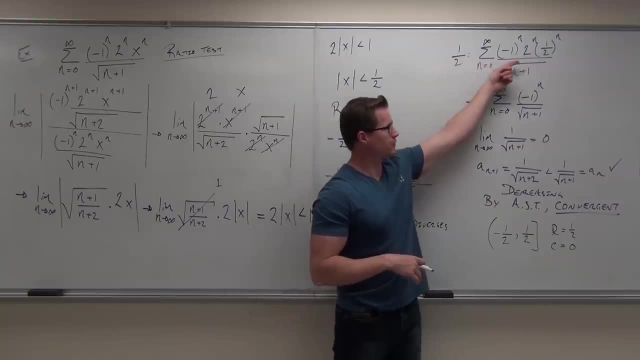 If you get that, the series, when you plug in that endpoint for x, does converge, then the endpoint is included. This is what we're looking for: the radius, the center and our interval of convergence. that makes this power series work. It makes it converge. 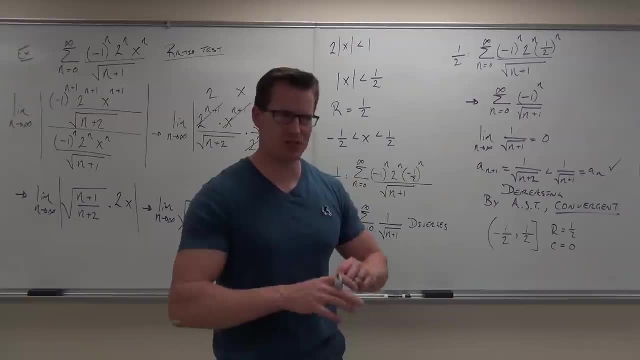 Therefore, we can define a function by using that domain. Have I explained everything well enough for you guys to understand it? Are you sure? I don't want to leave anything hanging. Do you guys get the idea? Can you do it yourselves? 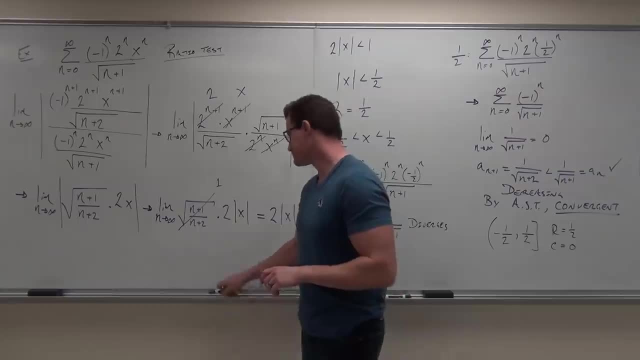 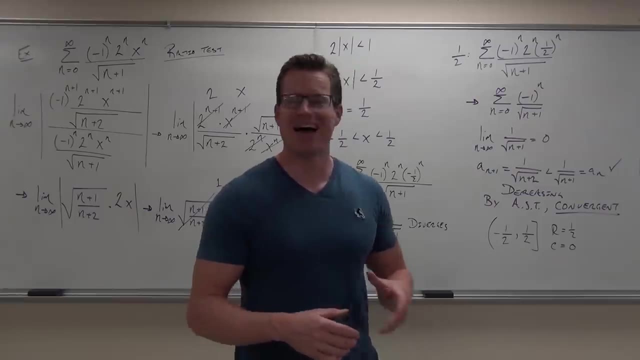 Okay, Then the last thing we talk about in this section is how to actually do calculus with these power series, Which is weird. like what Calculus? What do you mean? How do we do derivatives and how do we do integrals of power series? 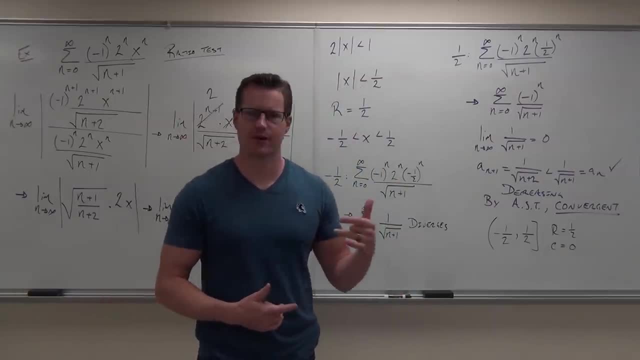 And honestly, it's not that hard, but it leads us to something very, very interesting. It's kind of like our stepping stone between this section and the next section, which is Taylor polynomials and Maclaurin polynomials. Well, Taylor series and Maclaurin series. 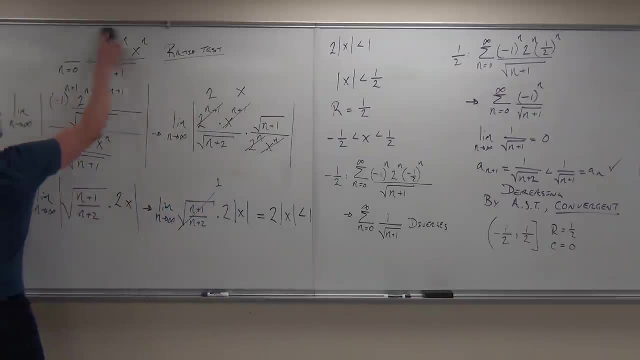 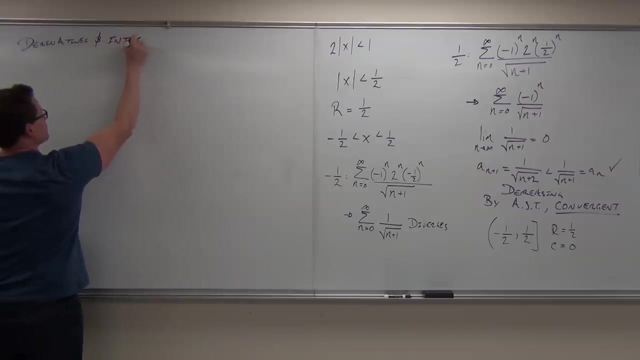 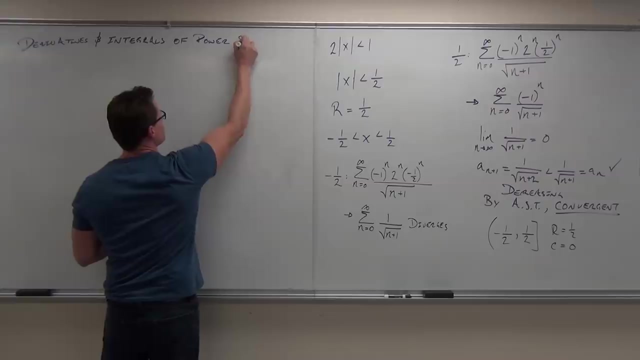 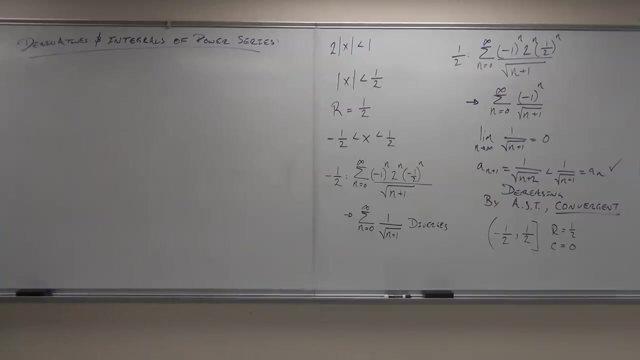 That leads to Taylor polynomials. But firstly we've got to learn how to do derivatives and integrals of power series. Well, how in the world are we going to do that? Well, you know what? Let's start with something general. 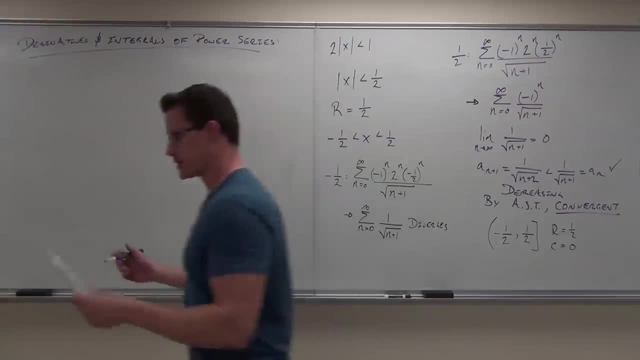 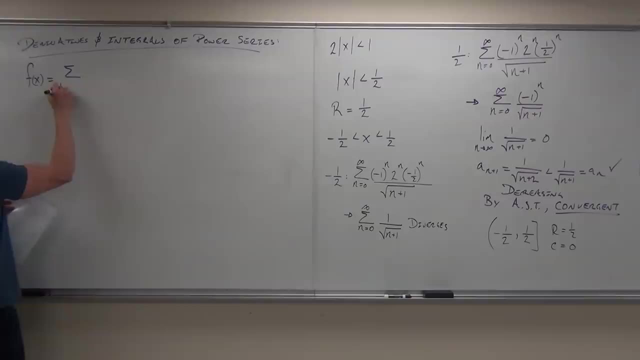 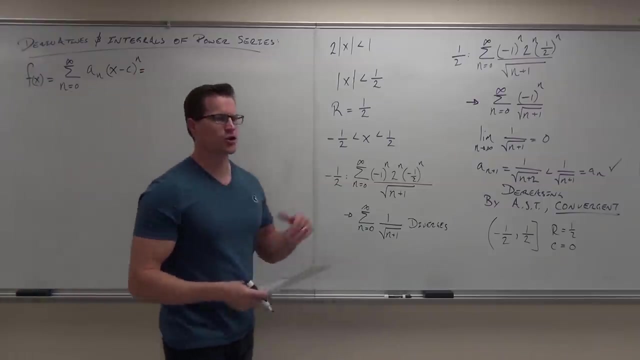 Let's just build on it. So let's assume that we have this power series. So f of x Is a power series Starting at zero, going to infinity, A sub n, x minus c to the n. Let's talk about the terms of what the series is going to look like. 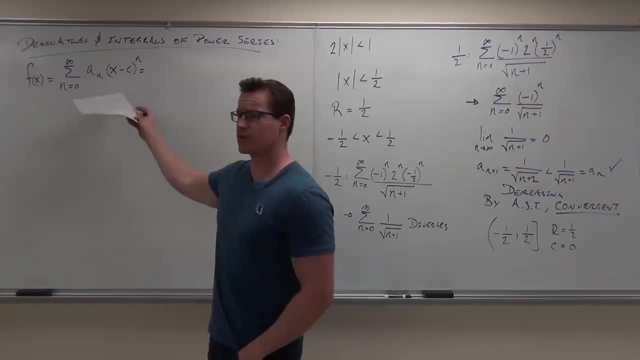 So we're going to say here that we have some power series. It will converge for some domain of x. Therefore, we're going to have this function. So where our power series converges, that's our domain for our function. 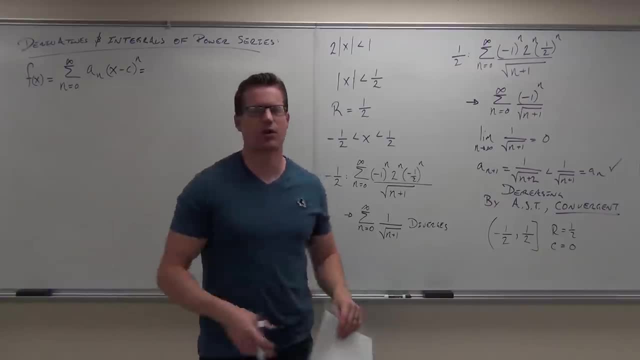 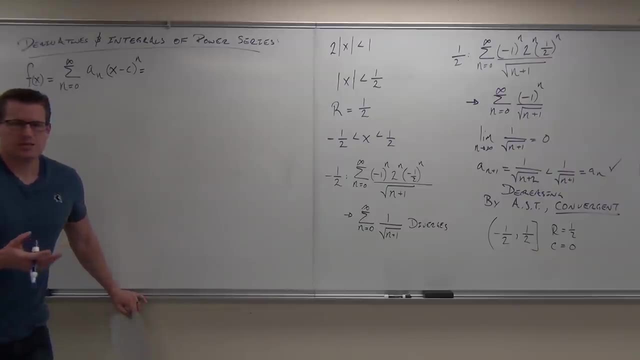 Okie dokie. Now what do the terms look like? What's the first term? A sub n? Yeah, a sub. what? A sub zero? A sub zero. How about x minus c? Is that going to be up there? 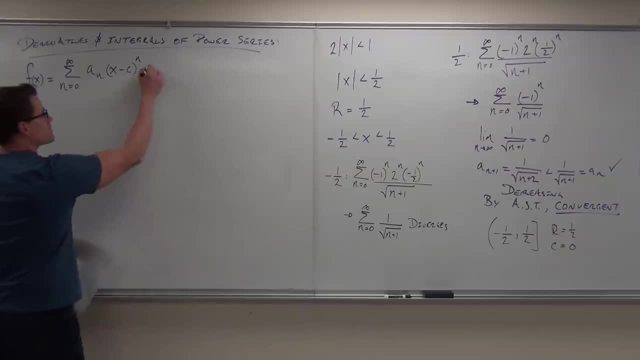 No, No, because it's being raised to the zero power That gives us one. So we just get a sub zero Plus what's the next term going to look like? A sub one, A sub one, Very good. 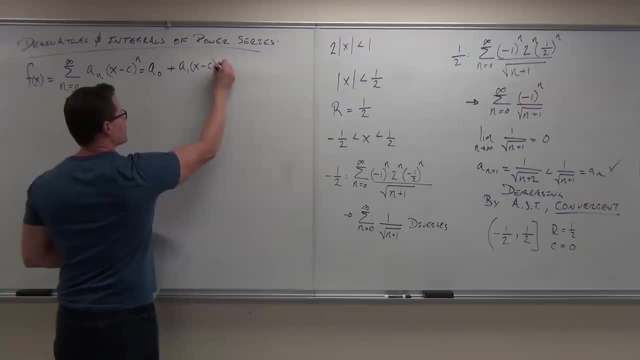 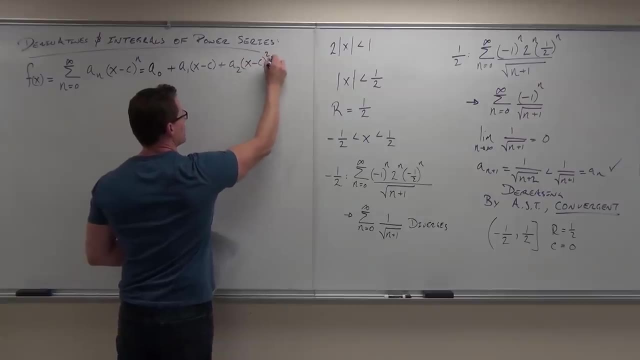 x minus c To the To the third. Plus- what A sub two, Uh-huh. x minus c to the second power. Good, Now we're getting the pattern: A sub three, x minus c to the third. 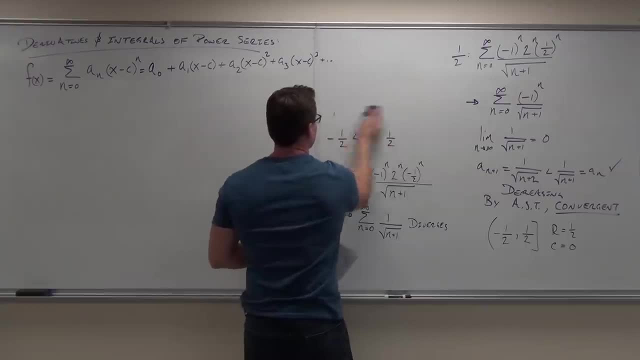 And it doesn't end Well. here's the cool thing You know about derivatives, right? Derivatives say: okay, well, take your function, And when you do a derivative, we basically just derive it term by term, don't we? 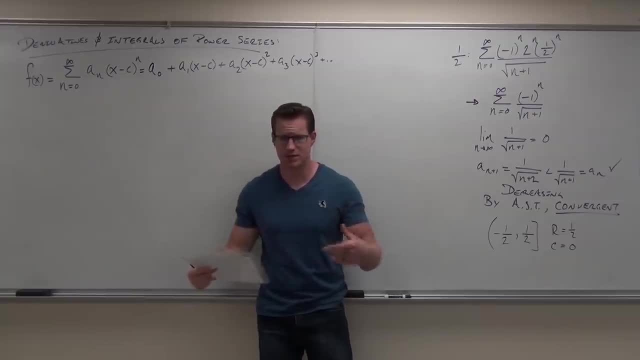 And when we have pluses or minuses, we know that with derivatives we can separate those pluses or minuses and just do the derivative of that term. Put it back together with a sign. You're good to go. Well, if you think about it. when I do all my terms, tell me what a sub zero and a sub. 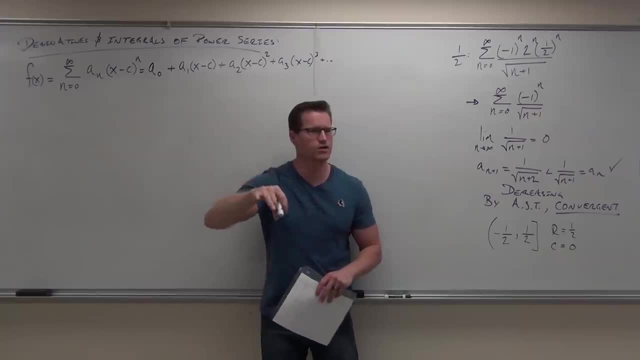 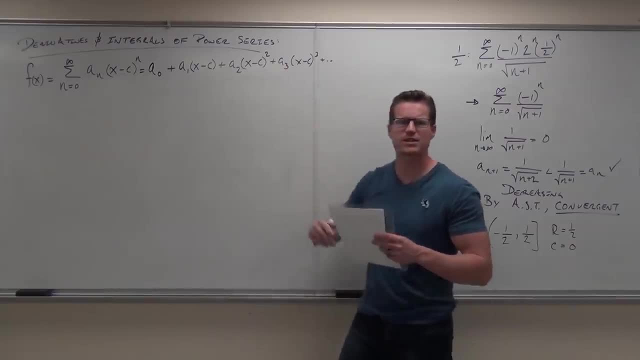 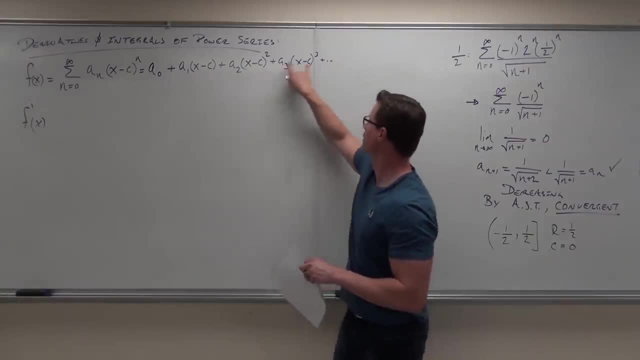 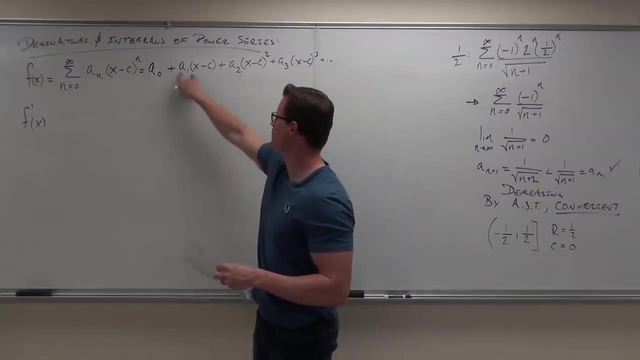 The only place I have my variable is here and here and here and so forth and so on. Does that make sense to you? So we notice that when we take derivatives here. am I going to need a product rule here? No, That's like a coefficient. 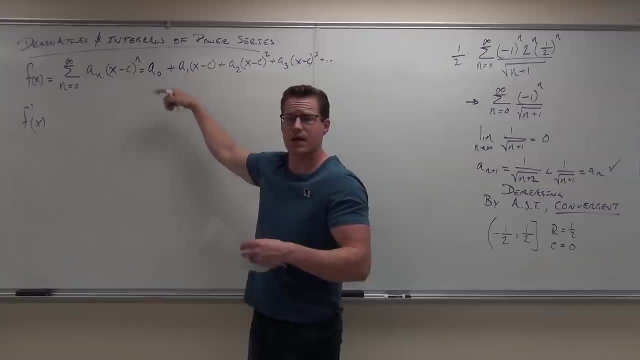 It's like three or something, It's like seven, I don't care what it is, It's a coefficient. So what we do with this is: yeah, if we have just a constant by itself, what's the derivative of a constant? 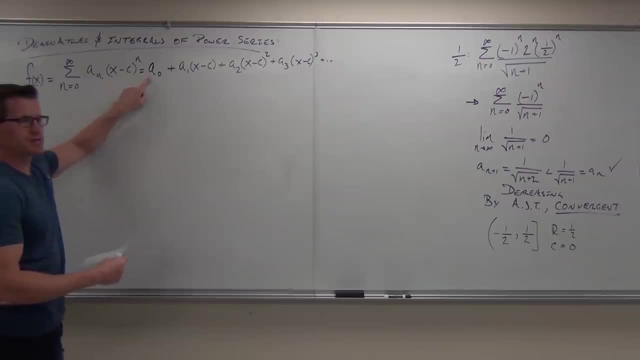 Zero. Okay, so we're going to take a derivative term by term. The derivative of a sub zero is Zero Gone. I don't care what it is, It's a constant. I'm going to do a derivative of that. 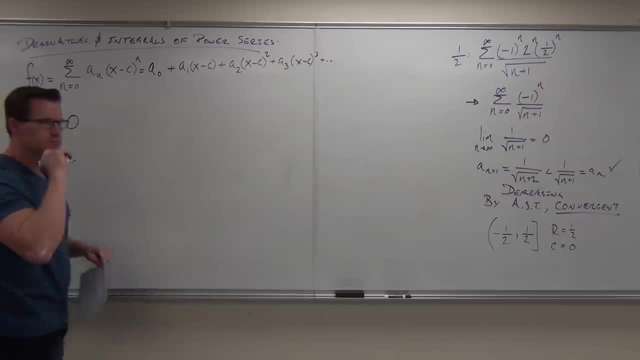 It's gone. So f prime of x gives us firstly zero. I'm going to write the zero just so we see what's going on with that. okay, So, derivative of a constant man: zero. What's the derivative of this guy? 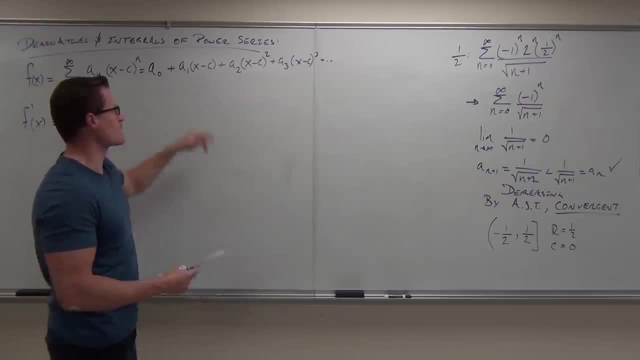 One, Not one. no, If this was three x minus c, it wouldn't be zero, It would be three times one x minus c to the zero power times, the derivative of the inside, which is one, And this is one, This is: 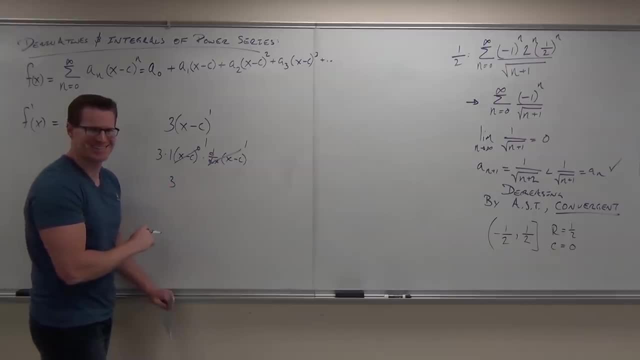 Three, Please don't forget your Bayesian calculus. okay, It's just the chain rule, folks. You bring down the power, You multiply by the inside. Good to go. So this would be, in this case, what A sub one. 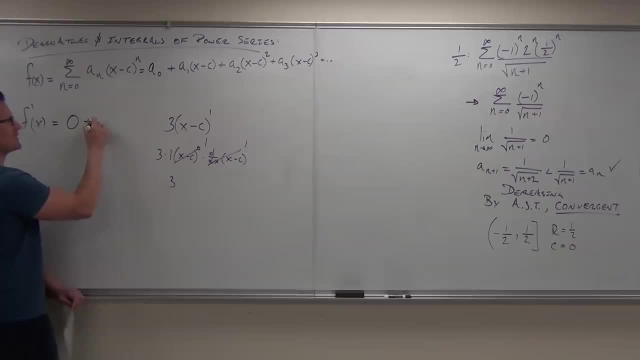 Don't say three, It was just an example. A sub one, A sub one, That's right. A sub one, What? Okay? Plus A sub Two, Two, a sub three. What are you going to do with this? 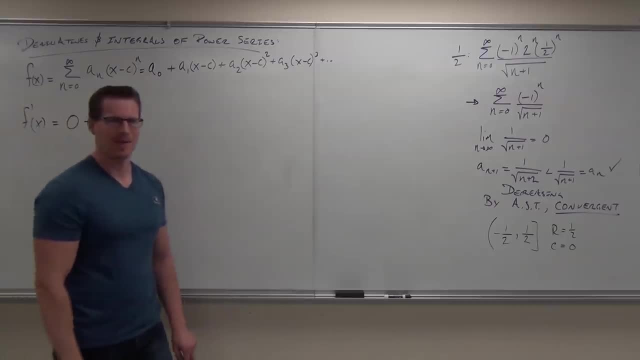 If that's a coefficient like three, you're going to bring down the two, aren't you? Two, Two a sub three. Two, Two a sub three. What are you going to do with this? If that's a coefficient like three, you're going to bring down the two, aren't you? 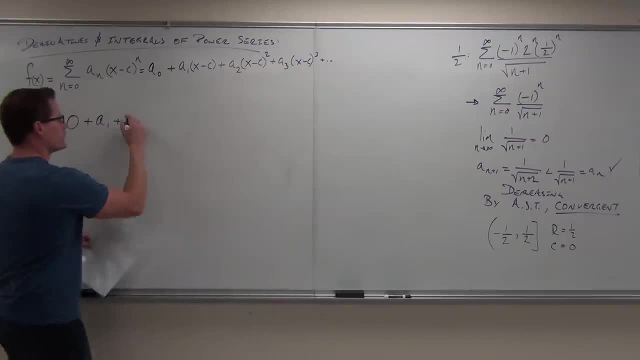 Two, Two a sub three. You're going to have two times a sub two. You're going to have your inside x minus c. You're going to raise it to one power less than what you had to the first power And you're going to multiply by the derivative of. 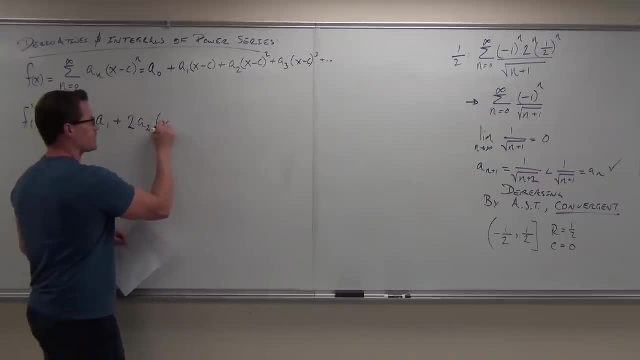 The inside, Which is One, One all the time. It's centered at c, It's just going to be x minus c, It's one all the time. So that's great. So we're using the chain rule. 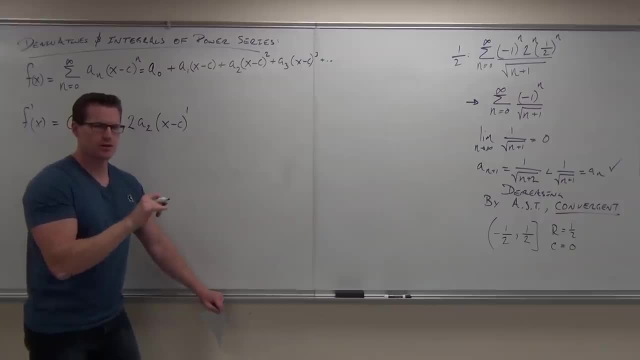 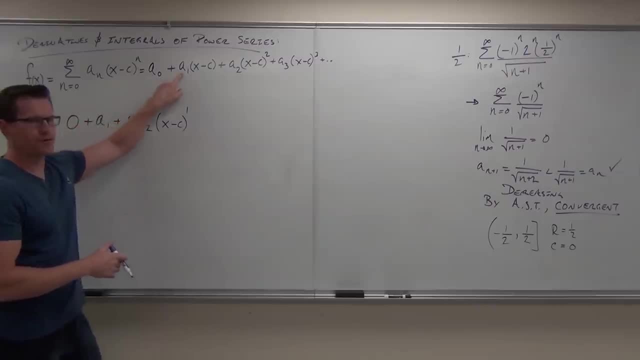 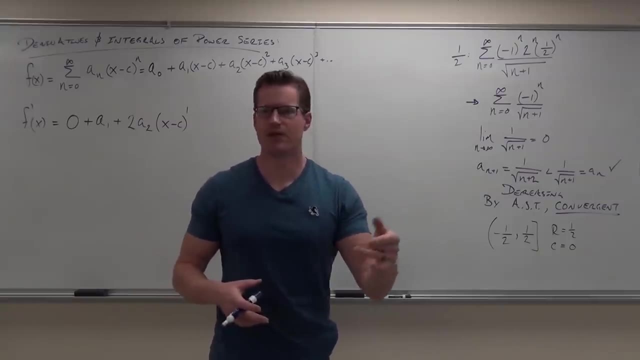 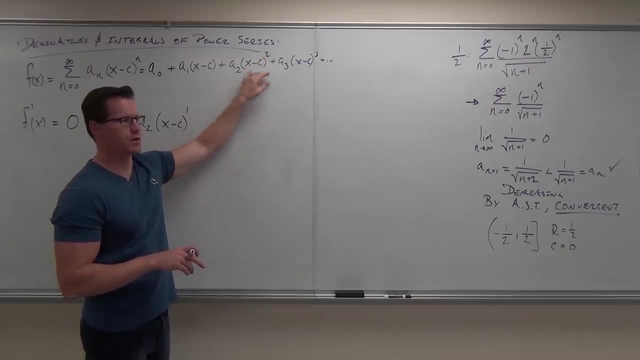 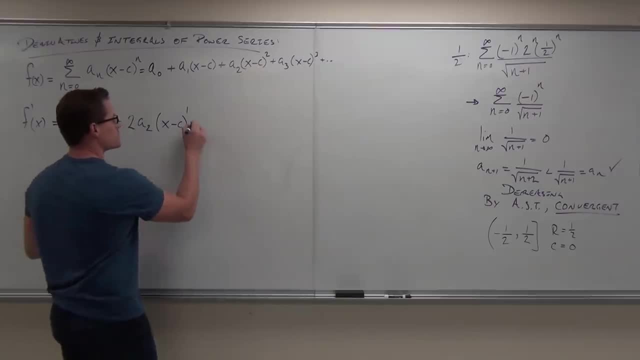 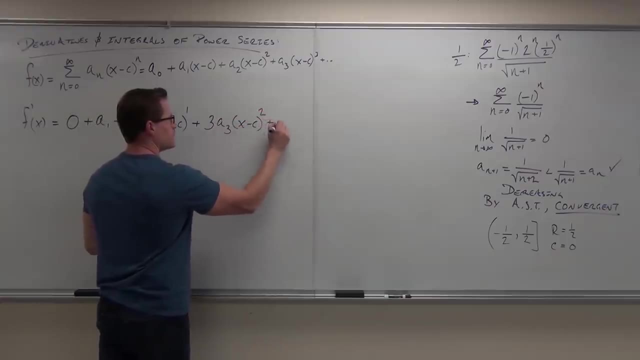 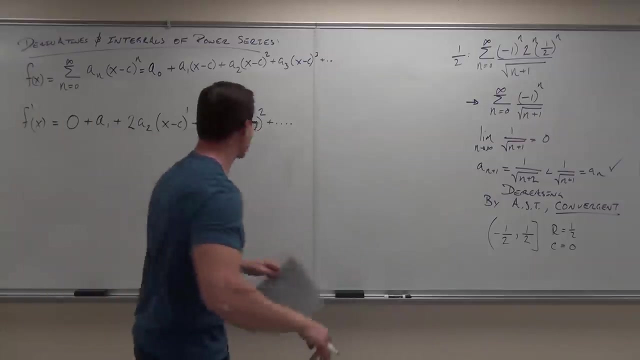 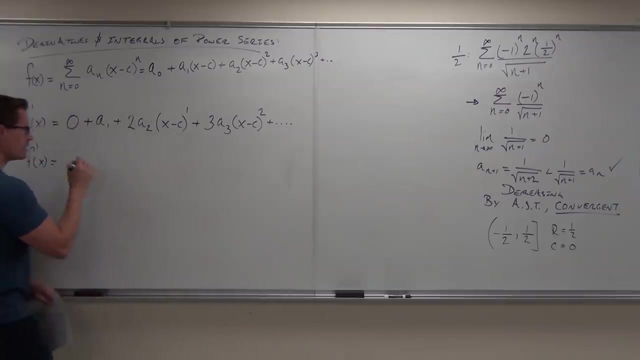 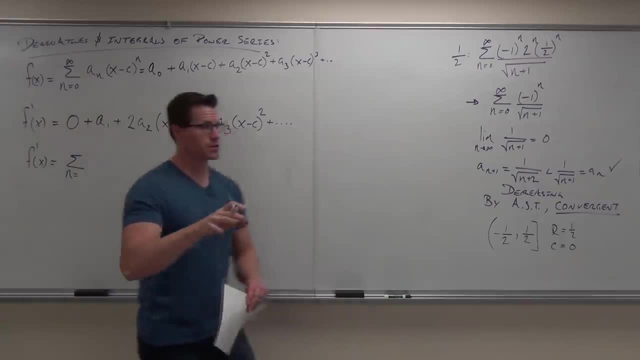 This is so cool, the way these actually work. Check out what happens. So F prime of X really just does this. First thing: Tell me where our series actually starts now. You see, our series here started at zero. We had A sub zero. 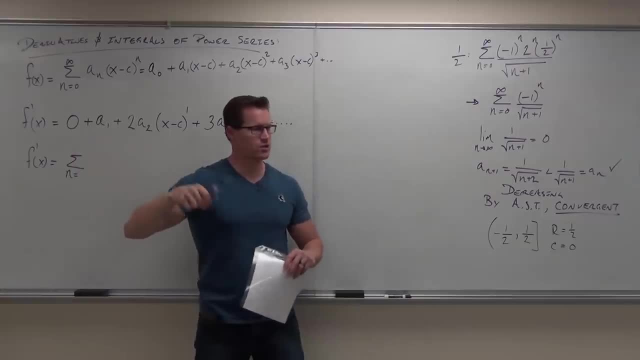 Where is our derivative starting? A sub one doesn't start at a sub zero anymore, it starts at a sub one. Why? Well, because the derivative of our very first term, gentlemen, gets rid of that constant. So this thing is gone, we start at a sub one. 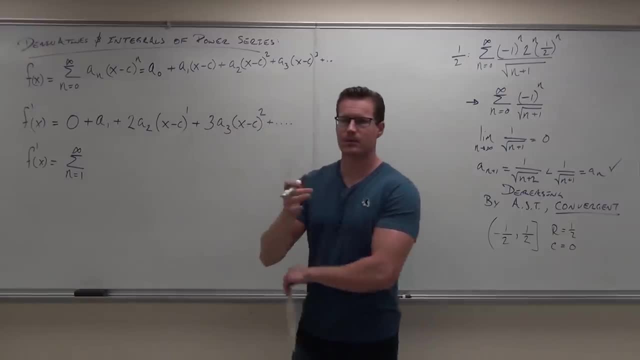 Question: Well, the a sub one, because you said you bring the variable down and leave the inside alone. so where's the x minus c attached to the a sub one Right here On that one? yeah, like that one over there. 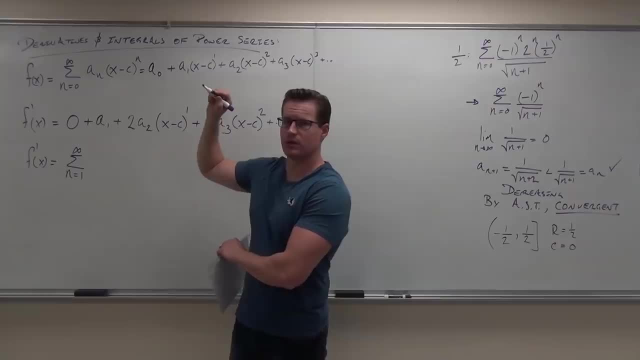 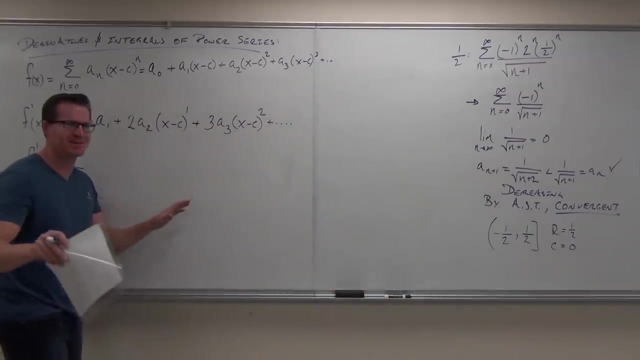 The derivative of that is one, What's one minus one Zero. You're right. Okay, You're right, it happens. I know I'm right, you're right. I like hearing that, though still, Especially from my wife. that never happens. 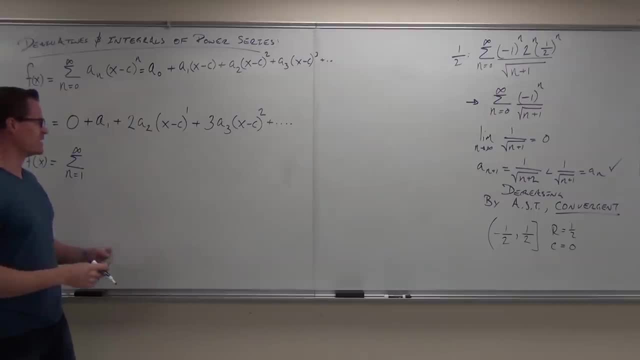 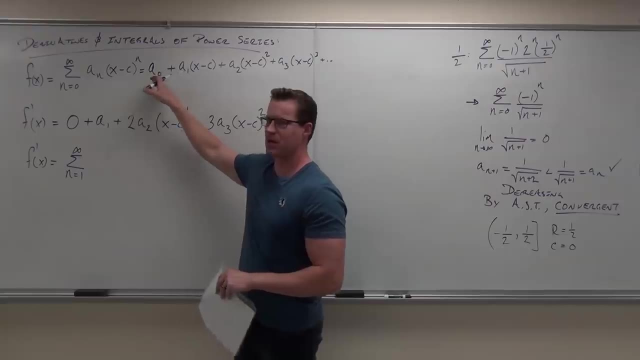 Especially if she's my female. so, Anyway, so here's what goes on. When you take the derivative of a power series, your first term is a constant. it goes away, so we don't have the zero of the term anymore. 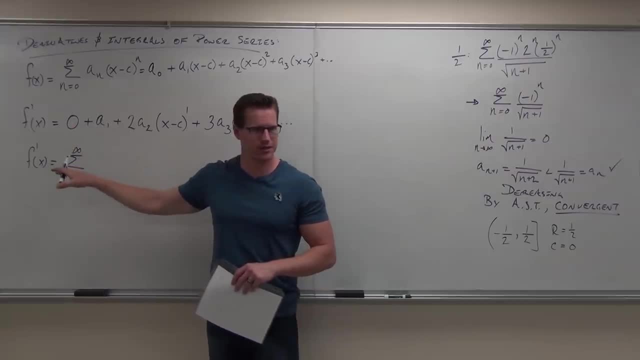 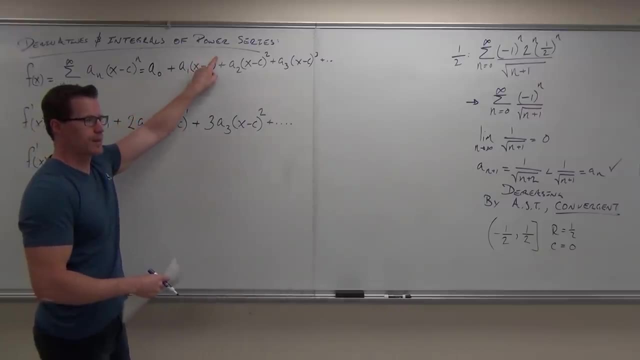 we start at a sub one. Okay, The a sub one term, or when n equals one. Are you with me? Now, what's happened here is for every single term that we've had, we've taken the power, we've moved it down. 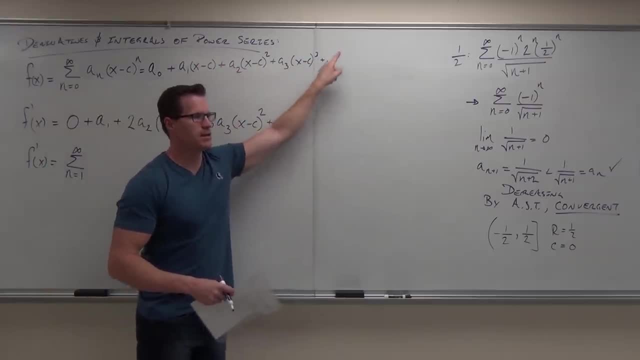 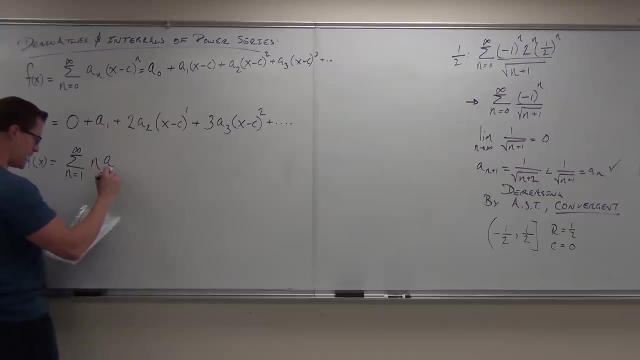 But notice, one one, two, two, three, three n n. We're moving the nth power forward. We're leaving the a sub n alone. actually A sub one, okay, a sub two, a sub three, a sub one. 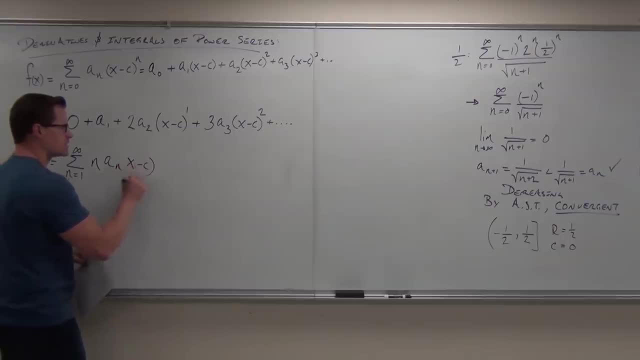 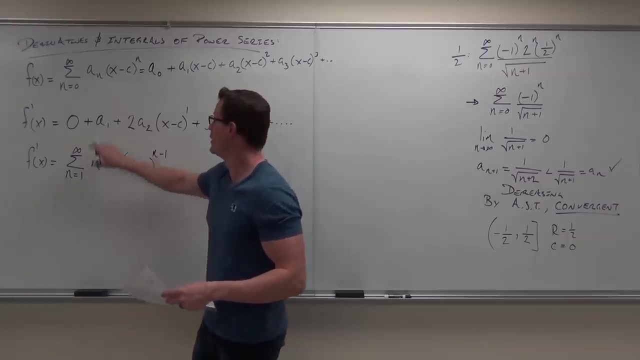 a sub two, a sub three, no problem, And we're doing x minus c to what's going on to our power. What are we doing with it? Do you see that? this from here to here? look at that. it should look very familiar to you. 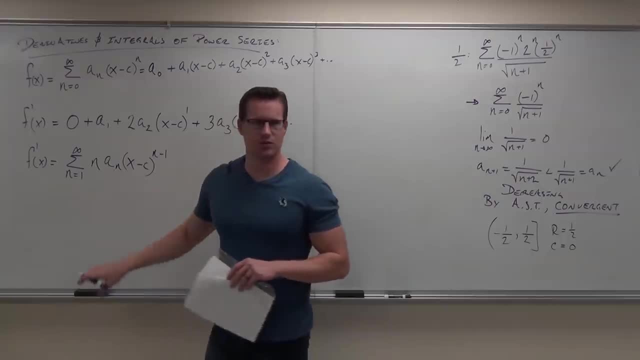 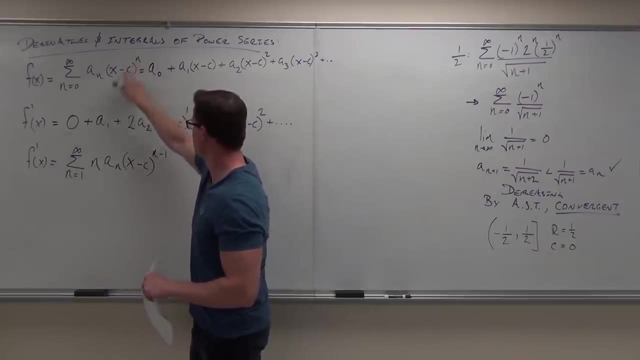 From here to here. do you see that that is just a change? Well, that's all that is. It's just that, or the general power rule. if you learned it as a general power rule, it says: hey, take your power, move it down front, no problem. 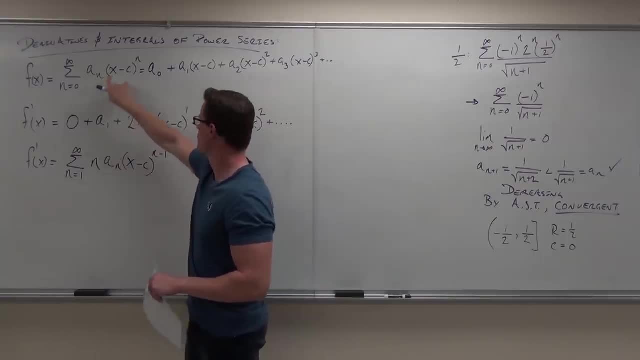 We got that. That's a coefficient. leave it That inside of something- chain rule. leave it. Subtract one from your exponent, no problem. Multiply by derivative of the inside. hey, it's one, It's just the chain rule. 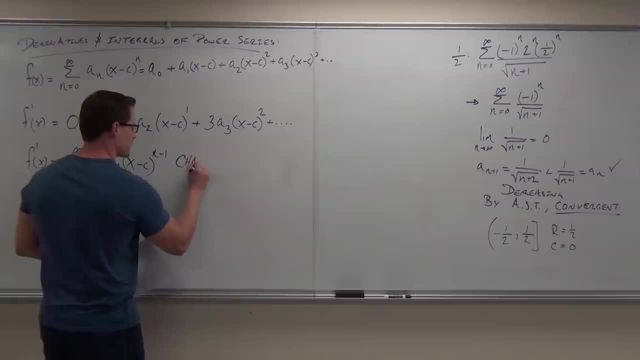 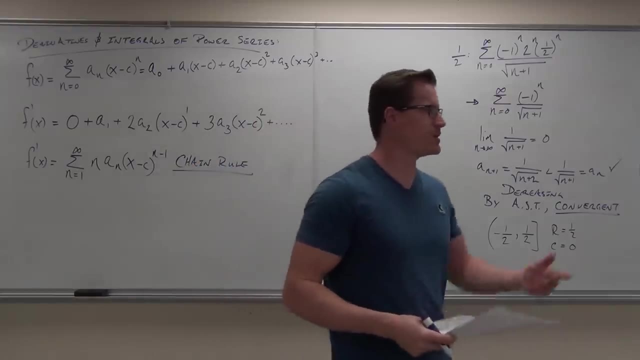 That's all this is. It's just very cool that that still works for our power series. Maybe it's not that cool, maybe it's obvious to you, because a sub n's a constant anyway, But most people say, wow, that's kinda neat. 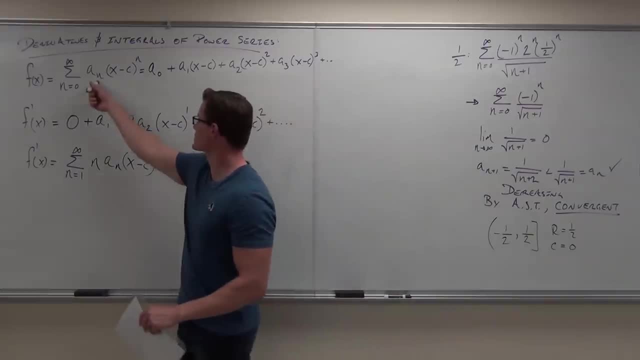 But when you think about it like it should be apparent, it should be: well, if that's a constant, that's a constant times, something x raised to a power, You can use the chain rule with it. You guys with me. 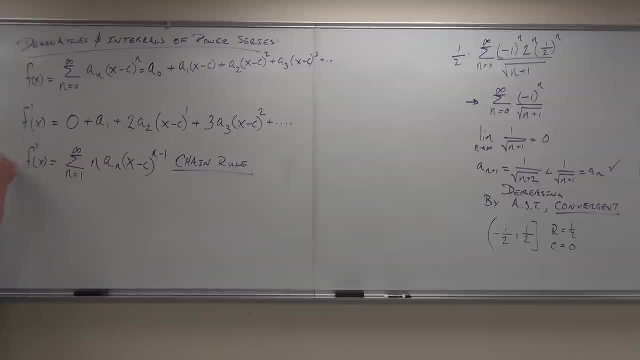 Okay, next one. So we had- let's call this part a derivatives, part b- integrals. If I do the integral of f, of x, dx, Let's go right from here If I integrate term by term, which I can do. 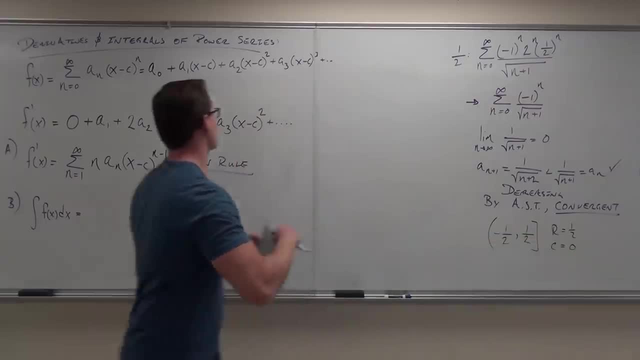 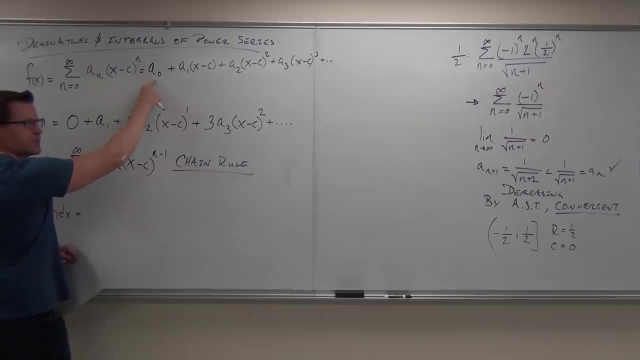 because if I can drive term by term, I can integrate term by term. no big deal. We've done that for years now. If I integrate, if I integrate term by term, what's this going to be? Is it gonna be a zero? 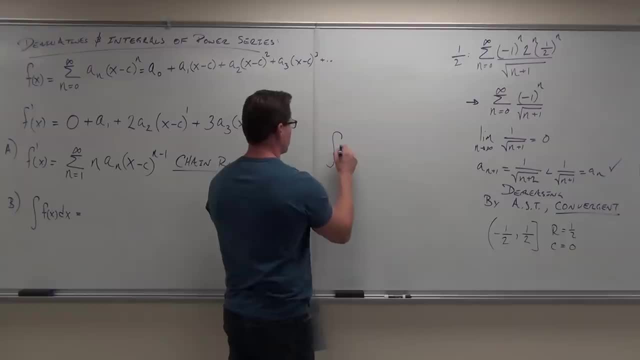 Integrals don't work like that. If I do like one minus or plus x dx, the integral of one becomes okay. Sure, so I'd get like x plus x squared over two. So okay, Now here when I do my integration. 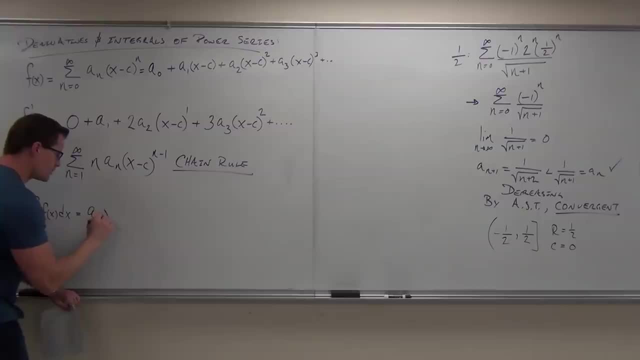 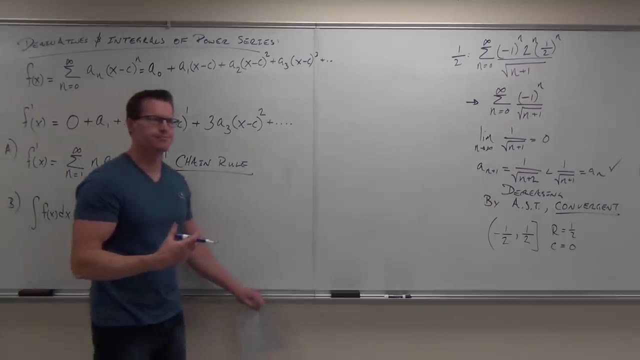 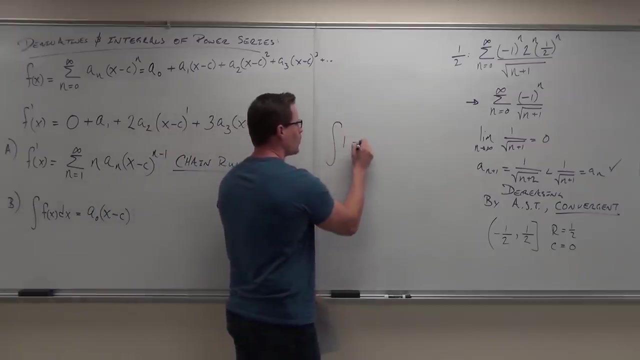 it's not just gonna be a sub zero x, it's gonna be a sub zero x minus c, But the same idea basically happens. It'd be like integrating with a substitution, kind of like that, where you'd have one plus x minus c. 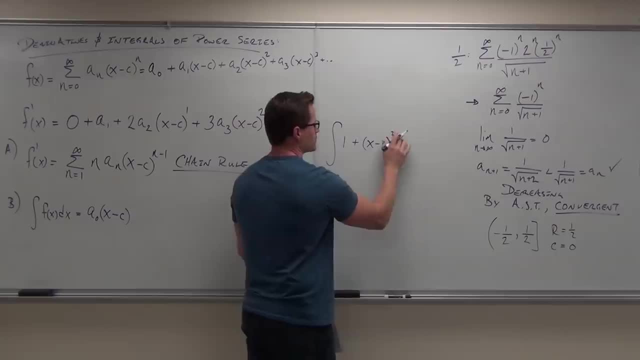 plus three, say squared or not squared. you just do it like that. You'd use a substitution, wouldn't you? You'd make u equal to x minus three And you'd go okay. well, no problem, Then when I do an integral, that would be u. 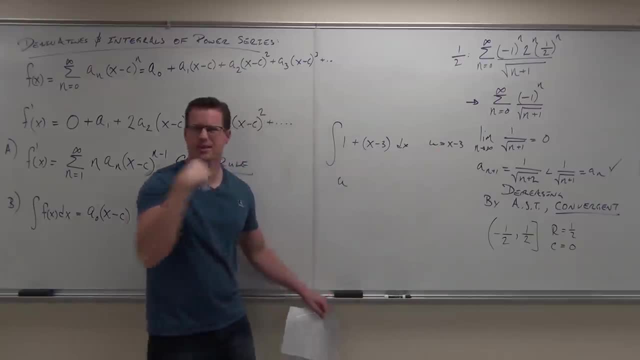 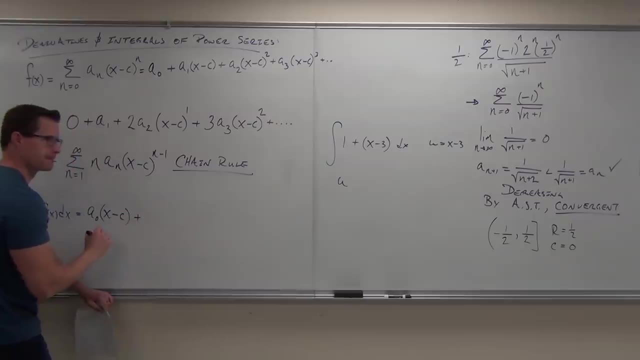 And when I did my u back to my x's, I'd get x minus three. Same things happen in here. Does that make sense to you? Okay, so we get a. okay, no problem. What's the next one then? 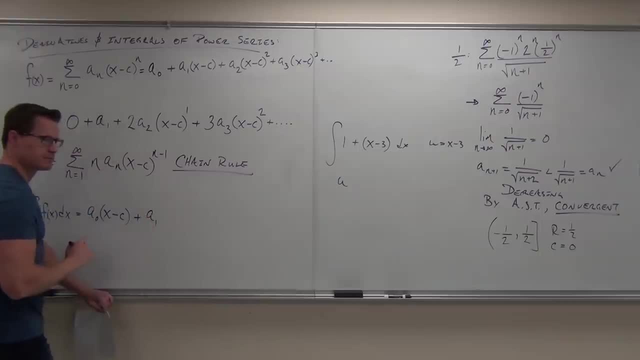 Oh, come on, A sub one. A sub one, That's gonna: yeah, Y half, Y half. Am I gonna have an x minus c? Yeah, What powers are you gonna be raised to? What Square Over? 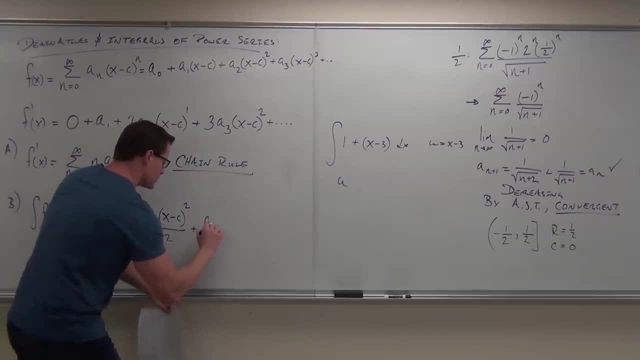 Two, Two, Next one Over two, X minus c, X minus c Over three Over three, And so on and so forth, which looks like this: The integral of f of x dx, therefore, would simply be a series. 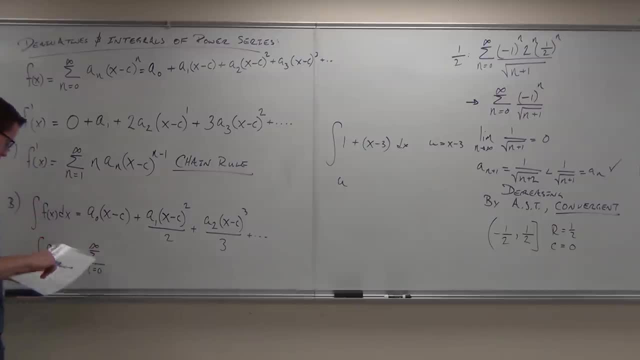 This one does start at zero. still We get a sub n. We get x minus c to the. let's look at what happened into our power. What's happening every single time? We didn't even have an x minus c. Now we have one to the first. 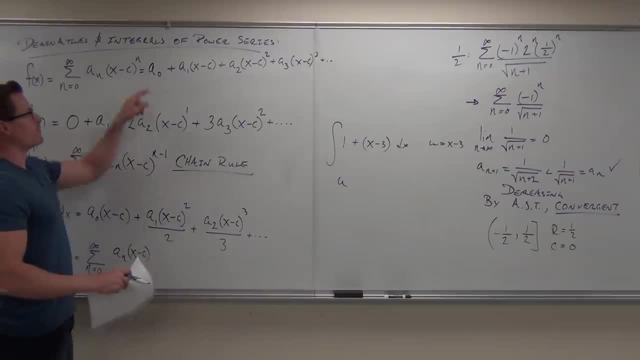 We had an x minus c, but now it's to the second. That's right. Over one Over one, That's right. Does that look familiar to you? That's our basic integration rule. It just says: hey, you know what happens here. 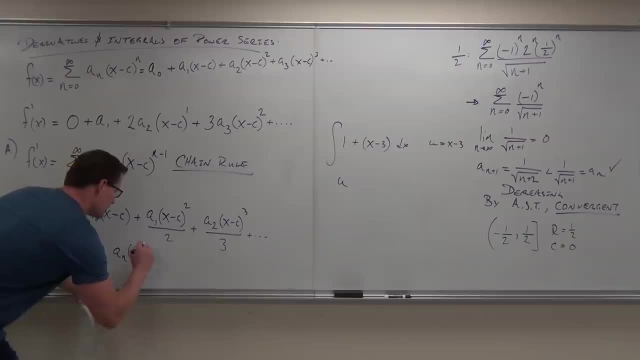 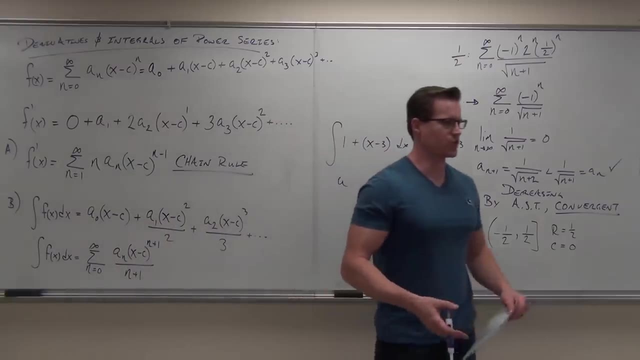 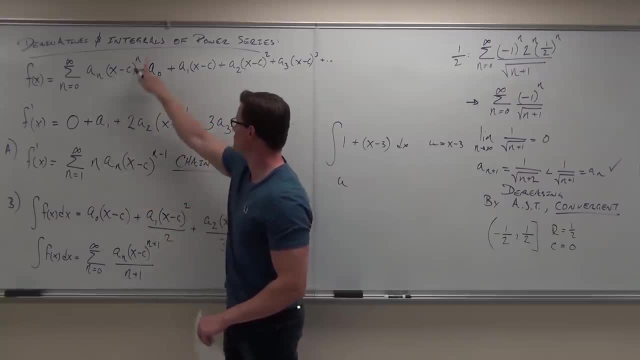 You add this, You take this, You add one to your exponent Bam, You divide by your new exponent. Got it? We don't need to worry about the x minus c, because when you do a substitution it's like the most trivial of substitutions. 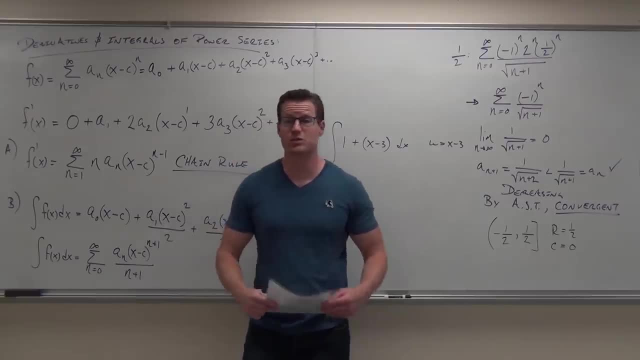 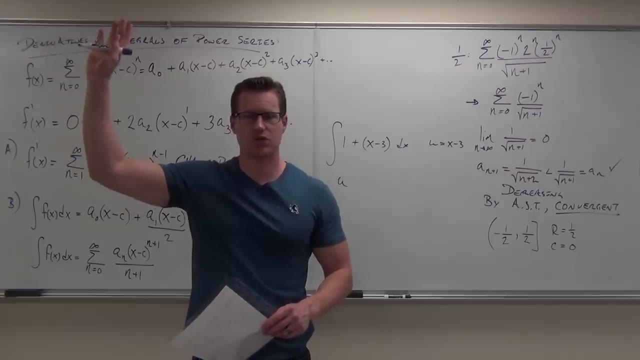 The derivative of x minus c is one. Therefore, your dx is a straight substitution to the du. whatever you use for your substitution, We got it. Chopin should be okay with this so far. You shouldn't. There's one thing I'm missing. 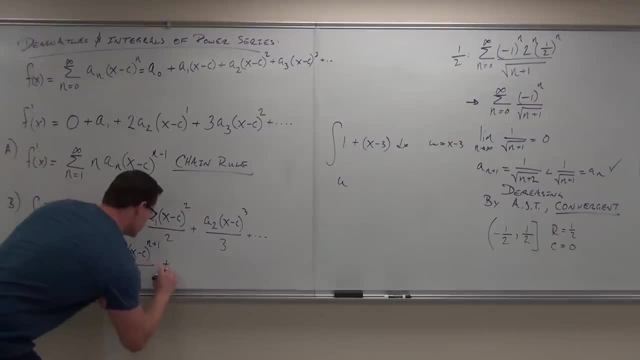 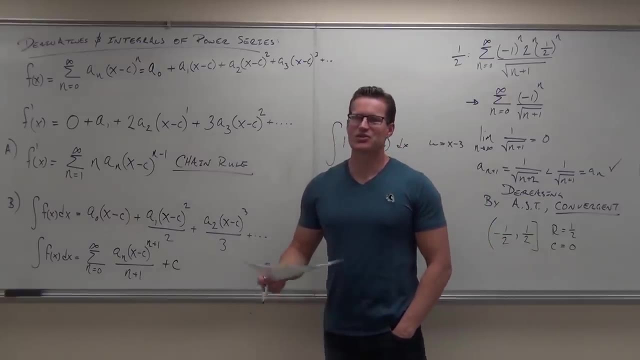 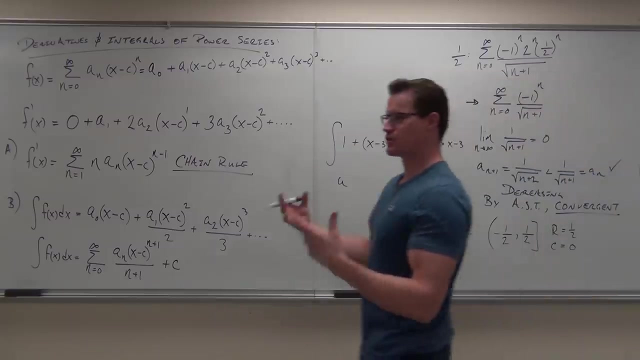 Plus c. Ah, Aha, Aha, Don't forget the plus c. You see, You see, You see, Now there is one other thing that can happen. You see, all of these series start out with an interval of convergence, right? 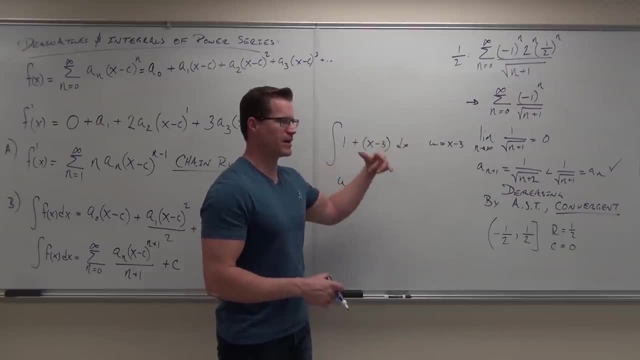 Some domain. So it's like from like. we had before negative one half to one half, where sometimes the end points are included and sometimes they're not included. Now what can happen is if you do a derivative or if you do an integral of your power series. 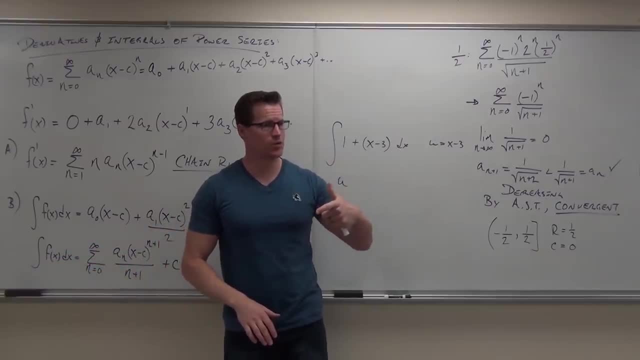 you can lose end points or you can gain end points. What's interesting is, the interval of convergence will remain the same. The interval is the same, but you can lose end points on derivatives and you can gain convergence of end points on integrals. 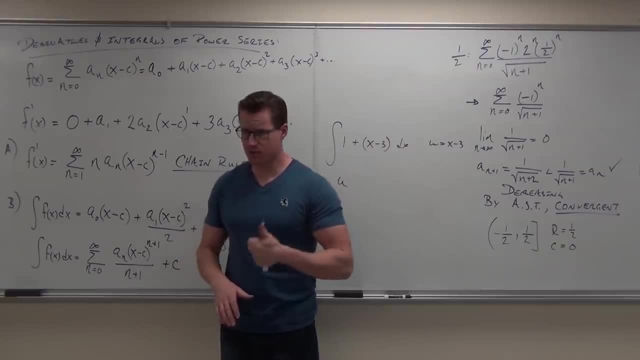 Does that make sense to you? So it's really. it's kind of an interesting idea. but when you do a derivative or integral of your power series, all you need to know is that the interval is not going to change, But the end points might. 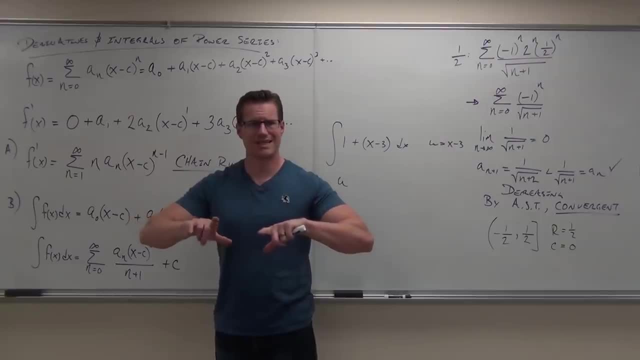 So be careful on that. one Chopin should be okay with the idea. Now I'm going to show you one example on how to use this very quickly. So you can do this, You can do this, You can do this. 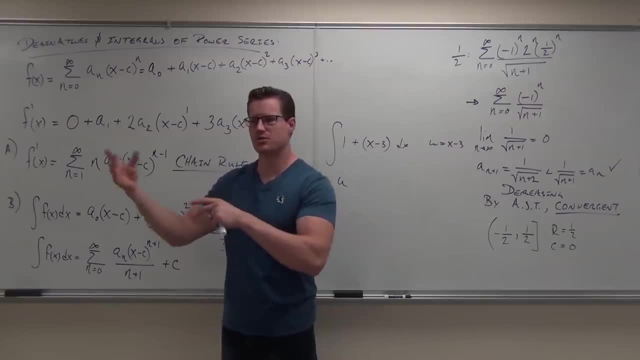 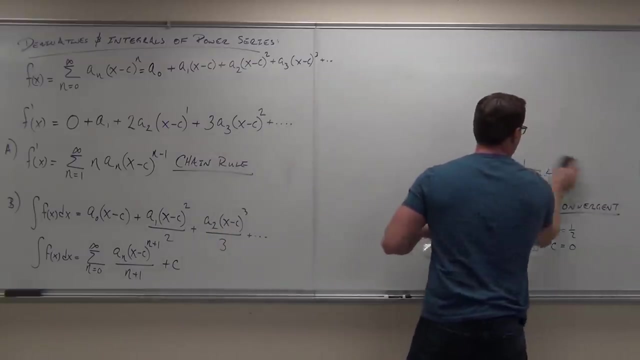 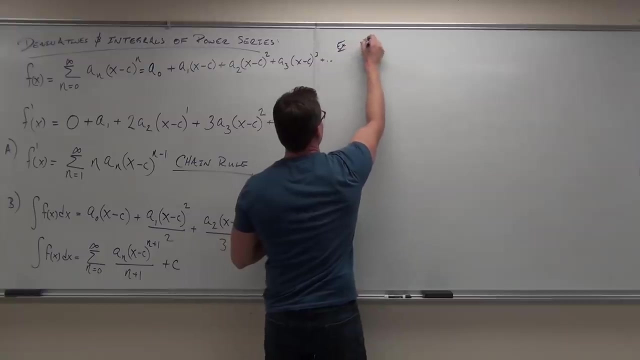 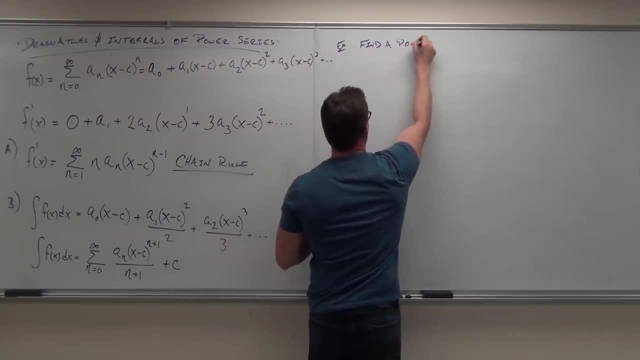 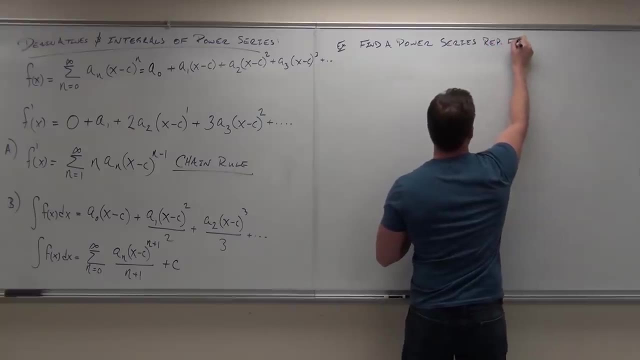 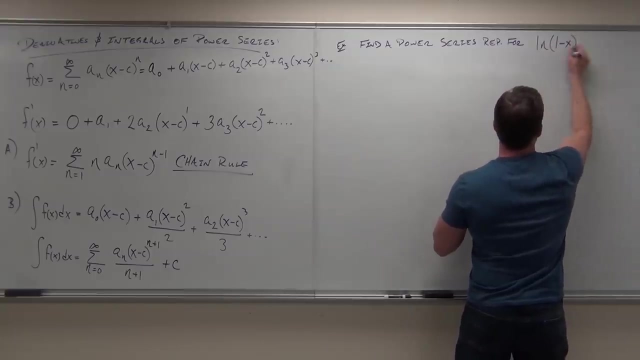 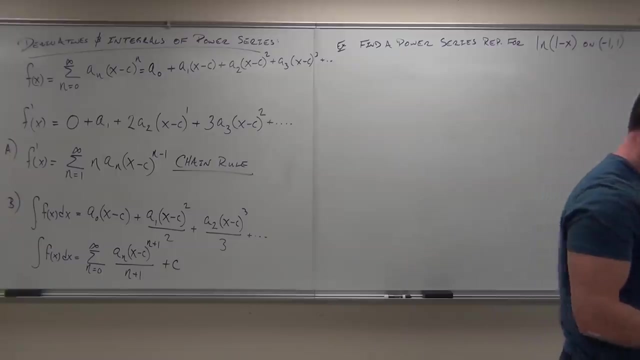 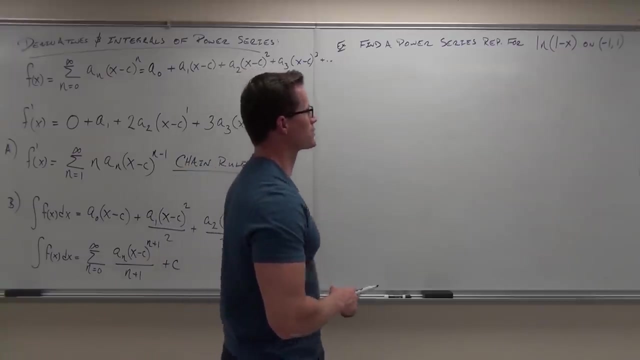 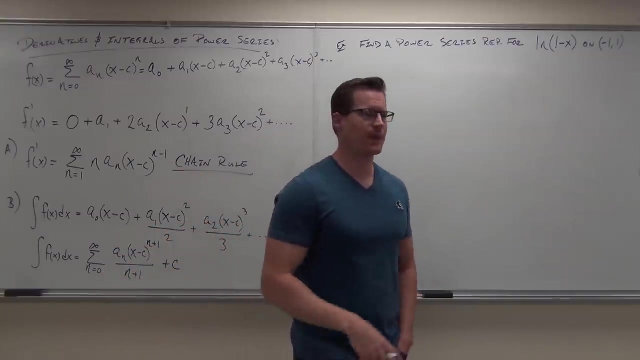 Okay, a power series representation for this, For ln of one minus x on the interval negative one to one. A power series representation for that thing. What we're going to do is we're going to use this idea to do that. So here's the start. 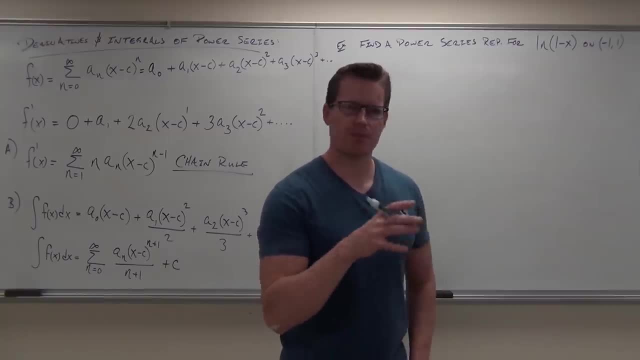 Are you ready for the start? I'm looking for some function that when I take a derivative or an integral of it, it gives me ln of one minus x. I'll say it again: I'm looking for some function that when I do a derivative, 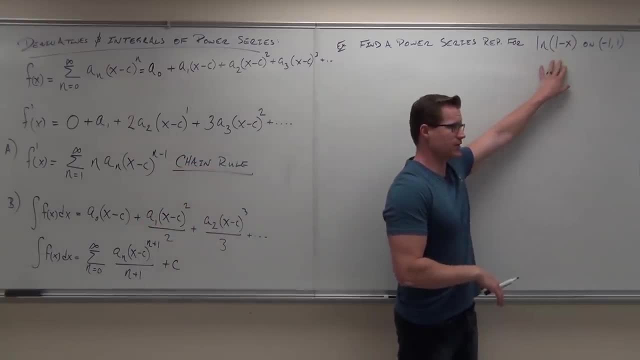 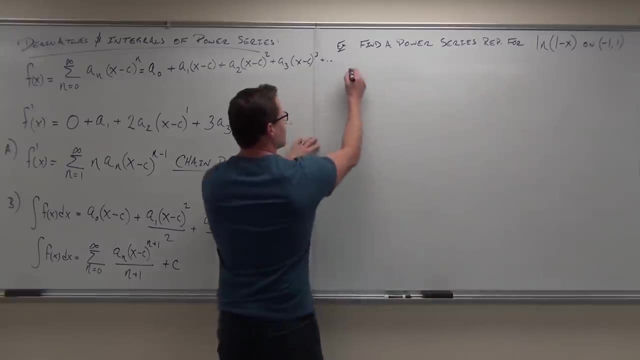 or an integral. it gives me this thing right there. Does that make sense to you? Now I'm going to cut to the chase because we're running out of time and I want to make sure that you get this. Well, here's the deal. I know that if I start with one over one, 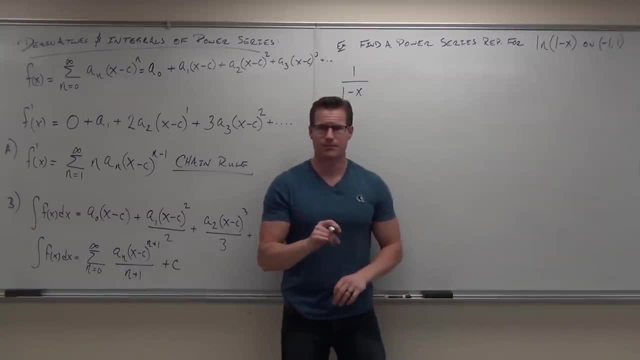 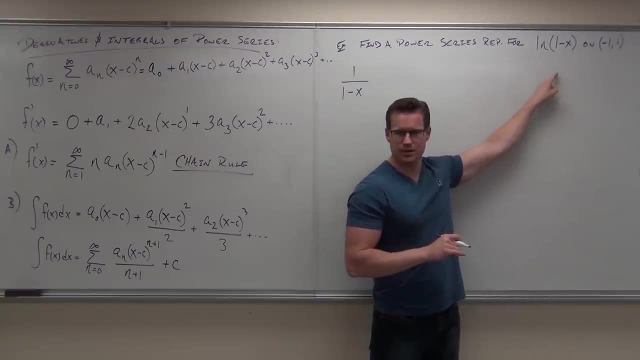 minus x and I do an integral of that thing. the integral is going to be pretty darn close to that. Do you see that It's going to be negative, but it's going to be pretty darn close. Are you with me on this, folks? 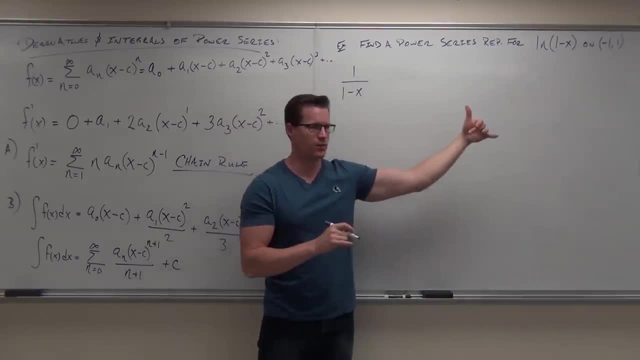 So the integral of this thing gives us negative ln of one minus x Quick hit, and I'll be ok with that. Now, the other reason why I'm choosing this one and why I'm not saying, well, it's only something that I can do, a derivative for that I'm also trying to make. 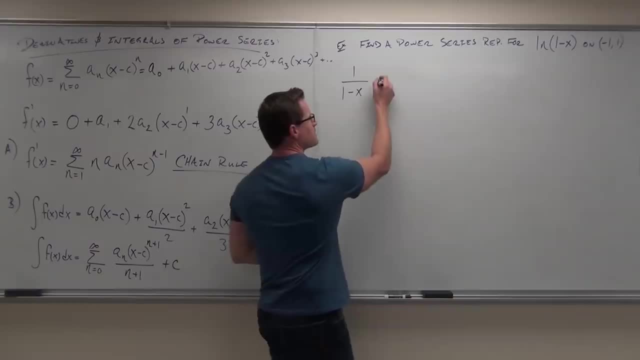 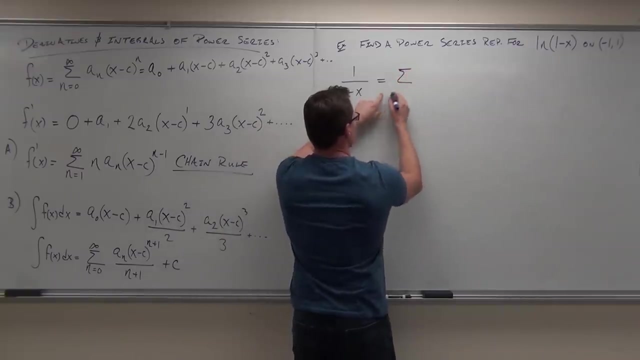 a series representation. What I know is that this thing right here, this is so cool. this is the sum of a? what type of series? Geometry, Do you see it? This is the sum of a geometric series. This is the sum of a geometric series. 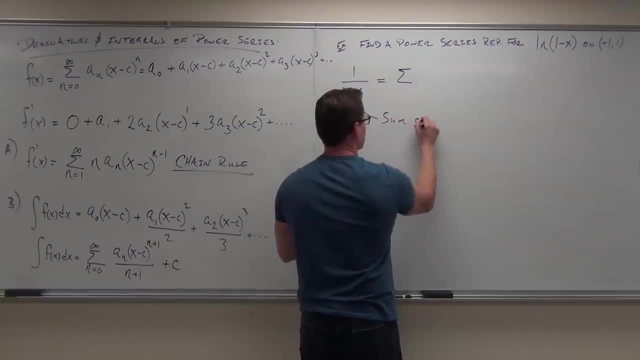 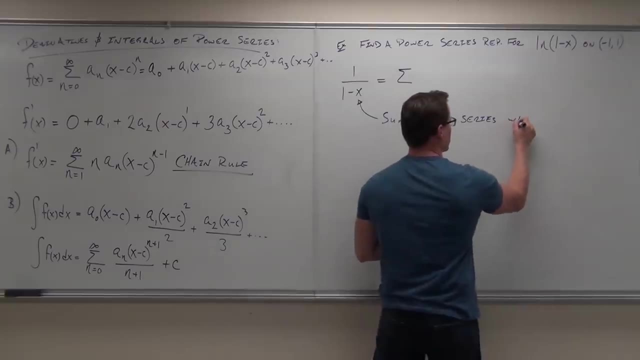 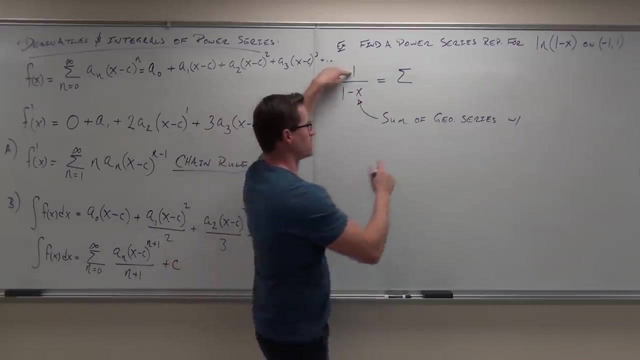 Geometric powers Of a geometric series with. ok, you tell me if this is a geometric series, what's my a? 1. Very good, a is right here. What's my r? x? Therefore, this is a geometric series with n equals. 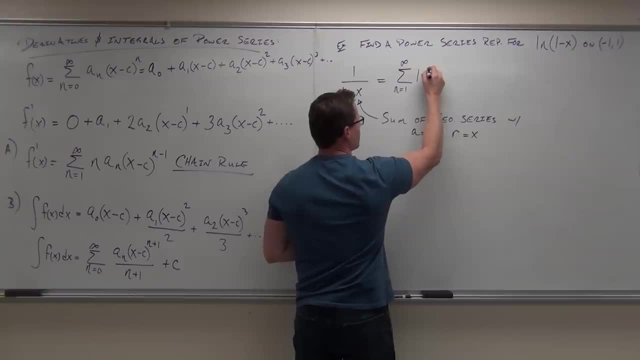 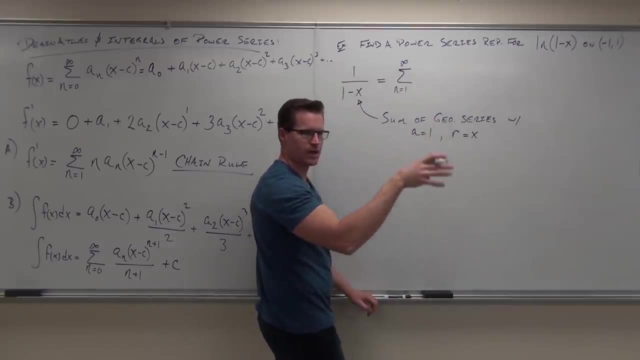 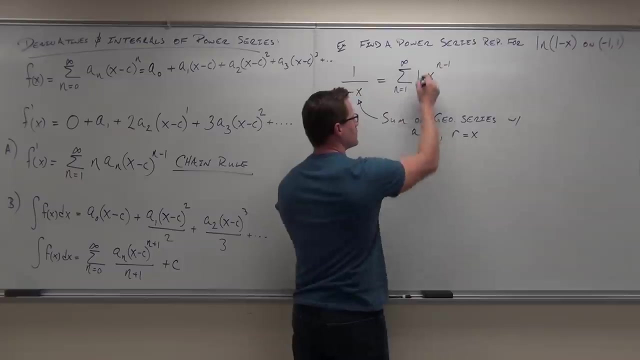 1 to infinity of 1. What else? Do you remember how geometric series look? Geometric series look a r to the n minus 1.. So a times r to the n minus 1.. That's it, That's my geometric series. Ok, well, that's cool. 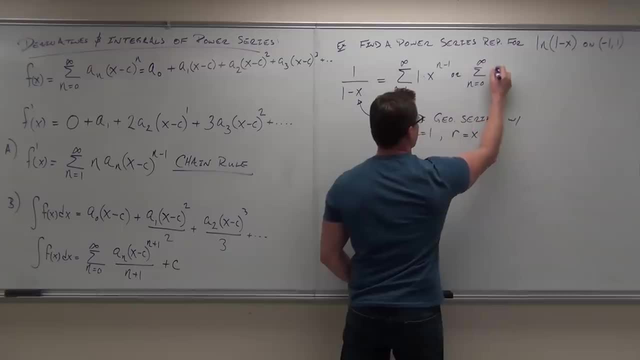 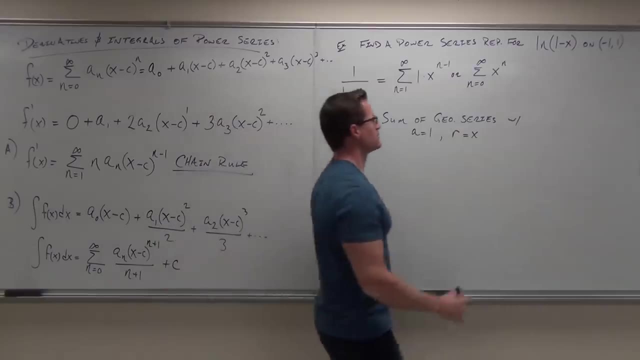 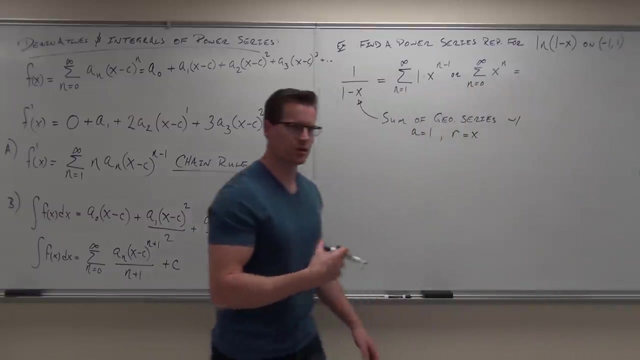 Or you could do it this way if you wanted to. We all see it this way. n equals 0 to infinity, of a x to the n, Either way, In both of these cases. in both of these cases, what do the terms of your series look like? 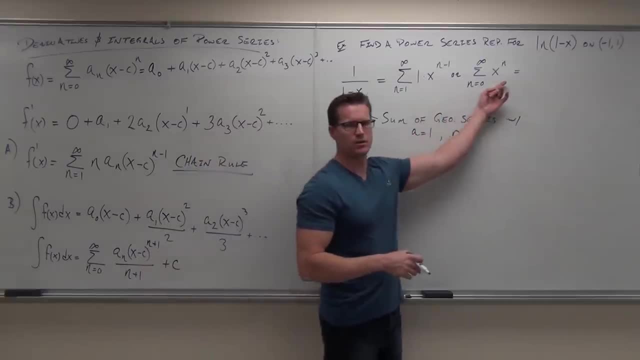 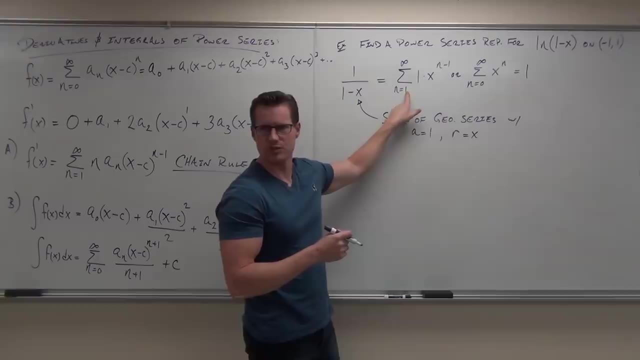 What's the first term here? 1.. Good Notice, the first term here would also be 1.. So I don't care how you do it. either way, This one's a little easier to see, ok, But either way, If you did it, you'd probably raise to 1.. 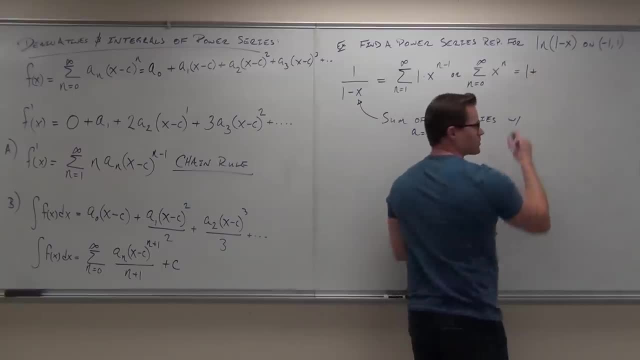 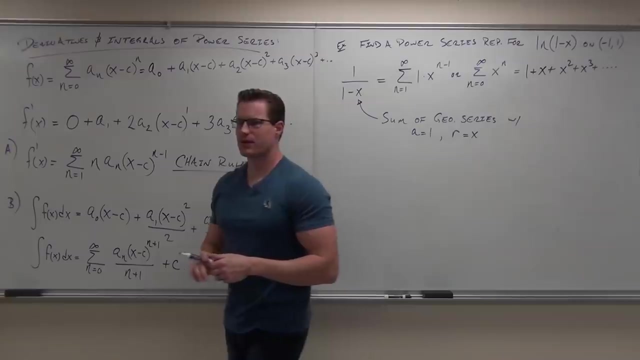 But if you did this, you'd still get 1.. Plus what's the next term? Come on, we gotta go quickly on this. one x to the Sure, Plus, what else, Plus, what else, Plus, what else, And so forth and so on. 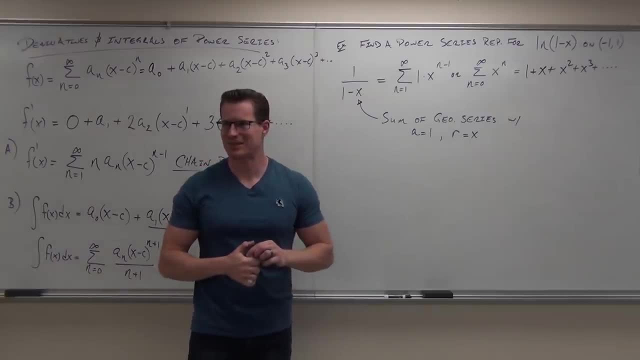 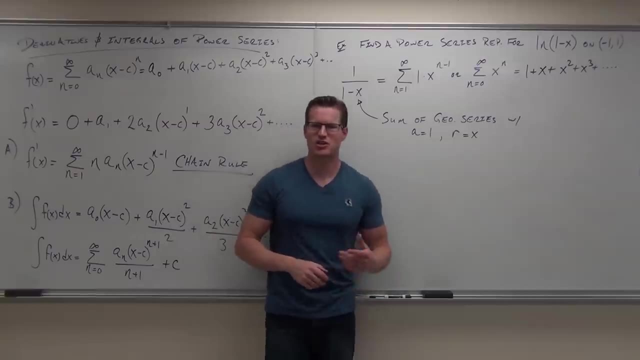 Ok, I feel like I've lost some of you. I've left you in the dust a little bit because I'm getting some blank looks and I never like the blank looks. You know, sometimes when I speak Spanish to my dog, he goes. 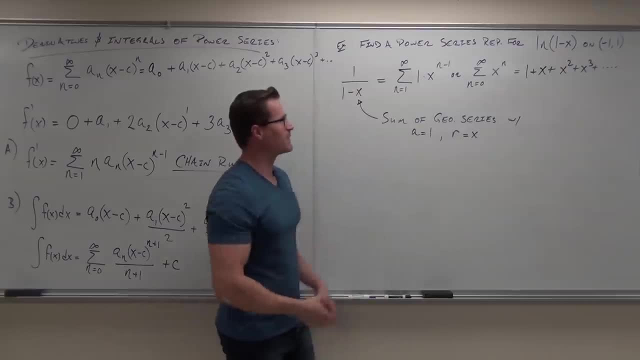 That was a little bit, never mind. Anyway, this is a little Greek, I get it. It's a little weird. Find a power series representation for that thing. What we're trying to do is say, hey, you know what, I've got a function that represents. 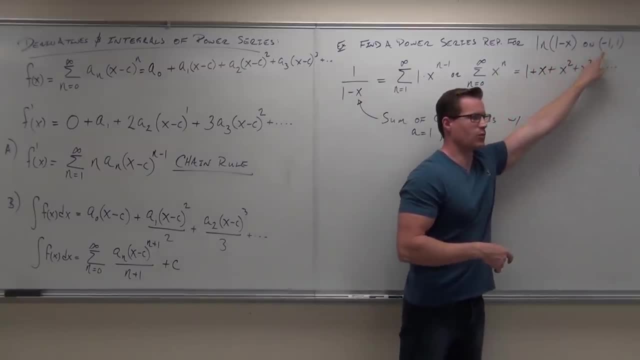 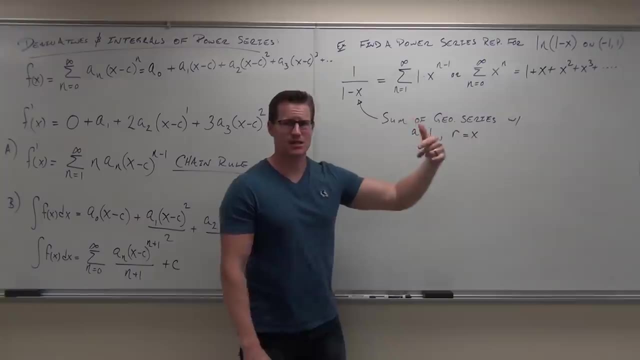 I'm sorry, I have a power series that represents this function. on that interval, We'll talk about why the interval is there right now. actually, First thing we do is say, hey, find me something that when I take an integral of it, 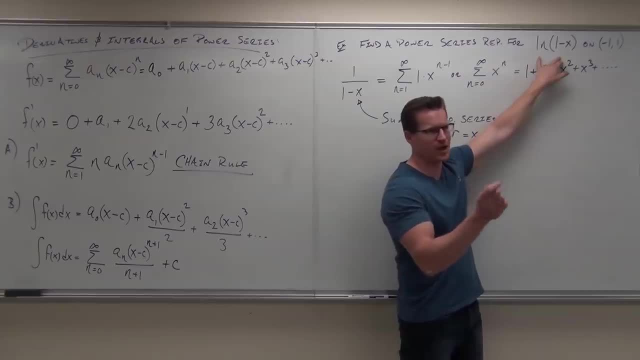 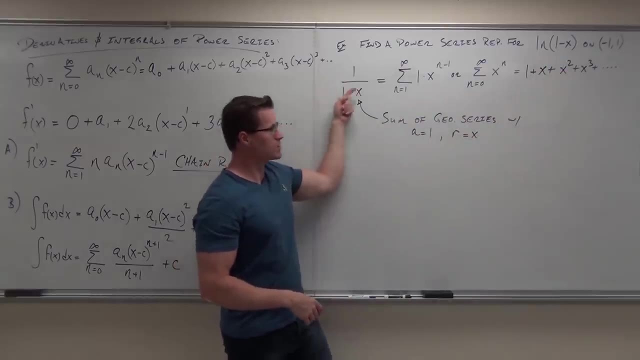 it gives me this thing Or that thing, with a positive or negative, I don't care, as long as it's this thing, because negatives I can deal with. Well, I know that if I integrate this, it is going to give me this. What I also know is that 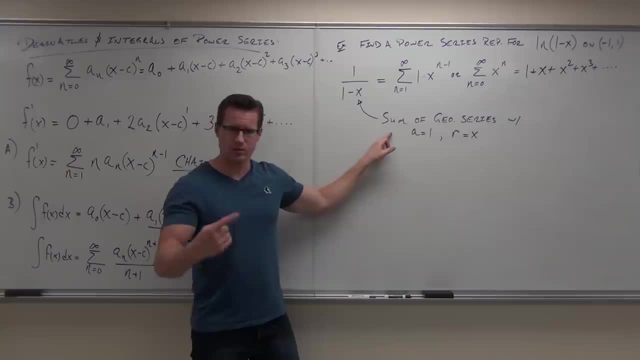 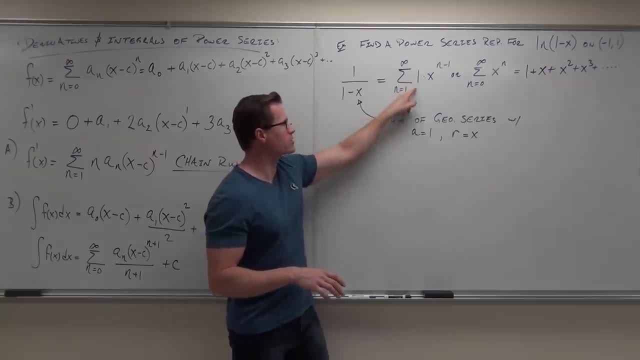 this thing is the sum of a geometric series with a equals 1 and with r equals x. Look up the geometric series. This is going to be apparent to you. Well, a geometric series is always one of these two forms. No problem, It's a. it's a. 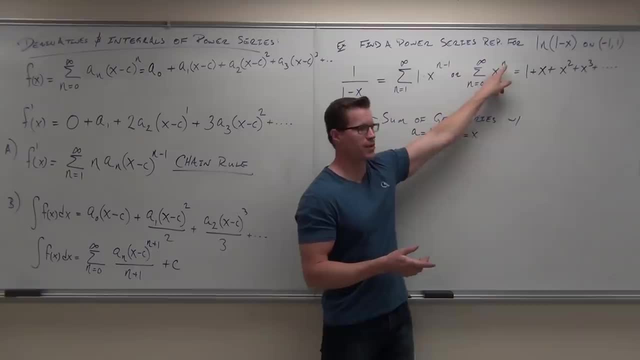 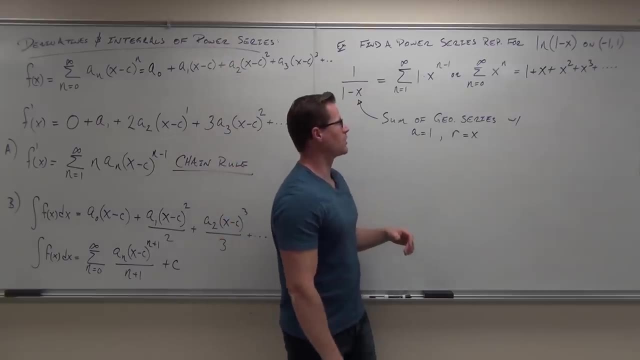 it's n equals 1 with n minus 1, or it's 0 with n and it's r to that power. That's exactly what we have right here, so eventually we'll be ok with that. Now those terms are 1 plus x plus x squared, plus x cubed, plus x to the 4th, plus blah, blah, blah. 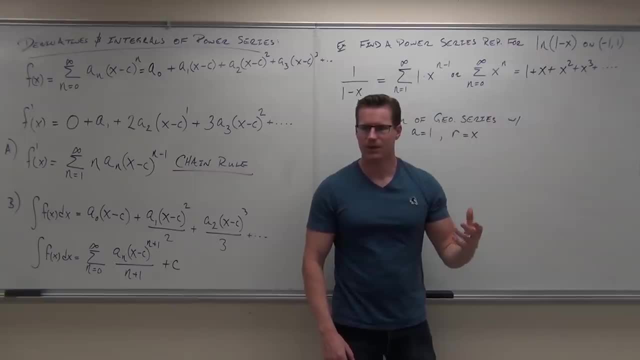 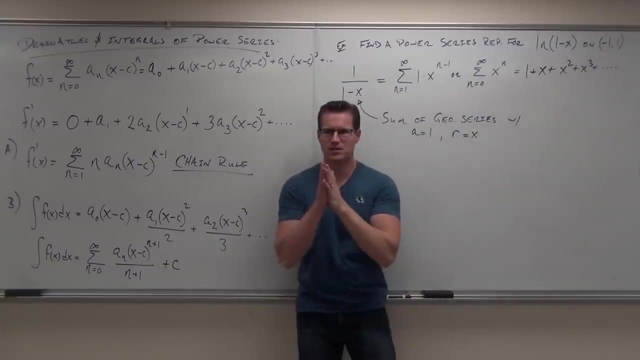 That's how geometric series look. Now can someone out there who's thinking critically explain to me why this interval is the way that it is? Why x must be between negative 1 and 1 for this, Because of absolute value of r is greater than 1.. 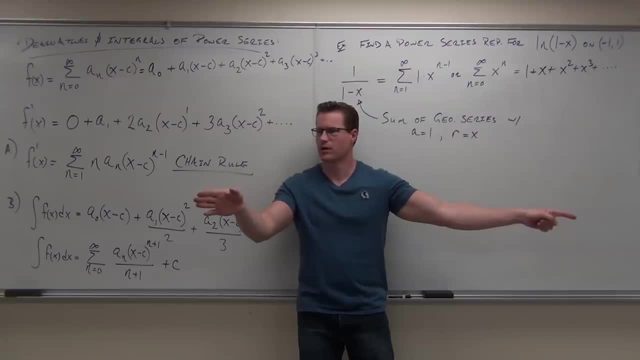 Why? Why is the absolute value of r less than 1 or greater than 1 important for us? Convergence or divergence? What type of series do we have? Geometric? So, if this, if this is not negative, 1 to 1,. 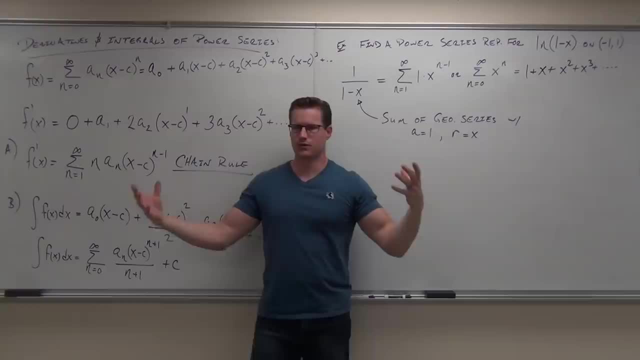 then my x, which is my r, would be outside of the interval of convergence. Does that make sense? Geometric series only converge from negative 1 to 1.. Hey, hey, it's a geometric series. so, because it's a geometric, 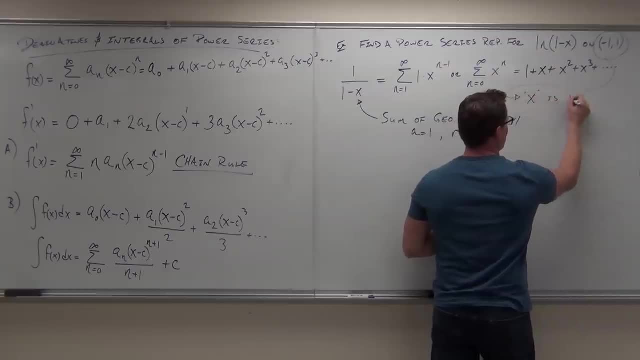 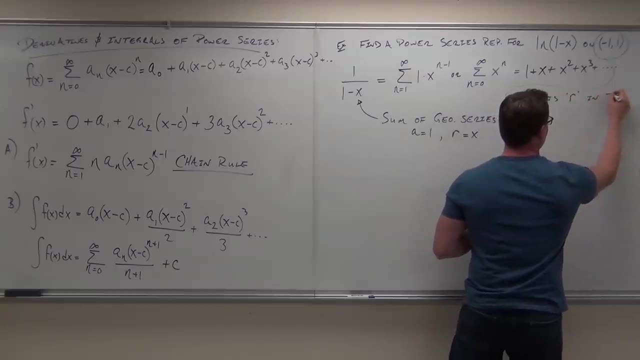 x is r. You know what different r? r in this case? Since r must be less than 1 for convergence of a geometric series, x must be less than 1 for the convergence of this geometric power series. I want to write that out because it's important. 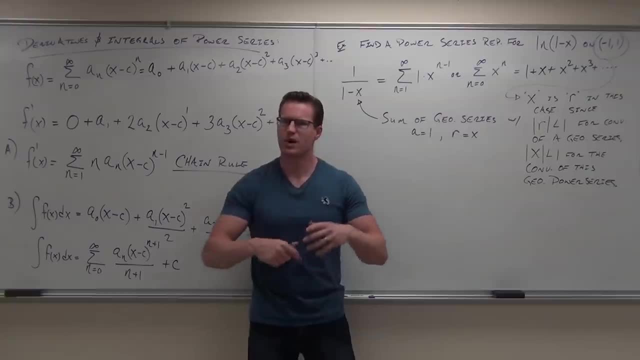 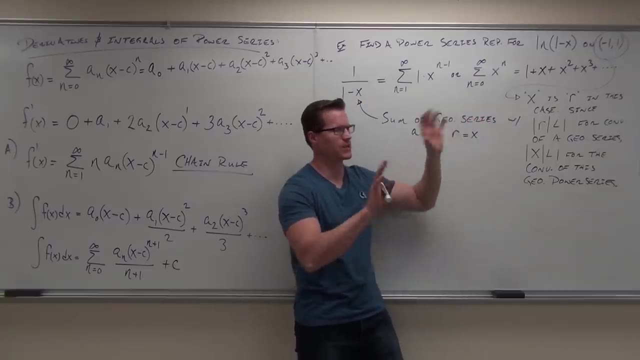 Make sure that you actually get that. Do you guys understand the concept here? The reason why this is defined only on negative 1 to 1 is because we are going to be using a power series to represent this. We have to use a geometric power series to represent this. 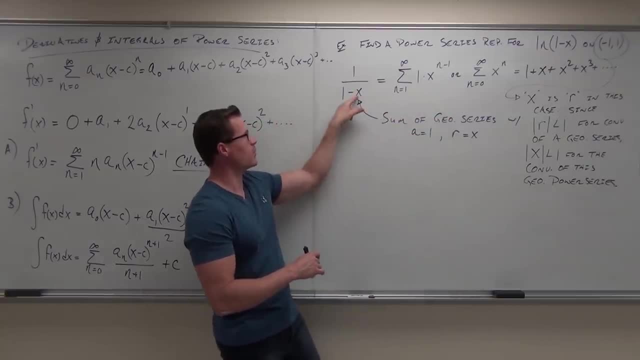 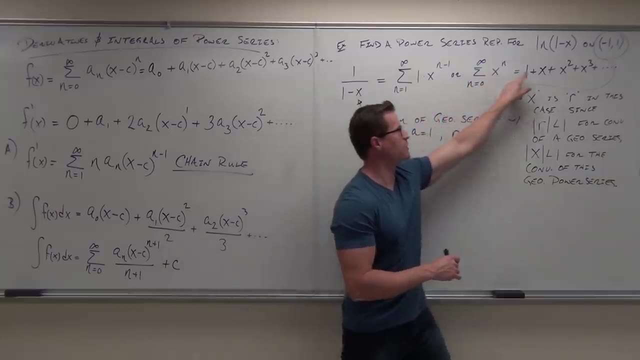 Because geometric series only converge when this number is between negative 1 and 1, it must converge when this number is between negative, okay, between. well, x has to be between negative 1 and 1.. That's the only way that this thing is going to converge. 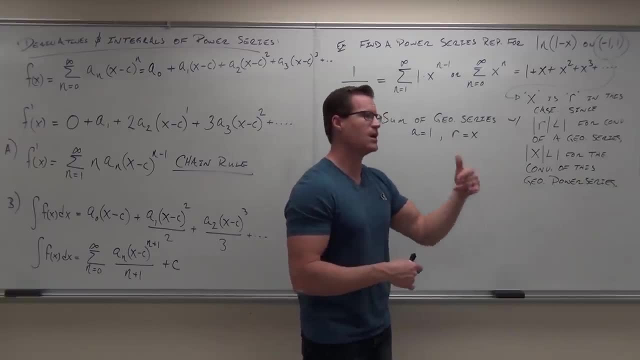 Therefore, it's the only way that we're going to get a function to represent this power, a power series to represent this function. Power series only represent functions where the series converge. Therefore, we have to have an interval for which our power series is going to converge. 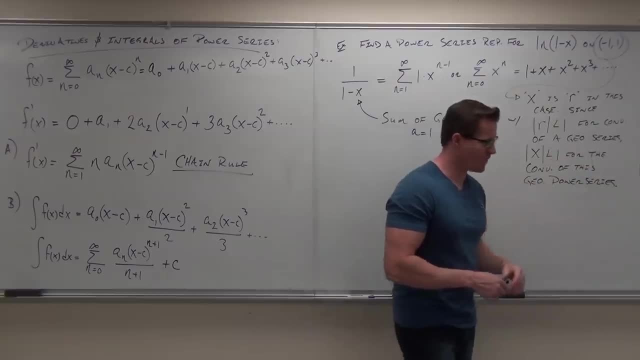 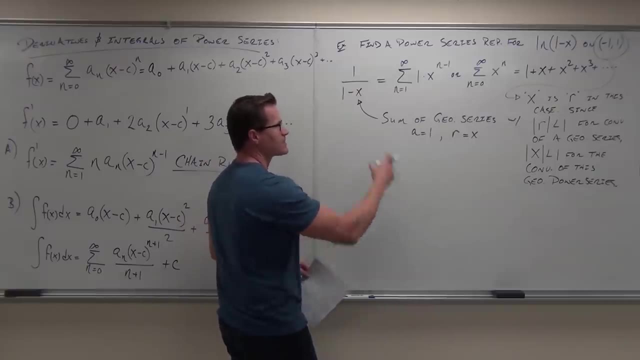 to represent this function. Does that make sense? Okay, Almost there, Very, very close to almost there. Well, what we have right now is this We got. this is the sum of the power series. This power series looks like this: 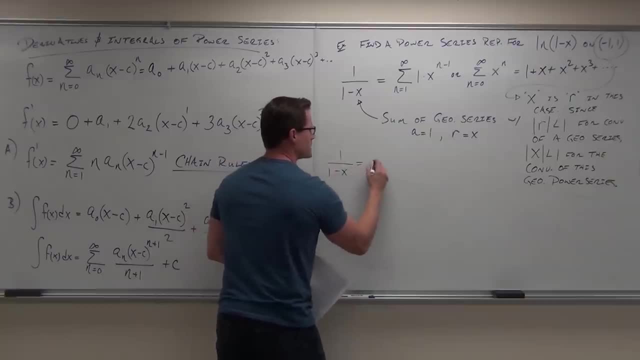 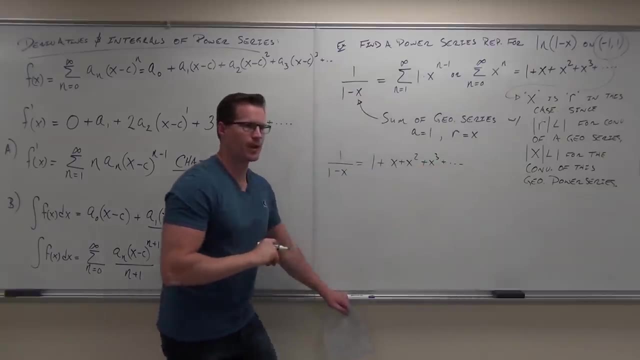 Therefore, 1 over 1 minus x is equal to 1 plus x plus x squared plus x to the third, plus forever and ever and ever and ever. What I also know about equations: can you guys make the jump with me? What I also know about equations: 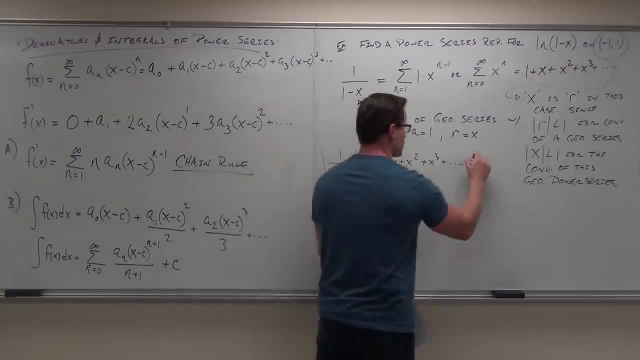 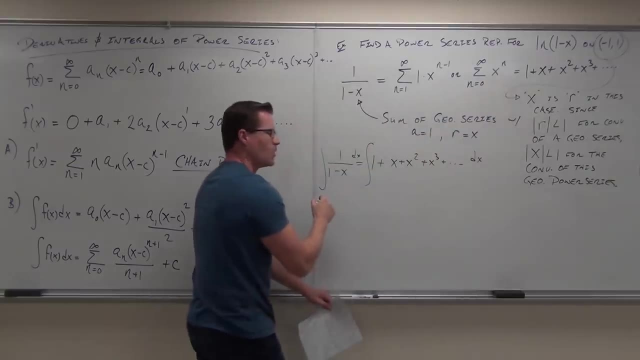 I can integrate both sides And since I know how to integrate a power series, I can integrate term by term. That's why we're making this jump. We're saying, hey, integrate that term by term. Well, check it out. 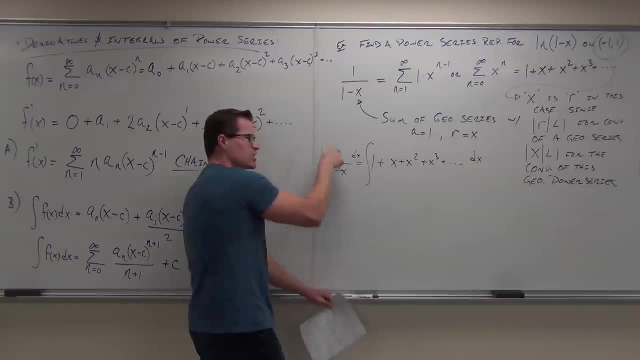 What's the interval of 1 over, 1 minus x? It's really not. It's not ln, it's not this, It's not that It's close, but it's not that It's negative. Do you know why? 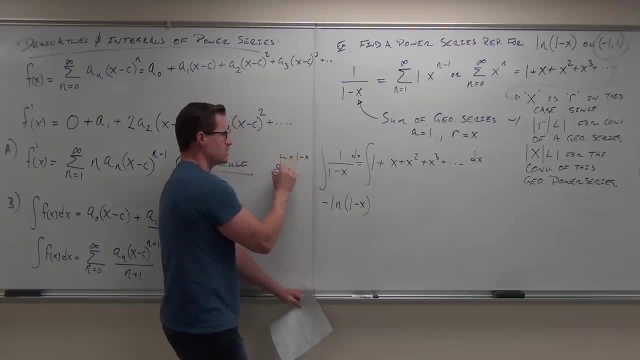 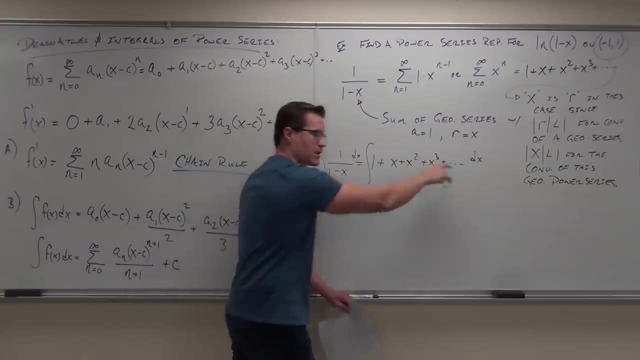 You have a u sub 1 minus x, du equals negative dx. That gives us that negative. Does that make sense? Now, I'm not going to do a plus c here. I am on the other side. I'm not doing a plus c because very similar. 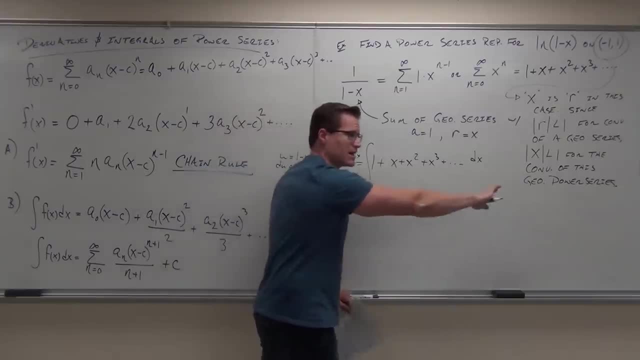 to our differential equation section. if I did a plus c, I could just subtract it and get a different constant. okay, So I'm not going to worry about it Here. I'm going to get x plus x squared over 2 plus x to the third over 3 plus blah, blah, blah, blah. 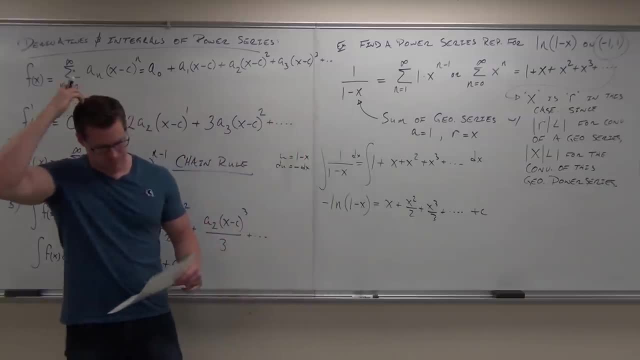 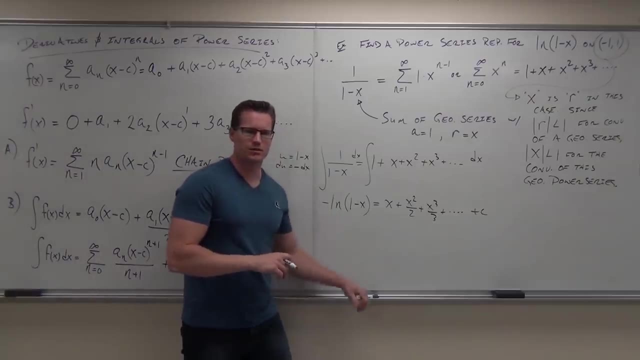 and then plus c at the very end. So close, almost done. Tell me what I can do with that negative. Say what now? If I divide by negative, all these signs are going to change. I'll get ln. 1 minus x equals negative. x minus x squared over 2. 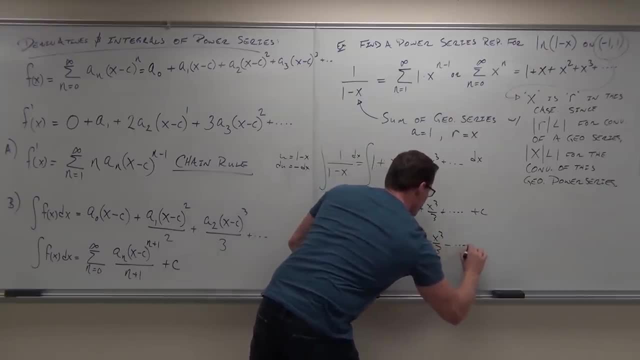 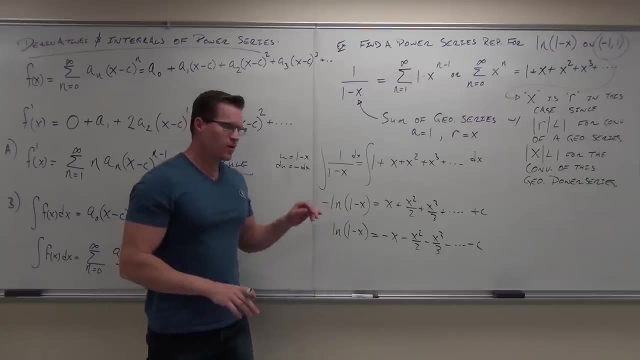 minus x to the third, over 3 minus, blah, blah, blah minus c. So close, almost done. We've got to find out what c is equal to. So if we want to find out what c is equal to, it's pretty easy to do. 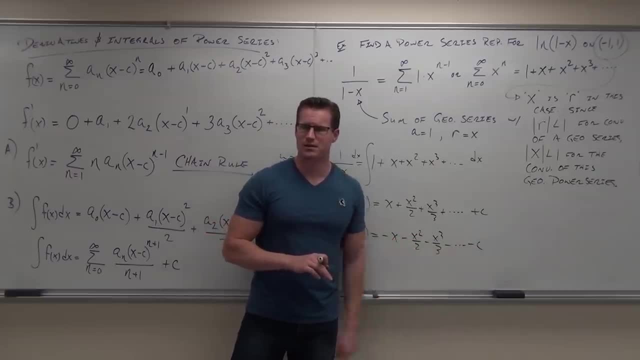 Do you understand that every single one of these terms are going to have an x in it, except for my c? Plug in x equals 0. If you do that, everything goes to 0, except for my c. So if I let x equal 0,. 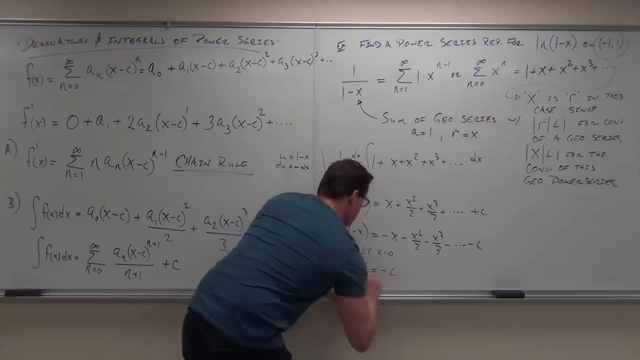 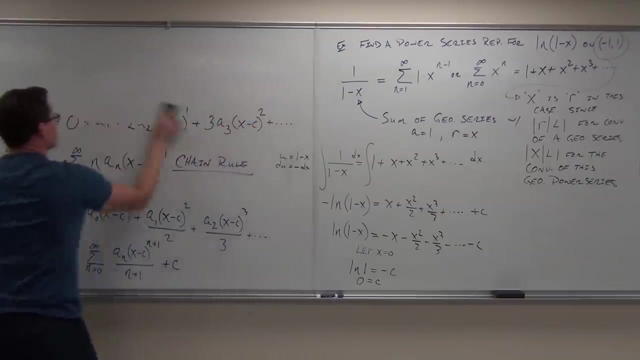 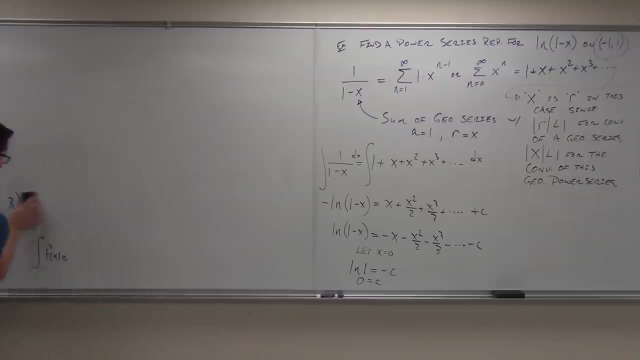 I get: ln of 1 equals negative c, ln of 1 equals negative c. How much is ln of 1? 0.. So then 0 equals c. Okay, So ln of 1 minus x equals negative x minus x squared over 2. 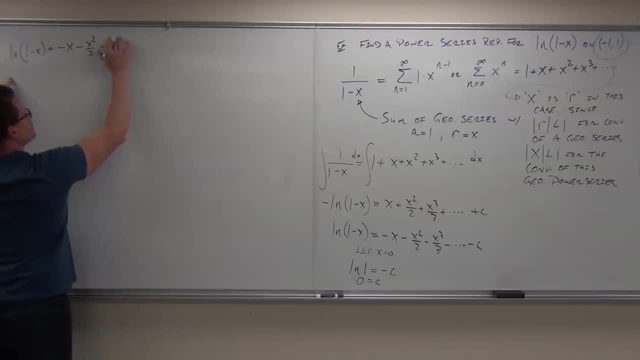 minus x to the third over 3, minus blah, blah, blah. but no plus c. If we factor out that negative, which we could have done from the very beginning, we could have had negative x plus x squared over 2 plus x to the third over 3, plus blah, blah, blah, blah, blah. 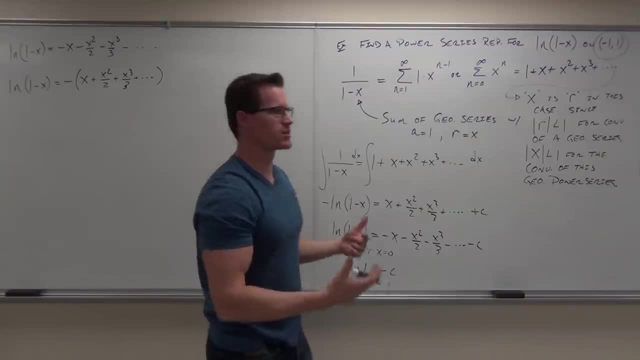 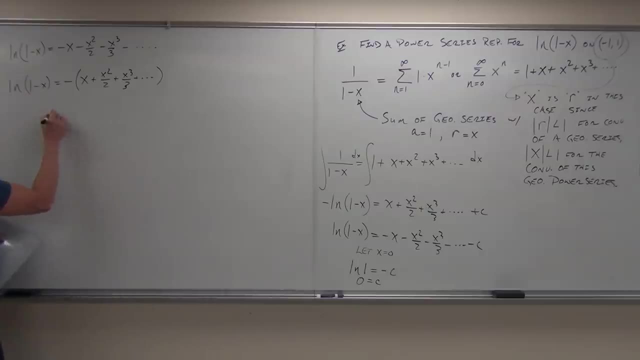 All we're going to do is find a series representation for that thing and it will be done, And it's really easy to do What this is. Can you represent that thing as a series? Probably x. x is going to be up there somewhere. 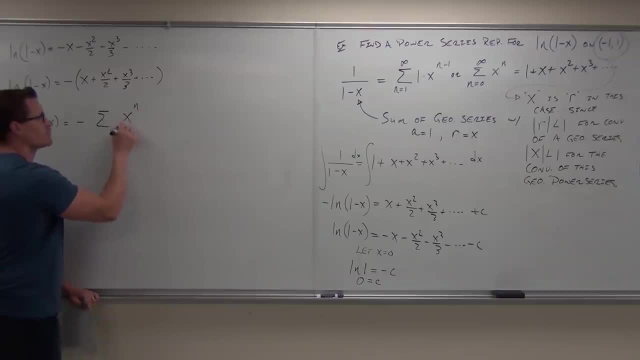 Yeah, To what Over? n? Yeah, Do you guys see it? 1, 1,, 2,, 2,, 3,, 3,, 4, 4, n? n? Where's n start? It starts at 1.. 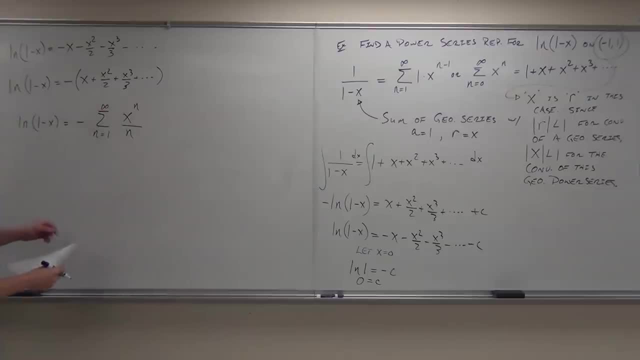 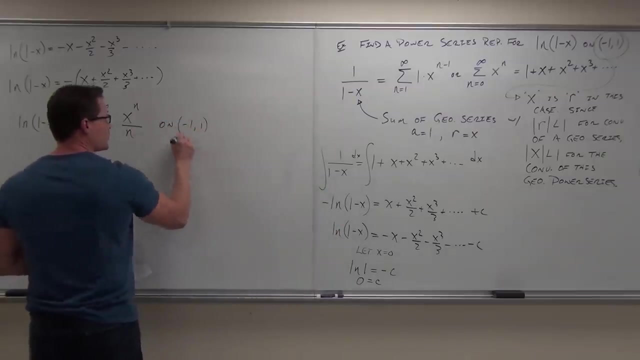 It goes to infinity. So here's what we know. We can represent this function, ln of 1 minus x by this series. on what interval? Negative? 1 to 1.. Why was negative 1 to 1? important Interval convergence. 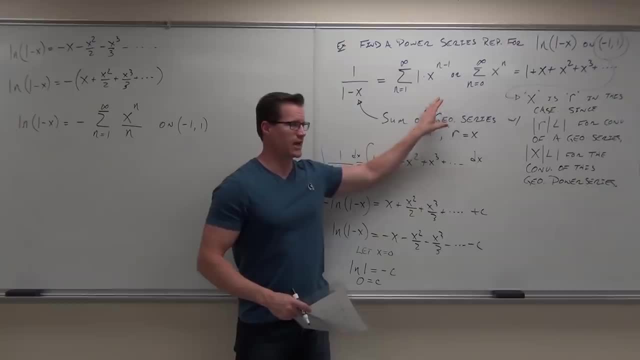 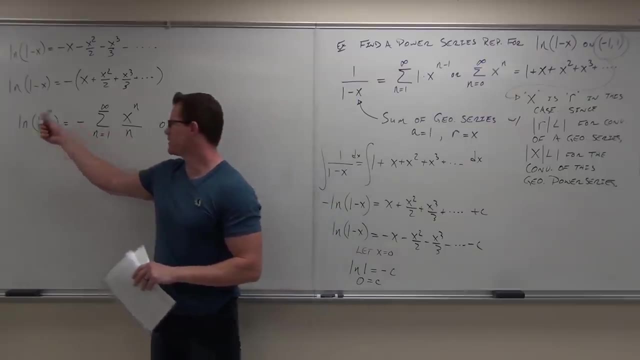 Because that's really a geometric series. That's where we got this from. We can't define it other than that. So what this says is that, on negative 1 to 1, this thing is going to converge and it will represent this function. 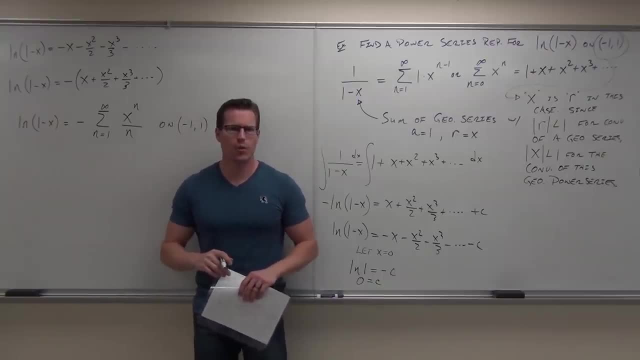 So if you wanted to find out, hey, what's ln of 1 minus 1 half, you could actually plug in 1 half here, here, here, here here, and do it for infinity and it's going to be exactly the same thing. 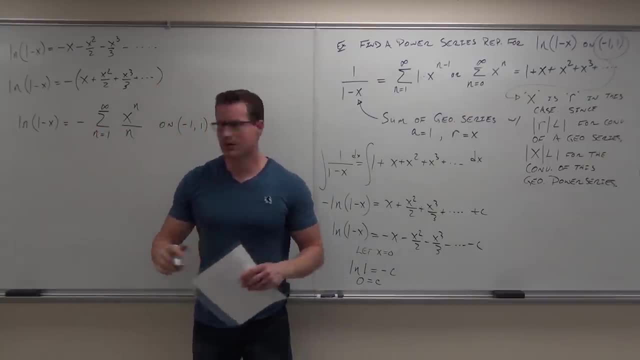 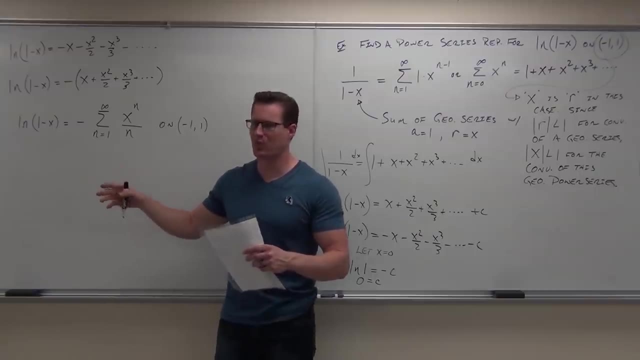 It's going to represent that function exactly on this interval, as long as you go n to infinity. Does that make sense to you? This is kind of out there stuff, but what we just did is we took a function and we used a power series to represent that function. 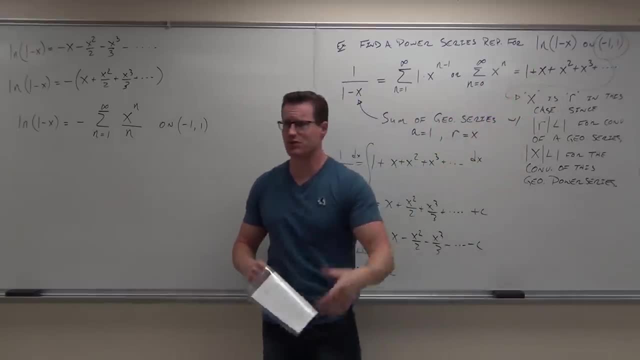 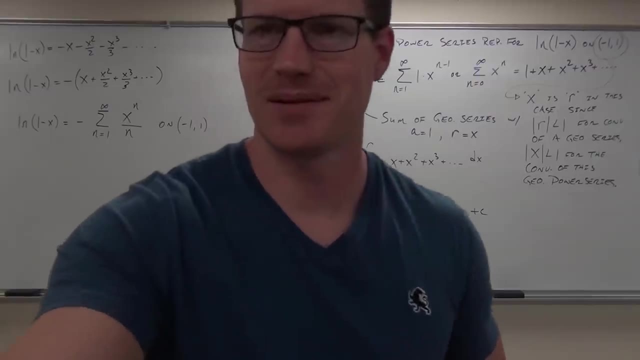 on a given interval for which our series converges. Show of hands, if this one made sense to you. Okay, Any questions or comments at all before we stop? All right, All right.